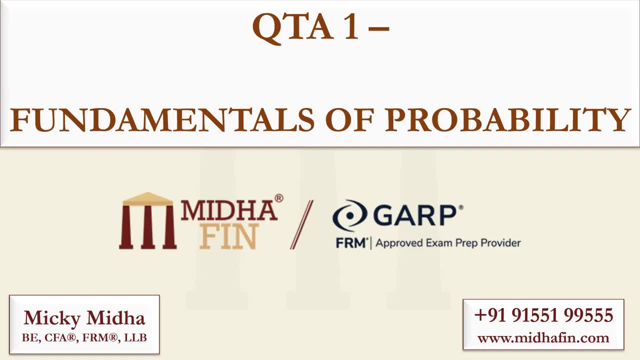 for your thoughts and having discussions. This time, however, we need to keep those interactions to a minimum to cover everything quickly. Also, I would like to request all of you to keep your comments in the comments section of this video, So, if you have any. 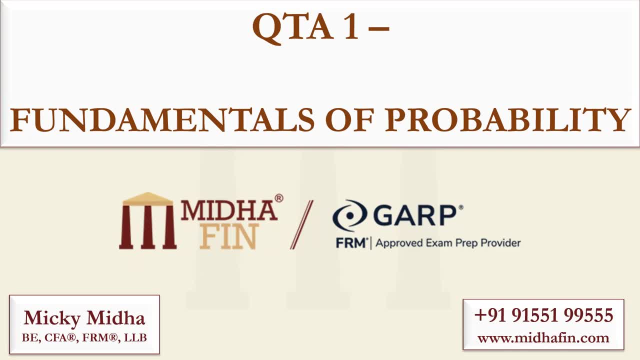 information about your topic or topic profile, tell me in the comments section below. We also want to make sure the videos are turned off during the class, as it might interfere not only with the bandwidth but with the PPT as well. The interface should not get disturbed. 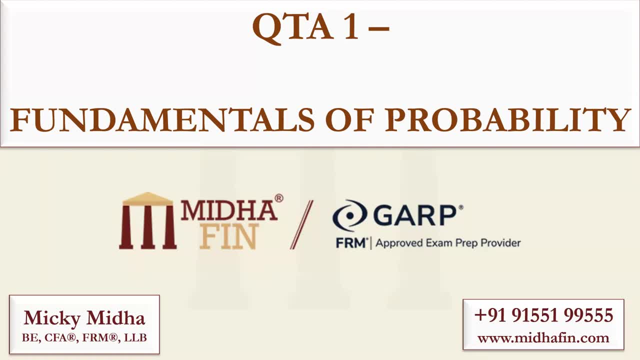 at all, And the good news is that you don't need to take any notes, So don't worry about writing anything down during the sessions, because all these slides will be available as PDF format in the same learning management system in which you are enrolled, which will be complete. 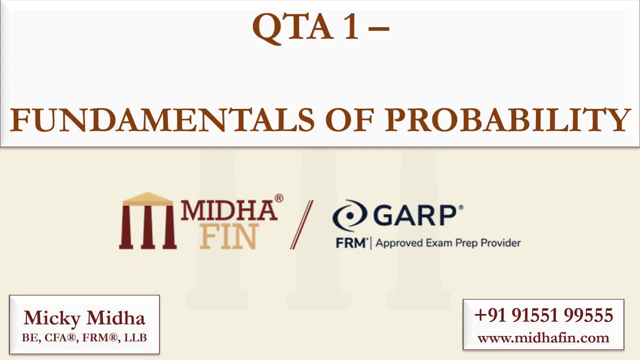 with all the text and all the annotations that you have. All right. Thank you, guys. so much are required also since we have to cover all the four modules over the next few weeks, say four weeks only. so each class it might be four to five classes in total, so each class will last between: 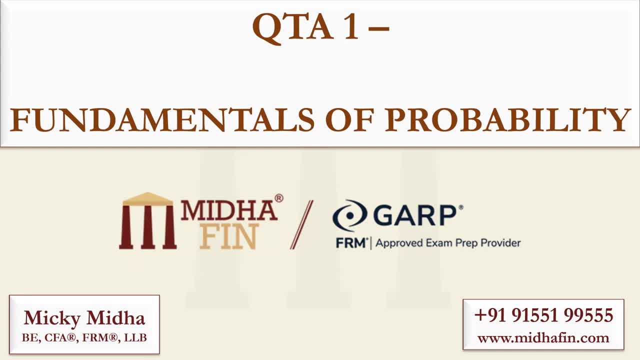 five to seven hours on an average. okay, so i can understand that it's it's like a marathon, but as far as the exam is concerned, it's actually a great practice, because exam you all are aware of, it's a four hour long exam. so this class will actually help you to. you can say, build exam. 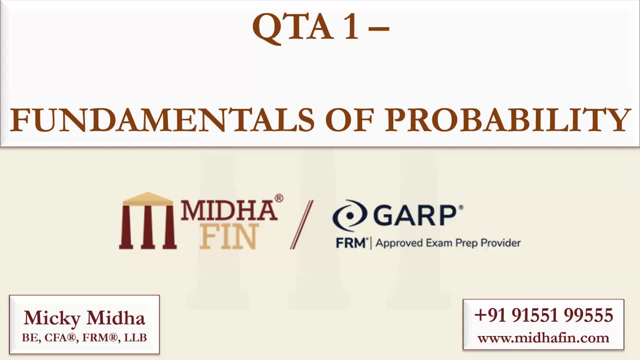 temperament, you will get used to sitting and focusing for extended periods right just before the exam. so, yes, these long sessions will be very challenging and you might be tempted to leave early, of course, but staying for the full session, i think, is very, very important, because- see for 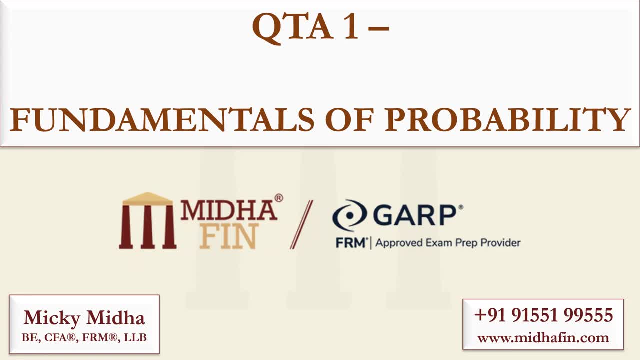 the exam. finally, patience, resilience, endurance- all these things are the key aspects, and being present throughout will actually help you, you know, become confident that you are fully prepared. and you are confident you are able to reinforce your learning properly, also one thing that i have taken care of. 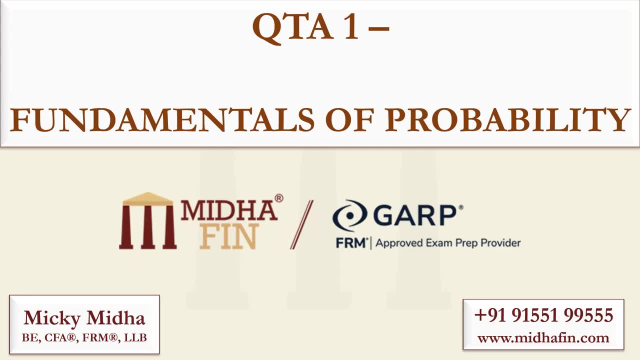 given the recent trend of increased theoretical questions, because, if you see, starting from- in fact, this trend started from 2018 only, even before the syllabus was changed in 2020- that the number of theoretical questions actually increased over the last few years, and this has actually been. 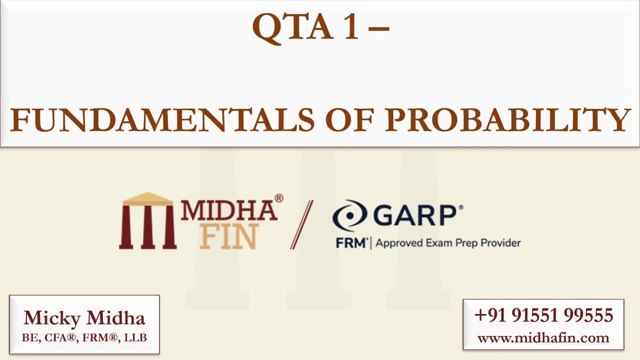 even more uh enforced and more emphasized after 2020, after the change in the curriculum, even for conceptual topics. say, let's say there's a topic in regression diagnostics with respect to the white test for heteroscedasticity. now, instead of performing the full calculations in the exam, 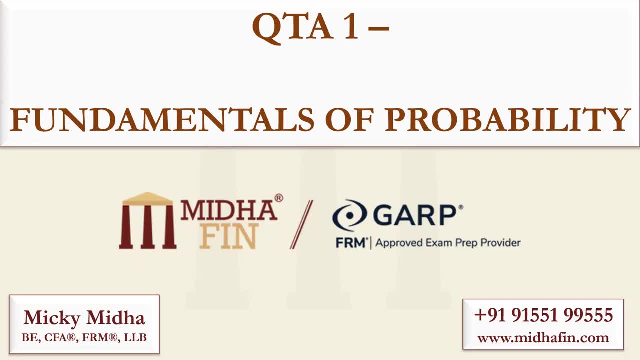 they probably will ask you, uh, the steps of the white test. i mean, if you see there are questions, not only in the graph- sample paper questions, uh- but also based on the feedback that we have got to our candidates, that steps of those tests were asked rather than the complete calculation. so 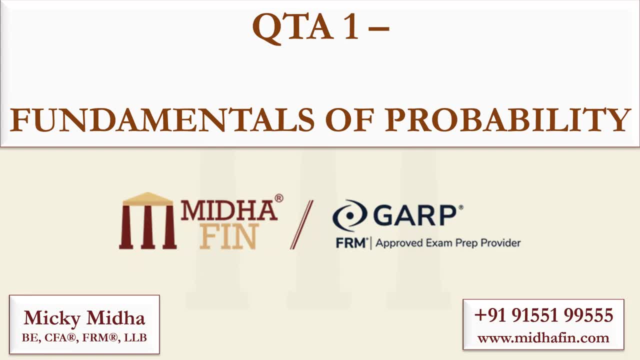 we'll actually adjust our focus accordingly. okay, and this, this shift, as i mentioned, it has been evident in past exams also, apart from the garb sample paper question, where a lot of theoretical understanding has been prioritized to some extent, then of course we've not, uh, we'll not be able to. 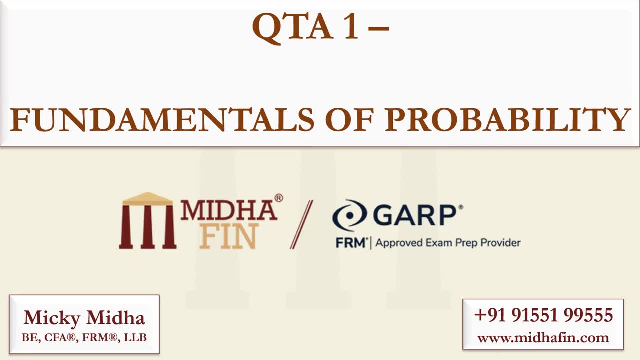 tackle numericals with long, detailed calculations due to time constraints, uh, but uh the again. as i said, there is a good news that the pdfs will be available. so if you are unclear about any solution, uh, even though we will not discuss detailed numericals, we'll discuss short numericals. 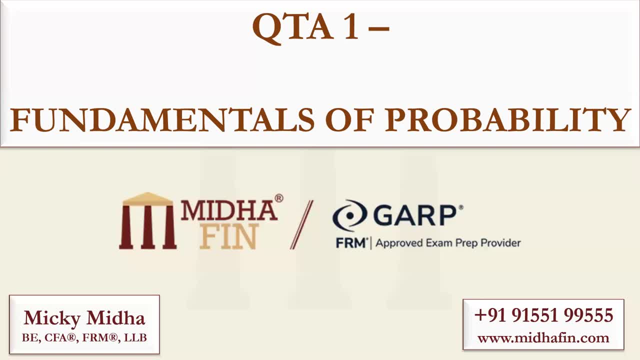 even then. uh, if you are unclear about any solution, you can always revisit the recording of our session and you can also refer to the detailed pdf slide. so recording will also be available of the class and detailed pdf slides will also be available. also, note that this is not a doubt. 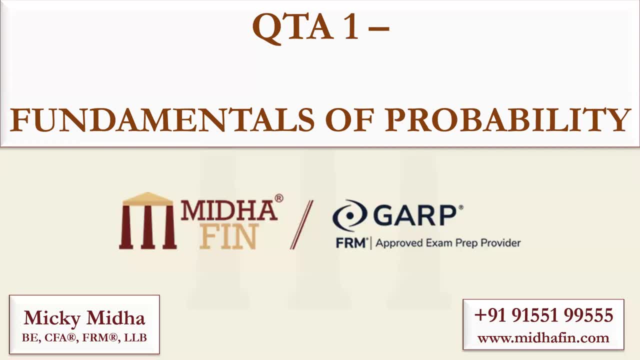 solving session. okay, this is not a doubt solving session, because for doubt solving sessions for the candidates who are enrolled with midafin we have a separate session. in fact, before the exam, we have multiple sessions dedicated to doubt solving, apart from the general doubt solving that we do throughout the year. 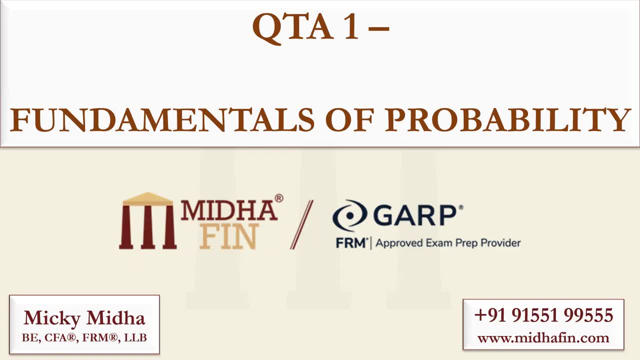 so we encourage you to save your doubts for those specialized sessions- this is especially to the midafin candidates- and let's start the course. i think it's a good opportunity for you to just solidify your knowledge and try to head into the exam with with a lot of confidence. 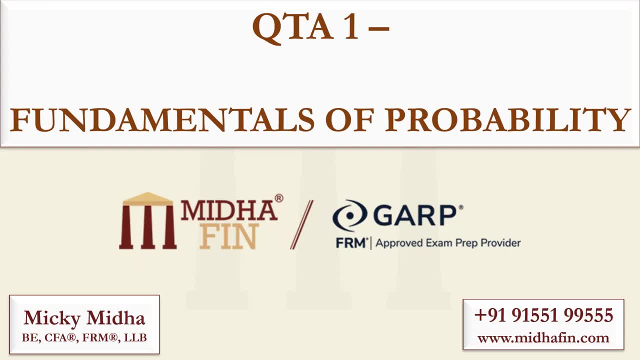 it is also possible that sometimes i might not be able to look at all the chats immediately, but i'll definitely have a look at it later on, whenever i i get time, and i'll answer to all of your, all your queries, later on. okay, so let's start. i look forward to try and help you. 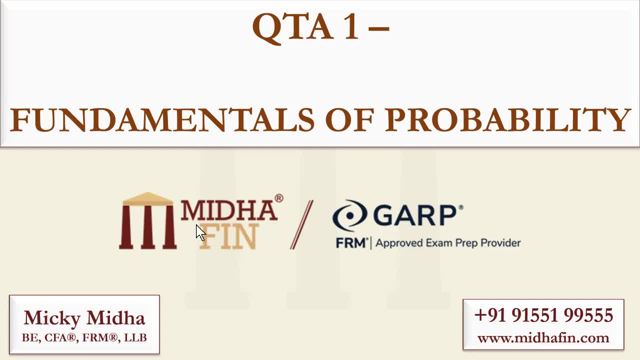 all to review and prepare efficiently. let's start with the first uh topic. today we'll try and cover four uh weeks. in fact, we have divided the course at uh, based on our study plan, into four blocks. out of those four blocks we are going to cover, you can say close to 0.7, 0.8 blocks. 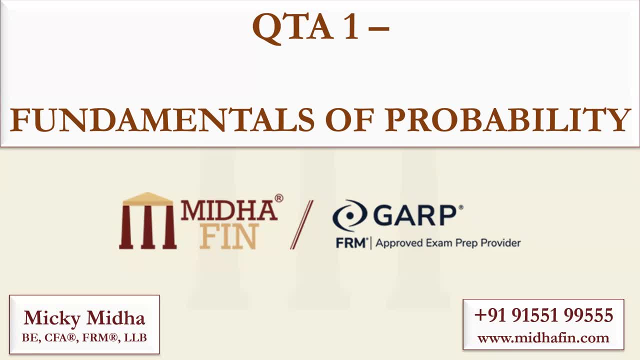 today. uh, if we are actually covering the first 12 topics of quantitative analysis, qta, today, starting from fundamentals of probability up to the times, these chapters okay and volatility chapters okay. so let me just have a quick look at all the chats till now. so, yes, yes, okay, uh. 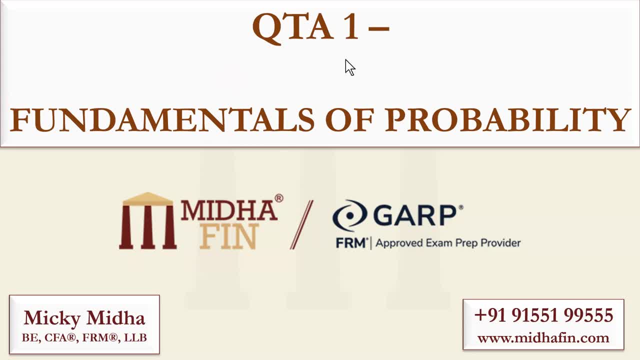 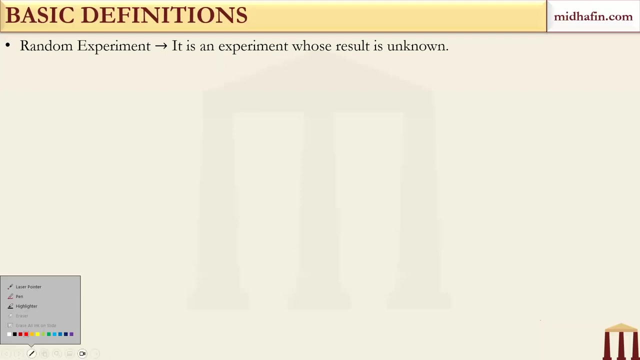 let's start with the fundamentals of probability. so random experiment: this is the maximum volume that we can have right now. is the volume? uh, okay, for everyone? okay, fine. so let's start with fundamentals of probability, some basic definitions. so random experiment is an experiment whose result is unknown. just give me one minute. 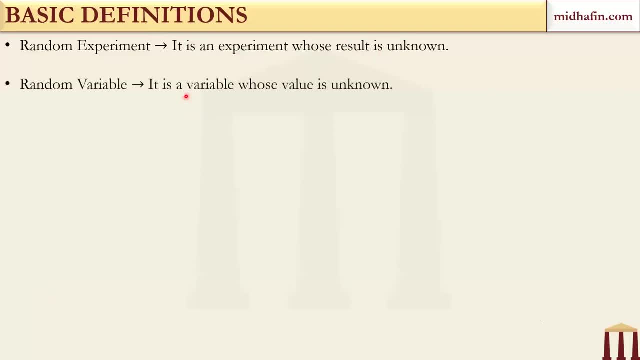 So it is an experiment whose result is unknown, then variable is a value. variable whose value is unknown, then outcome is the observed value for random variable. sample space is the set of all possible outcomes. event is the subset of the sample space, so that is one or several. 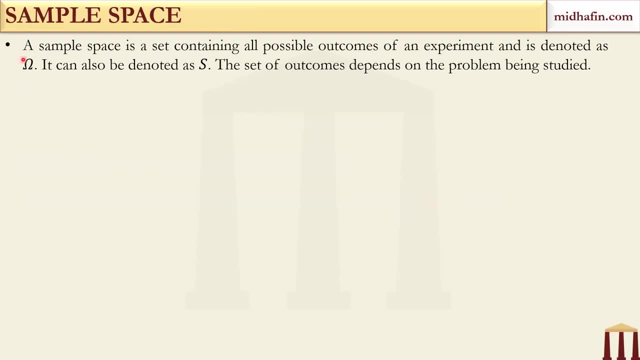 outcomes out of the sample space. that is an event. Now, what is the sample space? let us just explore a little bit. it is a set containing all possible outcomes of an experiment. it is denoted as either Ohm, capital, Ohm or capital. 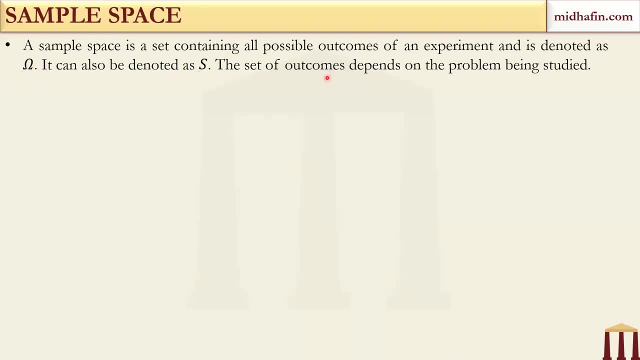 Sigma, sometimes people call it- or capital S, and of course the set of outcomes will depend on the problem being studied. So let us take some examples. so if we are studying the problem of returns on S&P 500, so we all know that the returns theoretically cannot be less than negative 100 percent. 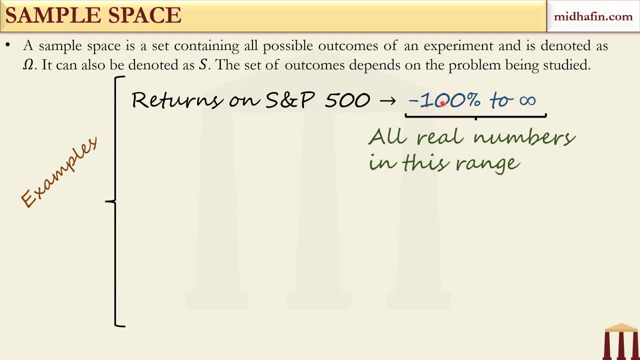 so if you lose all your money, then the return is negative 100 percent. it cannot be less than that and there is no theoretical positive bound to the returns. again, I am saying theoretical, So the sample space is all real numbers in this range: negative 100 percent to infinity. 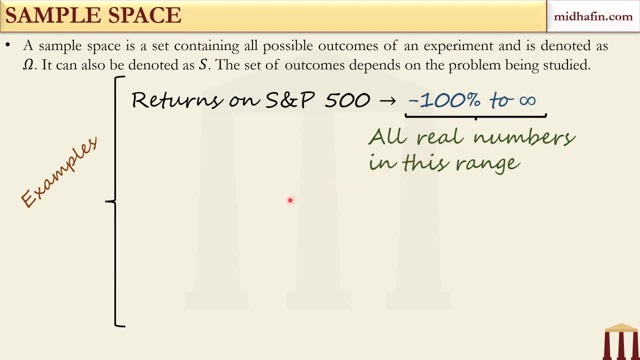 Now, if you are interested in the direction of returns instead of the actual returns direction of returns, either it can be positive or it can be negative, or maybe no movement at all. so these are the three possible outcomes. Then, if you are studying bond B, 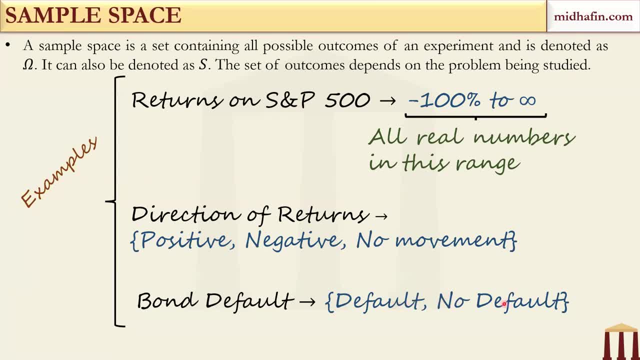 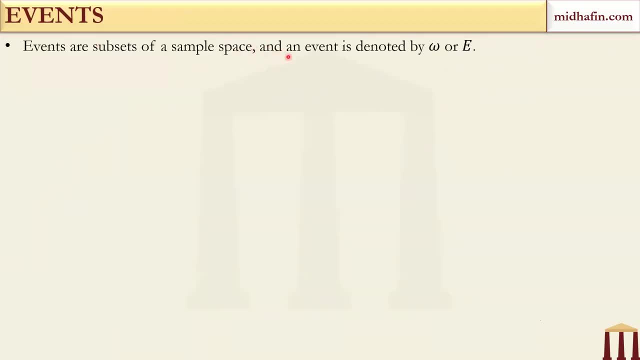 defaults. So either the bond will default or the bond will not default. So these are some examples. Now events: Events are subsets of sample space and any event is denoted by omega or capital E. So, for example, if you are rolling a six-sided die, this is your sample space 1,, 2,. 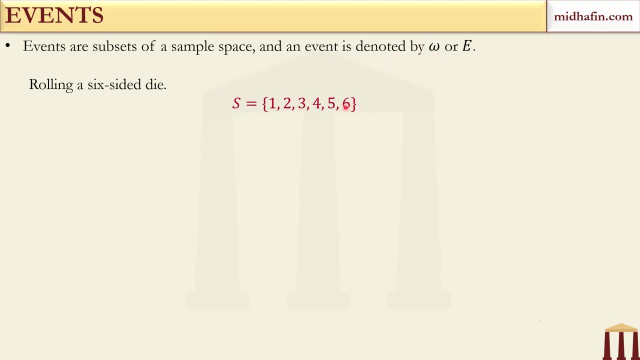 3,, 4,, 5,, 6.. And if you want to find out what are the outcomes or what is the event of getting an even number. So if, let's say, we denote E as the event of getting an even number, then E contains: 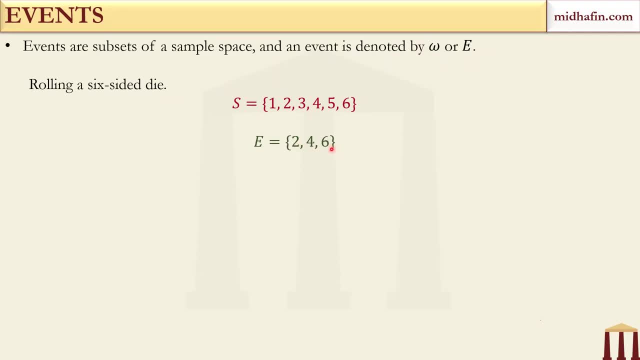 these three elements 2,, 4, and 6.. And as I mentioned that events are subsets of sample space, right? So mathematically we'll write it like this: E is a subset of S. It means all elements 2,, 4,, 6 are already present inside the bigger set S. Now an event with a single outcome is known as. 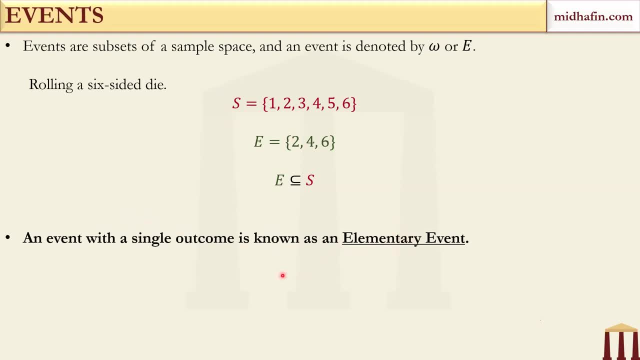 an elementary event. So, for example, if suppose you have an outcome in this experiment, only if I say that, what is the event of getting a number less than 2?? So obviously only one outcome will be there: 1.. So this is an elementary event. Then any event with no outcome is known as a null event. 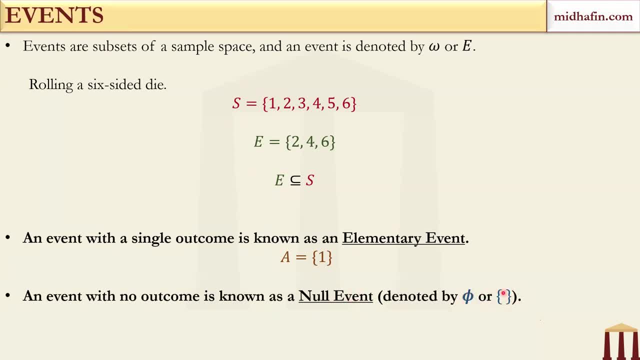 It is denoted by phi, or this null set, the empty set. So this is an example: G is equal to this empty set And, of course, for, for null sets, the probability will be equal to zero. So for null events, a definite probability. 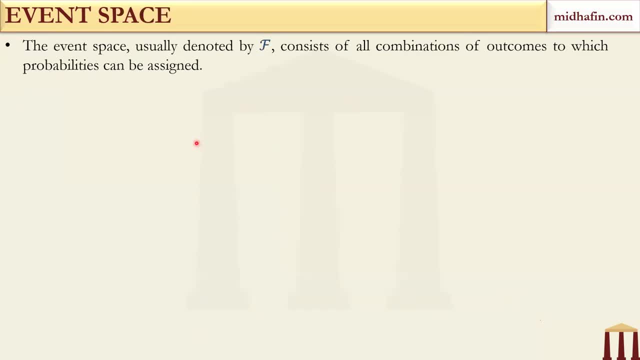 of zero can be assigned. Now let's move to another concept: event space. Now this is a concept which I have seen that it is not very well understood by many candidates, So they tend to skip it. So obviously we'll we'll not be able to go into details as we have done in the class. 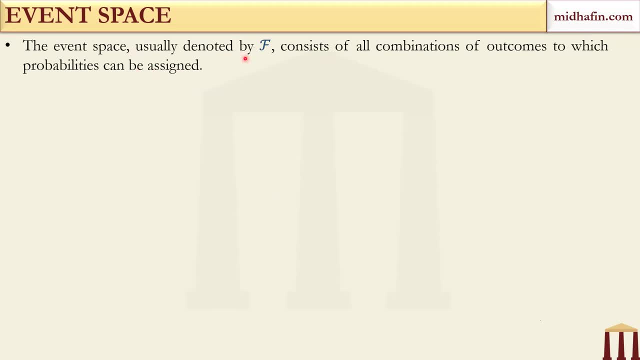 but I'll try my best to explain it quickly. So event space is denoted by this symbol. F consists of all the elements of the event space. So there are, there are thousands of elements of all combinations of outcomes to which probabilities can be assigned. So, for example, if suppose 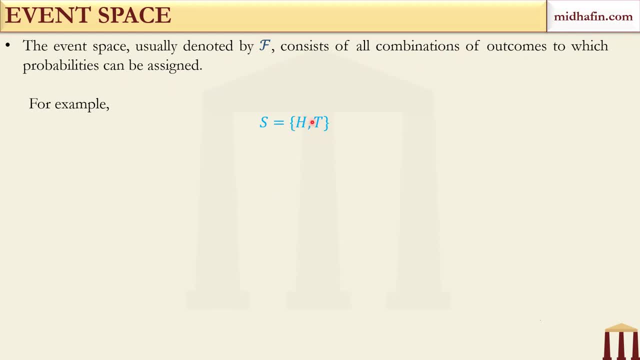 this is the sample space. the experiment is rolling of a coin, So two outcomes are possible, heads and tails. So when I say event space, so event space is basically combinations of outcomes to which probabilities can be assigned. So in simple terms you can say: 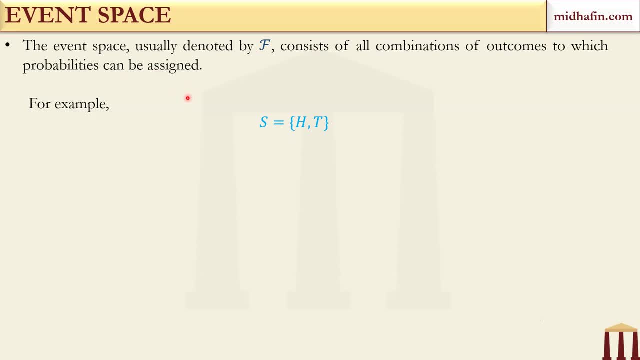 that it is the set containing all possible subsets actually. So, if you see how many subsets of this set are possible, actually four. So these are the four subsets: One is H, one is T, one is H comma T and one is phi. Now it is interesting to note that this phi is a subset. 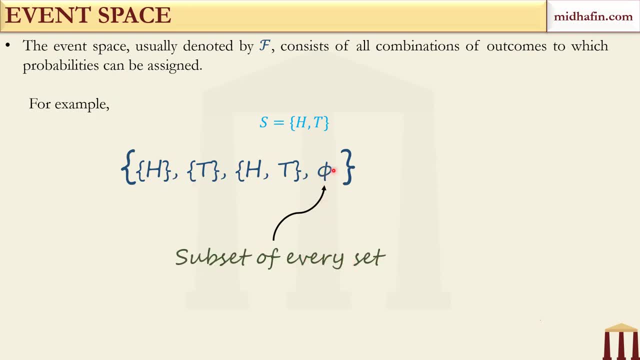 of every single set. Remember that So phi, or the null set, is a subset of every single set. Now, when you consider the subset of every single set, it is a subset of every single set. So phi is a subset of every single set. Remember that So phi, or the null set, is a subset of every single set. Now, when 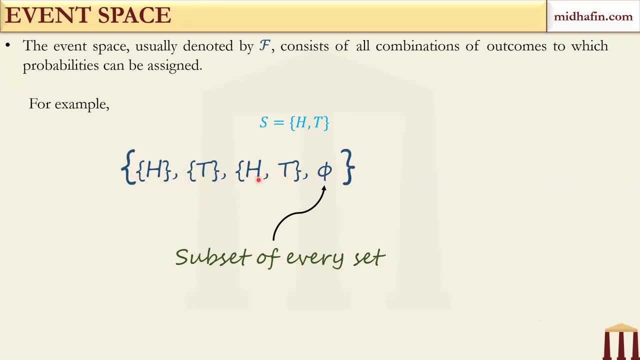 you combine all these four subsets into a single set, you actually get an event space. So that is the meaning of event space. It is the set of all subsets. Okay, Now one thing also: you can just note over here that in the event space even impossible events or null events are also 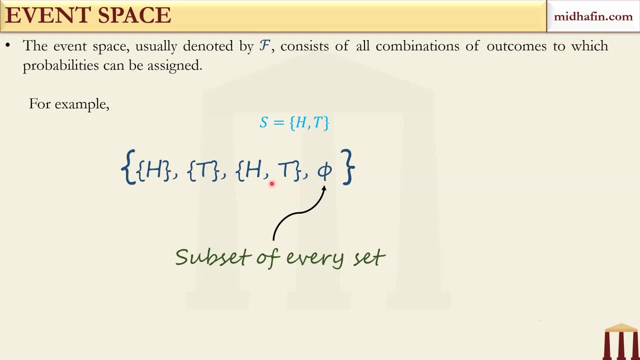 considered, For example, when you throw a coin, it is not possible to get both heads and tails at the same time. So if you consider the subset of every single set, it is a subset of every single set. So, if you consider the subset of every single set, it is a subset of every single set. So the 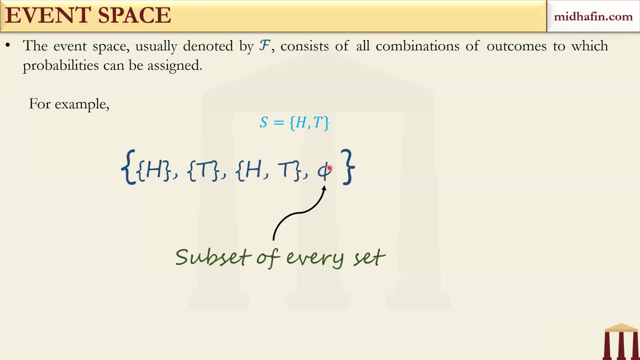 probability of this event is actually zero. right, Even the probability of phi is zero. So event space: there is no bound that only positive probability events have to be there. No Zero probability subsets: the events which are having zero probability will also be there in the 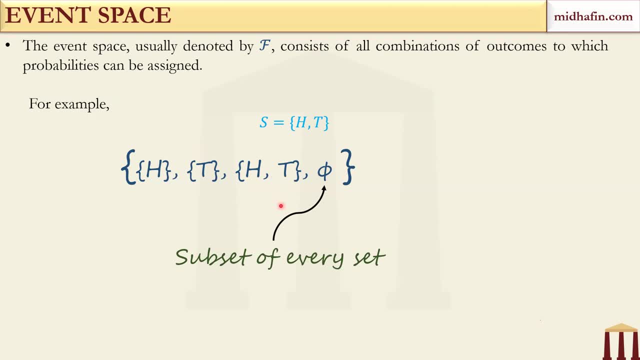 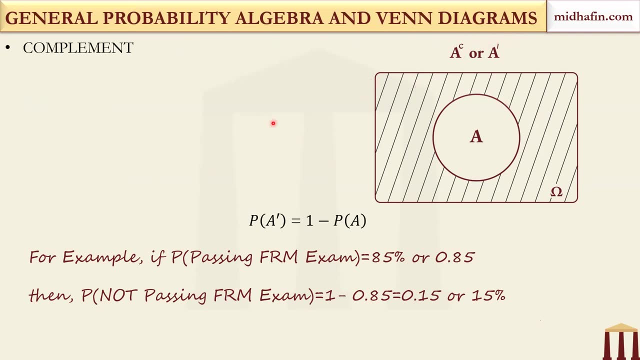 event space. That is one of the features of event space. Now let us go to general probability, algebra and Venn diagrams. So what is a complement? Complement is also known as not Okay. So this is the symbol for complement, and sometimes it is also written as: 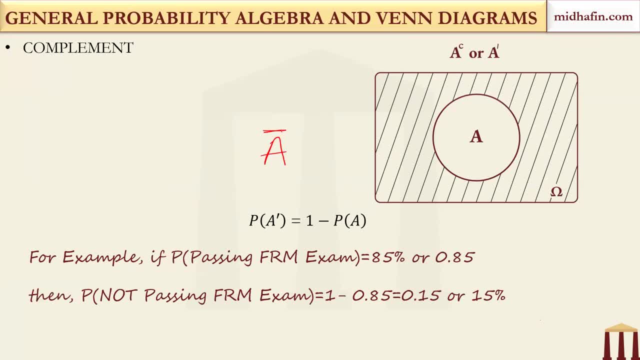 a complement like this. Okay, So, based on the Venn diagram, it is quite clear that anything which is not in A or outside of A, which is in the shaded region, which is in the sample space but not in A, it is nothing but the A complement. So what is the algebra over here? Probability of A complement. 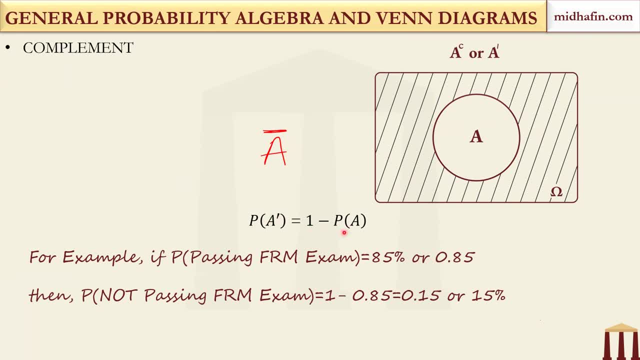 is equal to 1 minus probability of A. So, for example, if probability of passing the FRM exam is 85% or 0.85,, then probability of not passing the FRM exam is 1 minus 0.85,, which is 15% or 0.15. 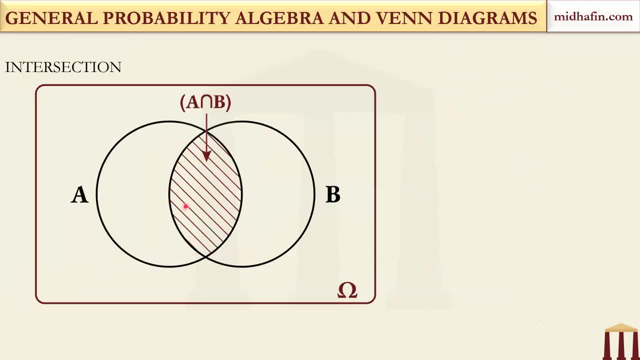 Now let us come to intersection. So what is intersection? Intersection is basically that event A intersection B, which contains the event A, intersection B, which contains the event B, intersection B which contains both A and B. So A and B, both are there, Okay. So let us take an example. If suppose A. 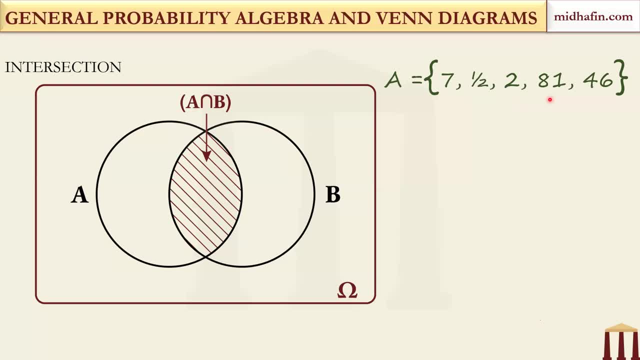 is this set: 7, half, 2,, 81 and 46. And we have B as 8, 4, 1 by 2, again half 74 and 7.. So if you want to find out A and B or A intersection B, then you simply have to check which elements are common. 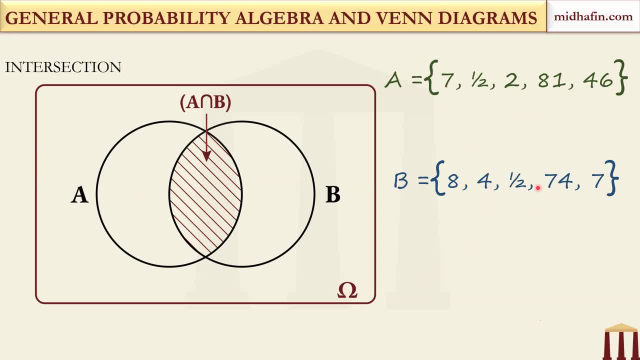 to both A and B. So if you want to find out A and B or A intersection B, then you simply have to check which elements are common to both A and B As well as B. So which two elements are common. one is half, the other one is seven, because it is. 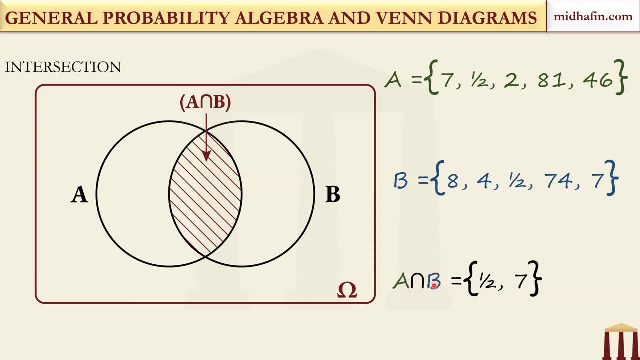 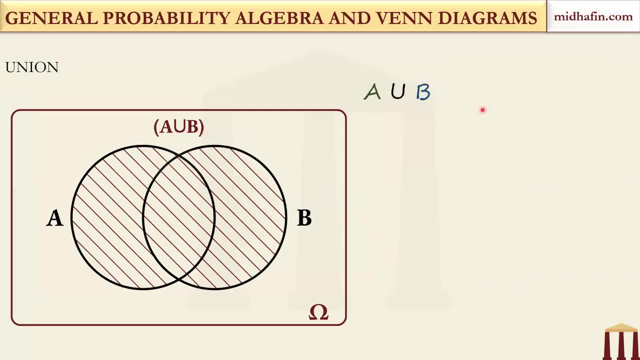 present in both the sets. So this will be my A intersection B. Now let us come to union. So union A, union B, and which is sometimes referred to as A or B. Okay, Now, even though we mentioned it as A or B, but it actually implies A or B or both. Okay, Because 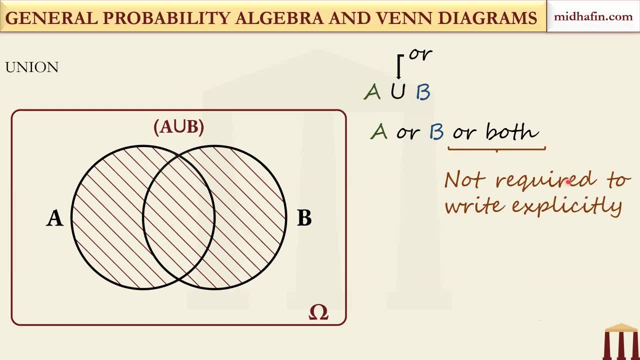 Now, although this or both is not required to write explicitly, but it is implied that even we are talking about the middle region, we are not talking about A exclusively. So that is why, even if I say A or B, it is actually sufficient to explain that the middle 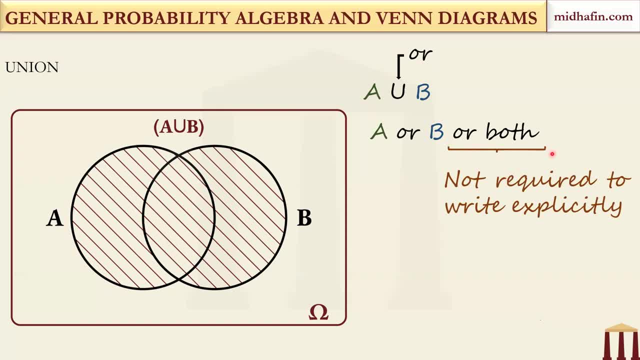 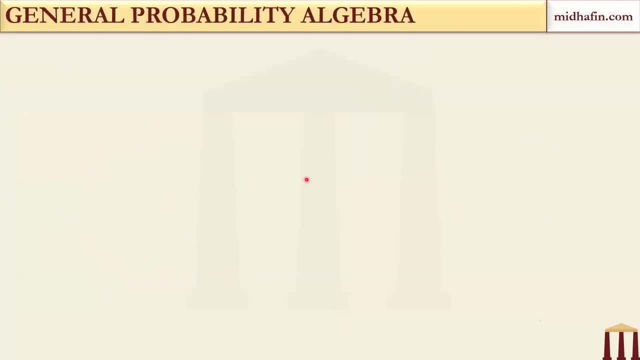 region is also being included. But just to make it more clear, it is imperative it is actually better to write A or both Now. in general, the probability of A union B is equal to probability of A plus probability of B minus. probability of A intersection B. This is our first algebraic equation of prime. 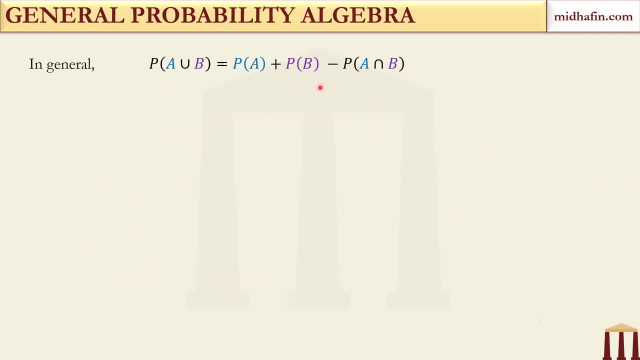 importance in probability, which has been tested many times in the Excel. So again, the logic behind this equation should be quite clear, because if there are two sets, A and B, and if you are adding them, you can clearly see that the middle region, which 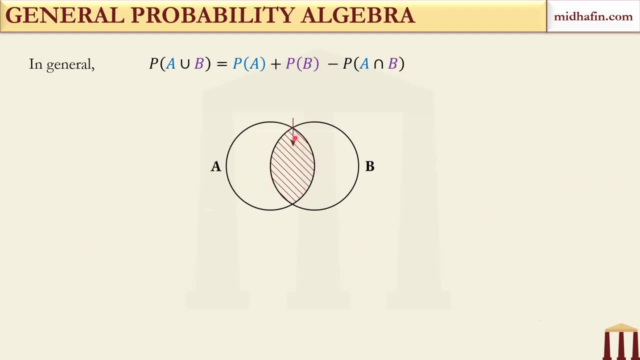 is common to both A and B is actually being counted twice. okay, So to give a proper adjustment, you have to subtract it once. So then you will get the full A union B. okay, Now, what are mutually exclusive events? Mutually exclusive events are events which cannot happen together. 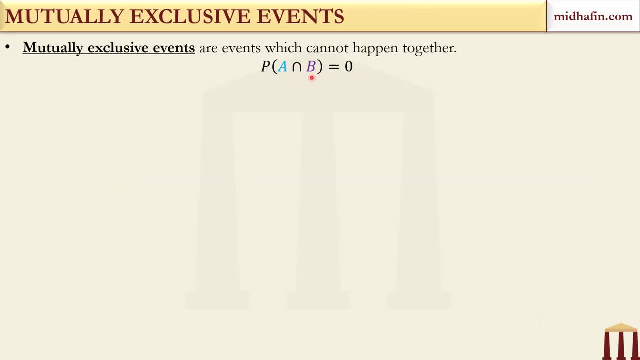 So for mutually exclusive events, the probability of A intersection B is equal to zero. Okay, So this is how we can denote mutually exclusive events using the Venn diagram formula. So A and B, nothing is common between them. That is why A intersection B is the null set. 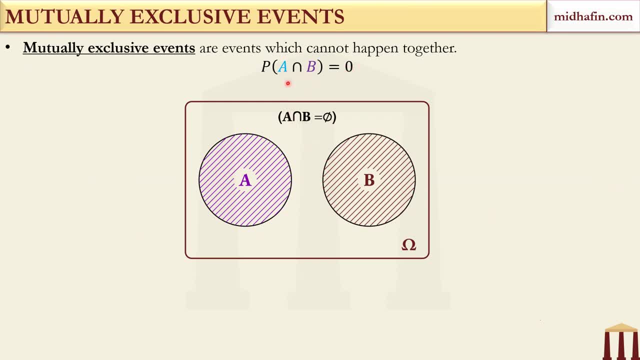 And so probability of A intersection B is zero. See, I have not written A. probability of A intersection B is equal to phi. no, Make a very clear distinction between sets and probability. So, when we are talking about sets, A intersection B, unless and until I have not written probability, 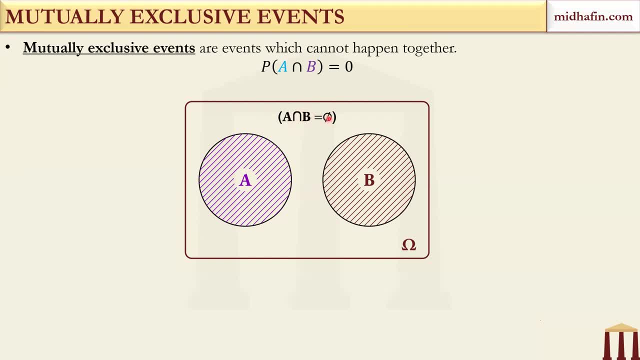 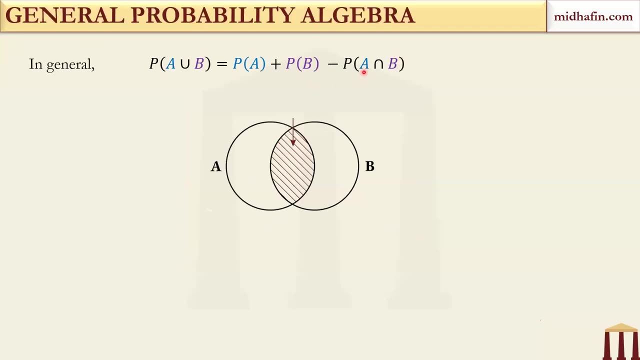 okay, we are talking about events, So this is a null event. Nothing is common. But when I say what is the probability of this null event, obviously it is equal to zero. So when you apply this P A intersection B to the general probability algebra over here, 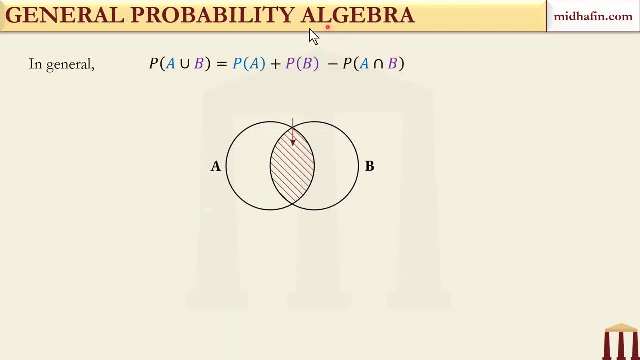 so this term becomes zero? okay, I hope my laser pointer is visible to everyone. The laser pointer is visible to everyone, right? I am highlighting A, intersection B. Okay, So if this term becomes zero, what will happen? What will happen? 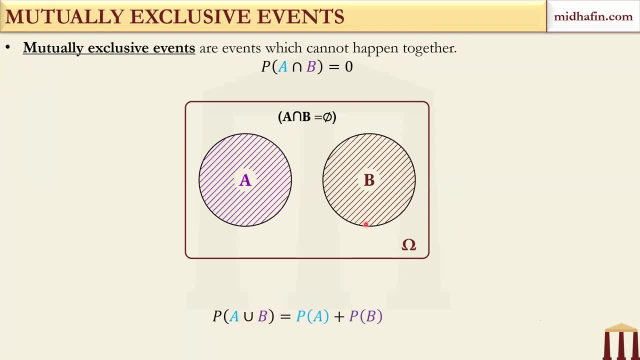 The probability of A union B in this particular case will become P A plus P B, And in our self-paced course, in our main videos, we have actually done a very beautiful derivation of this using some very practical examples. okay, so that these things are actually matching. 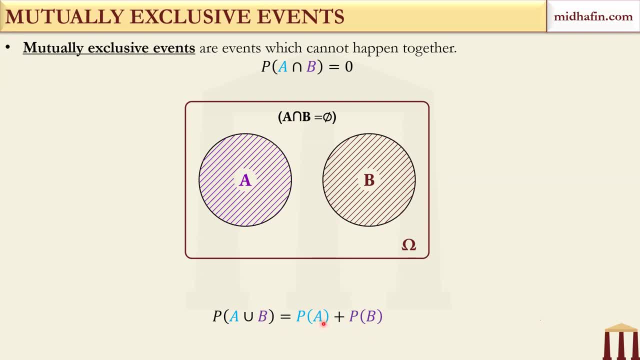 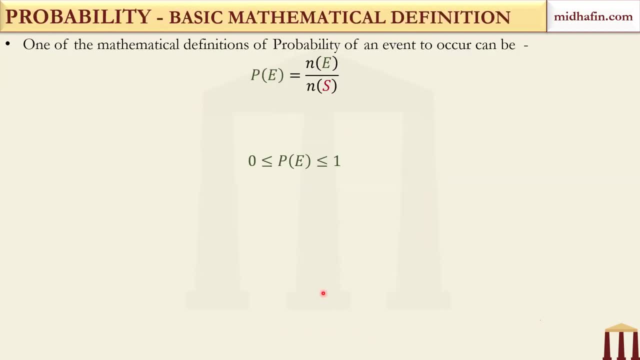 with our initial ideas. But anyways, as I said, this is a crash course, so detailed derivations can't be there, but at least for basic understanding purpose I think this is sufficient. Now we all know that one of the mathematical definition of probability of an event to occur 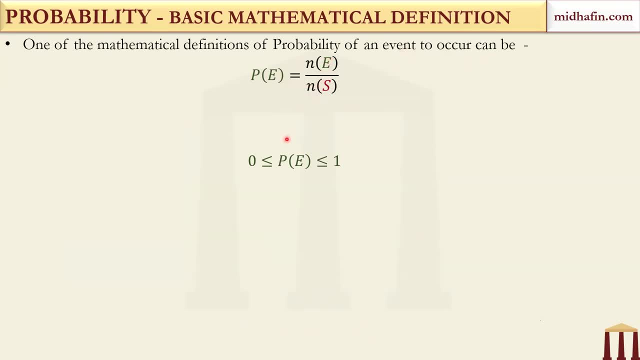 can be. P? E is equal to N? E over N S, So N? E is the number of favorable outcomes for event E and N? S is basically the number of outcomes in the sample space or total number of possible outcomes. That's it, Okay. 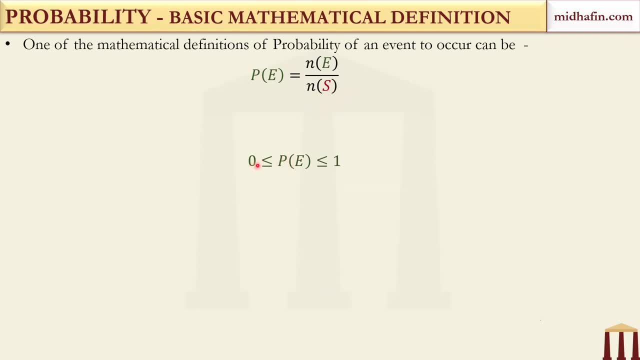 That's it Now. mathematically, this assigns a number between zero and one to each event, E, And it is very important to note that this probability that we are talking about is actually the unconditional probability. So over here till now, we are referring to unconditional probability. 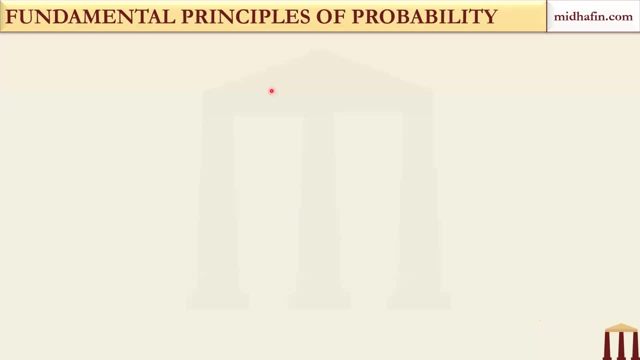 Remember that. Now let's come to three fundamental principles according to the GARP curriculum, although this is something in which different Authors have a different viewpoints and different literature has listed these principles in a different manner, But based on the GARP curriculum, you have this fundamental principle: the probability. 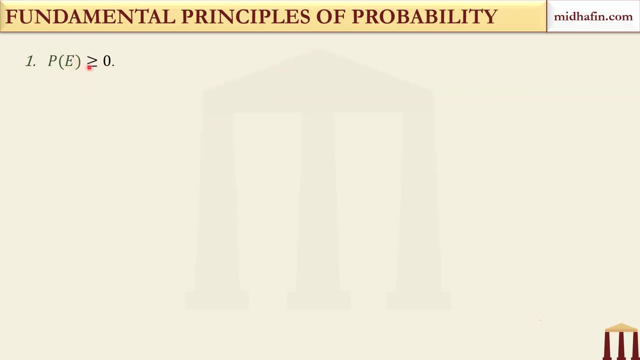 of any event cannot be negative. Of course, it has to be greater than equal to zero, And we have all seen in the previous case that it has to be less than one. also, And the probability of sample space is equal to one, Also for any number of N mutually exclusive events. probability of A1 union. A2 union. 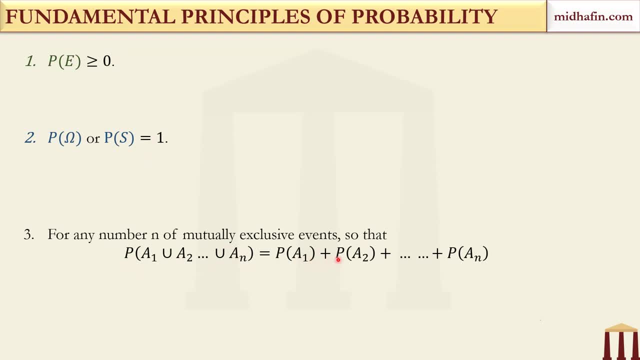 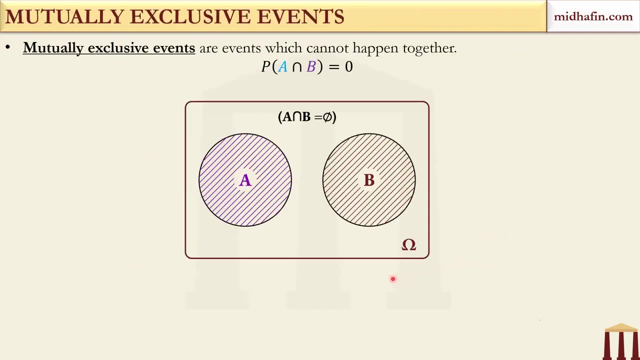 up to AN is equal to PA1 plus PA2 plus up to PAN. okay, So we saw this for two events Over here. for two events. we've already seen this: PA union B is equal to PA plus B. So the third principle states that you can extend this idea to N number of mutually exclusive. 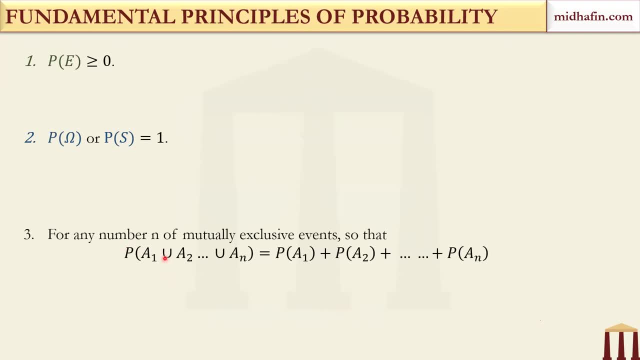 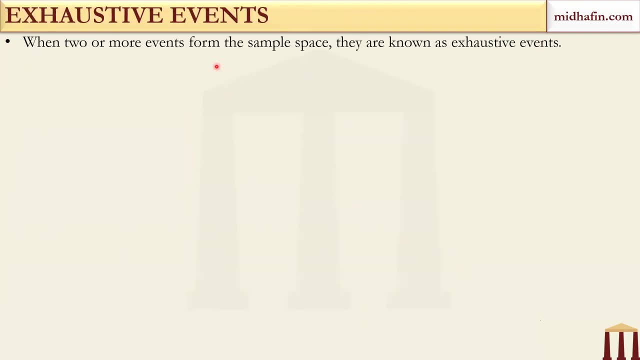 events, So that you are getting PA1 union, A2, union, AN up to PA1 plus PA2 plus up to PA. Now what are exhaustive events? When two or more events form the sample space, they are known as exhaustive events, So the word itself exhaust is actually quite clear to explain what are exhaustive events. 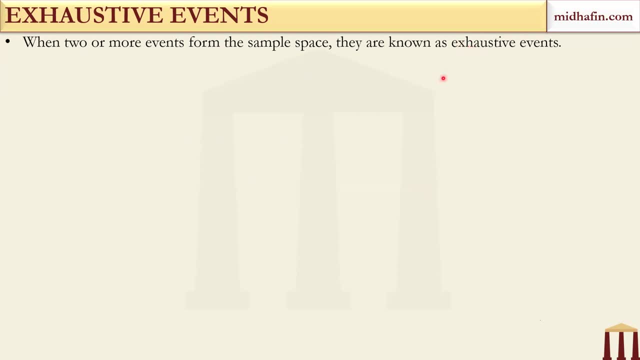 So exhaustive events. basically they exhaust the sample space altogether. So let's take an example. So if suppose this is The data set for six sets over here, six or seven sets, A, B, C, D, E, F, N, G, 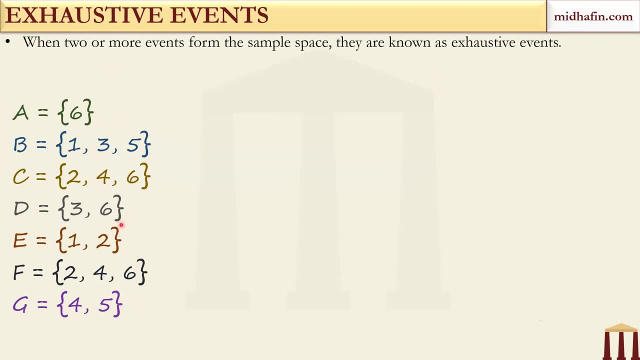 Now, if I have to check which of these are exhaustive events. So one thing I'll also do: apart from the exhaustive check, I also perform a mutually exclusive check. I'll tell you why: because there is a special class of events which we discuss in probability. 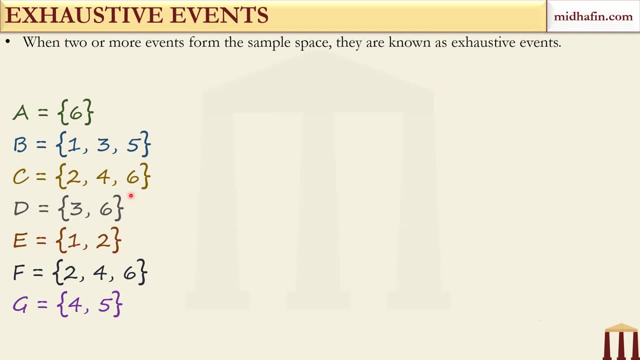 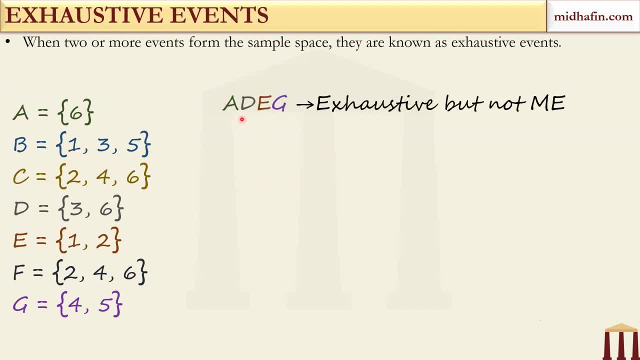 Okay, So if you combine these events, let's combine randomly. some events Say we combine A, D, E and G. So if you combine A, D, E and G, they are exhaustive. Why? Because you can see, if you combine, six is there. 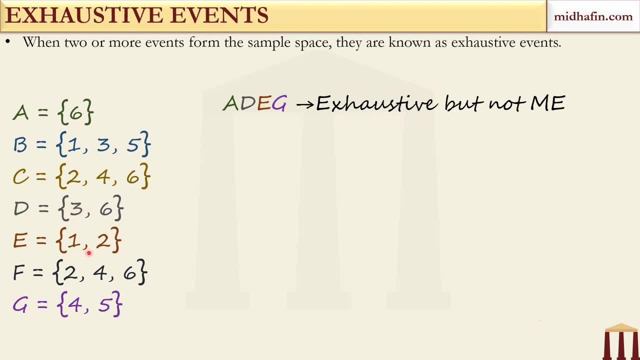 Okay, Three is there. Okay, One is there. Two is there, Four is there. Five is So? one? two, three, four, five, six is there? All the and the experiment being considered okay is actually the role of a single six-sided die. 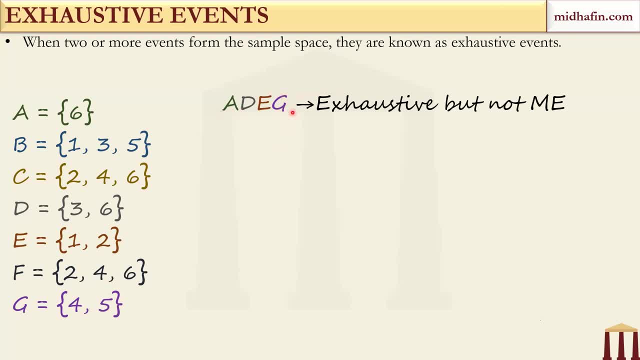 So all the possible outcomes are included if you consider A, D, E and G together, But they are not mutually exclusive. But they are not mutually exclusive Why? Because six is common in A and D, Although mutually exclusive events make sense for two events only. 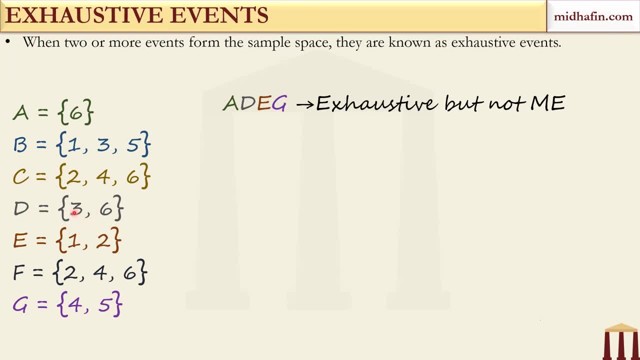 we take them in pairs. But just to make things simple, I'm just assuming that even if one of the pairs is having a common event, we'll assume that this. we'll say that, okay, these are not mutually exclusive events. Then let's consider only A and E. 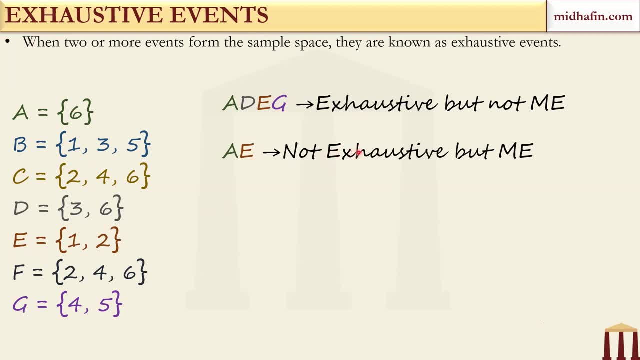 A and E. So A and E, they are not exhaustive, but they are mutually exclusive. Because if you combine A and E, do you get the entire sample space? No, You do not get many numbers, You only get one, two and six. 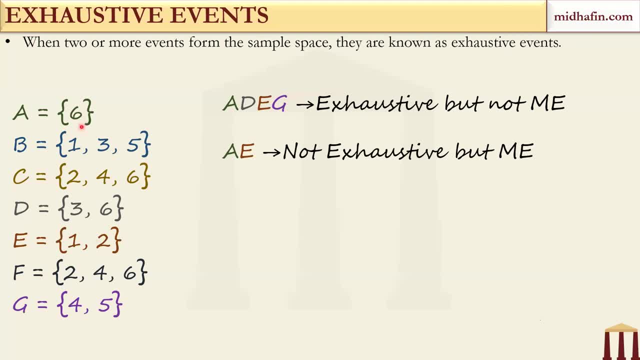 But they are mutually exclusive because there's nothing common between them. Now let's consider a very special case of events, which is B- C. These are exhaustive as well as mutually exclusive, And together we call them as mutually exclusive and exhaustive events. 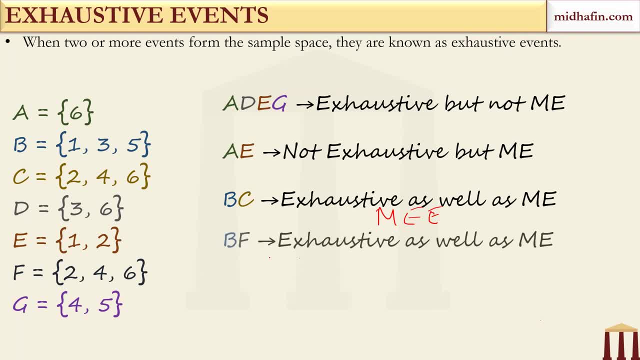 M E E events. Okay, Now let's consider B F. B F is also M E E- exhaustive, as well as mutually exclusive, Because there's nothing common between the exhaustive and mutually exclusive events. So let's consider B and F. 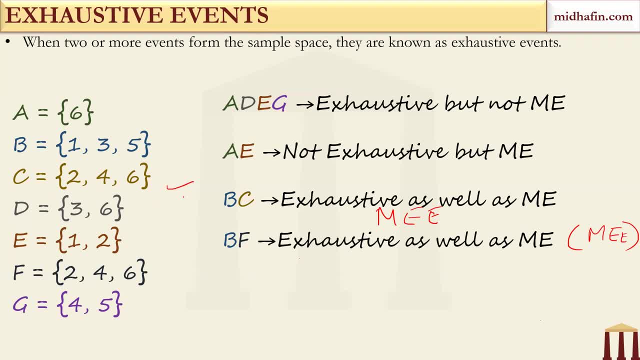 Okay, Because, see, you might say that C and F are same sets. Yes, in terms of the outcomes they are definitely the same sets, But maybe we have defined them in a way that, coincidentally, the outcomes are the same, So maybe C we have defined directly. 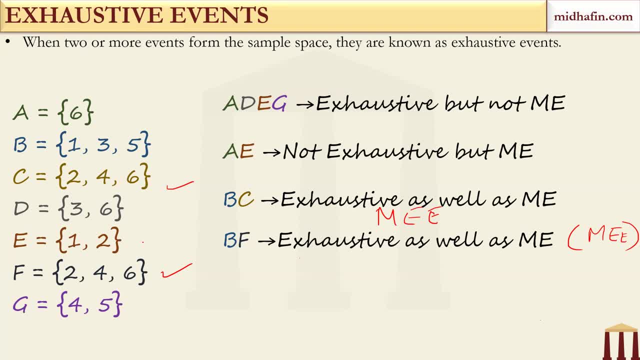 as the event of getting an even number, And F we define as say, the event of getting a number more than one but less than three, and greater than three but less than four, something like that. Okay, So we can definitely have our literal definitions. 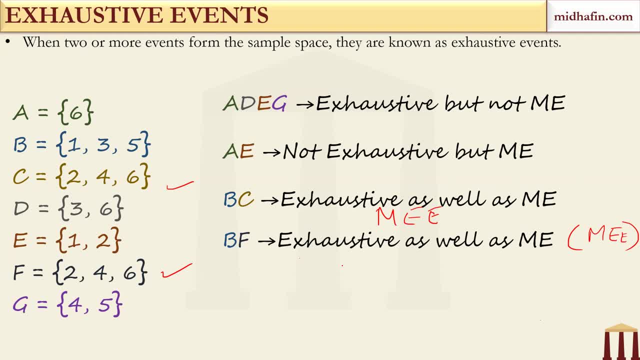 But finally, the sets are identical. So B, C, B and F, they're exhaustive as well as mutually exclusive. E, A and G: they are not exhaustive, but they are mutually exclusive. Okay, So this M, E, E, this class of events. 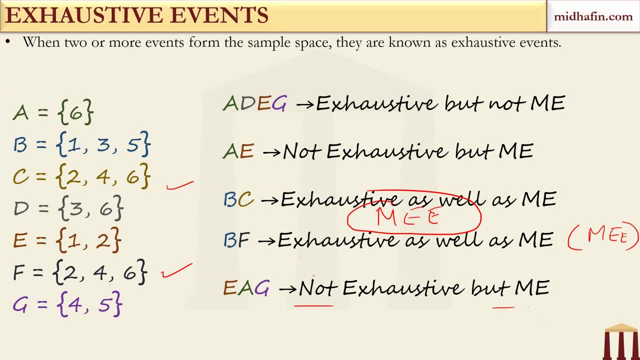 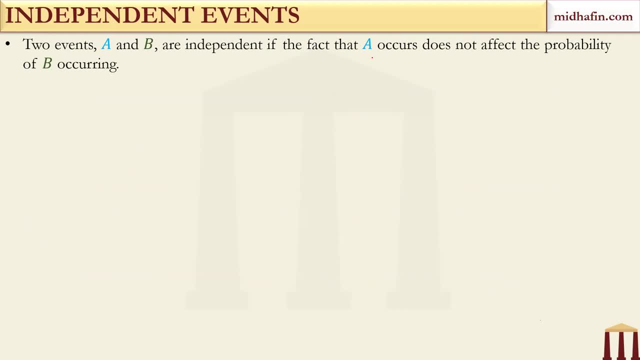 are very, very important in probability theory. Okay, So we discuss why later on. Now, what are independent events? Two events are independent if the probability of occurrence of A does not affect the probability of occurrence of B. Okay, So PA intersection B is equal to PA times PB. 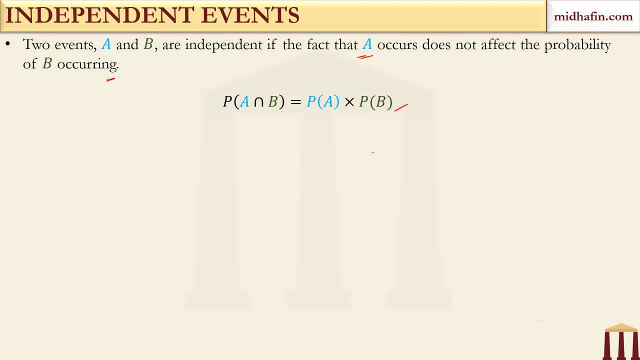 This is the algebra for independent events. If the two events are independent, then the probability of their intersection is similar to the probability of their intersection B. So this is simply the multiplication of the two individual, unconditional probabilities. Now I'll just pause over here. 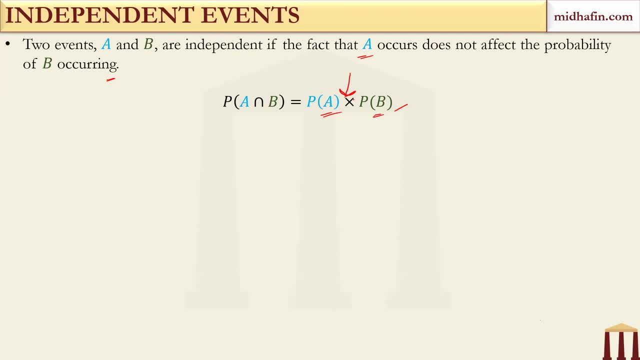 Okay, And although I mentioned that we'll not be able to have a discussion kind of class, a lot of discussions will not be there, but some minor discussions. we can have some small discussions, because this doubt is asked many times. Are you all clear with the idea? 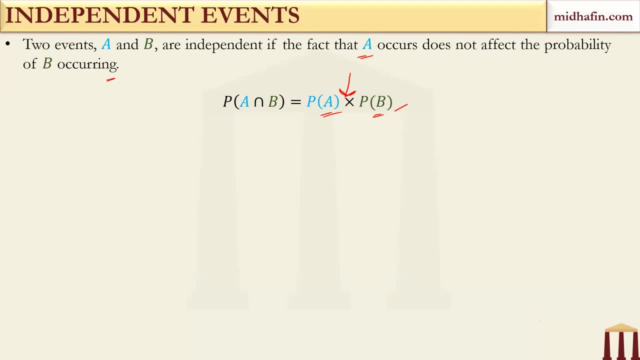 of the difference between mutually exclusive and independent events. Have you ever thought that? what is, what can be, the relationship between the mutually exclusive and independent events? anyone? Mutually exclusive and independent events Are they same or is there any relationship between them? 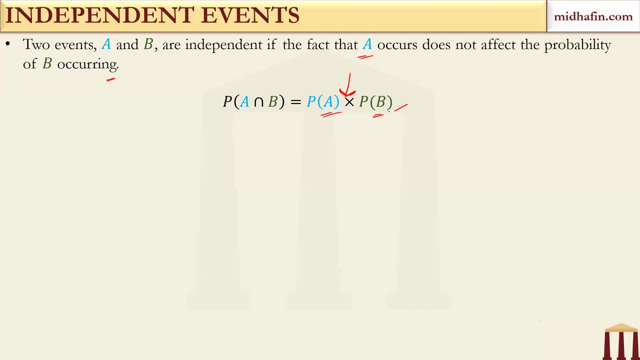 Anyone who'd like to answer. They're not the same. They're not the same. So any relationship between them, Not a direct relationship but any implied relationship, Can you say Between independent events and mutually exclusive. Can I say that mutually exclusive events? 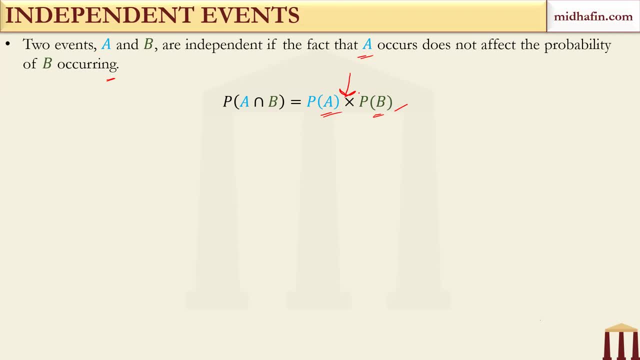 listen to my statement very carefully. mutually exclusive events can never be independent. If I say this is the implied relationship. if the events are mutually exclusive, then they can never be independent. Is this correct? Yes, absolutely correct, Because see, mutually exclusive events means what? 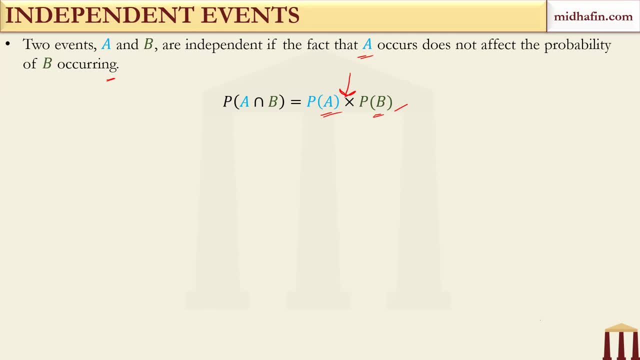 That if one is occurring, the other cannot happen. That is mutually exclusive. Nothing is common between them, So either of them can happen, Happen. either It will rain today or it will not rain today. Either the candidate will pass the exam or the candidate will not pass the exam. 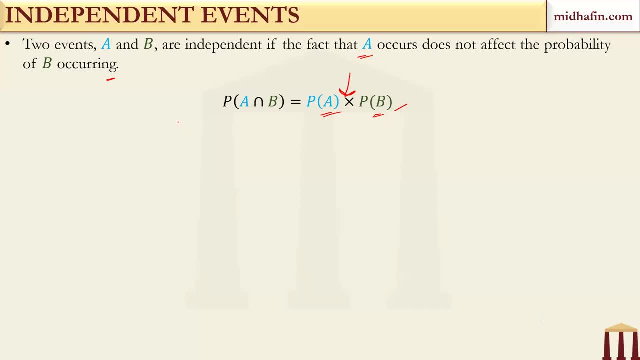 Okay, So mutually exclusive events. If you see, by definition there is an element of dependency between them. They are actually dependent on each other. So this is the implied relationship, that mutually exclusive events. they can never be independent of each other. They are always dependent on each other because if one happens, 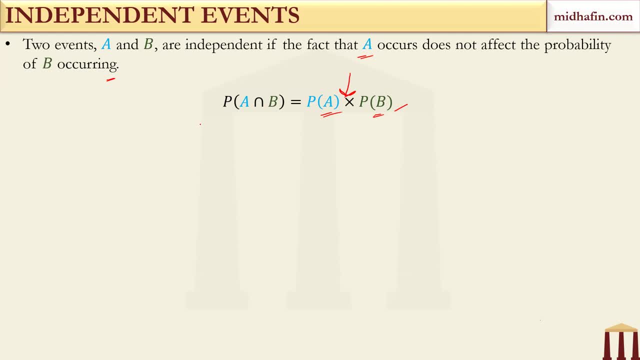 the other cannot happen. Okay, So this is an indirect observation, indirect interpretation regarding the relationship between independent and mutually exclusive events. Now, if suppose you apply this to the general probability algebra, then if you apply this to the general probability algebra, 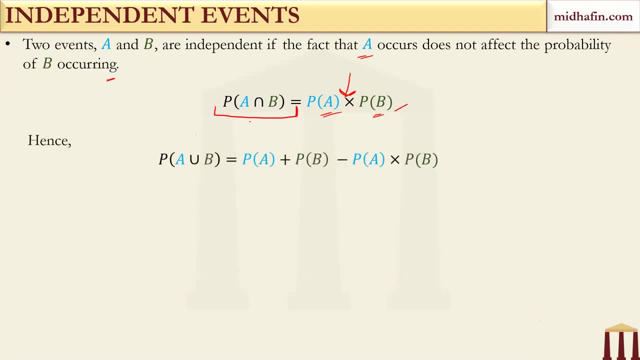 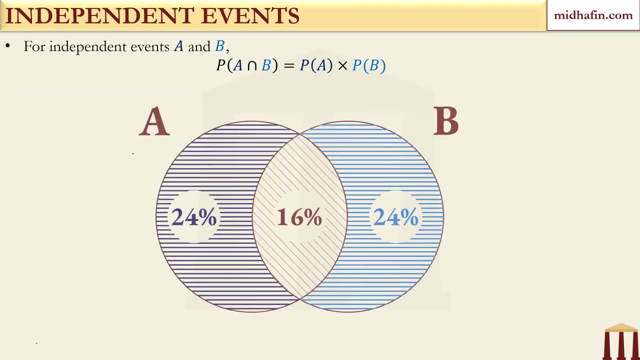 then your general probability algebra becomes: P A union B is equal to P A plus P B, minus P A times P B. Okay, Now how to try and visualize independent. So let's say we have this Venn diagram over here and the probabilities are demarcated based on regions. 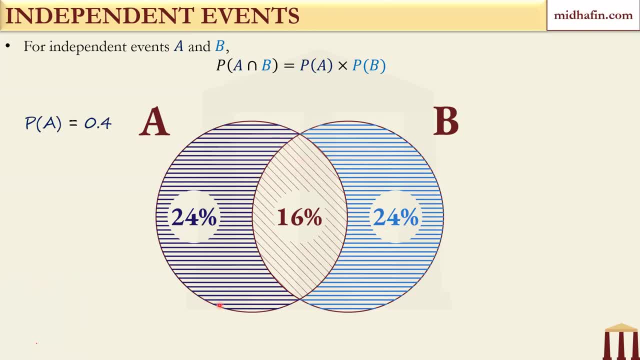 So what I mean to say is, if you want to calculate the total probability of A, this 24% is exclusively for this region. Remember that. Okay, So this is how the other Venn diagrams will also be done when we'll try to visualize conditional probability. 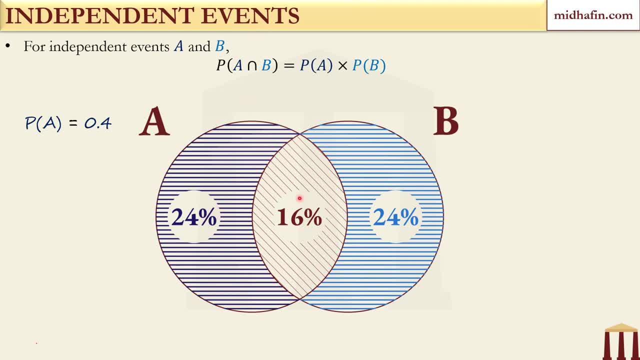 So if suppose you have 24% over here, 16% over here, so this is 0.4, 24 plus 16,. 40% is P A. P B is how much. P B is also 40%. 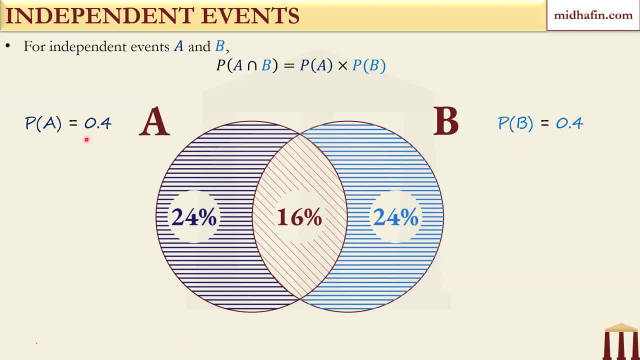 So can you just say, by looking at this Venn diagram, let's say: nothing else is given to you in the exam, Only this is given to you in the exam. Can you say that these events are independent or not? Anyone, Are these events independent? 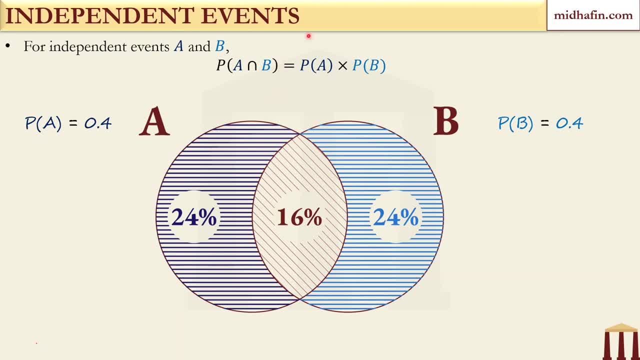 What do you think? Yup, Yes, they are, because P A intersection B is actually 16%, So P A intersection B is 0.16.. It is clearly given, which is same as P A times P B, also because P A is 0.4,. 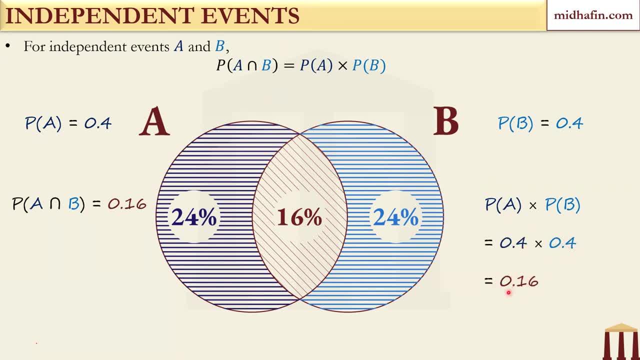 P B is 0.4.. So P A times P B is 0.16, which is same as P A intersection B. So if this kind of a Venn diagram is given in the exam, you can just calculate and multiply the individual probabilities and check if the intersection is common. 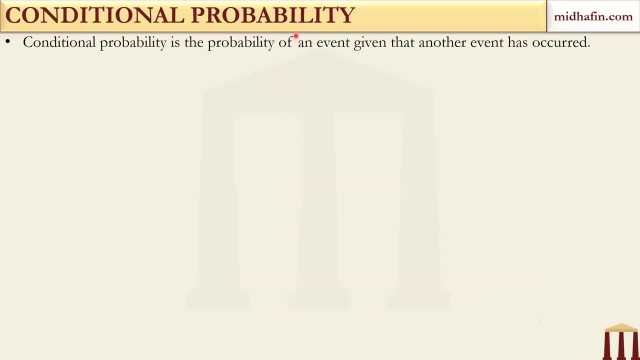 Now let's come to conditional probability. Conditional probability is the probability of any event given given that another event has occurred. So this is how it is denoted: P A given B. So this sign, this bar over here, is actually given. 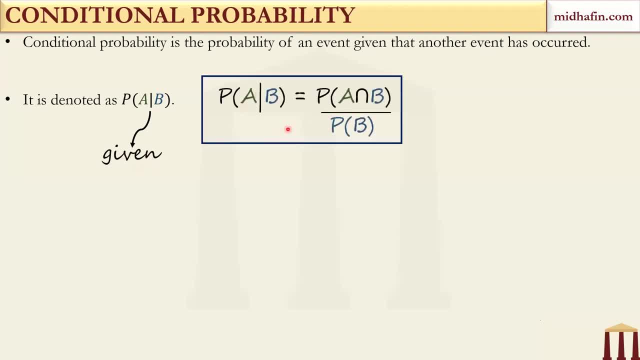 Okay, This is how it is stated And this is the general algebra for conditional probability. Again, we cannot derive this today in the crash course. P A given B is equal to P A intersection B divided by P B. So if two events are independent, 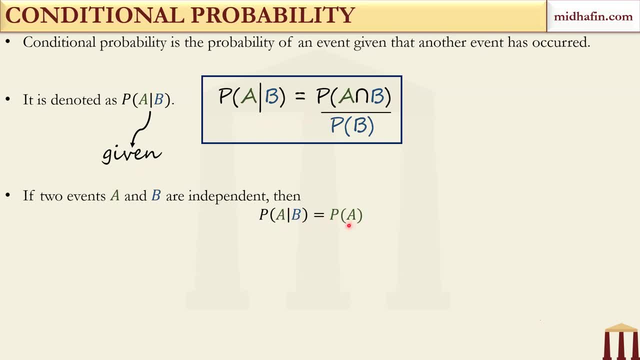 then P A given B is equal to P. Again, all these statements we have actually derived in the class So, but from the exam point of view it is important to remember that if two events are independent, then their conditional probability and unconditional probability are same. 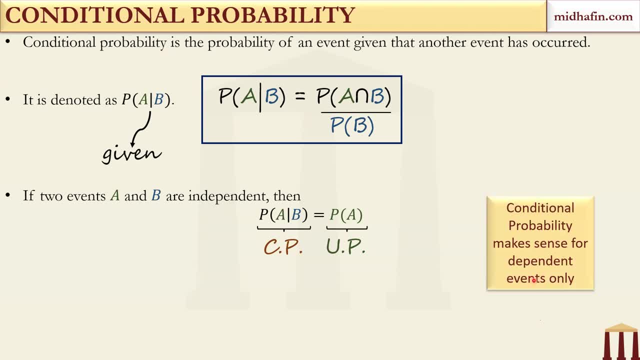 So conditional probability makes sense for dependent events only. This is a very, very important point: Conditional probability, it makes sense for dependent events only. This is where I've seen a lot of people making mistakes. Even some experts make mistakes, You know. 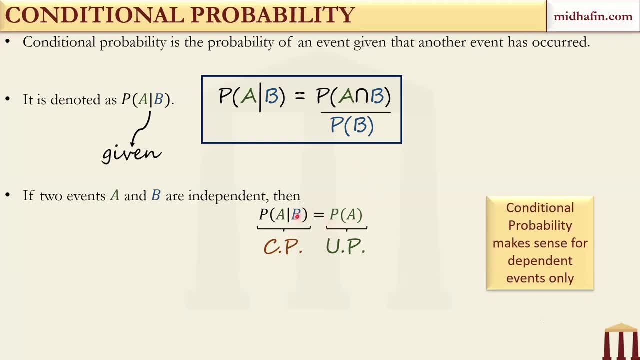 when they try to identify two events and they say that, okay, this is the dependent event, This is the independent event. No, Whenever P A given B is written, it means both of them are dependent on each other. unless and until this equation is holding true, 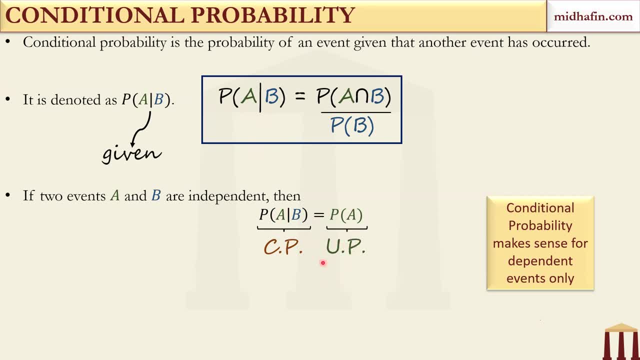 Okay, Also, tell me, if A and B are mutually exclusive events, what do you think the conditional probability will be P A given B according to you? If suppose A and B are mutually exclusive events, then very good, P A given B will be how much? 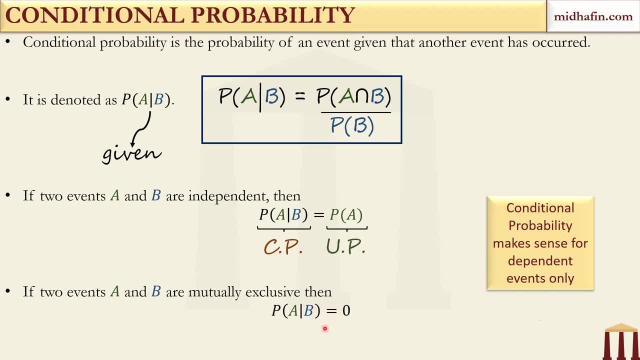 It will be equal to zero. This is also something which we have derived, but you can understand it logically. Let's forget the mathematical definition right now. Mathematical definition is also quite easy. In fact, you just substitute P A, intersection B as zero in the numerator. 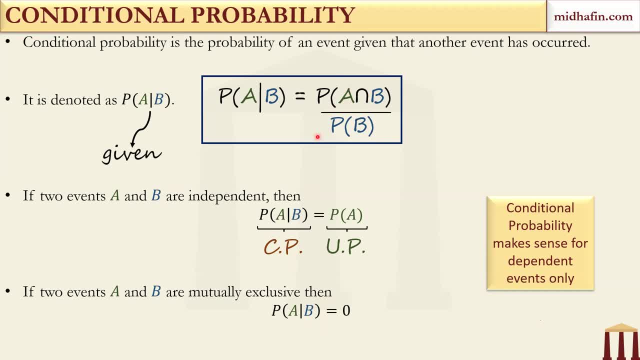 you'll get zero because for mutually exclusive events the numerator itself is zero. But logically also, it's quite clear, right? If they are mutually exclusive events, then if B has already occurred, then it is guaranteed that A will not occur. So obviously P A, given B, has to be equal to zero. 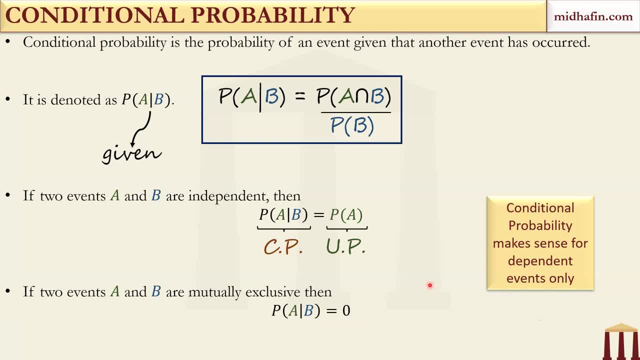 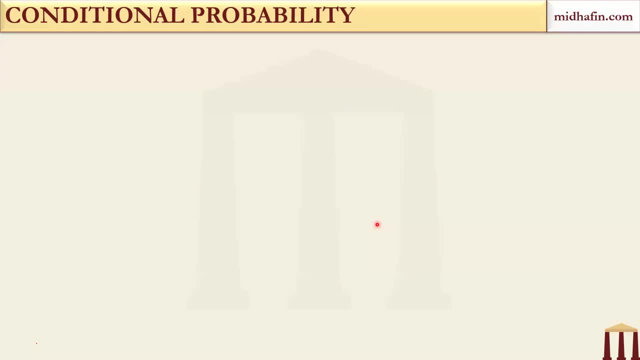 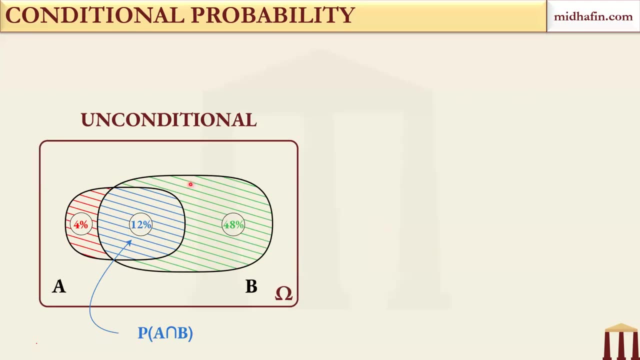 If B has occurred, A can never occur. Okay, Now comes the important part, As I told you: visualization of conditional probability. Visualization is very, very important. It makes you understand how conditional probability actually should be interpreted. So let's say- this is an example which I have taken- 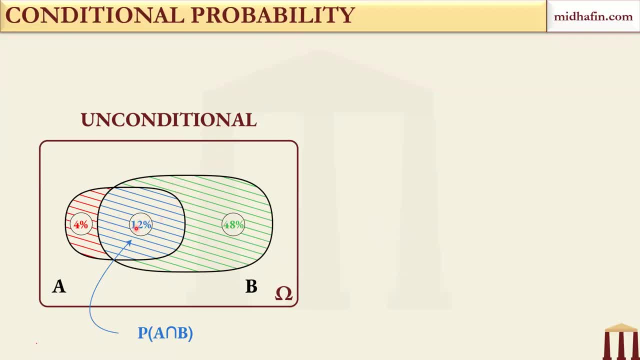 Now just quickly pitch in past. What is P A over here? I told you, probabilities are demarcated region wise: 16. 16%, Very good. What is P B? 60.. 60%, Very good. 48 plus 12,. 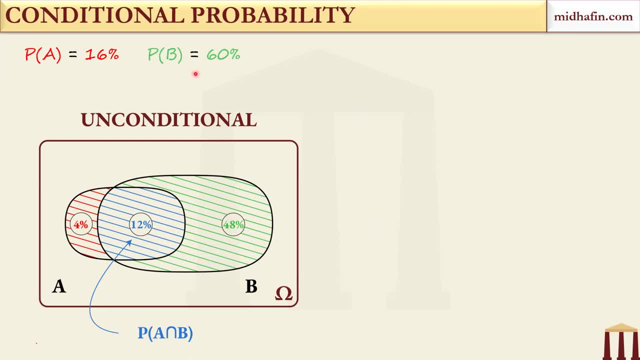 60.. 4 plus 12, 16.. So P A is this much? P B is this much? Okay, And P A intersection B is obviously 0.12 or 12%. Now, if you do the mathematical calculation, 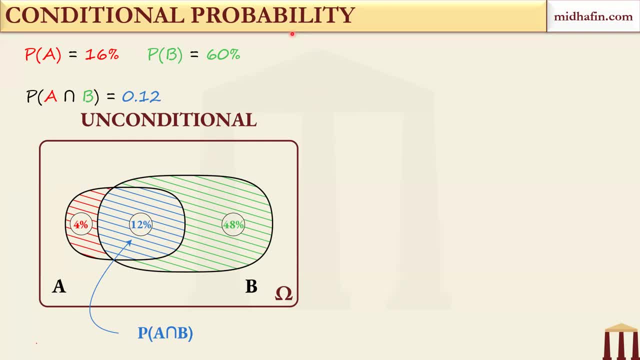 you will get a result like this. Now, if you do the mathematical calculation, if you do the mathematical calculation, you can get it quite easily. You can get: P A intersection A given B is equal to P A intersection B by P B. 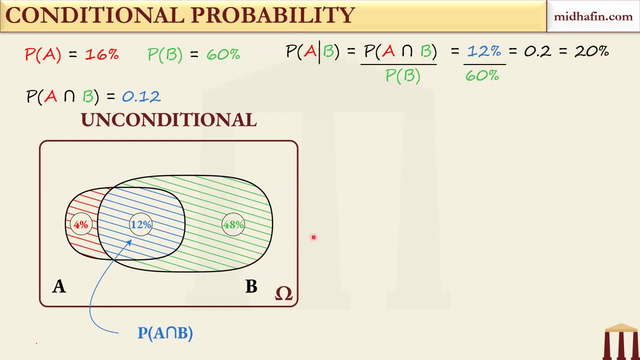 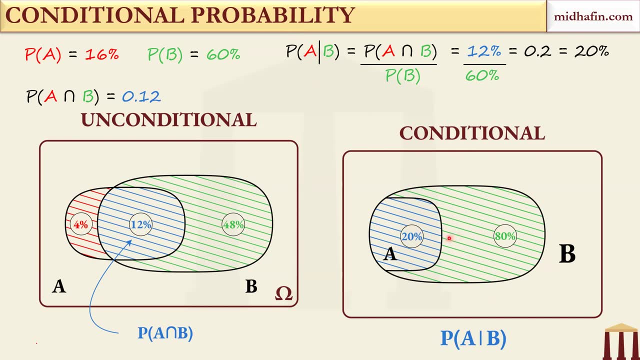 which is nothing but 20%. Now how to visualize it. This is how we visualize it, So I'll explain. See, there are two universes over here. One is my original universe, So this Sigma or S, whatever you may call it. 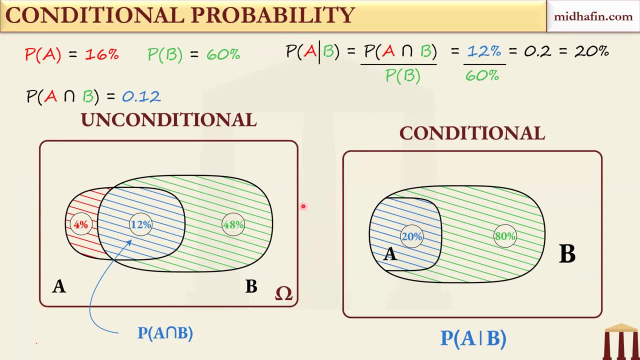 this entire sample space is my old universe, So initially, all possible outcomes of our experiment are considered. So this is your full sample space. Okay, Now what you have done? you have built a new universe. You let go of the rectangle. 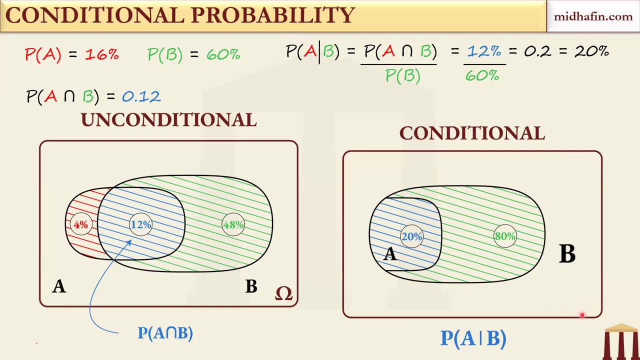 In fact, in this diagram you ignore the rectangle and that's why I have not written any Sigma in this diagram. So this is this does not exist. Okay, Now your new universe is actually B, so everything is happening inside B, because B is something which has already happened. 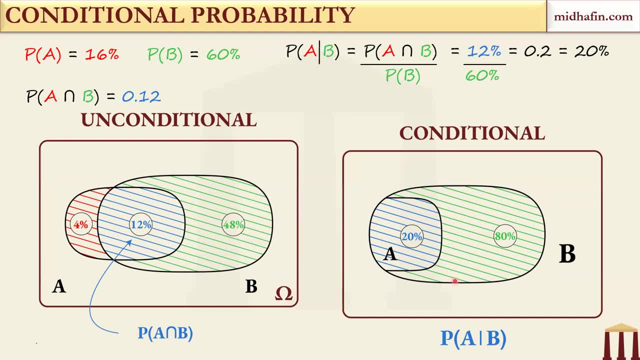 B has already occurred. So this is your new universe. So when you condition on an event B, you actually restrict this universe to only those outcomes where this B has occurred. Okay, So this subset now of your original universe, because in the original universe 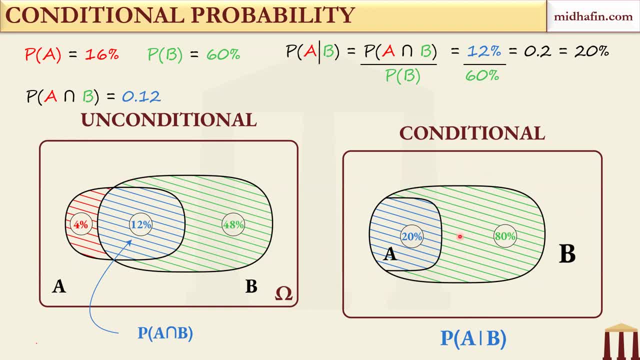 B is nothing but a subset of the original universe. So this subset of your original universe now becomes your new universe and it becomes your new sample space. Okay, Is it clear? This B has now become your new sample space. So B is not just any subset. 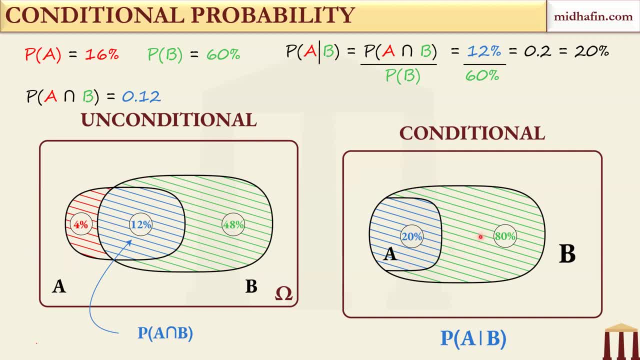 It is now the effective universe in which all the further probabilities base, based on the condition that this is your new universe, or B has already occurred. All the future probabilities will now be updated and calculated. And finally, you are seeing that, if I want to find out conditional probability, 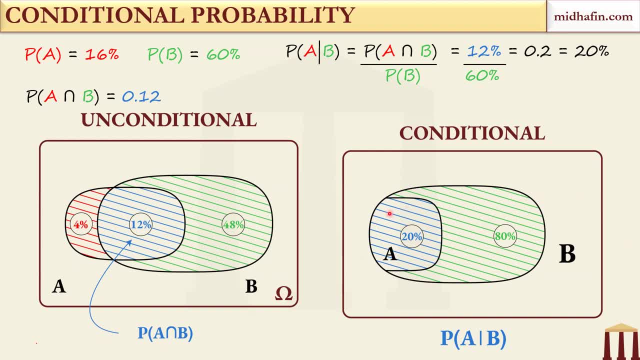 there is a dependence on intersection now. So now, since everything outside of B is ignored, so it means this red region is now gone. So this portion of A will not be considered, Only the portion of A will not be considered. Only the portion of A will not be considered. 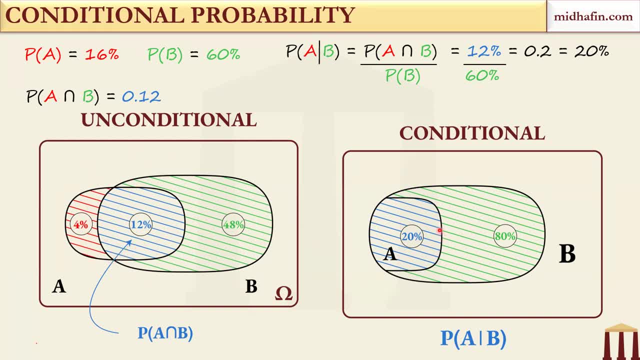 Only the portion of A which was common to B or inside B now will be considered. So the probability of observing A given B is dependent on A intersection B. now, Okay, And now you can see that, since your new universe, instead of this, 100%. 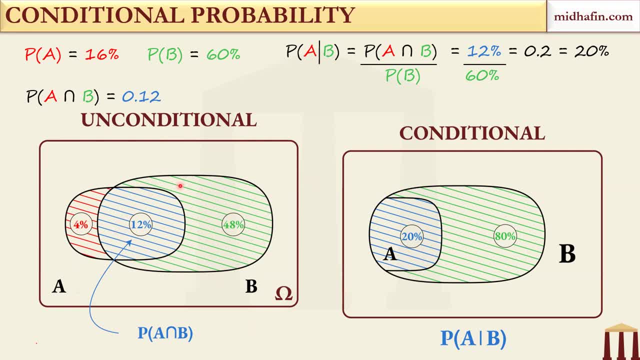 the new universe has become 60%. Okay, So if 60% is now your new universe, so that is why 12% has been scaled up to 20%, Because if 60%, this entire 48 plus 12, which is 60%. 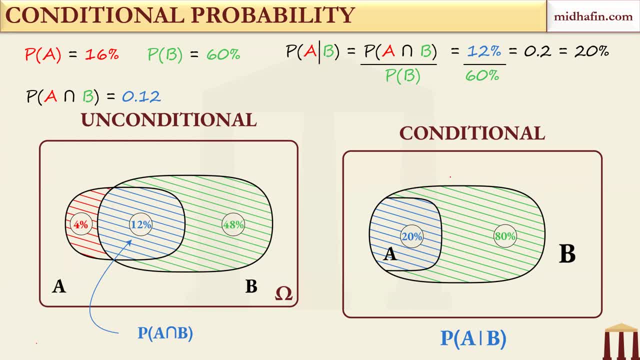 is now your 100%. this total is how much? now 80 plus 20?? This now becomes your 100%. So, out of this 100%, what is the space taken by the common region of A and B? 20%? This is your conditional probability. 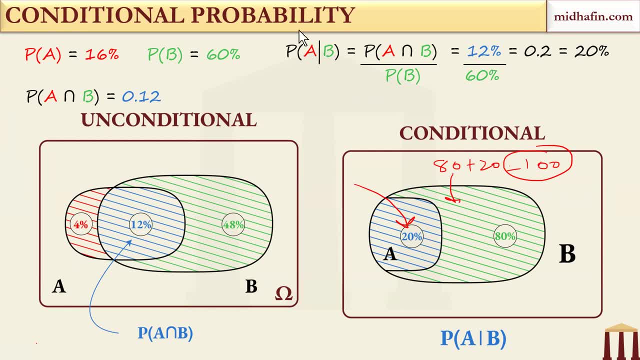 Is the visual interpretation clear to everyone That how, in conditional probability, your universe changes. first The new universe becomes this set, B right, And then, based on this new set, the new universe, you actually find out what proportion of A is inside this new universe. 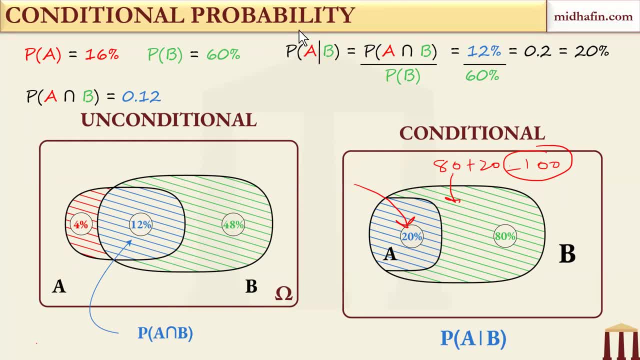 So 20% of A is inside your new universe. Okay, Leaving everything outside of B. So this part of A is not considered. now This part is gone, Only the part which is inside B. how much percentage of that occupies B? 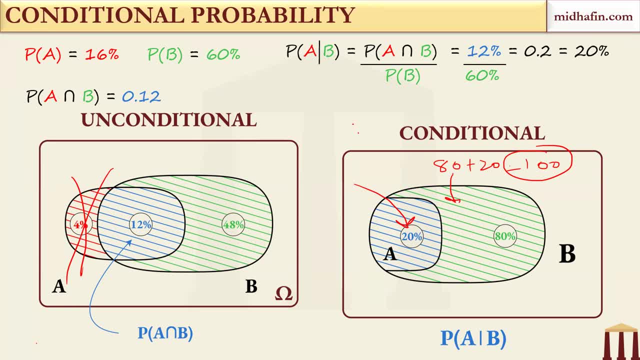 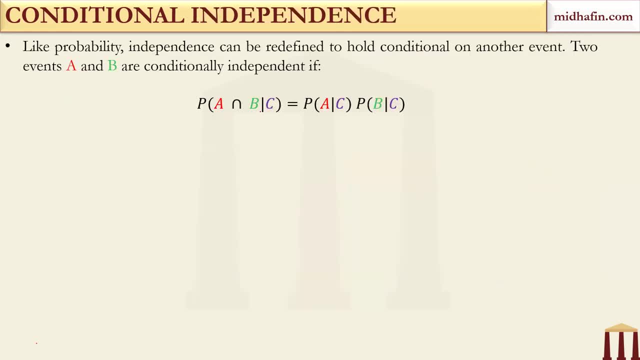 That is your conditional probability And it means that B has already occurred. B is your new universe. Okay, And again, these things we have done in great detail in the class, So this was the best possible way in which it could have been explained in a short way. 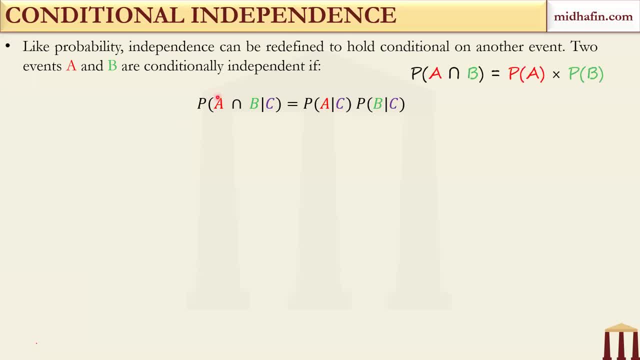 Now, like probability, independence can be redefined to hold conditional on another event. So this is the algebra for conditionally independent events. So P A intersection B given C is equal to P A given C times P B given C. This is quite similar. 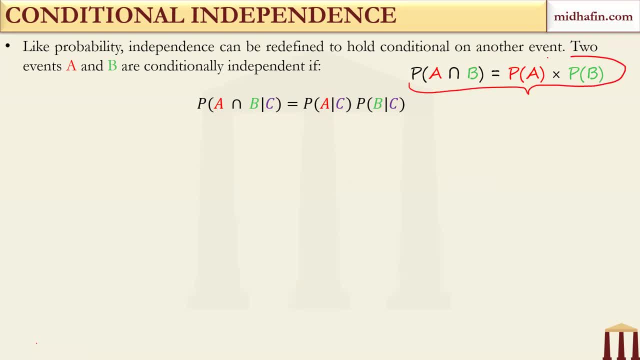 In fact, quite similar- I will say identical almost, In fact, to this. this was the independence condition, normal independence condition, Okay, And this is the conditional independence condition, Okay. So this is the difference. Again, we have discussed an example in the. 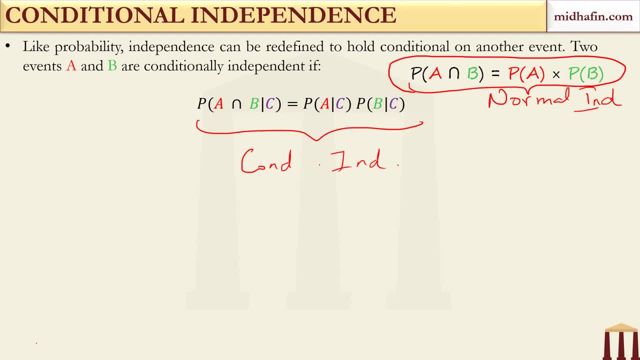 the live class and the self-paced course, but that is very, very detailed. The visualization has been discussed of conditional independence also, But I think from the exam point of view this is sufficient for you because probably it might not be asked the visualization part. 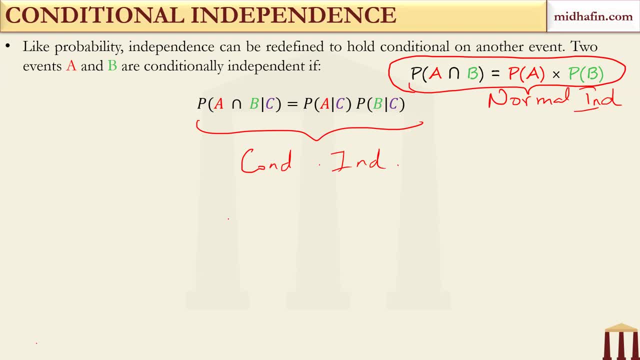 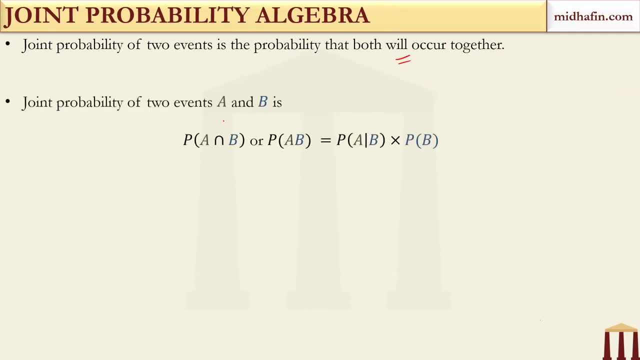 If conditional probability visualization is clear, then you will be able to visualize this also. Now let us come to joint probability. Joint probability for two events is the probability that both will occur together. This is the formula for joint probability: P A, intersection B or P A- B. 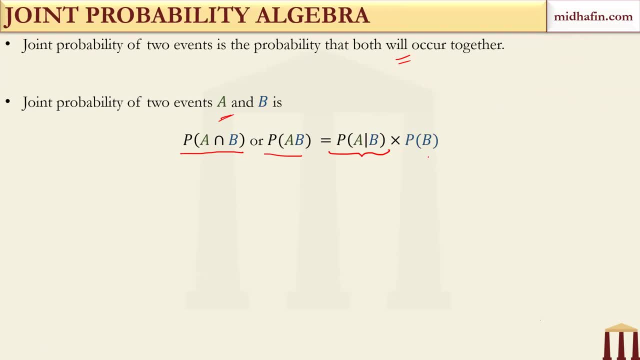 is equal to P A given B times P B, P A given B times P B. And, of course, if they were independent events, then this would be replaced by P A in that case, if they were independent events. If they are not independent events, 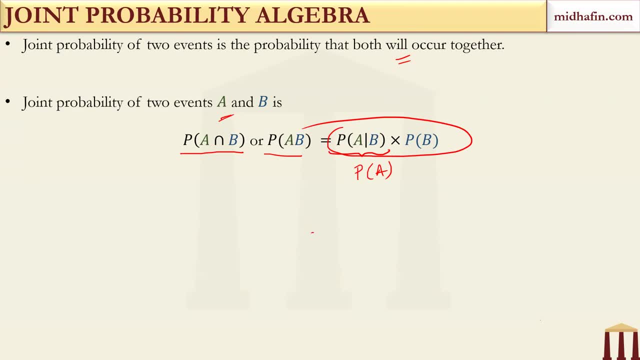 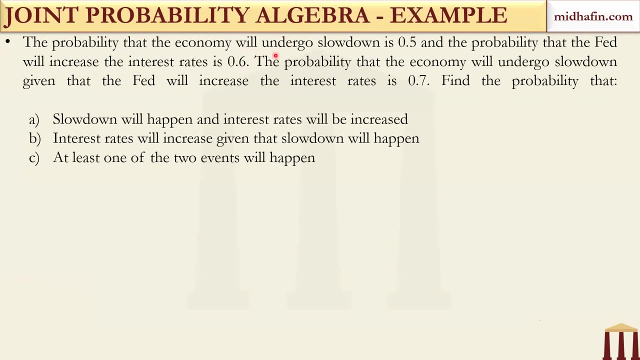 then. this is the general algebra for joint probability. Okay, Next, So let us discuss an example. The probability that the economy will undergo slowdown is 0.5.. And the probability that the Fed will increase the interest rates is 0.6.. 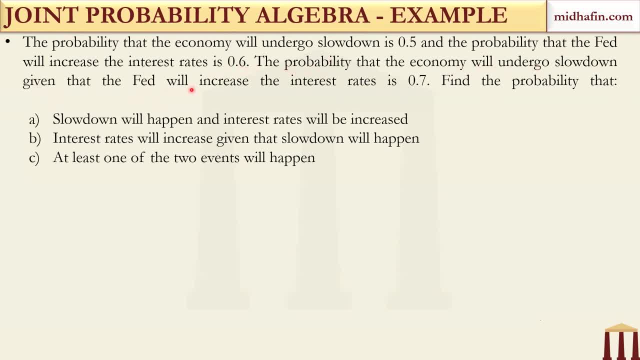 The probability that the economy will undergo slowdown, given that the Fed will increase the interest rates, is 0.7.. These probabilities you have to find out First. one slowdown will happen and interest rates will be increased. So the first job always: 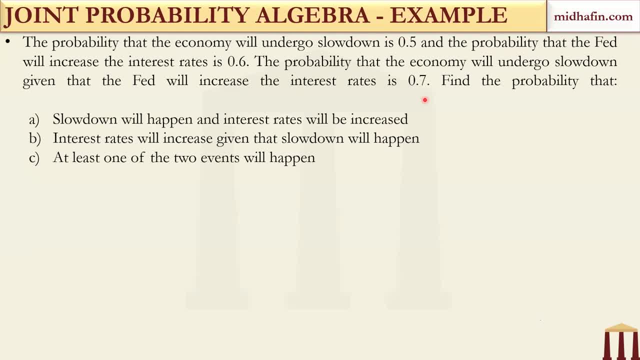 when you see the question in the exam should be to translate the literal language into mathematical notations. That's your half. the battle is won there. only That is what I say to my candidates, If you are able to just transform them into the probability notations. 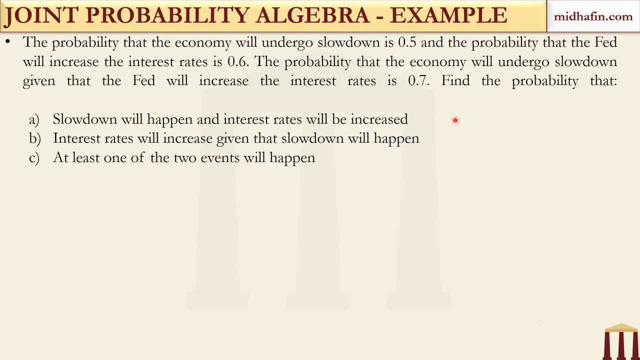 and in terms of probability, then your job becomes quite easy. So this part over here, if you see, this part economy will undergo slowdown, is 0.5.. This is nothing but P? S If we assume this is event S, slowdown is event S. 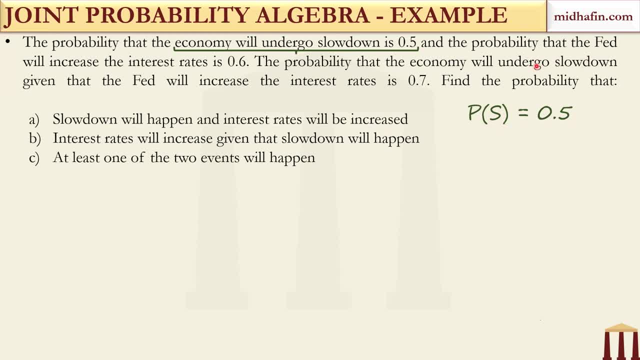 So P S is given as 0.5.. Let's assume that increase in interest rates. the event is I, So P I is given as 0.6.. Now also one of the conditional probabilities is given. Can you tell me what is given? 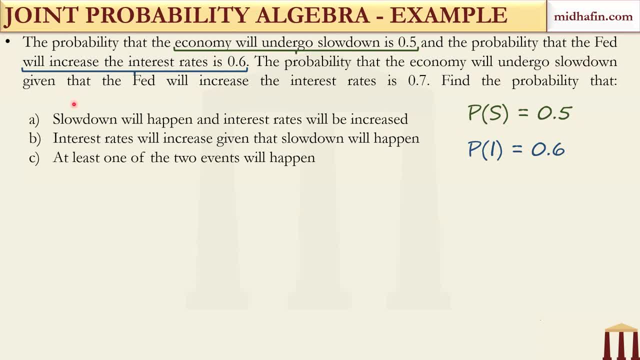 Is it P S given I or is it P I given S? What is given? What is provided in the question? P S given I or I given S Quickly S given I, Perfect. So it's provided that P S given I is 0.7.. 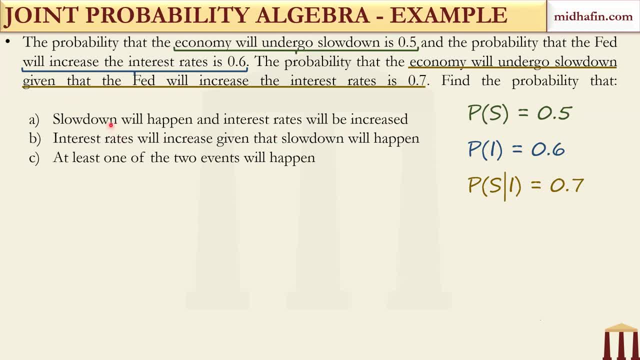 This is what this information is provided to you. So first thing that you have to calculate is S intersection I. You can see that and is there? Slowdown will happen and interest rate will be increased. So we'll just use the joint probability. 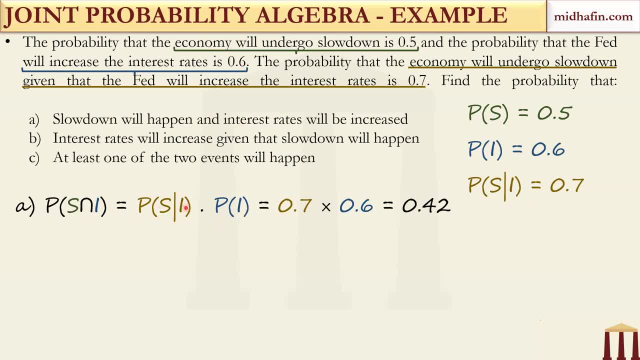 P? S intersection I is equal to P S given I times P I, which is 0.42.. Next you have to calculate I given S. So again, we'll simply use the conditional probability algebra. P I given S is nothing but. 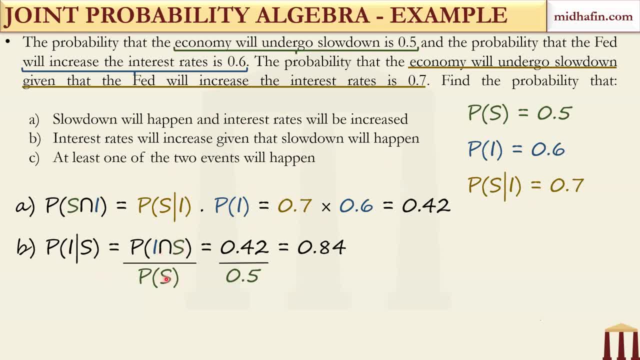 P, I intersection S, divided by P- S. And of course, it is quite clear that I intersection S and S intersection I. they are the same event. There's no difference, right? There's no difference. Whichever you write first, it doesn't make any difference. 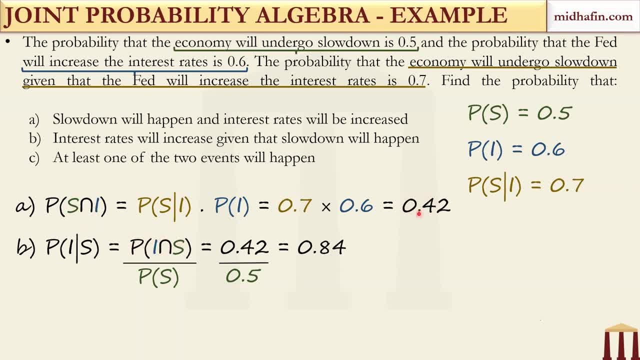 So the probability of I intersection S is also same as 0.42.. So this becomes 0.84.. Then you have to find out at least one of them will happen, At least one of them Now in the exam. they might not be very direct. 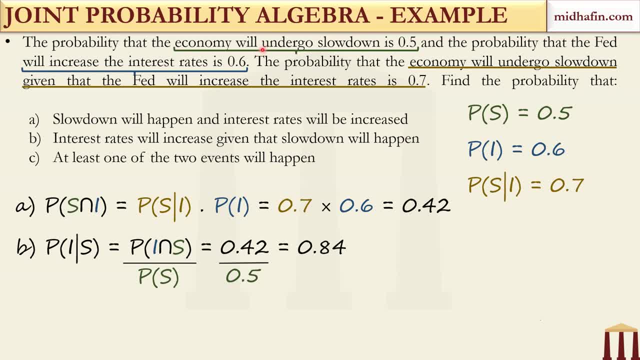 Find the probability of A union B- They might not ask like that- or find the probability of A over B. So it will be very obvious to you In the exam. they might frame the question like this: At least one of the two events will happen. 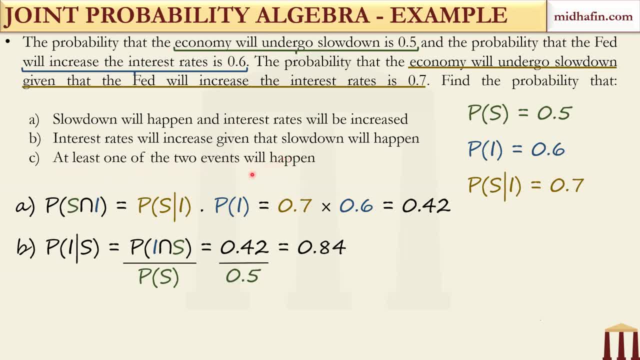 So try and understand what is the meaning of at least Either A or B or both. Either only A or only B, or both. Okay, so at least one is nothing. but they are actually talking about union over here, So this question has been framed. 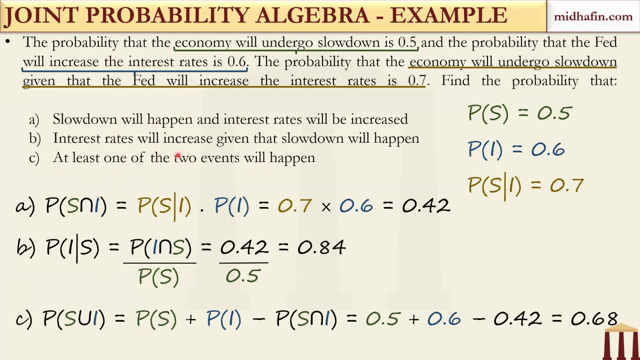 to make you understand a lot of things that they can ask you in the exam in different terms also Okay. And how they can extend the idea of conditional probability to include intersection events. Okay, you just have to calculate intersection, Then you have to calculate the opposite. 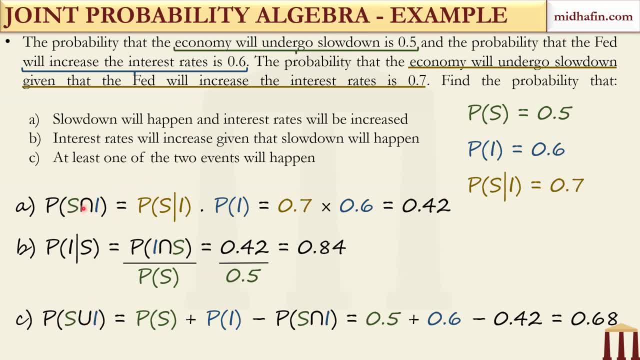 And you may also have to calculate union part, which they frame in a different language. So at least one of them is also nothing but union. So this is quite simple. Now it becomes 0.68.. So see why we are skipping a very 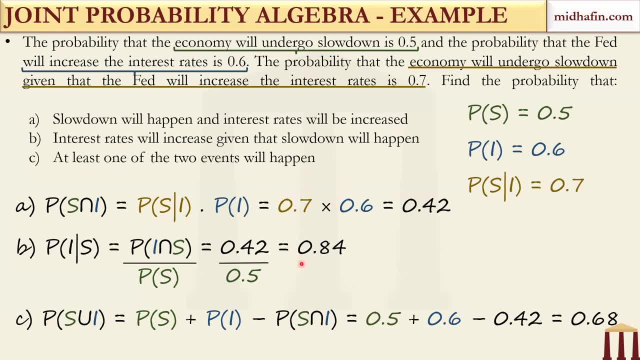 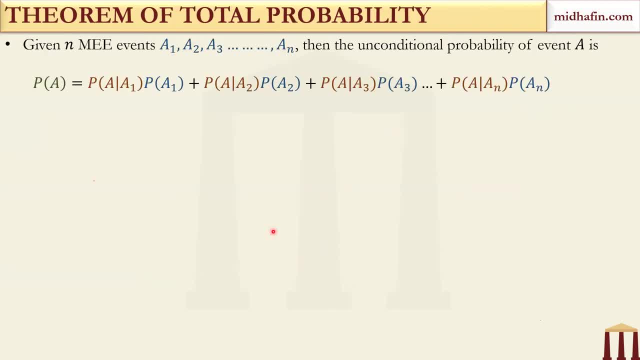 we are doing these things very quickly, These slides. Hopefully we take some time because you already you will have the PDF right to revise. So we will just do these things very, very quickly. And I said in the beginning only that I'm assuming. 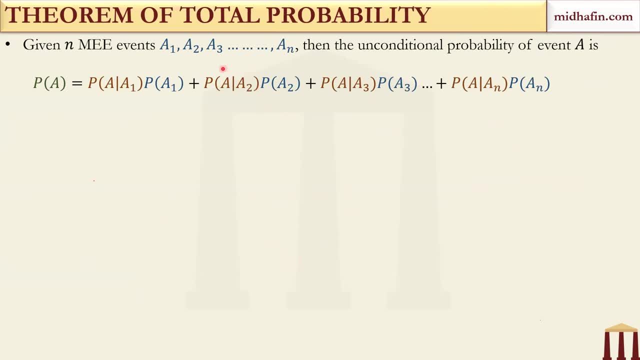 that you have completed the course at least once. Now I said that MEE events. these are very special class of events. Any unconditional probability can be calculated from conditional probability if the events which have already occurred, they are mutually exclusive and exhaustive events. 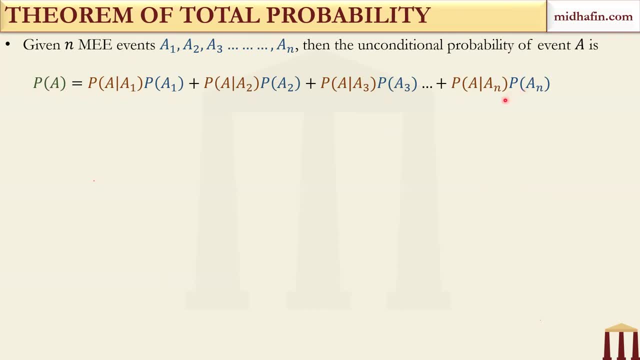 So this is the theorem of total probability. Again, a very beautiful visualization we have done for the theorem of total probability. But from the exam point of view the special case is more important actually, Because you know that two events, B and B, bar. 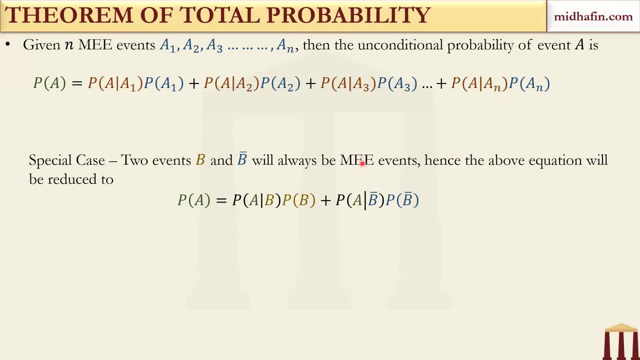 they will always be mutually exclusive and exhaustive events, for sure. Guaranteed B and B bar. You draw the diagram over here. Suppose you have B over here And B bar is outside of B, So this is your B bar. So can I say that B and B bar or B and B complement? 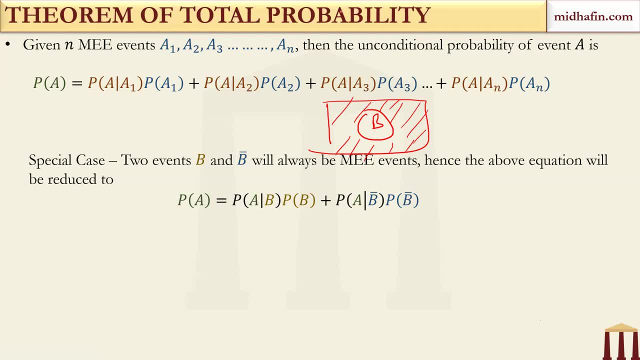 they are mutually exclusive also and exhaustive also. Do you agree or not? A very important and subtle observation, But very, very important, as I said, from the point of view of the exam, Because there is nothing common between them. B bar is outside of B. 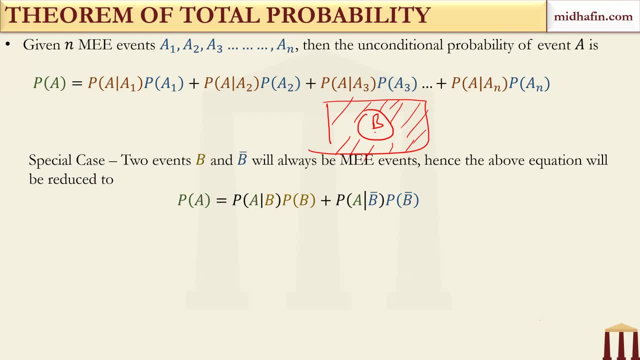 So they are mutually exclusive. They are exhaustive also Because when you combine them, when you combine the circle and the outside part, what do you get? Do you get the entire sample space? Yes, So B and B bar will always be mutually exclusive. 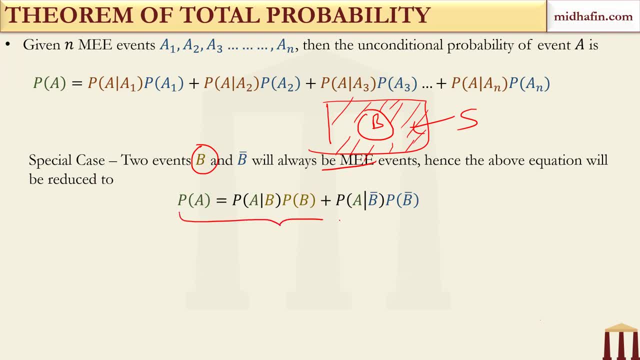 and exhaustive events. So this will be the algebra for mutually exclusive and exhaustive events. Now, this is one way to remember the theorem of total probability. Either you use the formula, Okay, Or you use the tree diagram, which is way too simple, And that is what we have recommended in the class also. 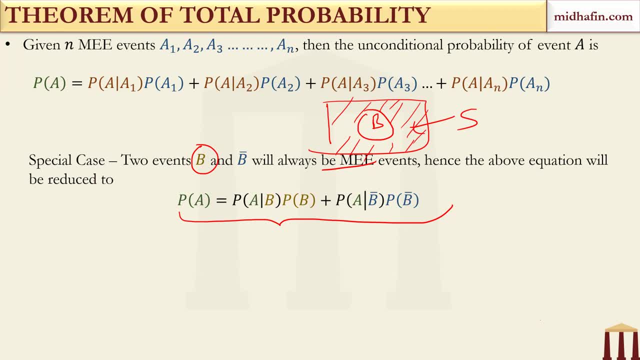 Although we have solved the question using both the methods Today. also, we will do that. We will take an example And we will solve them using both tree diagram as well as this formula. Okay, But I think it is important that you understand the formulas. 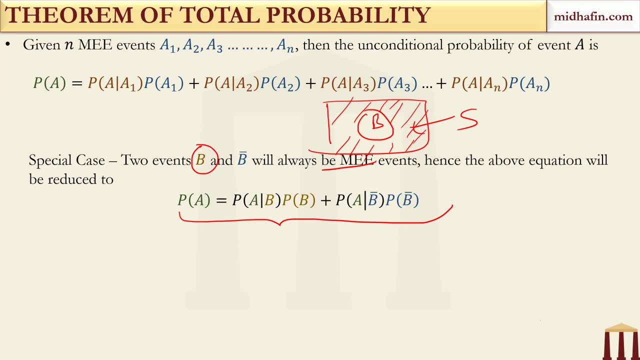 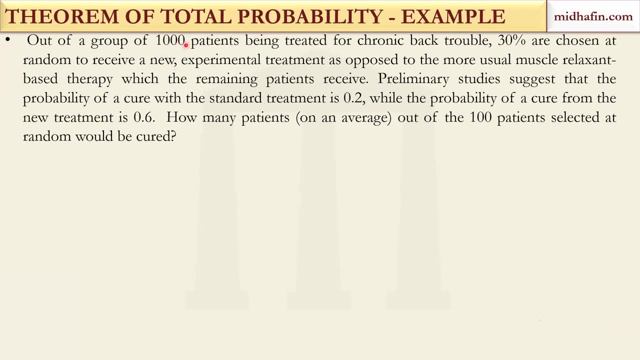 Definitely in the exam. use the tree diagram without any doubt, But understand the logic behind the formulas. So this is an example. Out of a group of 1000 patients being treated for chronic back pain trouble, 30% are chosen at random to receive a new experimental treatment. 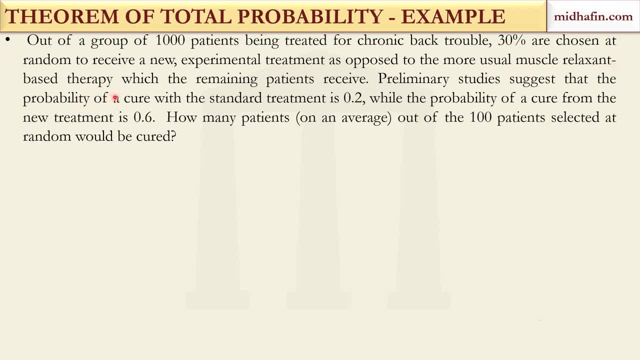 as opposed to the more usual muscle relaxant based therapy which the remaining patients receive. Preliminary studies suggest that the probability of a cure with the standard treatment is 20%. So 30% are receiving new treatment And the probability of cure with the standard treatment is 0.2, 20%. 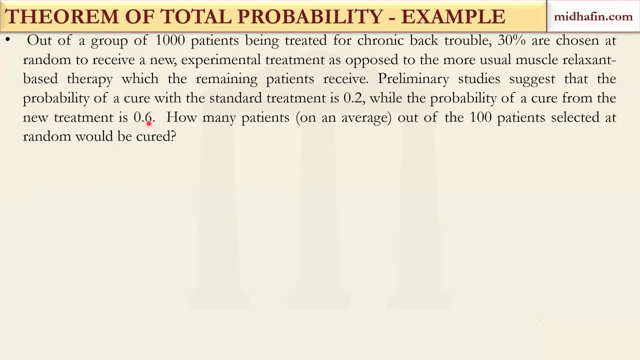 But for the new treatment, the probability is 60%. So how many patients out of 100 patients selected at random would be cured? So the first thing I will do for you, I will just define the events in terms of alphabets. 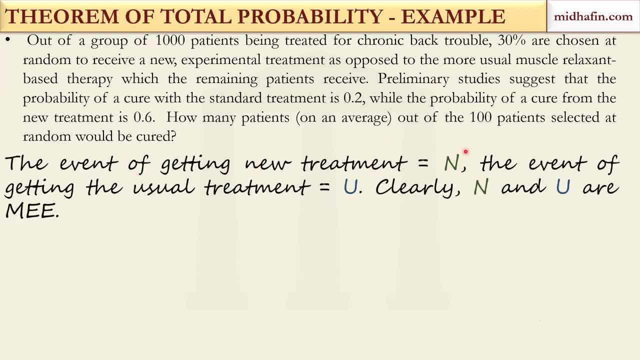 So let's assume that the event of getting new treatment is capital N, The event of getting the usual treatment is capital U. Do you agree that N and U are mutually exclusive, as well as exhaustive Yes or no, Because N is nothing but U bar V. 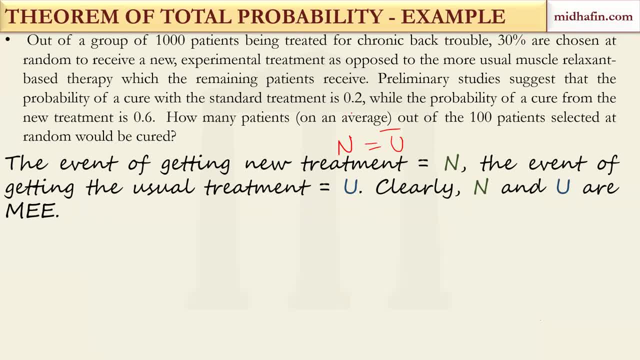 Those who receive the standard treatment, they don't receive the new treatment. Those who don't receive the new treatment, they receive the standard treatment. So at least either they will receive the new or the standard. So they are actually combining the sample space. 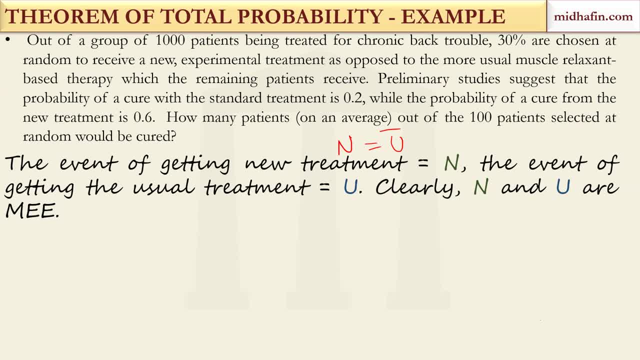 All the patients are included, 1000 patients. all are included, either new or standard. So they are definitely exhausted. They are mutually exclusive, also because one patient cannot get both at the same time. Either the patient, he or she will get new, or he or she will get standard. 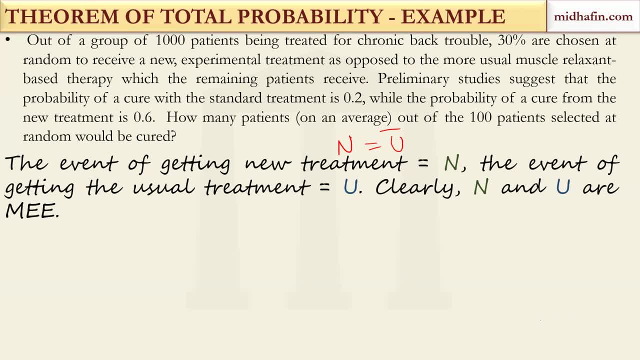 Or usual standard. I mean usual treatment. Okay, So what is PN? Tell me PN, If I only have to find out PN. what is PN from the question Quickly? What is PN from the question? Very good, 30%. 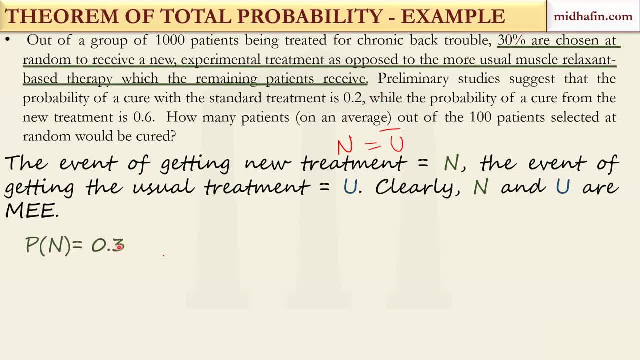 In fact it is given, So you can say that simply 0.3, right, 30%, at random. Okay, What is PU? What is PU Correct? 1 minus 30% or 1 minus 0.3, 100% minus 30%. 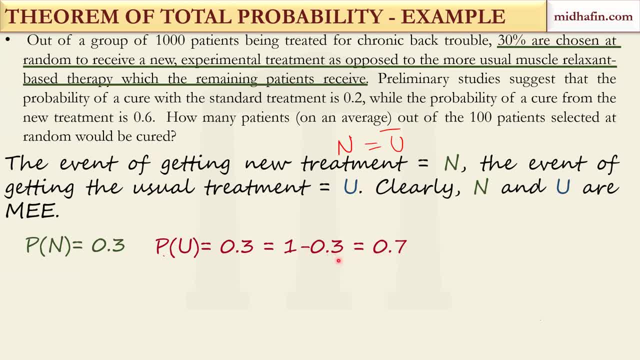 whatever you want to call it, 70% or 0.7.. Okay, Now tell me one thing. This statement over here, here, with the standard treatment, what kind of probability is this? Conditional or unconditional? Quickly, According to you, 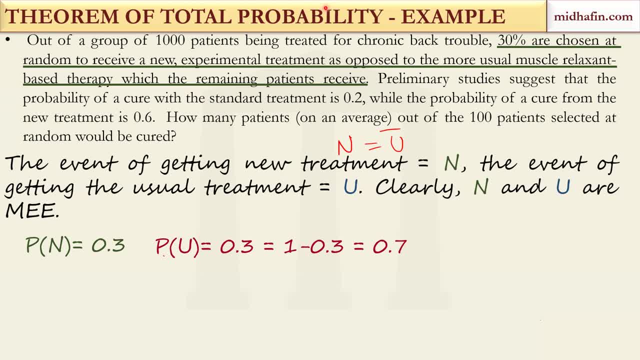 Is this conditional or is it unconditional probability? Conditional, Very good, It is conditional probability. As I said, if you are able to transform the statement into a mathematical notation, the job becomes quite easy. So can I say that this statement implies P, C, give. 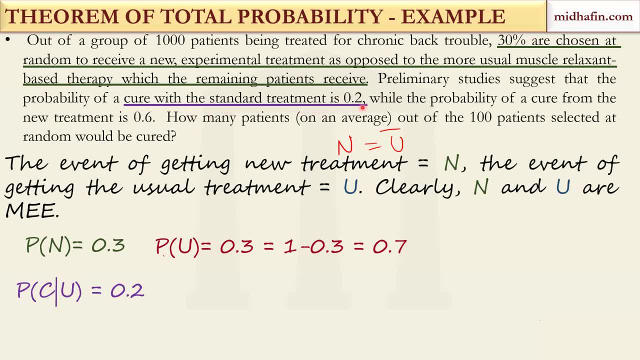 and I have tried to color code it as much as possible. I mean, sometimes it might not be there, but mostly you will find that if suppose this is a purple line, then the equation will also be in purple in most of the cases. 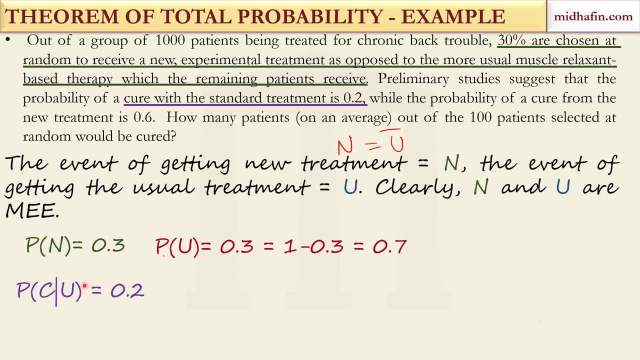 So cure with the standard treatment is 0.2.. So it means that, given that the patient received the usual treatment, the patient got cured. the probability is 0.2.. So do you agree that 0.2 is nothing but P? C given U? 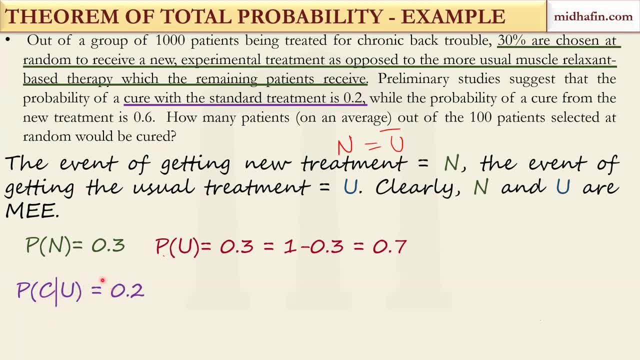 Is this part clear to everyone? Okay, And just one quick note I want to give you Again. everyone has a different way of understanding and perceiving things and remembering things, and they have their own tips and tricks for the exam. So for me, I always used to write conditional probability. 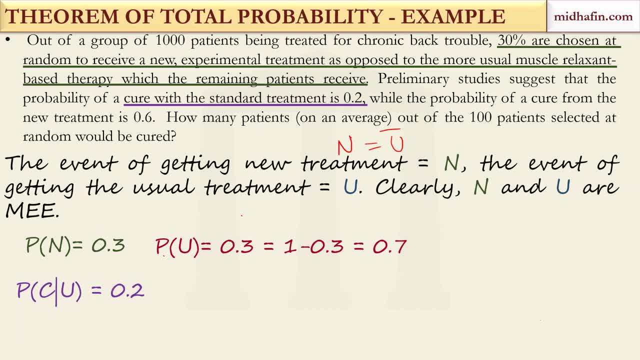 When I was preparing, when I saw conditional probability for the first time in class 11, can you just mute your microphone please, if you are not speaking? So when I used to write conditional probability, I had this tendency. I don't know whether it works for you or not. 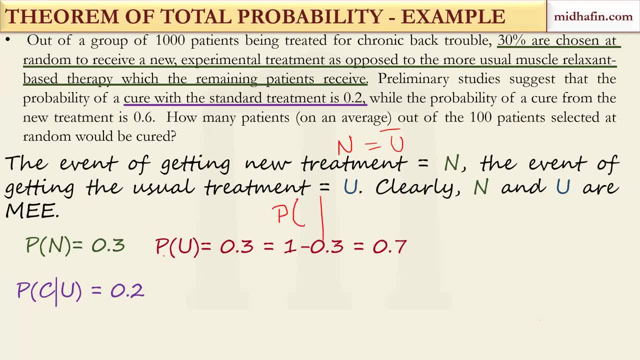 that I will write P and I will write the given event first. So I will write this first and then I will write this. So this is my way of making things easier for myself. Again, if it works for you, then it's good. 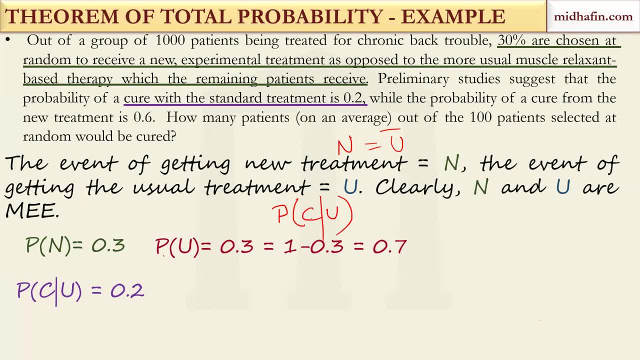 Otherwise you can use your own way, right, Because it makes it, yeah, okay, okay, yeah. So actually it makes my job easier. That's what I feel. So, given if it is, given that the standard treatment is there, 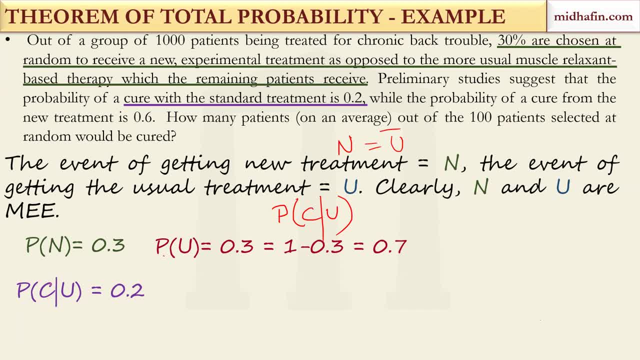 so I write P given, U is given. Then after that the patient has been cured, So 0.2.. Okay, now can you tell me from this line, cure from the new treatment. what can I write? similarly, Cure from the new treatment is 0.6.. 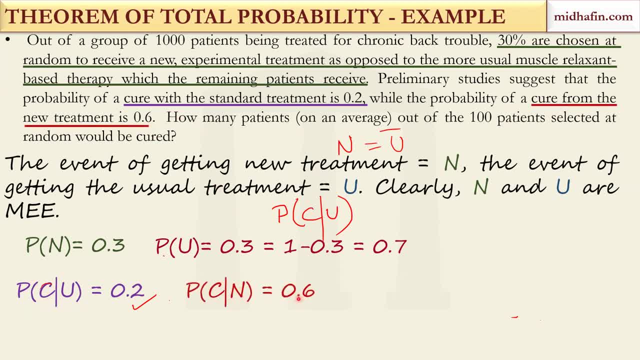 Can I write this: PC, given N is 0.6.. Agreed, Okay, fine, Great. So then now it becomes quite easy. You have: PC is equal to PC, given U. Use the conditional probability formula And you'll get this as: 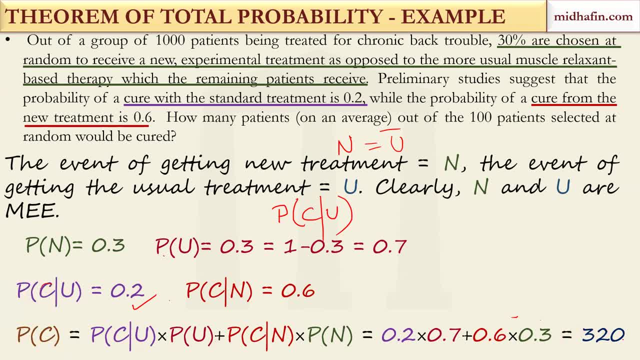 in fact, you'll get this as 0.32.. There's a typo over here. This will be 0.32.. Okay, 320 is basically calculated after this number is multiplied with 1000, because there are 1000 patients. 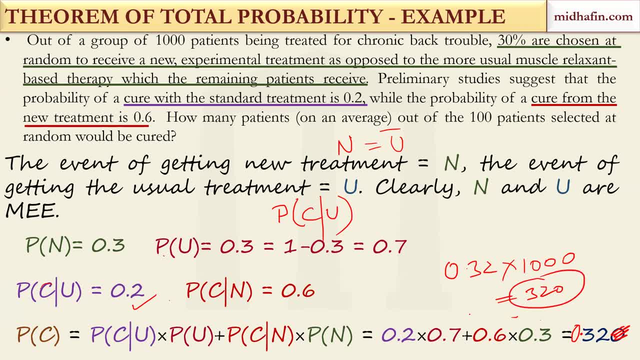 So, to find out the number, you'll have 320 patients, because the probability you'll get as 0.32.. So obviously the total number of patients will be 32% of 1000 patients. Okay, 32% of 1000.. 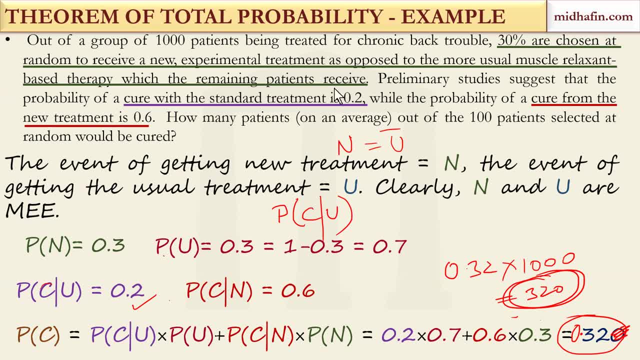 Okay, Now the same question. as I said, we solve using tree diagram. only Now, actually, again, there's a typo. Sorry, Divesh, there's a typo. Actually, this you can see this is 1000,. 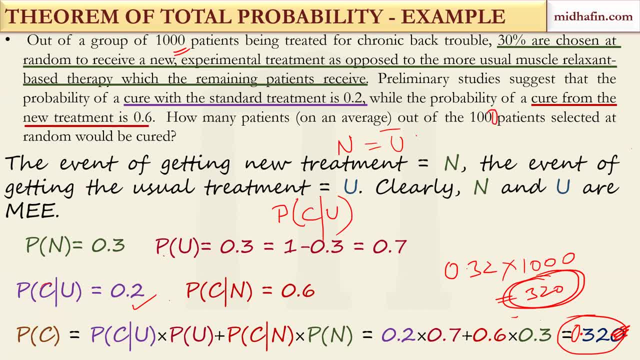 right Over here And, by mistake, instead of 100,, 1000, they have by mistake- it's a typo, So it will be 1000.. Okay, This is a typo, Got it. So 1000 patients are being treated. 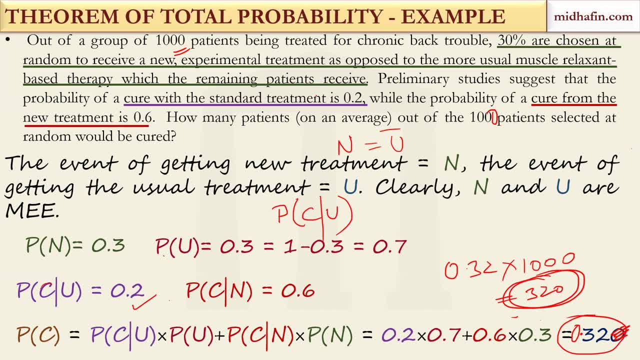 And the final answer has to also be calculated. Okay, This is a typo, So is the formula application clear? How to transform the statements into notations: Is this clear? Okay, And then the formula application: Fine, And when we solve this using the tree diagram? 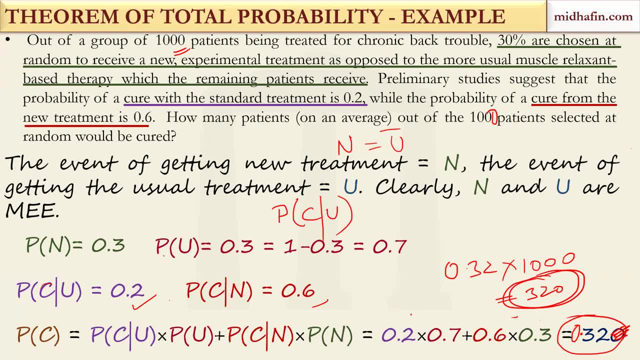 I think almost all of you will agree that tree diagram is simpler. But, as I say, you should always try and understand the answer. Okay, try and understand the application of the formula first and then go for the tree length. So first we'll see what is Bayes theorem and then we'll come back to that same question later on. 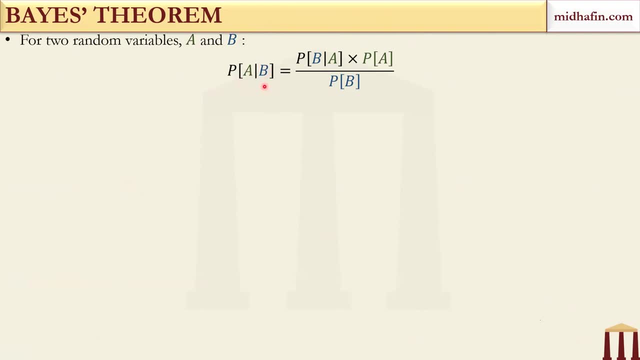 So this is what Bayes theorem is and again the derivation we have done in the video. it is quite simple, but over here we'll just focus on the statement of the Bayes theorem. For two random variables, P is equal to P multiplied by P. So over here the conditional. 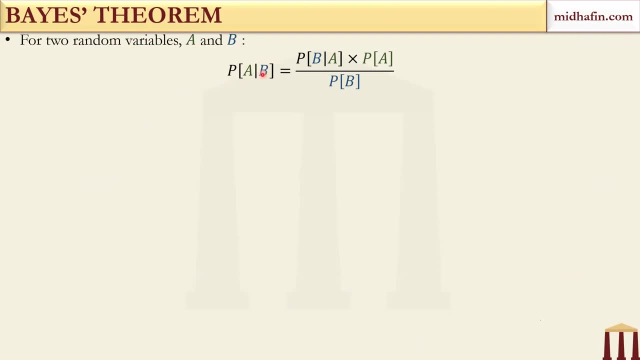 probability you have to calculate, conditioned on B, and the input that you use is the conditional probability conditioned on A. So you reverse this, okay, and then you multiply it with P and divide it with P Again. this is the formula which many of you might remember, using different tricks. 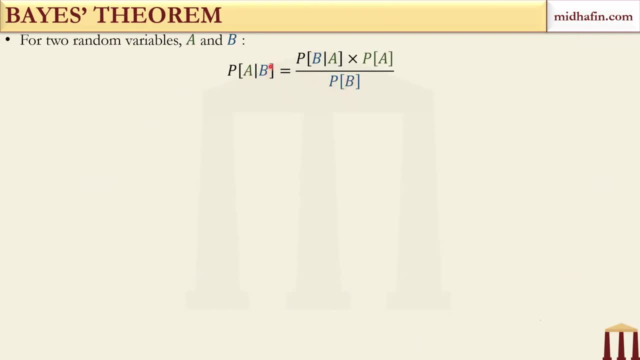 either you can use or remember it by multiplying P to the left hand side and by seeing that both of them are finally same P. that is what the derivation we have done in our video, or else you can remember it in a very straight, a different manner. you can see that B is given over here, so just 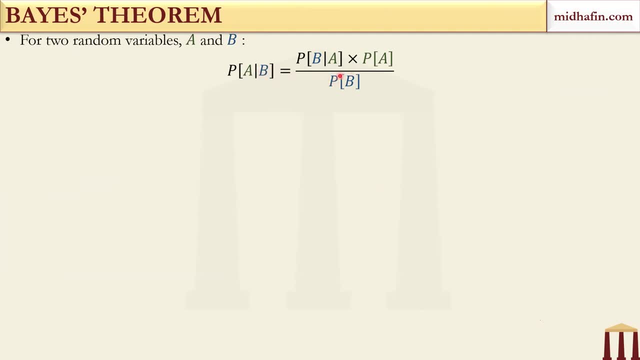 remember in your mind that since B is given over here, so let's place B in the denominator on the right hand side and this will be reversed. okay, P given A will be reversed and then it will be multiplied with P. but of course, if you remember the visual derivation and the proper derivation, 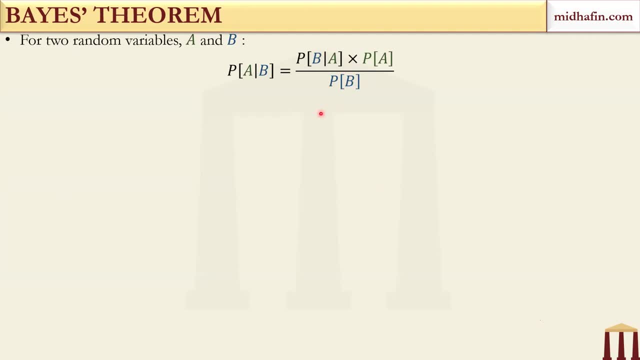 then even this will not be required. okay, this trick will not be required again. your choice, completely. So what is Bayes theorem? Bayes theorem is a plan to change our beliefs in the face of new evidence. so till now, whatever evidence you had, you calculated some probabilities. 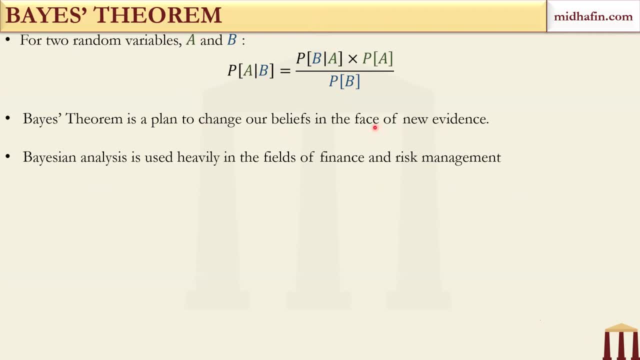 now, based on new evidence, you are updating your probabilities, and that is what Bayes theorem does for you, and it is, although a very, very simple formula, but it is used heavily in the fields of finance and risk management. One thing which you need to note is that this denominator- 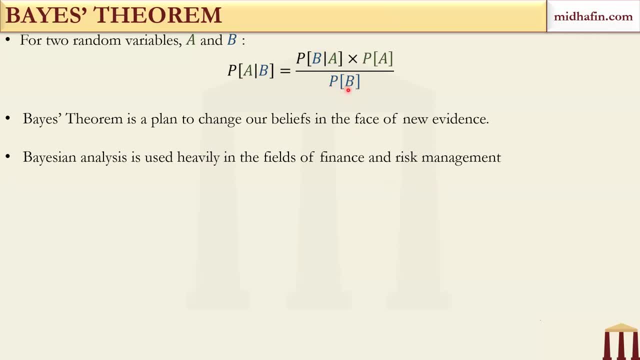 has to be calculated using the theorem of total probability. that is where total probability comes into picture in Bayes theorem, this denominator, remember it- has to be calculated using the theorem of total probability, pb. whether you use the formula or the tree diagram is your choice, but it has to be the theorem of total probability. okay. 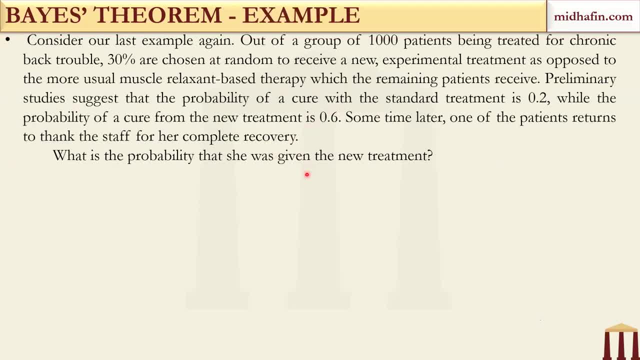 So let's go for the same example. example. so the complete statements, all of them are same, but there is some new evidence. this last line presents the new evidence. sometime later, one of the patients returns to thank the staff for her complete recovery. this is your new evidence, and now you have to find out, based on this new evidence, that what is. 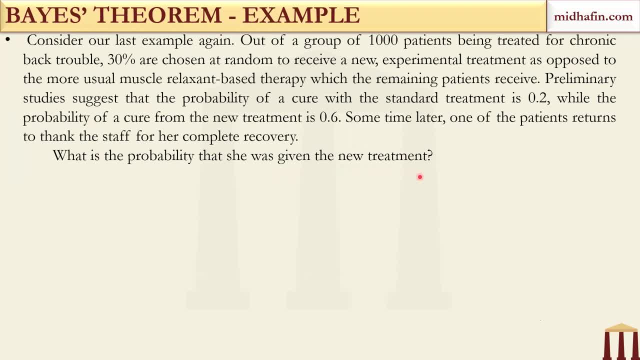 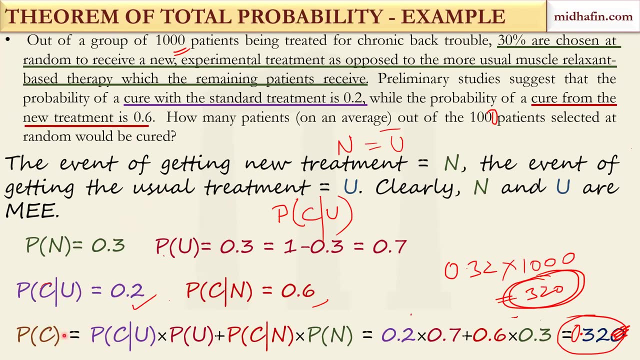 the probability that she was given the new treatment now PC has already been calculated in the previous exam PC- the probability of being cured has already been calculated. this is the unconditional probability based on both the treatments. okay, it was 32%. the probability of being cured is 32% already. 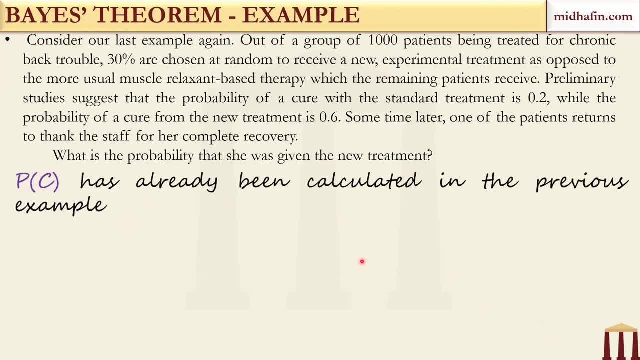 calculated. can you tell me what you have to calculate in this case? which conditional probability you have to calculate what is given to you? now tell me what is given to you. this last line will tell you what is given to you worth: C yes or no? Okay, great, C given N was no Pooja C. C given N, we don't have to. 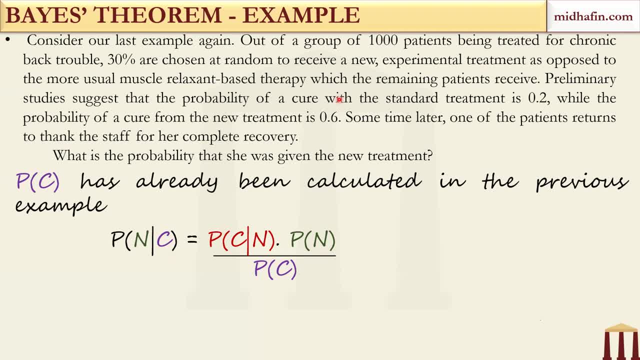 calculate. Okay, Pooja, we have to calculate N given C because C is given. See sometime later one of the patients returns to thank the staff for her complete recovery, Pooja, Okay, So the patient, she goes and she thanks the staff for her complete recovery. It means 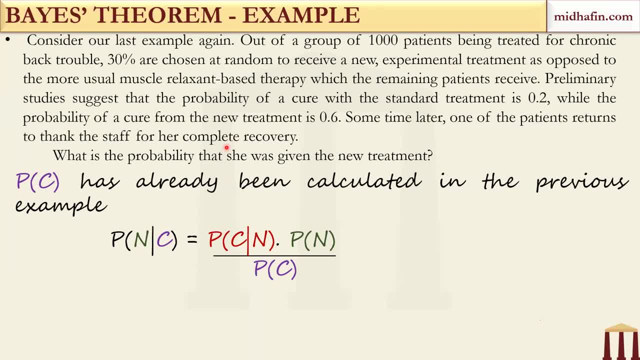 the patient has been cured. Agreed, Pooja. Okay. So given that she has been cured, what is the probability that she was given the new treatment? P, N, given C. And that is why I say, once you are able to formulate the notations, you know, once you are able to. 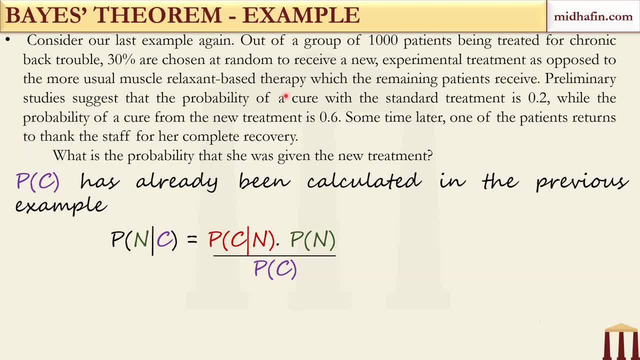 understand clearly what you have to calculate, then your job is more than 50% done. Then you just have to apply the formula or use the concept or the diagram. Finished. So P C given N. It was already provided in the question. What is the information with? 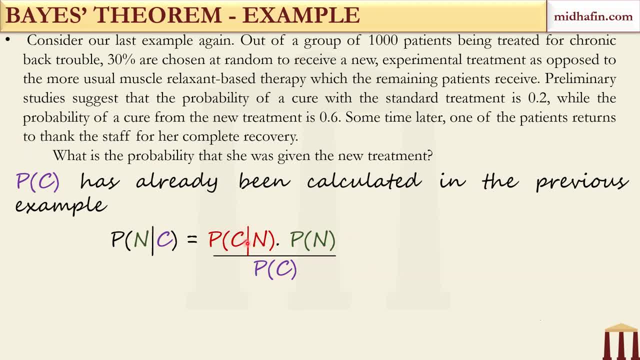 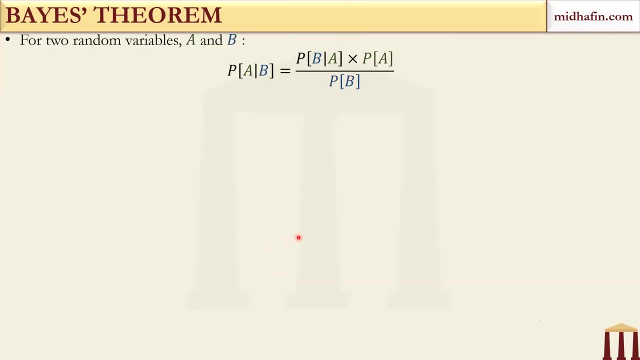 respect to P C given N in the question. I will not go back to the previous slide. I want you guys again to look at the example and tell me what is P C given N? What is P C given N? 0.6.. 0.6.. Very good, This is exactly what we did earlier. also, P C given. 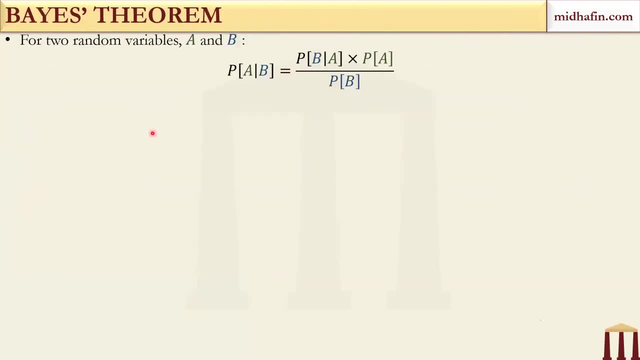 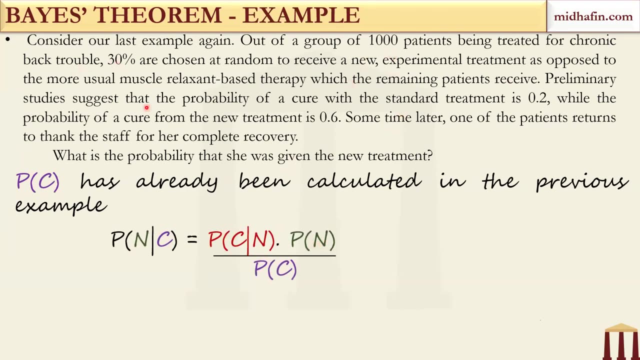 N is 0.6. from here Cure from the new treatment is 0.6.. Okay, And we know that P N was 0.3. That is also given 30% was chosen and done, Okay, So this. 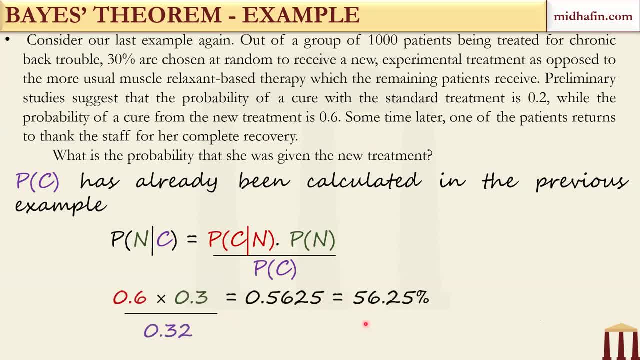 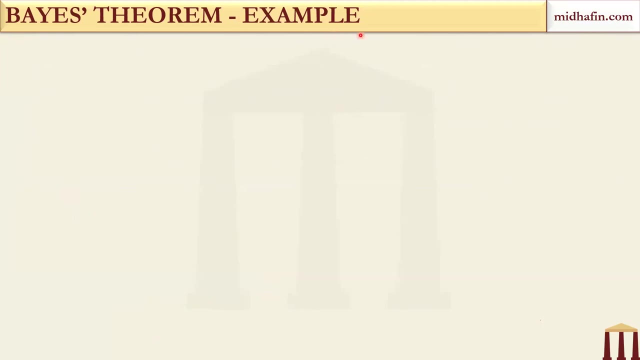 is how we calculate. So, given that the patient was cured, the probability that she was given the new treatment is 56.25%. Now let us solve the same question using three diagrams. So how to start? See, although tree diagram seems quite simple, and most of you are already. 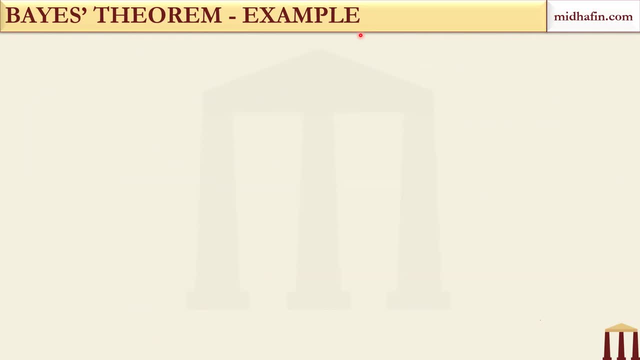 comfortable with tree diagram, But still, how do you start with the branch of the tree, the first branch of the tree? Do you start with cure or not cure, Or do you start with new treatment and usual treatment? Because there are two options. Either you can start. 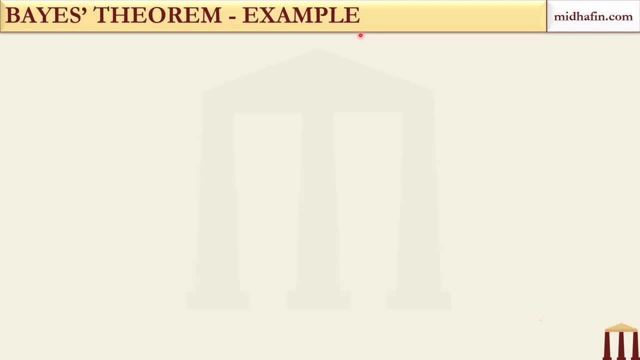 with cure, not cure. Those can be your first. you know two segments of the tree, the first branch. Or you can start with new treatment, usual treatment. So in that case, how do you decide? Because see, when you solve these questions, it becomes quite obvious to you, don't think? 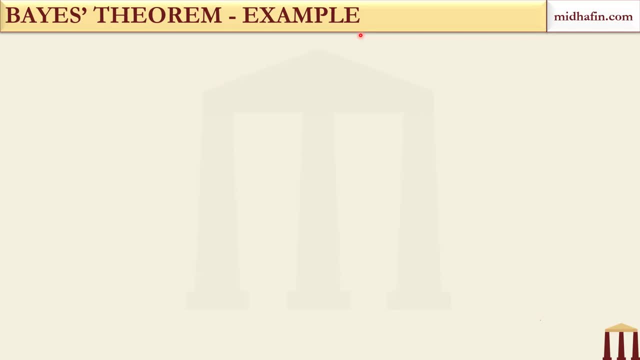 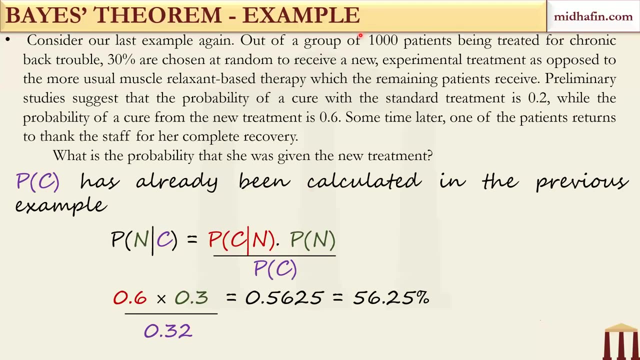 about these things in detail. What if I had done the opposite? What would have happened? You would never have been able to solve the question if the start was wrong. So in the beginning you always start with the information that is provided in the first place, So chronological. 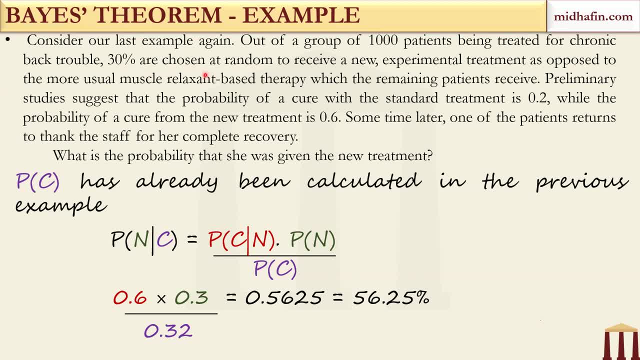 order what is happening. See first the patients are being given the treatment. Cure is what? Cure is an outcome. Do you agree or not? Cure is an outcome of the treatments, Yes or no? So first you will plot the outcomes in the tree, or first you. 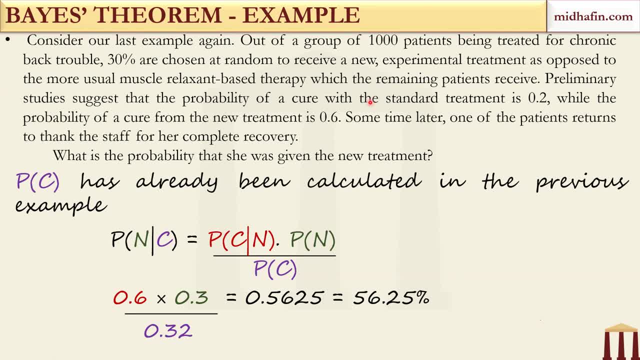 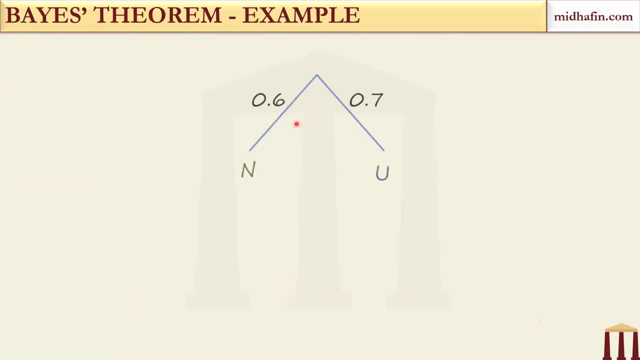 will plot the correct sequence First. you will plot what is happening, Okay. What kind of treatment is being given? So treatment first or outcome first? Tell me: Treatment first or outcome first in the tree. Very good. Treatment first, Okay. So new treatment or? 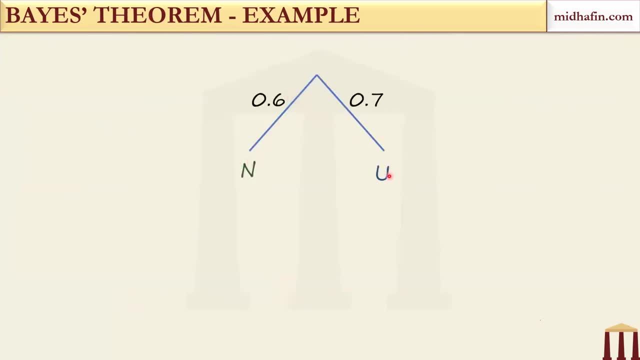 So, new treatment, usual treatment? okay, Again, there is a typo, there is a small typo. What was the probability of new treatment? 0.3, correct, So 0.3, 0.7.. Now, under the new treatment, also, what was the probability of getting cured? 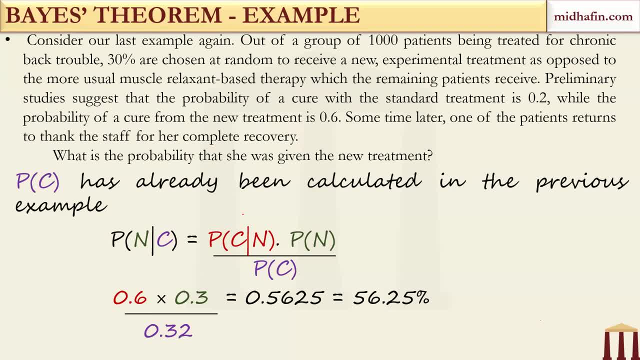 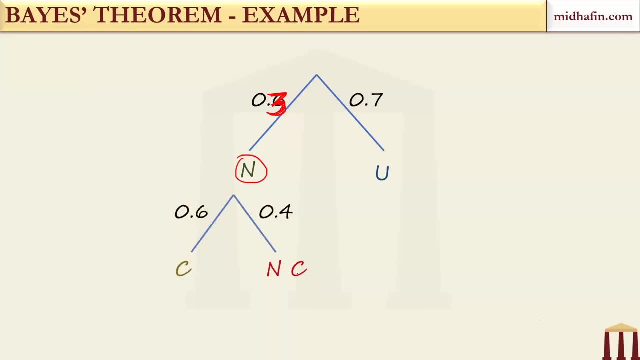 Given the patient was having new treatment, tell me, let us go back. If the patient is having new treatment, what was the probability of getting cured? Perfect, 60%. So let us go to the tree now. This is under N. we will have now two more branches: cure or not cure. 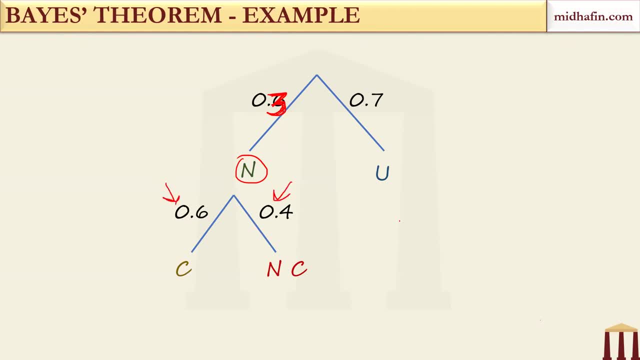 60% probability of being cured. 40% probability of being not cured. Similarly, can you tell me, under usual we will have again cure and not cure. What was the probability of cure under usual? What was the probability of cure under usual? 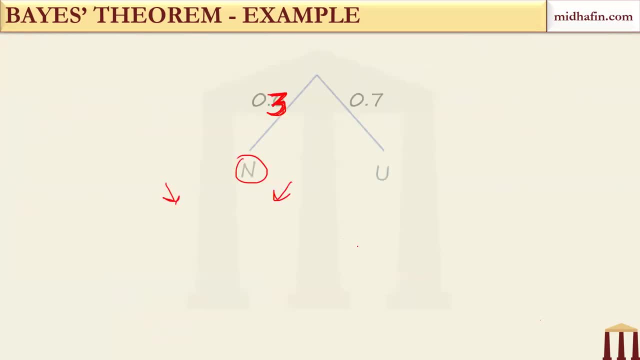 Perfect: 20%. So if 20% is the probability of getting cured, it means 80% is the probability of not getting cured in usual. Is the tree clear? Is the tree clear to everyone? Is there any doubt? You can ask immediately, because this is the critical part, I believe. 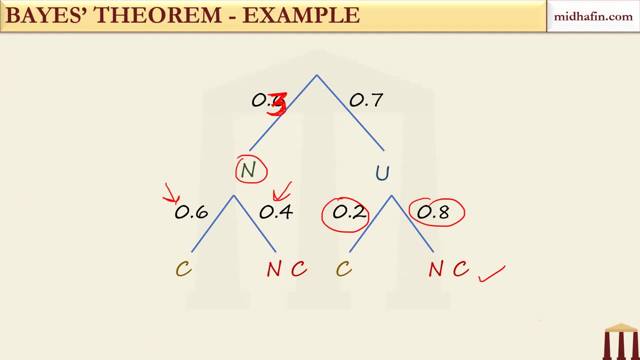 Okay, fine, So now there are two options. See what is the event now which has happened. Finally, yes, Rohit, I am repeating. So I said that you start with the Treatment first, You don't start with the outcome. 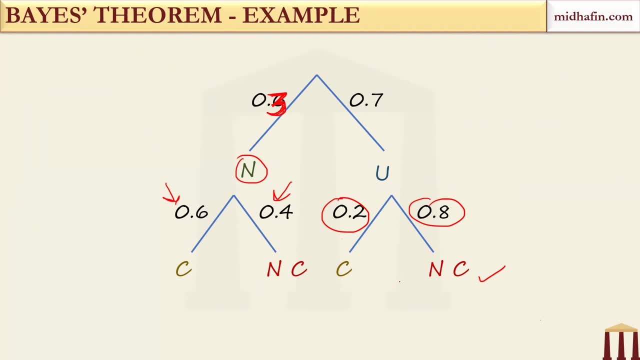 So there are two possible treatments. There are two possible treatments: New treatment or usual treatment. 30% or 70% Clear- First part is clear Rohit. Then, under new treatment, there are two possibilities If you get the new treatment. 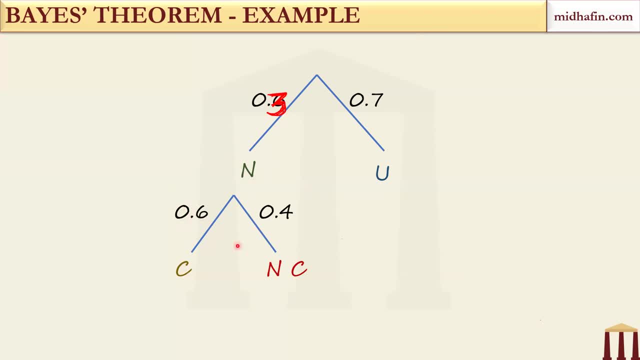 Either the patient can be cured with a 60% probability or the patient will not be cured with a 40% probability. Similarly, for usual treatment, the patient will be cured with a 20% probability. The patient will not be cured with a 80% probability. 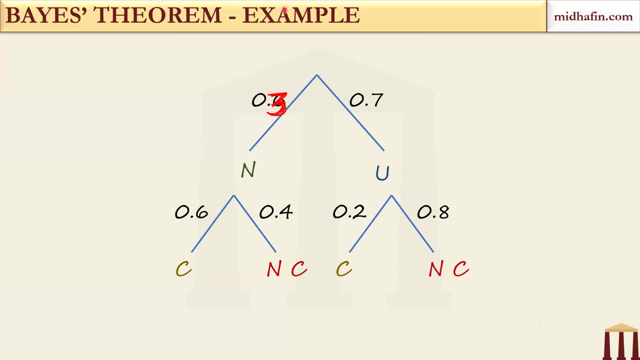 That is the tree. Is the tree clear, Rohit? no, Okay, great. Now it is given that the patient comes and thanks for her recovery. So it means that the patient has been cured. So we have to reach cured now. 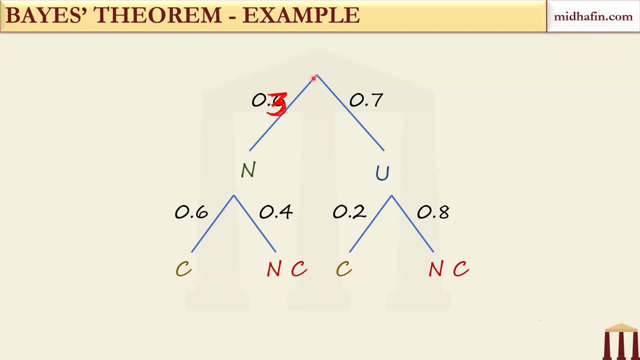 We have to reach C. Starting from the top, we have to reach C. How many routes are there, How many possible pathways you can see from top if you have to reach C? There are two Cs, So there are two paths right. 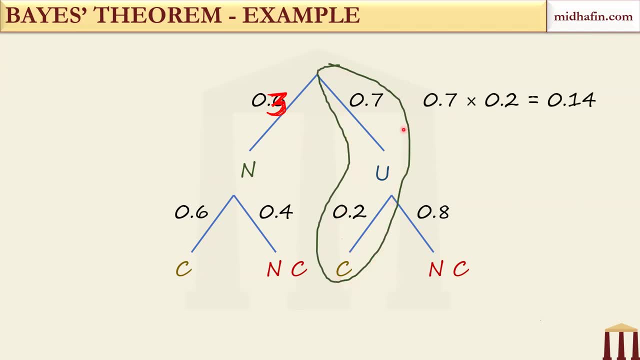 One is this path. Do you agree? this is one path To reach cure, Agreed or not? Okay, So you simply multiply the probabilities 0.7 times 0.2.. So the probability of reaching cure through this path is 0.14, 14%. 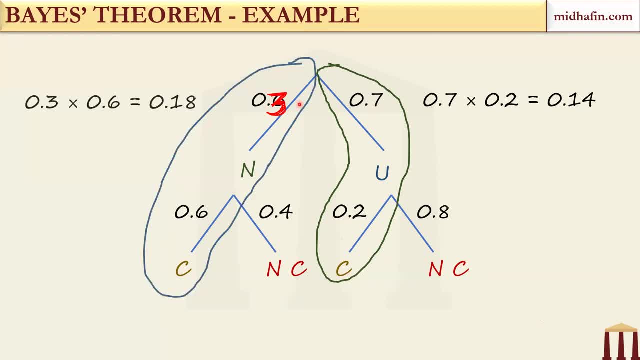 There is another path. right, This is the other path. Okay, The probability of reaching cure through this path is 18%. Okay, So what is the total probability of being cured? Simply 18 plus 14, which is 32%. 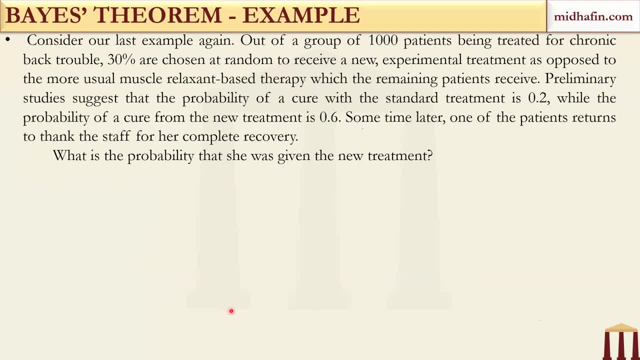 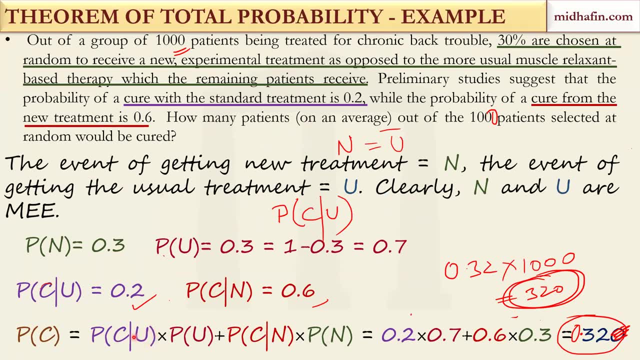 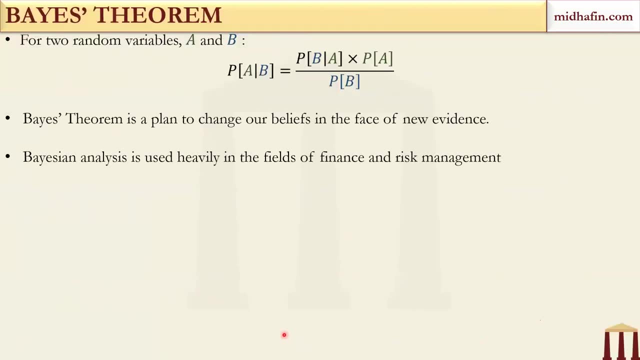 And that is how you visualize this formula. So the first part Was actually the reaching cure from one of the paths, reaching cure from the other path. This is actually the formula, also The formula and the tree. they are conveying the same thing in slightly different ways. 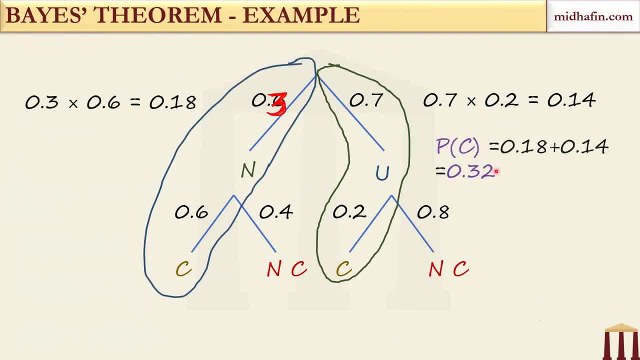 That's it Okay. So is it clear. How do you calculate the probability of a cure to T-diagram? So which one will you use in the exam? Tree or formula Tree or formula? What will be your formula? 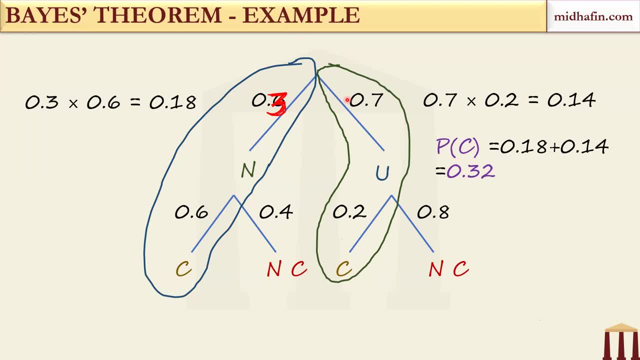 That's great. Okay, Very good. Okay, So do whatever you want. Okay, Fine, That's one very nice tree. So yeah, Okay, Great. So then the next part is the same. Then you just apply the Bayes theorem formula and you get 56.25.. 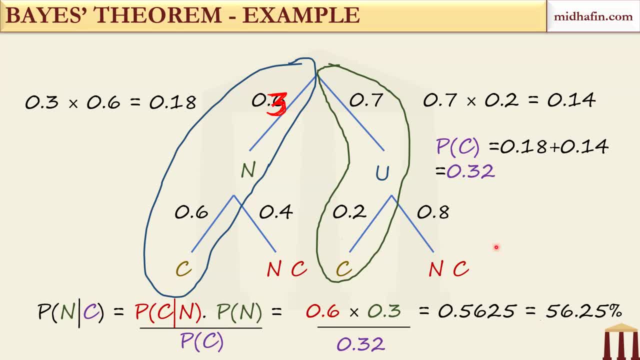 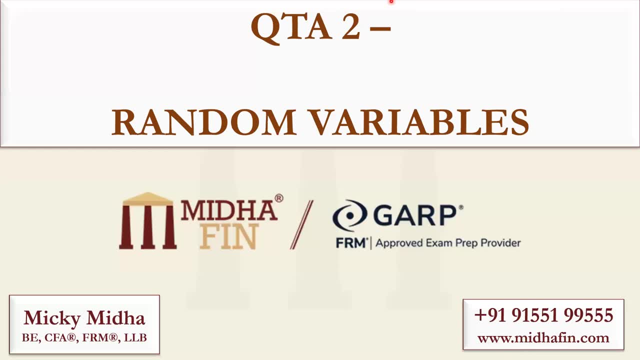 Okay, Fine, So that is it for the first chapter. Let's go to the second chapter and we'll just take a five-minute break over here, Only for five minutes, Okay, So we'll have four breaks in total today. 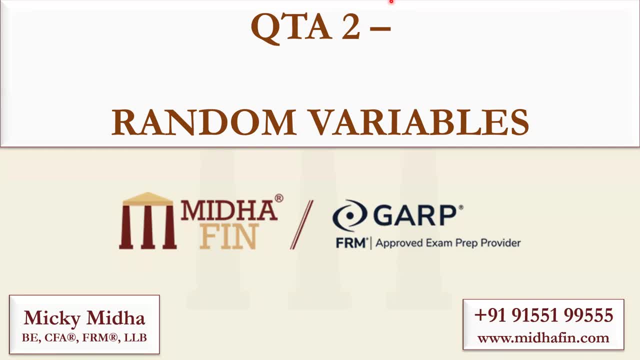 There will be short breaks between chapters- five-five minutes- And then there will be 15-minute break after we complete every three chapters. After every three chapters, there will be 15 minutes. So right now we'll just take a five-minute break. 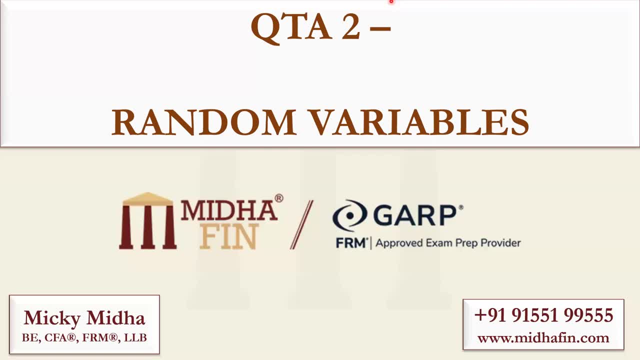 So please be back in five minutes. We'll start at 12.16 pm IST. Thank you, Twelve chapters puja will be covered today. Okay, Please be back in five minutes And those who will be watching the recordings of this video, they can just fast-forward it. 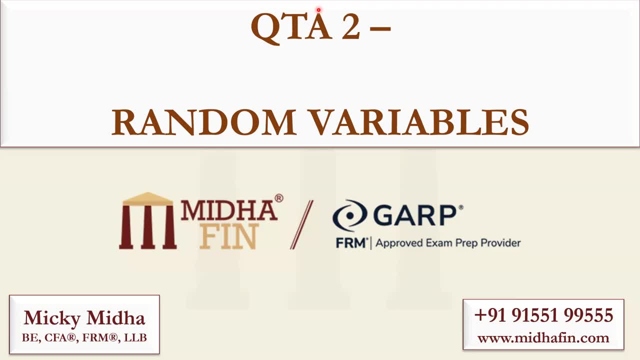 You know you can skip the next five minutes, the break part. They can check when the audio resumes, Because I'll not pause the recording. I don't want to miss resuming the recording or any problem, I don't want to have. 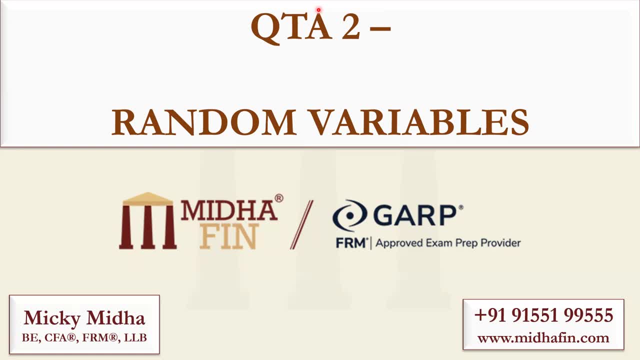 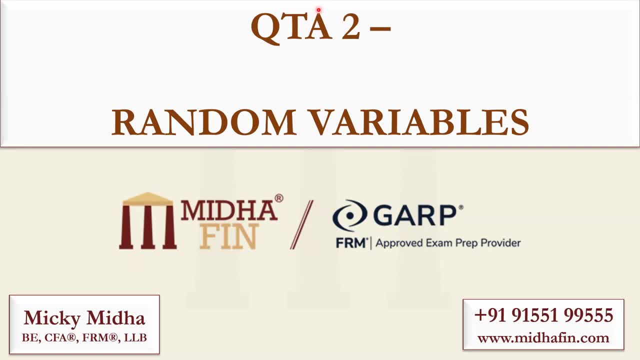 Thank you. Okay, Let's resume. Yes, Satish is asking: can we get access? Yes, definitely, As I mentioned that recordings will be made available to all of you In the LMS only it will be there. 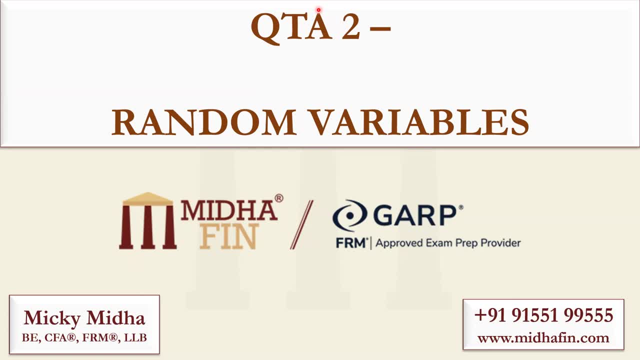 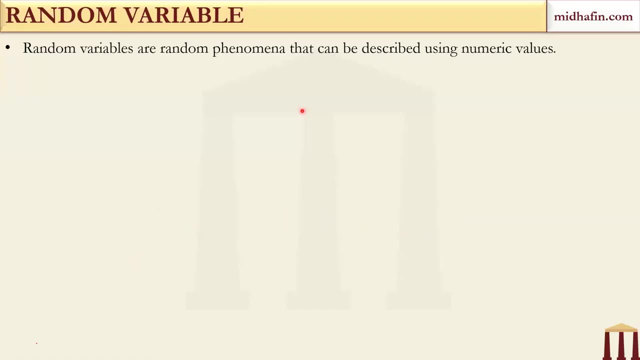 And probably, if required, we can also put it on YouTube. We'll see about that And you'll get access to recordings. definitely, Okay, And most probably this will be put on YouTube as well. Okay, Let's continue with random variables. 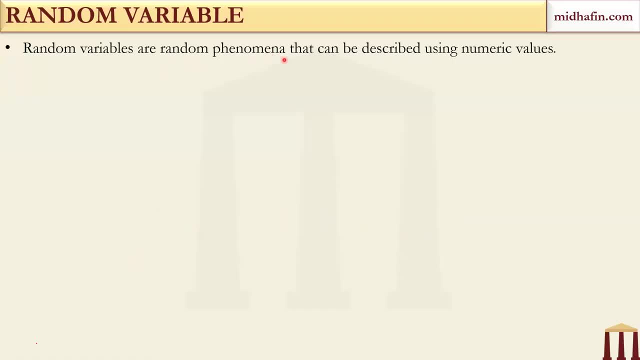 Now, random variables are random phenomena That can be described using a numeric values. So examples: of course we can have a return on a portfolio of stocks, let's say, or default on a corporate bond. Now the set of values that a random variable may take is called a support of the function. 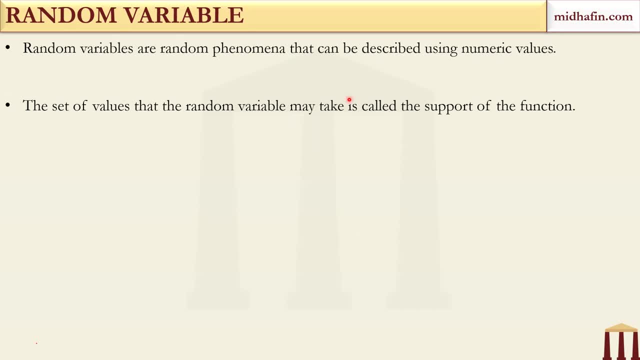 Yes, yes, As I mentioned at the beginning only that the PDF or version of all these slides that we are giving you right now, the PDF version of these slides, will be shared by the LMS directly. Okay, And if the video is put up on YouTube, then probably we might also have a link so that you can download it directly from the website as well. 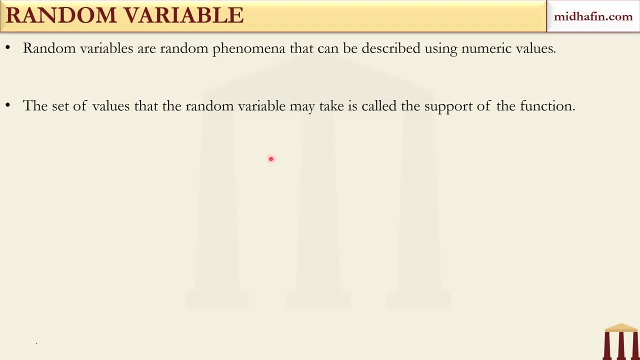 Okay, Fine, So what are the types? There are univariate random variables. You can have bivariate random variables, Okay, And you can have multivariate random variables. We'll discuss about these in detail. And univariate: they are of two types. 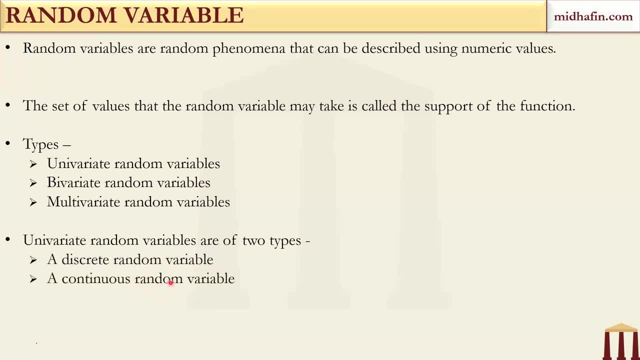 We can have discrete and we can have continuous. We can have continuous random variables. Remember that the key properties of discrete and continuous random variables are identical. And again, I'm repeating: See these things that we discuss in the videos. we discuss in great detail. 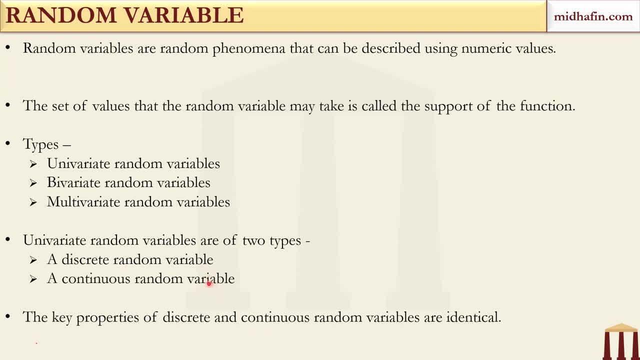 Discrete, continuous, the introduction part also. You know countably, infinitely many. What is the distinction between discrete and continuous? Discrete does not mean that only finite number of outcomes will be there. It can be countably infinitely many also. 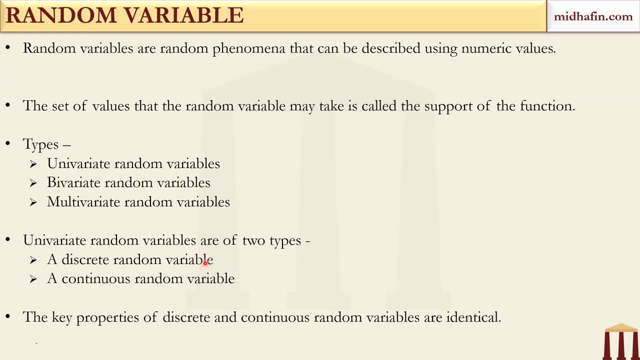 All these things are there But because of lack of time it is just not possible to discuss everything in the crash course. But The good news again, as I said, that since you get the PDFs and the recording, the good news is that the structure that has been prepared. 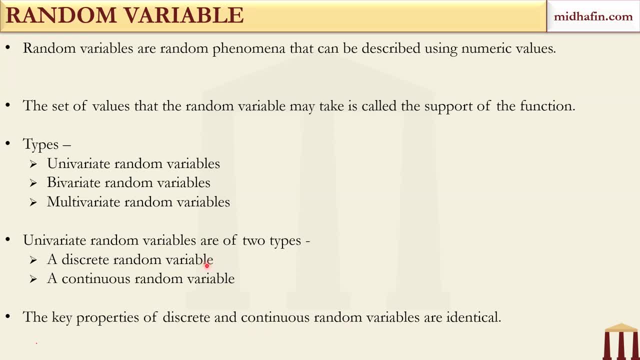 you know, when you go through the PDFs, the details that we have omitted. you know you can be almost 90% sure that they are not going to be asked in the exam. Okay, Those are for detailed explanations, for understanding purpose. 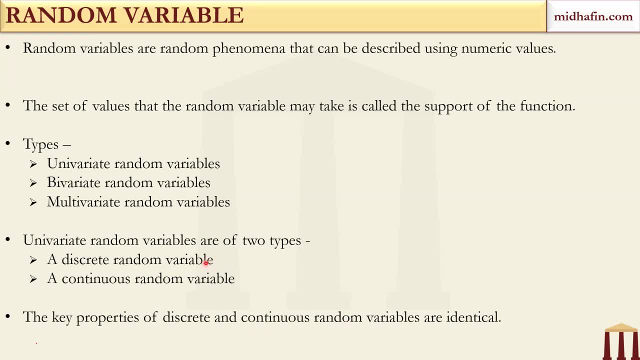 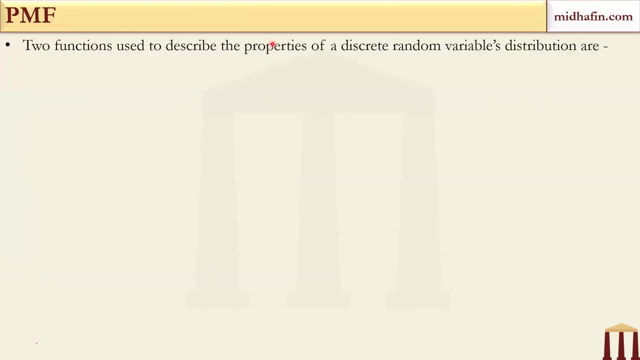 So that is why we have omitted those stuff, So there is no need to worry that you are going to miss something which is very, very important. Okay, Now PMF Probability Mass Function. Yes, Linio has mentioned that. please slow down a little bit. 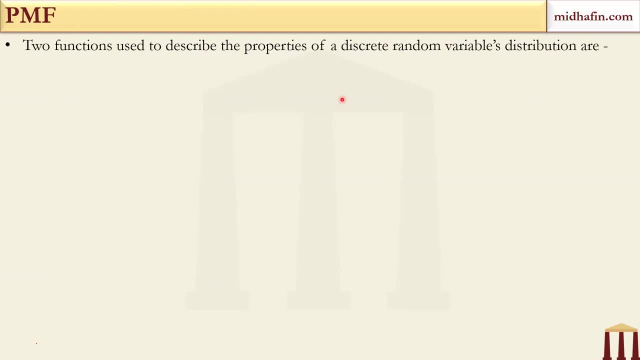 I think you are going too fast. See, I totally get your point, Linio, that I am going too fast. And see, the problem is that we have to cover 15 chapters. are there in points? Out of that, we have to cover 12.. 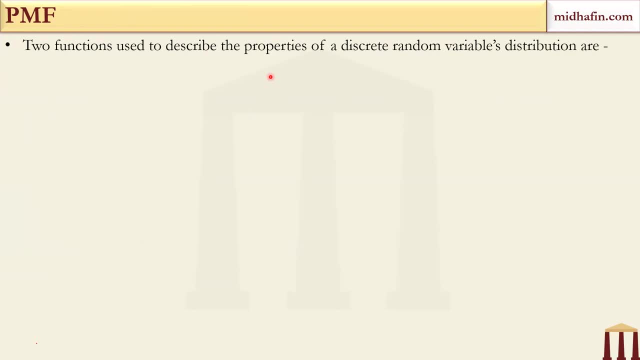 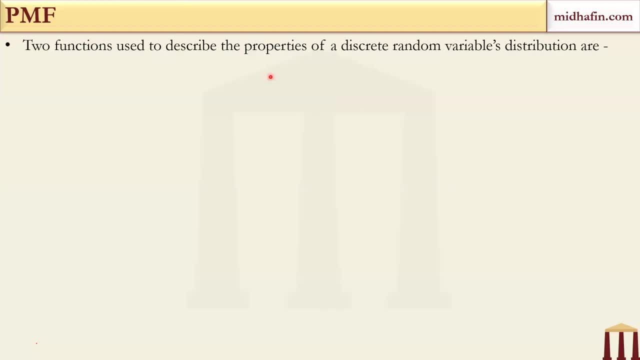 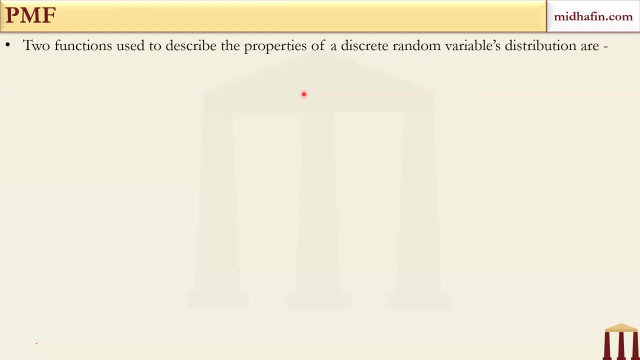 If suppose there are a few points which you are not able to understand, let's say, when I am going quickly, then you always have the pdf and the lecture notes for revision got it, so go through that part so i'll see all of the other candidates they are mentioning. speed is fine and everyone is. 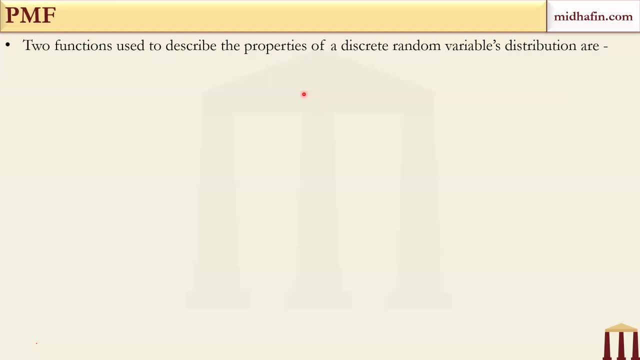 mentioned because it's a crash course. right, crash course means speed has to be there, so go through the recordings and the pdfs quickly. fine, and apologies for any inconvenience caused. so, but this is what we are trying, uh, our best, and if there is any problem, just let us know later after. 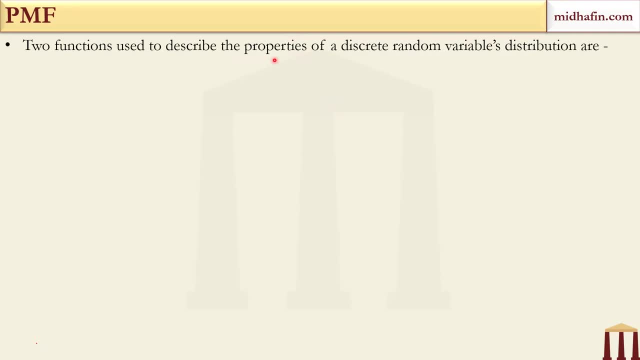 the class. maybe we can. we can uh have some extra doubt solving session also, which will have a for our candidates if possible. we'll see if we can include you in that. so two functions are used to describe the properties of discrete random variables distribution. they are pmf, which is 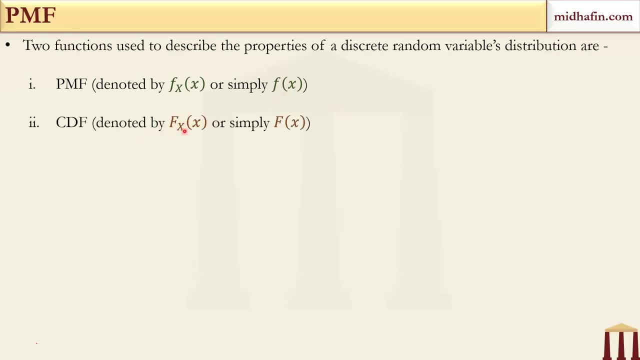 denoted by small fx, and cdf, which is denoted by capital fx. now, pmf is the probability that a random variable takes a certain value. there are two properties of pmf. just like probability, fx is greater than zero. the only difference is that now you are talking about functions. 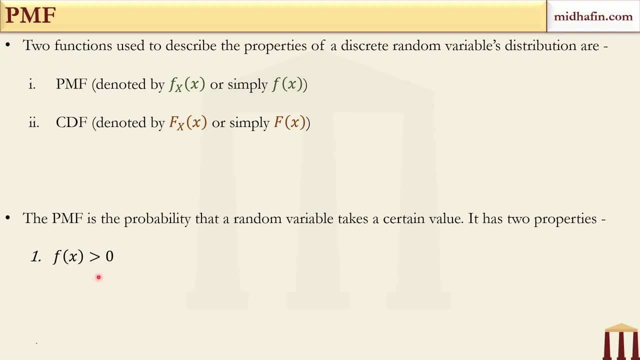 probability functions instead of core probabilities, so everything will be in functional notations. fx is greater than zero and summation fx equal to one. this is just like the property of probability, where the, the probability of all outcomes, has to be equal to one right. what is cdf? cdf is the sum. 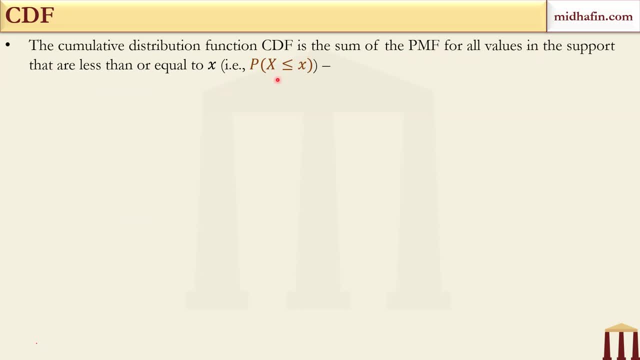 of all sum of the pmf for all values in the support that are less than or equal to x, less than or equal to x. okay, so starting from the minimum point up to that particular point, if you want to find out the probability, that is the cdf. so this is how cdf is calculated. summation. 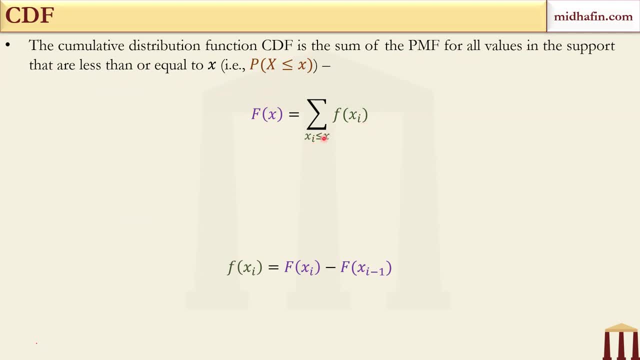 fxi, where xi is less than or equal to x. again, notations are not very important from the point of view of probability. so this is how cdf is calculated. so this is how cdf is calculated of the exam. concepts are important, so remember this point. you sum all the probabilities less. 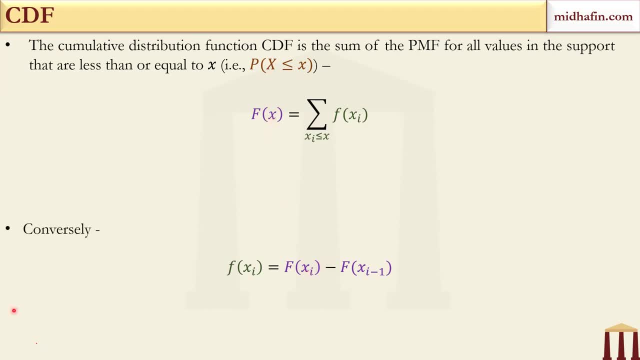 than or equal to a particular one. conversely, conversely, you can also calculate pmf. now, this is a very important point and this is quite analogous to the concept of you can say summation and differentials. okay, no, cdf is not the sample space. no, cdf is not the sample space. cdf is the 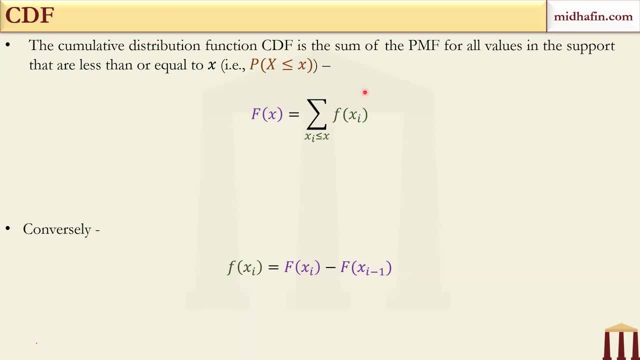 probability and in fact then we'll see examples later on- it will be quite clear to you. this is just the definition. cdf is the probability that the probability of observing a value x which is less than or equal to a particular value. that's it. so, for example, let's say, in this classroom there are 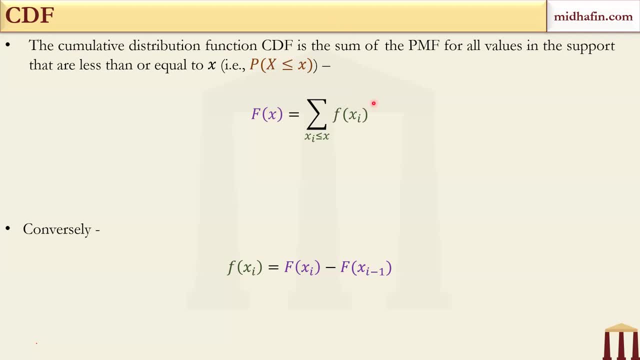 say 50 students, right, okay, and i take a surprise test and you get some random marks out of 100 and if i ask that, what is the probability of getting uh taking a randomly selecting a student who has got marks less than or equal to 70? understood so less than. 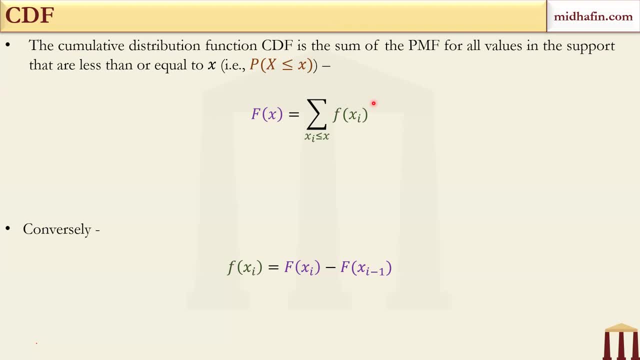 or equal to a particular value, starting from the minimum, if you want to find out the probability that is given by the cumulative distribution function, cdf. now, conversely, pmm is the difference of the cdfs for consecutive values in the support of x. remember that so if you actually do capital. 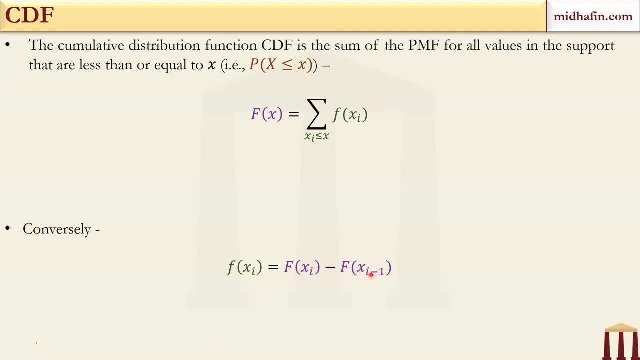 fx- i minus capital, f- x- i minus x. you can substitute this value and we will get some minus 1 consecutive values. if you subtract the CDF values for consecutive values of x in the support of x, of course, you get the PMF for that. a very, very important point. okay, this is as I was. 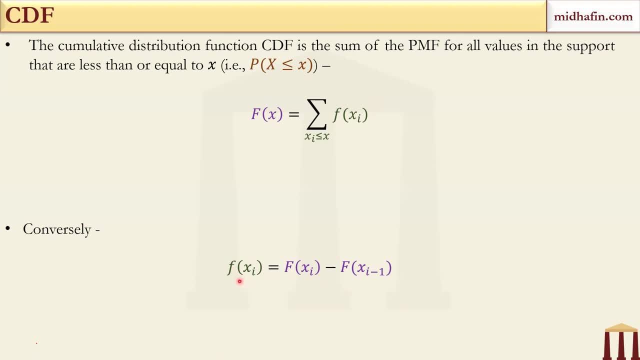 saying this is analogous to something that differentiation is the inverse of integration and inverse is the integration is the inverse of differentiation, something like that. but of course it is not in the course so we will not discuss in detail. but this part, the conceptual understanding, is important. okay, so when you sum all the PDF PMFs you get CDF. when you take a difference of 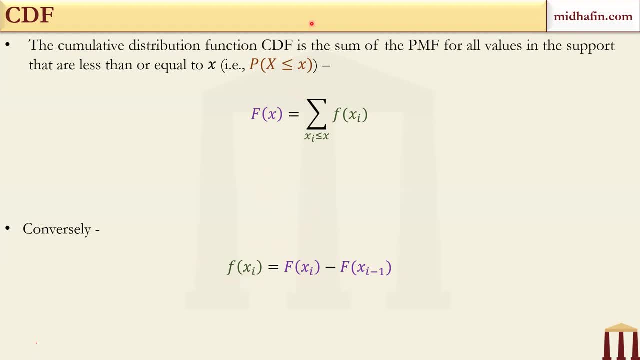 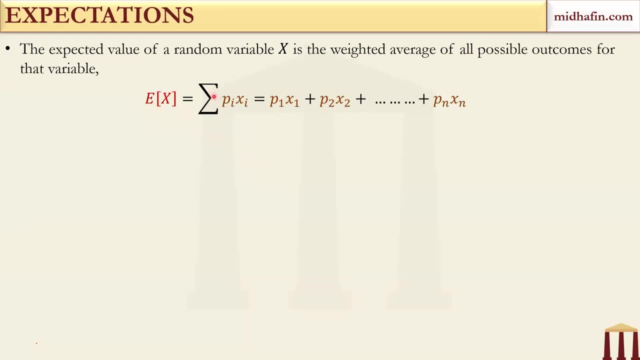 the CDFs, you get PMF. obviously, this is the inverse of the state, the above statement. okay, now what is the expected value? expected value of any random variable is equal to summation of PIXI, which is P1X1 plus P2X2 plus up to PNXA. now, expectation function of any 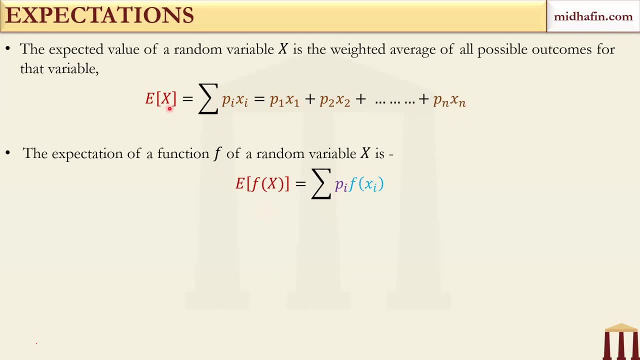 random variable is equal to summation of PIXI, which is P1X1 plus P2X2 plus up to PNXA variable is similarly see: either you can find out the expected value of X or you can find out the expected value of a function of this logic is same over there. you do summation PIXI over here. 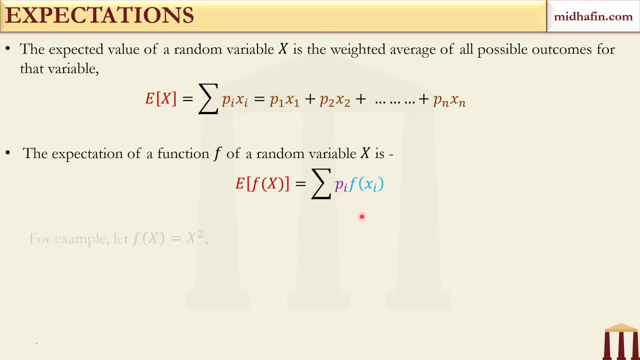 you do summation PIF of XI. so if suppose you have this example, suppose FX is equal to X square- then to find out the expected value of X square or FX which is X square, you will simply do PIXI, XI square, that's it, nothing else. okay? so PIXI square will be your expected value of FX. now these 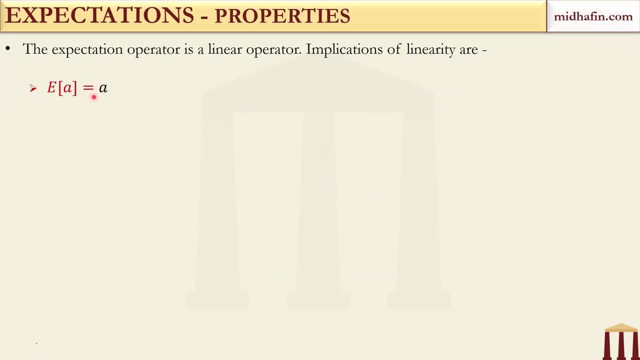 are the properties of expectation. it's a linear operator, so expected value of any constant is the constant itself. expected value of expected value is the expected value. an expected value of a random variable is always a constant, so expected value always gives you a constant, whether it is of a constant or a variable. so inside, the expected value of a variable is always a constant. 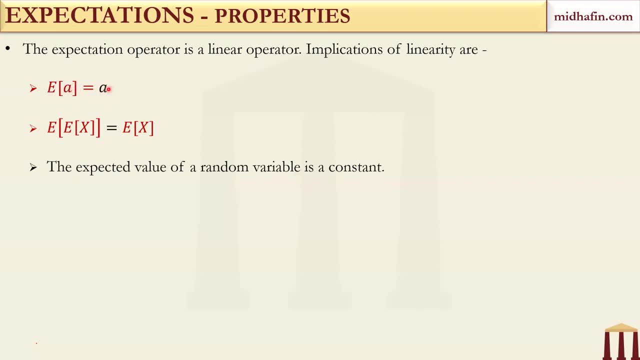 so for the expectations operator you might have a constant or variable, but on the right hand side you will always have a constant. and these things, they are testing the lot you know in the past few years, lot theoretical concept, theoretical ideas. they are testing a lot in the exam. now for non-. 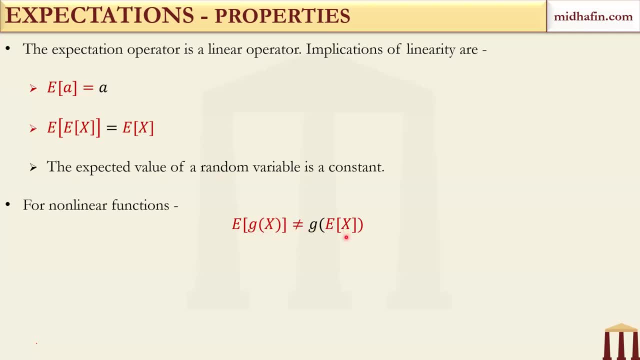 linear function, E of G is not equal to G of EX. so, for example, expected value of 1 over X is not the same as 1 over X, is not the same as 1 over EX. so all these are also called expectations over expected value of x, because 1 over x is not a linear function. If you draw the graph of 1 over 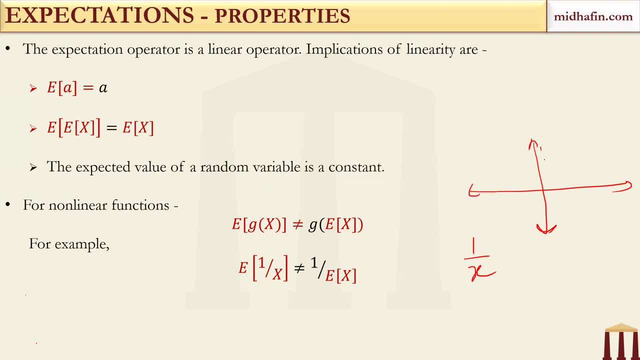 x. you can clearly check that in the first quadrant you did something like this and overhead you did something like this. So this is not a linear graph, right? So if the graph is not linear, then this property will not hold Expected value of gx, like 1 over x is not equal to 1 over. 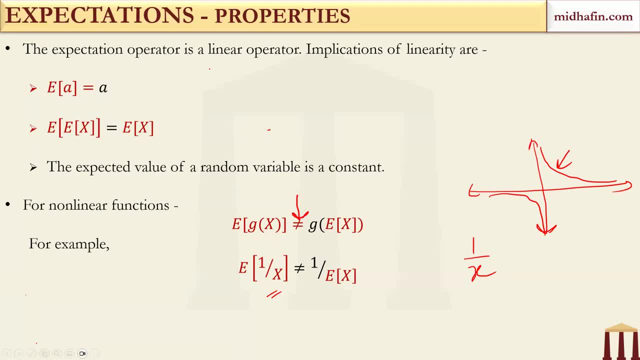 expected value of ex. okay, Now in the video, in the live classes we had a lot of examples, numerical examples, also a few examples to cover these things. but properties are important, So we'll just discuss the properties in the crash course. Expected value of cx is equal to c times. 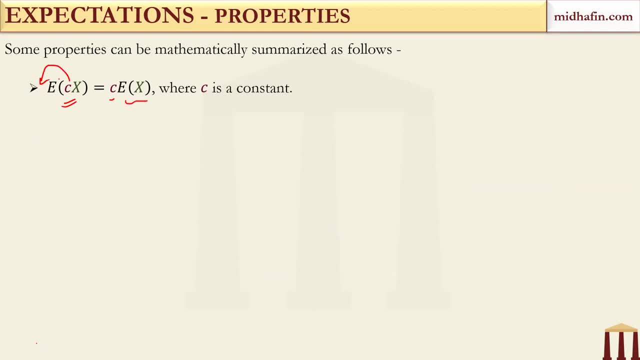 expected value of x. So c comes out okay. Expected value of x plus y is equal to expected value of x plus expected value of y. Expected value of cx plus a: again c comes out of the bracket and we know that expected value of a is nothing but a. 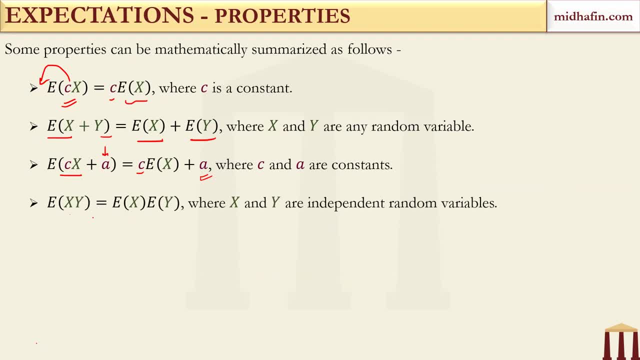 Expected value of xy. if x and y are independent, random variables, it is equal to ex times ey. This is just like probability for independent events Probability. the joint probability was nothing but pa times pv, right, So expectations operator also behaves something like that. 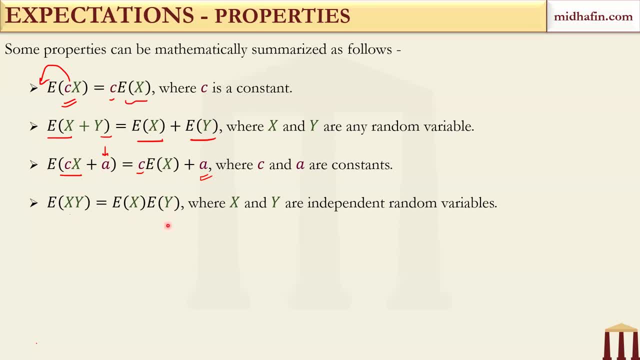 And, of course, if the events are not independent and the random variables x and y are not independent- over there we were talking about events, Over here we are talking about the random variables. So if they are not independent, then of course this equation will not be true. 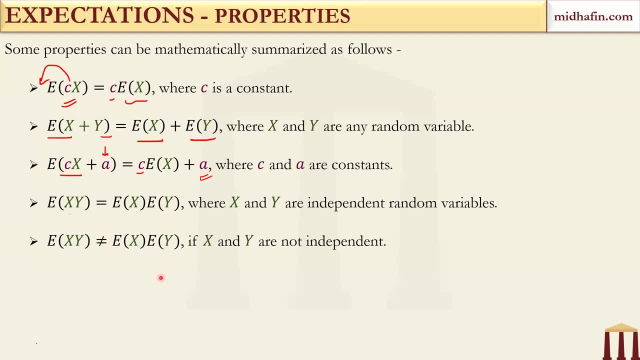 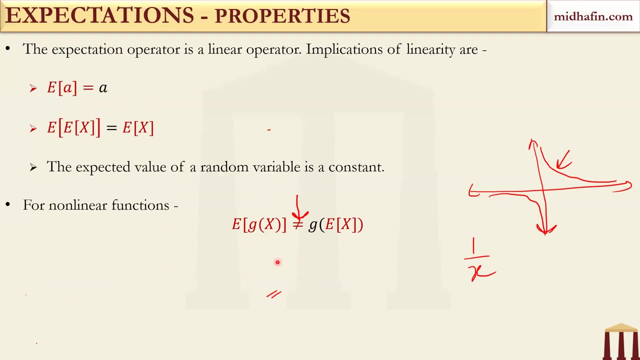 So it will not be equal to ex times ey. Also, remember that if you want to find out expected value of x square, you do not just square the expected value of x. This will not work out. You actually have to do this. You have to do summation of pi xi square. This is how you find. 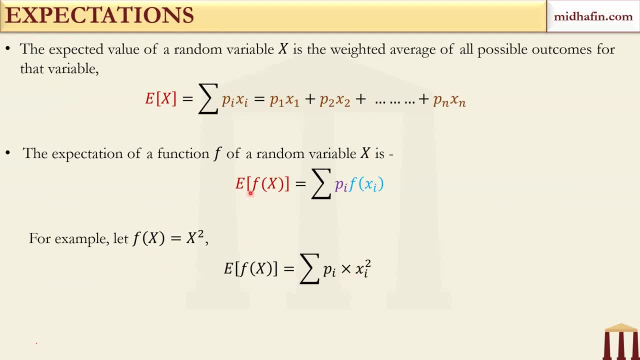 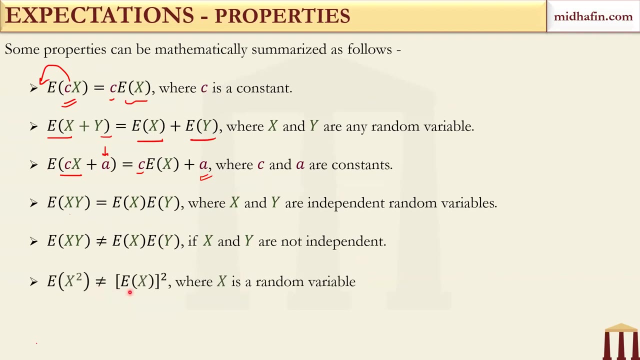 out expected value of x square. okay, You just do not square this, because this is different. This is summation pi xi. If you square this, you will get a different number. This will give you a different number. okay, So they are not the same. Expected value of x square is not equal to expected value of x. 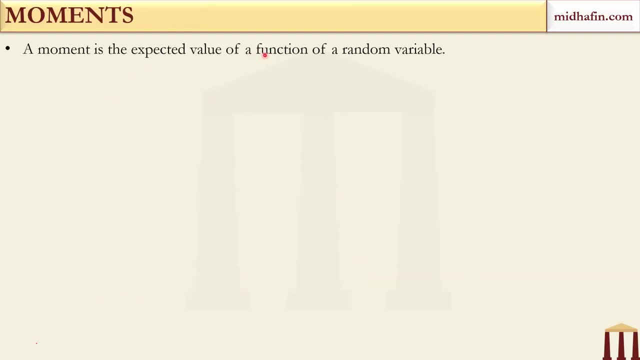 whole square. Now, what is a moment? Moment is the expected value of a function of a random variable. So there are four common moments. We have mean, variance, skewness and kurtosis. Mean is the first moment and is denoted as mu. 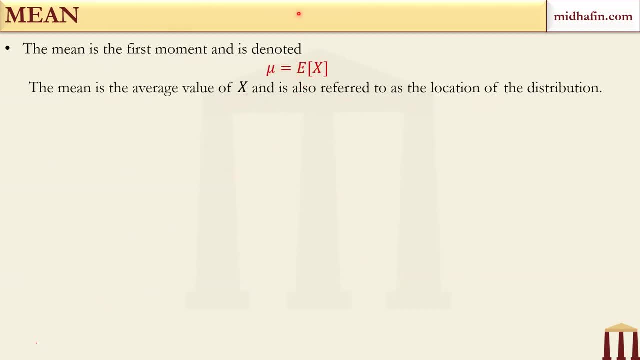 Is equal to ex, It is also the average value and it is also referred to as the location of the distribution. Then you have variance. Variance is the second moment. It is denoted by sigma square. Now, this is the formula, This is the formula of variance. So variance. 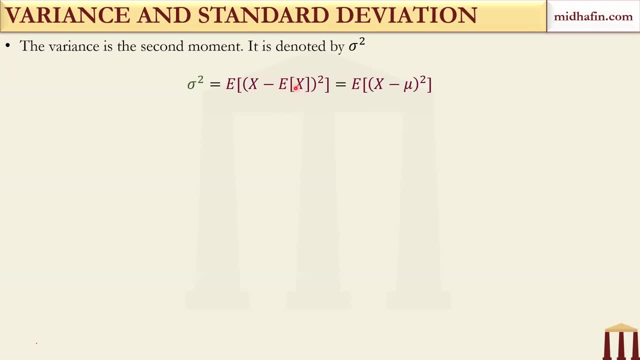 is measuring the dispersion around ex. That is why you can see, And again, the difference between central and non-central moment we are not going to discuss in the crash course. That is not very important, okay, from the exam perspective. So we are talking about. 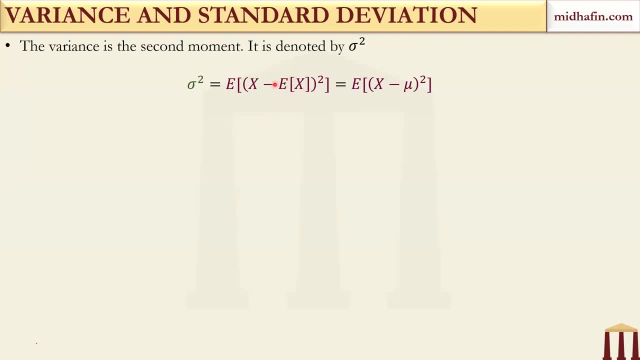 central moments right now. So you see, over here there are two formulas. actually This is the first version of the formula. So actually you take all the x's, you subtract the mean okay, and you take the square and you find out the expected value of that. And in some 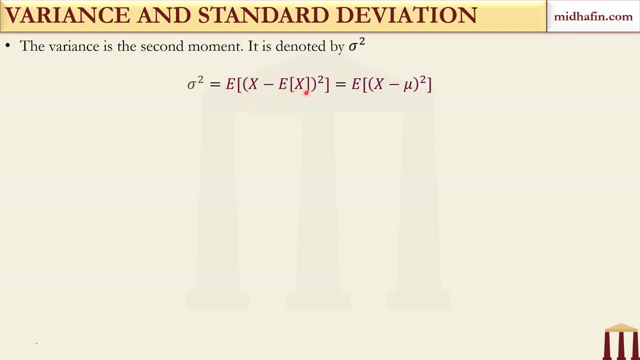 cases, you simply sum those xi minus ex values, whole square values, because the probabilities for all, the outcomes are same. But what is so important- and I keep saying this in the exam all the time, many a times in fact- is that whenever these kind of questions are given, they forget to pay attention to. 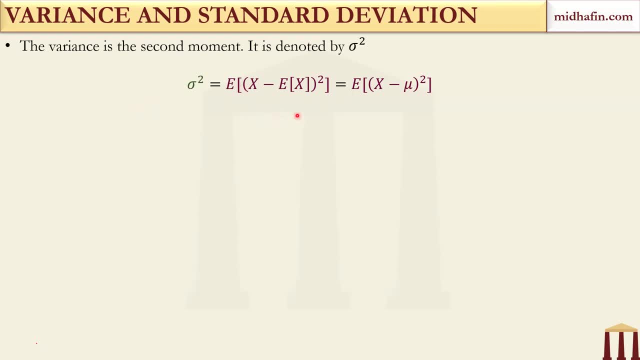 individual probabilities. Remember that. That is why I have not just divided it by n. You will divide it by n only when the probabilities are same, They are equally weighted. Something like that is given or no information is given. If probabilities are given explicitly, then 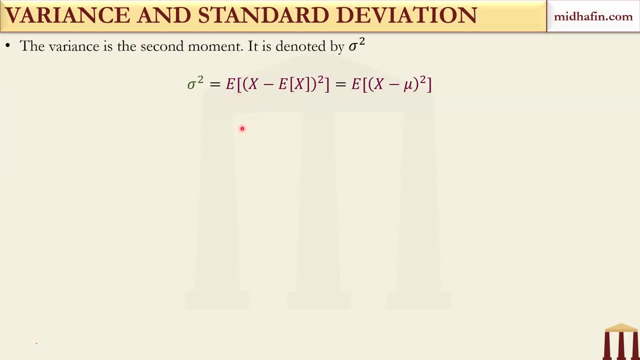 to find out the expected value. then there is another version of the formula. this version, Sigma square is equal to e x square minus e x whole square. in fact, okay, so this is actually e x whole square. this is a better way to write from the exam point of view. let's say three or four data points are given to. 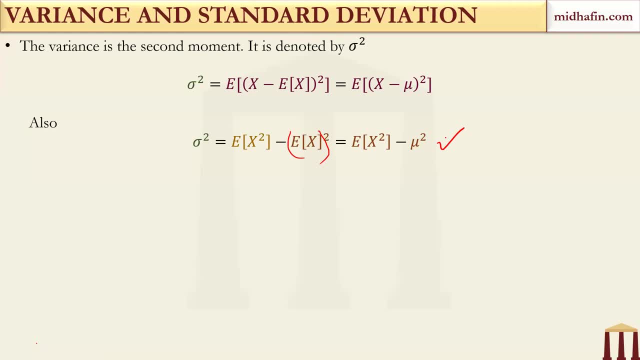 you. you should prefer this formula. this will be easier for calculation and I hope everyone knows how to calculate these values using the BA 2 plus calculator, because once you use the BA 2 plus calculator all these values become quite easy. so I'll just give you a quick heads up. there are two buttons in your 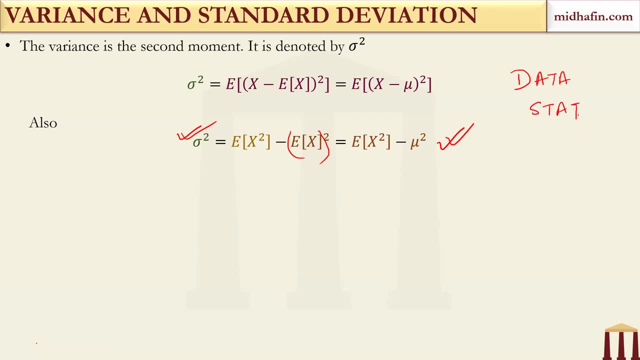 BA 2 plus calculator. one is data and one is stat. one is above, I think, seven, the other is above eight, if I'm not wrong correct. so if you have not learned the use of these buttons, do it today itself, because these buttons will help you calculate everything. 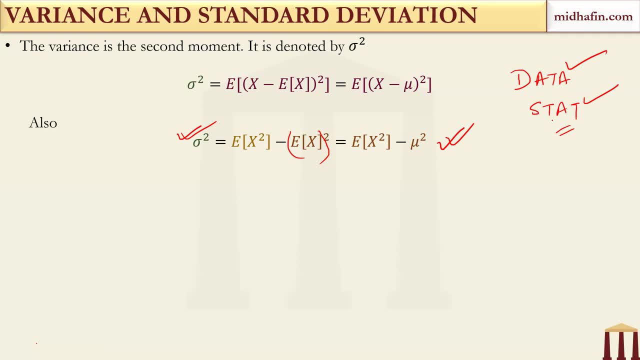 you know right, from mean variance, standard deviation, sample standard deviation, population standard deviation to even correlation, R square and everything okay. so learn data and stat button today itself. that is very important from the exam point of view. then, square root of variance is denoted by Sigma. it is known as the standard deviation. it is the measure of volatility. 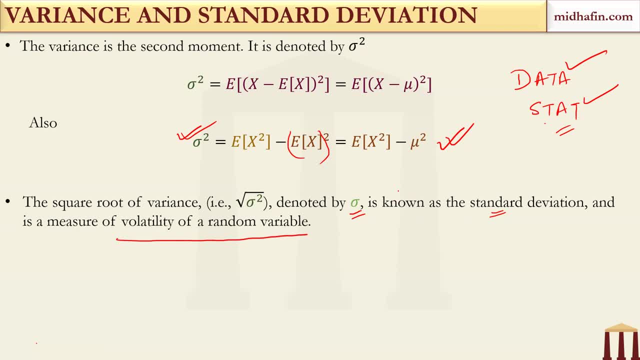 of a random variable. so Sigma square, the variance, is the measure of dispersion, how much spread the random variable is about its mean. now, one point which I want to highlight over here is this, because there is a mistake again: many uh books, third-party books, or even uh uh not frm related, only frm related, non-frm. 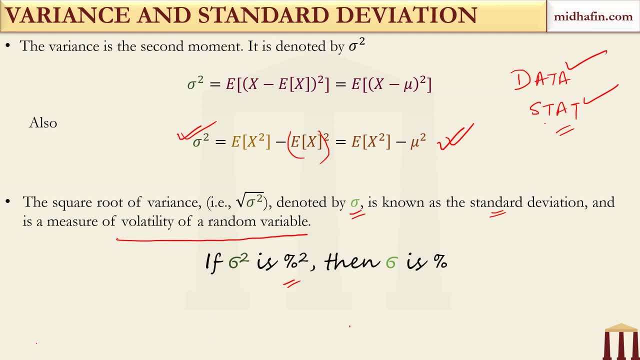 related books. they tend to make this mistake that when they give the value for variance, they give the value for variance in percentage. that is wrong, because if you are having expressing Sigma in percentage, the percentage is not a unit. also, okay for convenience, you can call it as a unit. just for convenience, for. 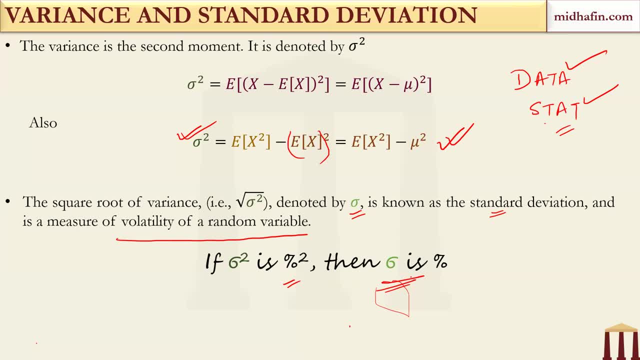 understanding purpose. but it is not. a unit is a way of expressing. you can either express in decimals or percentage, but you have to be very careful that standard deviation is in the same units as the original data. so if suppose you are talking about returns and returns are given in. 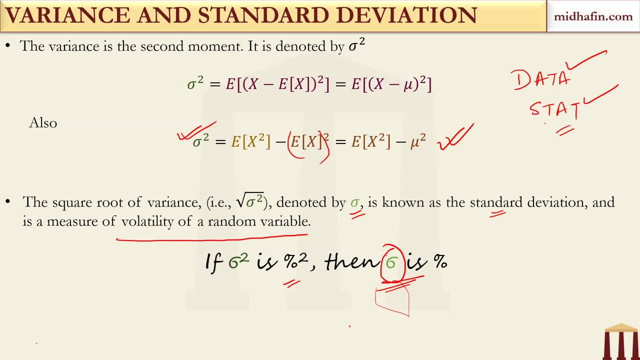 percentage, then standard deviation will also be represented in percentage. but can variance also be represented in percentage for that data? if I am already saying that variance is the square of standard deviation, should I also express variance in percentage? what do you think? is it correct? no, so variance. 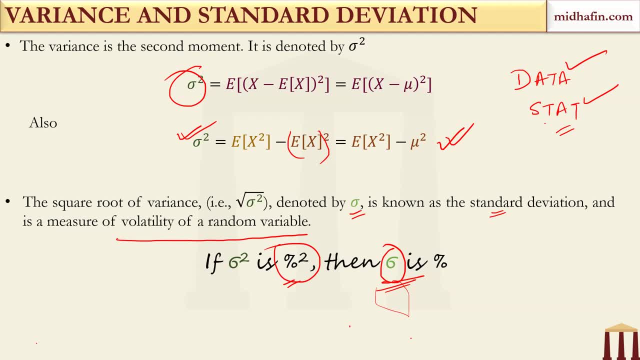 should always be expressed in percentage square. okay, so this is one mistake which you should not make. and the square root of percentage square is percentage, so everything becomes consistent. okay, if you are able to follow these conventions properly. now let's talk about skewness. skewness is the standardized third central moment now when 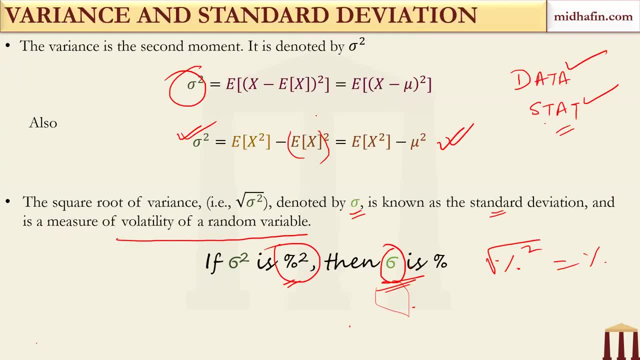 we say standardized. you might have noticed one thing over here. see, when I calculated variance, did I divide by Sigma square or any uh measure, any squared of something? no, it is not divided by Ex square or mu square or any square right, it is simply the spread about the mean. 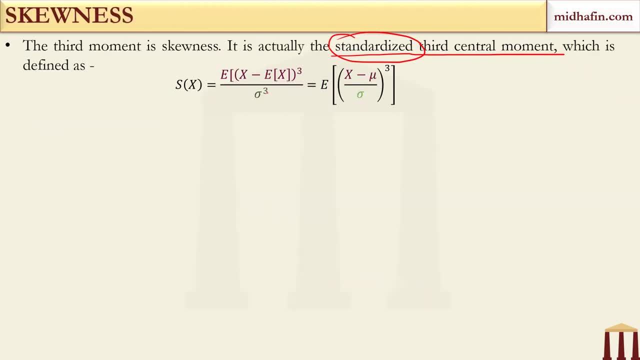 that's it. but skewness, when I define skewness is actually not the third central moment, it is the standardized third central. here also I have seen some candidates making this mistake. they'll say: okay, first moment is mean. second central moment is variance. third central moment is skewness. fourth, 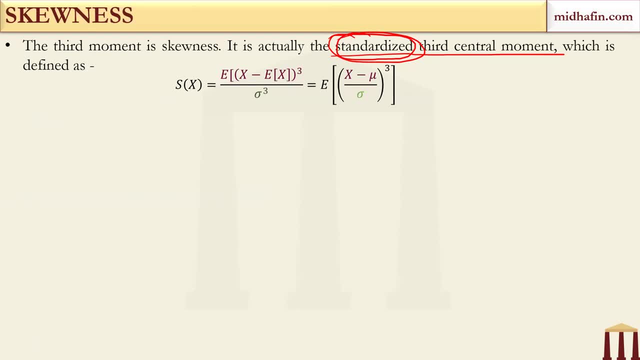 central moment is kurtosis. no, you are right up to point two, you are right up to variance, but you are wrong. after skewness: once you start with skewness, you are standardizing it by dividing it by Sigma Q. okay, so it is the standardized third central moment. 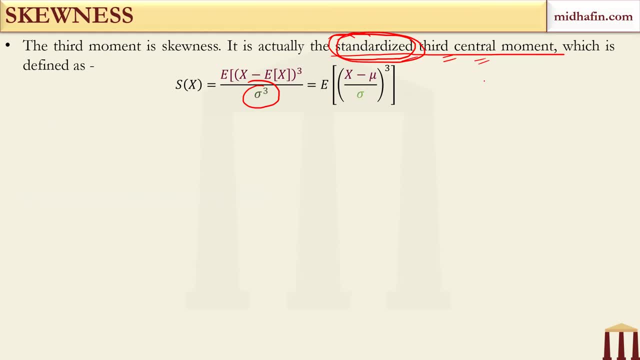 okay. but if you are asked, what is the third central? so third central moment is simply this: that's it got it. this is your third central moment. once you divide it by Sigma Q, you get the skewness. okay, because it is easy to deal with in terms of. 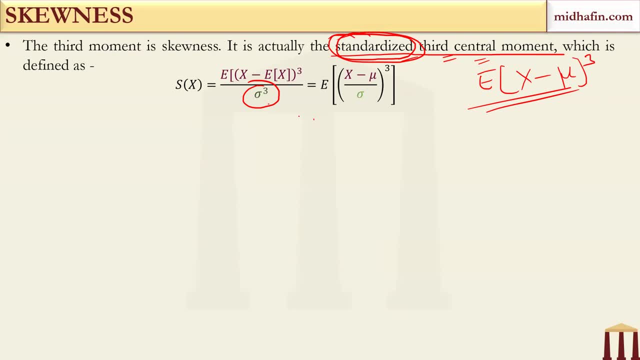 calculation and there are some other reasons also, some statistical properties also, which we will not discuss. so you can see that you can have positive skewness, you can have symmetrical no skew or you can have negative skew overhead. in the second diagram they are overlapped over each. 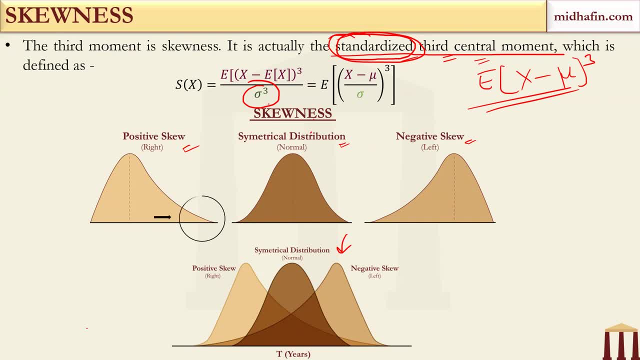 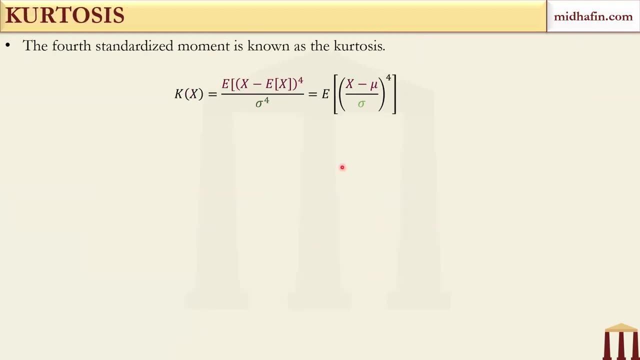 other, and the first one: it shows a longer right tail. so if the distribution is positively skewed, you will have a longer right tail. if the distribution is negatively skewed, you will have a longer left tail. okay, next let's come to kurtosis, kurtosis, whatever you want to call it. so kurtosis or kurtosis is the. 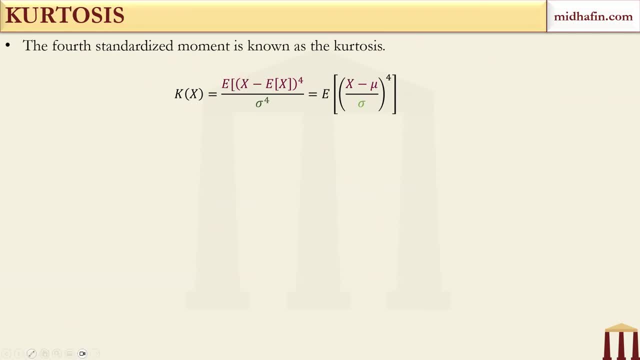 standardized fourth moment. again it will be central. the standardized fourth central moment. because why I'm saying central? because we are subtracting Ex all the time. so it is about the center, if suppose I take directly Ex to the power 4. When you are subtracting Ex all the time, you are taking central. okay, then you divide it by 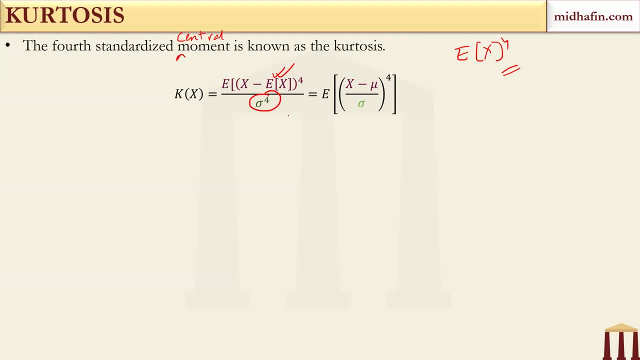 Sigma to the power 4, you get standardized fourth moment, standardized fourth central moment. this is kurtosis, now remember, and of course, distributions part we'll deal with later on. okay, what is a normal distribution? and all remember that kurtosis, for a normal distribution, there is something called. 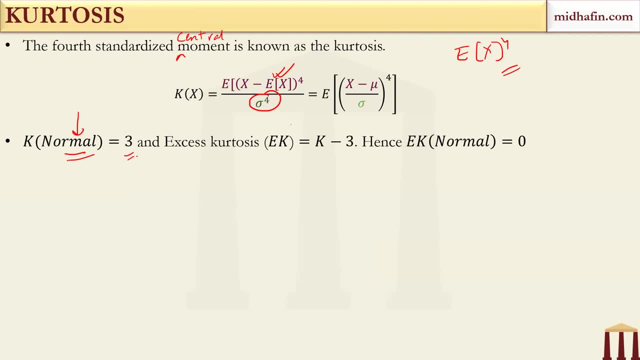 as a normal distribution, which is a very important distribution- is equal to three. Similarly for skewness. also for a normal distribution, there is no skewness, it is not skewed, skewness is zero. so for a normal distribution the kurtosis is three and excess kurtosis. we define it like this: K minus 3.. so it means for a normal distribution there. 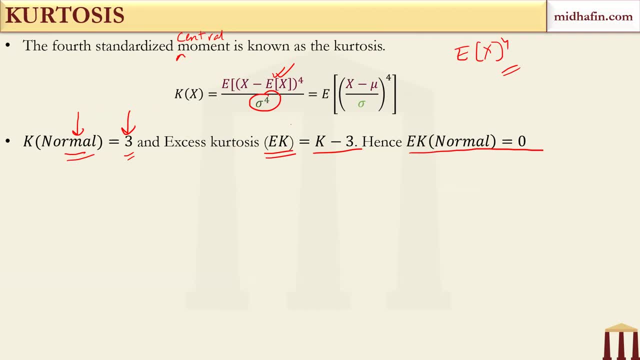 is no excess kurtosis. we standardize it. actually, we standardize it by subtracting it with okay. okay are usually heavy-tailed, So they have a lot of kurtosis. So kurtosis is basically just like. skewness was a measure of the degree of asymmetry. How much asymmetric. 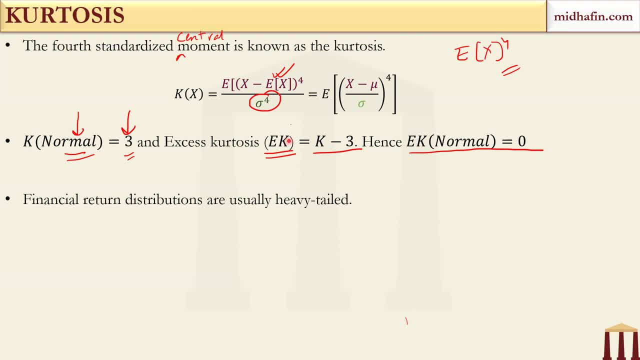 your distribution is. Kurtosis is a measure of how much thick the tails of your distribution are, How many large deviations you have from the mean. That is how kurtosis actually, that is how kurtosis should be interpreted- Got it? 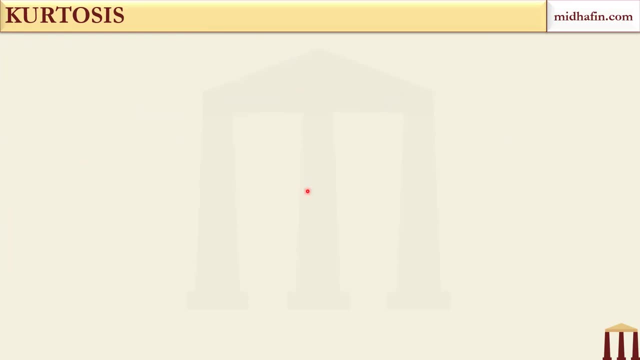 Okay, now this diagram, which, again, you will see a lot of mistakes in almost, I will say, more than 80 percent of the figure that you'll find everywhere FRM or non-FRM related books. First we will discuss the theory part. So for leptokurtosis, 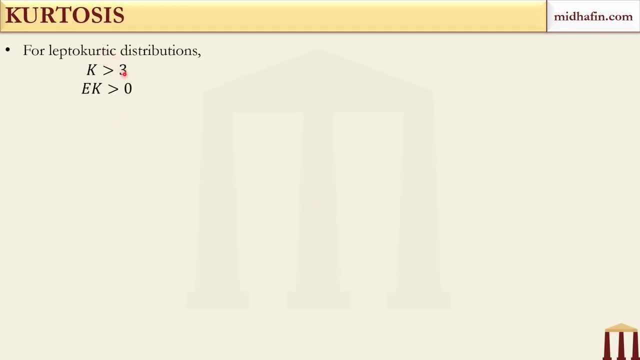 there are three kinds of distributions. There are leptokurtic distributions. For them k is greater than 3 and excess kurtosis is greater than 0. This is more peaked than the normative distribution and it is heavier tailed. So leptokurtic distributions, they are more peaked. 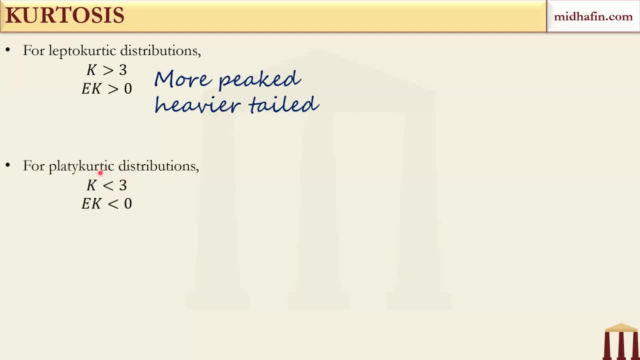 and heavier tailed Platykurtic distributions. they are having k less than 3.. So ek will be less than 0. So they are less peaked and lighter tailed Mesokurtic distributions. they are exactly having the kurtosis of 3 and excess kurtosis of 0. Now the diagram which 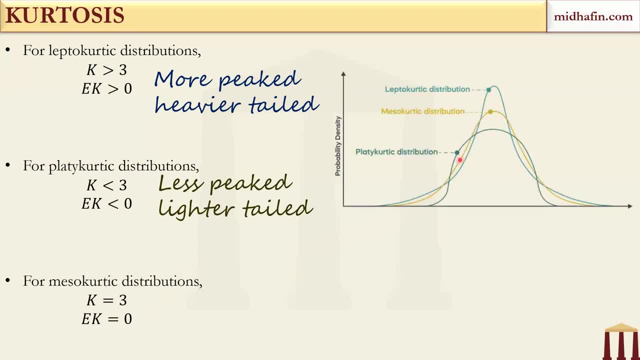 I am talking about, which you will find there is a lot of mistakes. this is the correct version of the diagram. See, it is very, very important to point out that in this diagram, in the central region and tails in the central region, so this central region and the tail region. 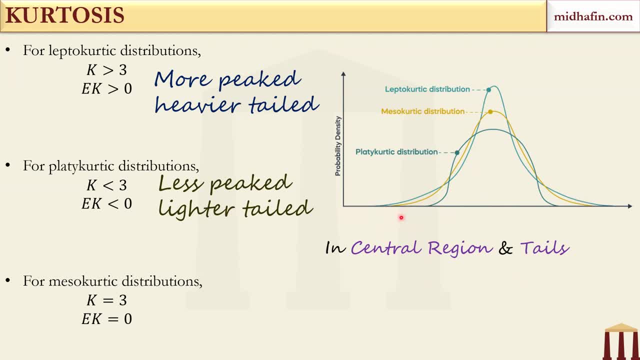 can you tell me which distribution is having the highest probability density- Quickly, Very good lepto- And which is having the most probability density? This is the minimum Minimum Platy. Correct, See, platy is minimum over here also. 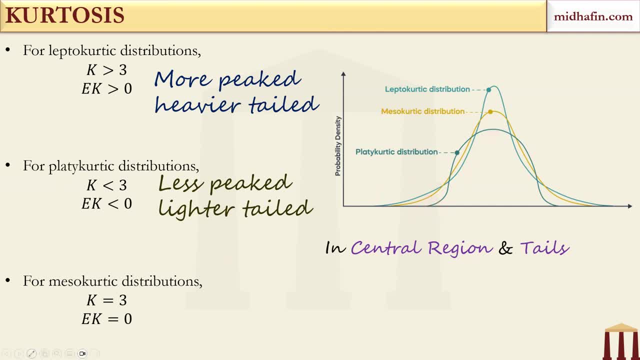 Platy is minimum over here also. So in the tails you can see these two paths. See the tails. This is the lowest correct And this is platy. That is why I say: see, this concept will only be clear if you look at the correct diagram. So this is the lowest correct And this is platy. 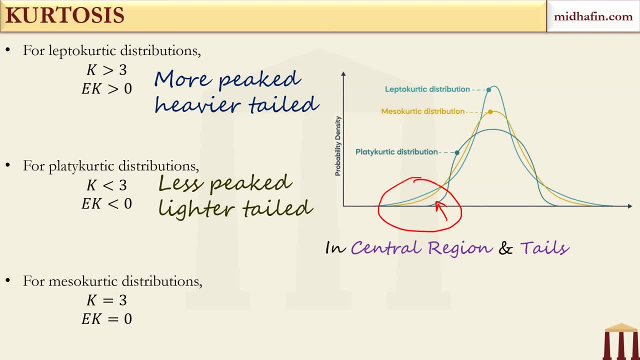 And most of the diagrams. you know the tail part. they completely ignore That which one is lowest and which one is highest. You can search on the internet also You will see you will get a lot of wrong diagrams. Platy-Kurtik is lower, both in the tails as well as center, So in the 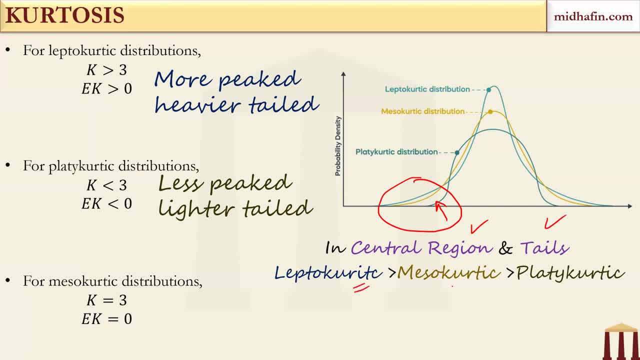 center, as well as tails. lepto is greater than meso, is greater than platy in terms of probability, density, function values, Got it? Is the diagram clear? Yes, Yes To everyone, because this is heavily tested in the exam. You know when they talk about kurtosis? 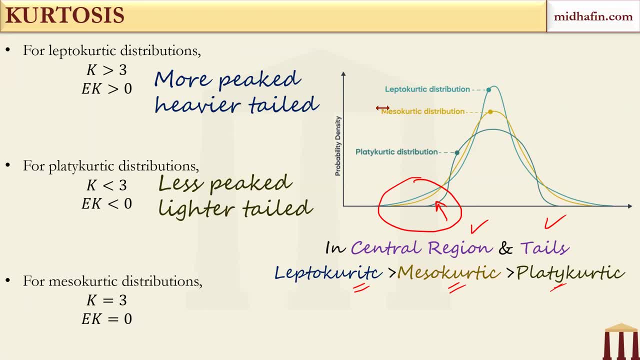 this is one of their favorite questions. Okay, So, central and tail, both the regions, Lepto greater than meso greater than platy, But what about intermediate region? What about the intermediate region? Which one is highest? This is the intermediate region. 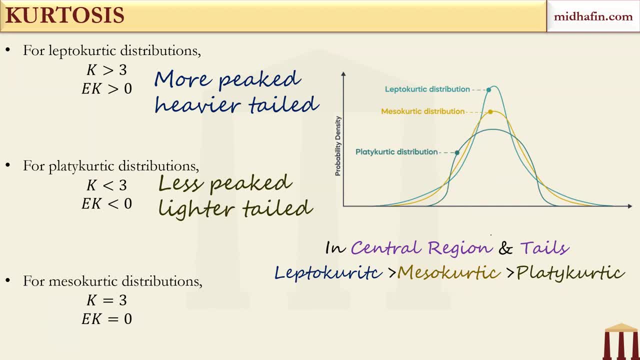 So in fact I should do one thing. I should do proper color coding: Central and tails we have given in purple. So let me just use purple for central and tail, Okay, And let me use another color for intermediate Platy. Very good. So in intermediate region, red one. 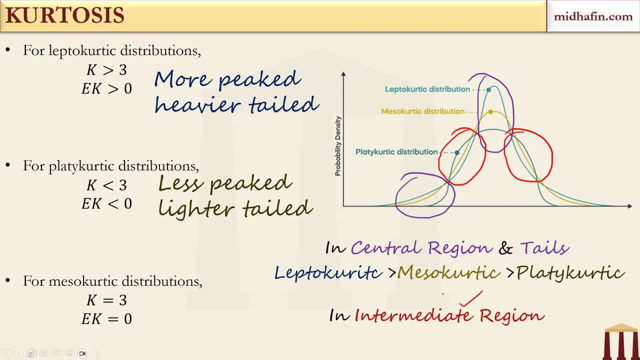 This is red, intermediate-intermediate. Okay, Maroon, Not red Maroon region. Okay, Platy is greater than meso is greater than lepto. This distinction should be very, very clear. Okay, So is it clear to everyone, Any doubt? 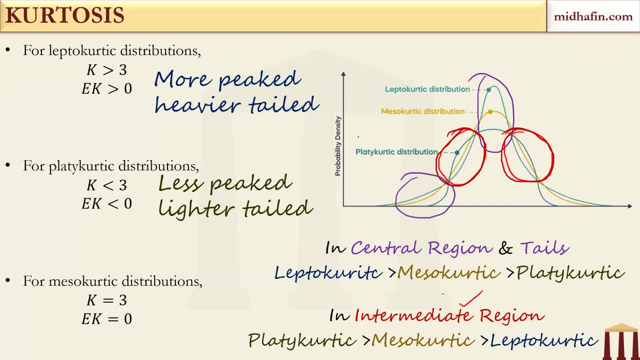 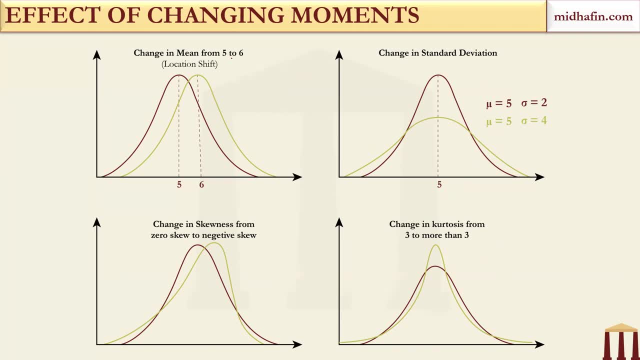 Okay, Great, Let us move forward Now. what will happen if you change the moments? So let us start with the first one. What will happen if you change the mean? only If you change the mean. it means that you are just changing the location of the distribution. 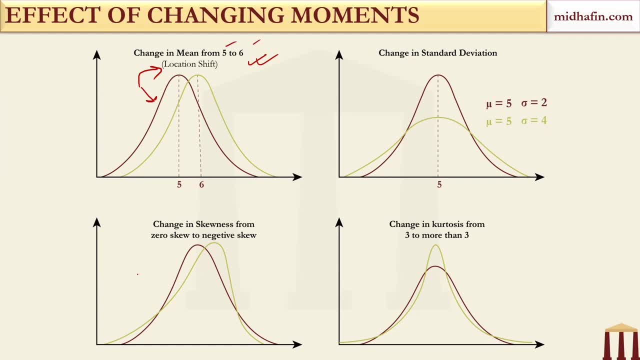 So this is the original distribution. Change the mean from five to six. Nothing changes. No shape of the distribution changes. The shape is completely conserved. The distribution just shifts right by one unit To have a new mean of six. That is the location shift. Then you change the mean. 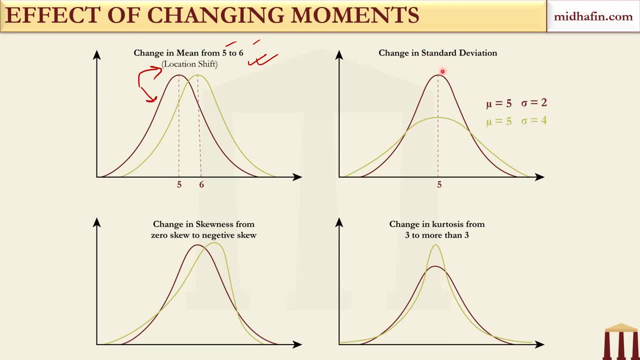 What will happen if you change the standard deviation only? So in this case the mean is same. You can see that mu is equal to five in the old distribution also. Mu is equal to five in the new distribution also. This is the old distribution, But you have. 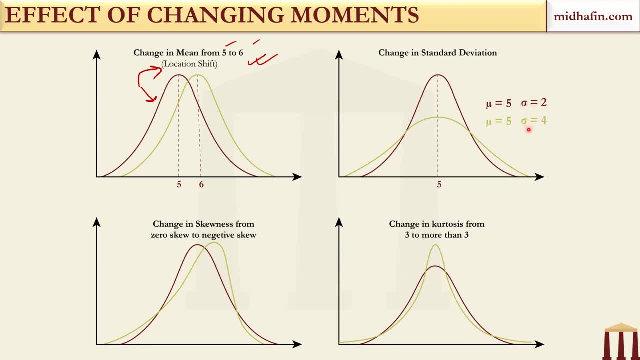 actually increased the standard deviation. So what will happen? The distribution will become more dispersed about its mean. It will become more spread out. You can see green one is more spread out, Light green one right, as compared to the brown one. Ok, then if you change the skewness from 0 to negative, それを変える. 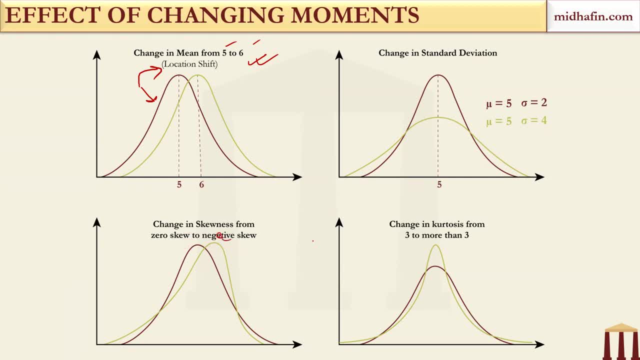 say there is a typo negative. okay, So if you change the skewness from 0 to negative, what will happen? The tail will get pulled to the left side. This tail- left tail- will get pulled to the the left. it will have a more elongated tail, more outliers on the left hand side, Got it? 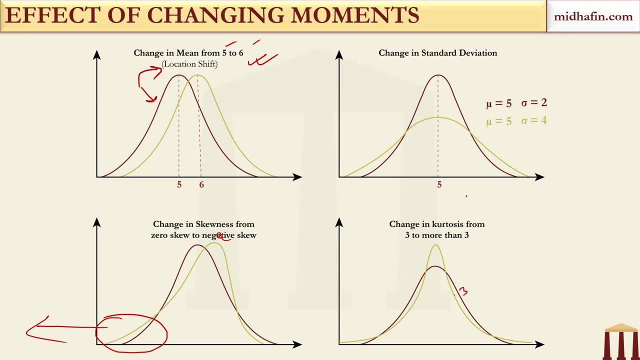 And if you change the kurtosis- let's say the original kurtosis was free- if you increase the kurtosis, then it will become heavier in the center as well as in the tails, and it will become lighter in the intermediate region. Now this actually gives us a very 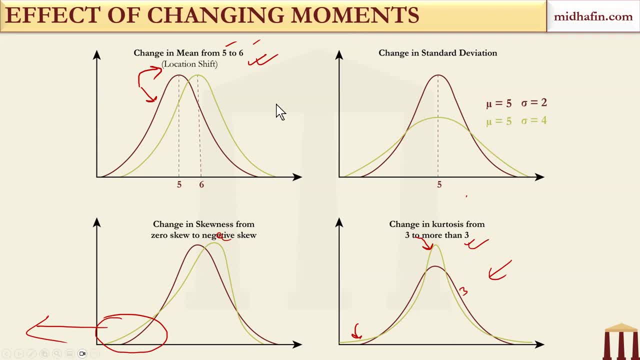 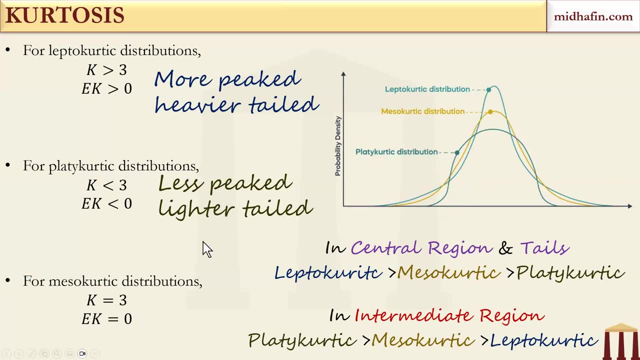 interesting interpretation of kurtosis. So let's go back to this diagram again. I'm just removing all the annotations once again, So let's just go into this diagram Now. just look at the mesokurtic distribution. Remember, mesokurtic distribution is like the normal distribution: Normal distribution. 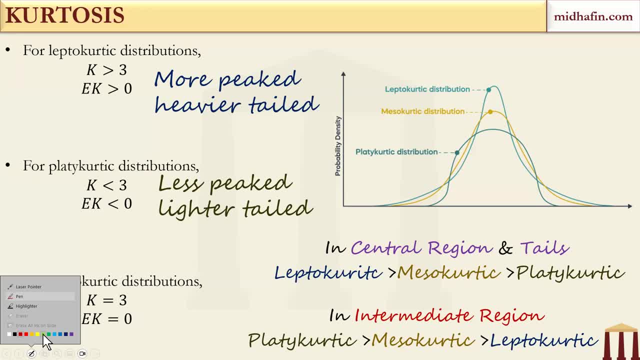 is the mesokurtic distribution. So let's look at the mesokurtic distribution, this one. So if suppose I have the mesokurtic distribution, can I say that to construct leptokurtic from mesokurtic? 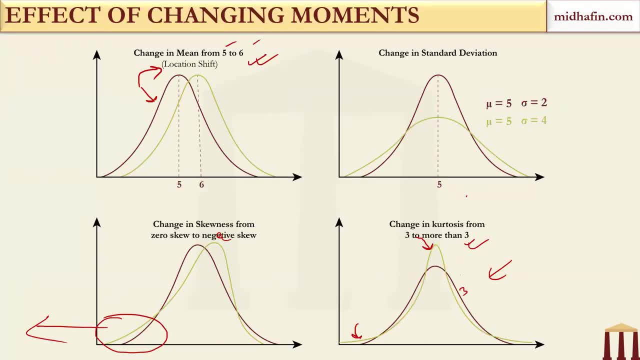 to construct leptokurtic from mesokurtic I can in fact show in this diagram also, and then I go back to that diagram because platy is also there, so you might get confused Over here. we have only two lepto and meso. So to construct lepto from meso, can I say that I 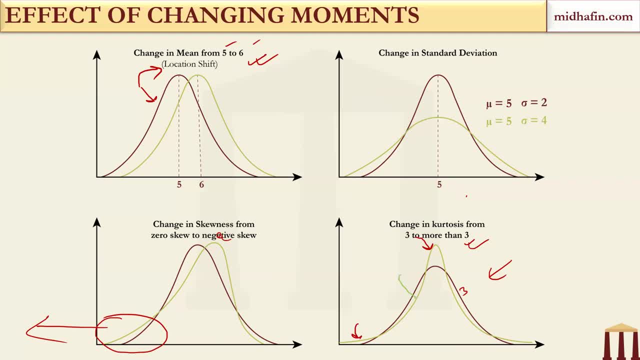 squeezed something from the intermediate region. I deleted this. I squeezed it. I took some portions out. I filled that portion in the center region and in the tail region. Do you agree? Can this be a valid visual interpretation of leptokurtic construction from? 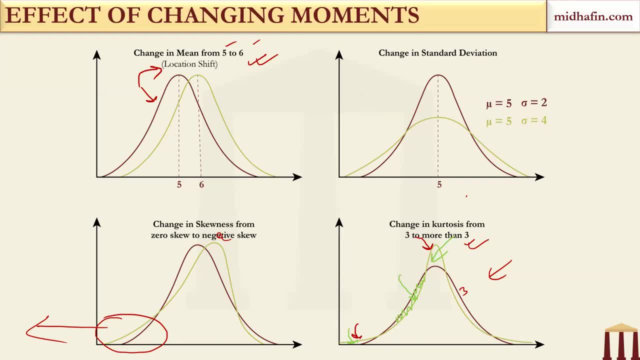 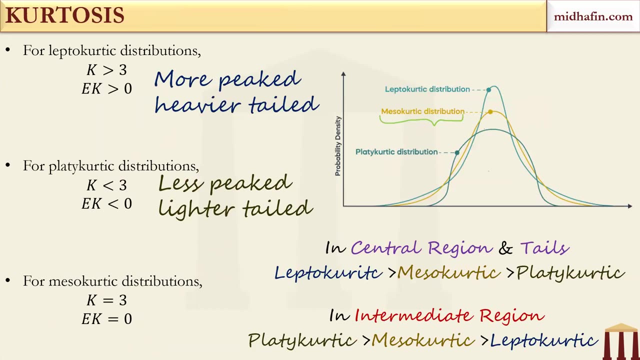 mesokurtic, Everyone, Everyone should be active. As much responses as possible, Okay. Similarly, can I say that for platy I am doing the opposite. For platy, actually it, I am taking out portions from the center and from the tail, so the tails are thinner, center is. 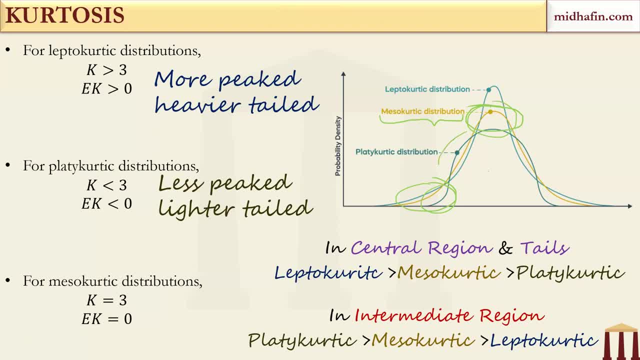 shorter and I am squeezing those portions in the intermediate region for platy so that platy becomes thicker in the intermediate region and loses some weight in the tail and in the center. do you agree for platy? okay, so this is how you can interpret it visually, right? 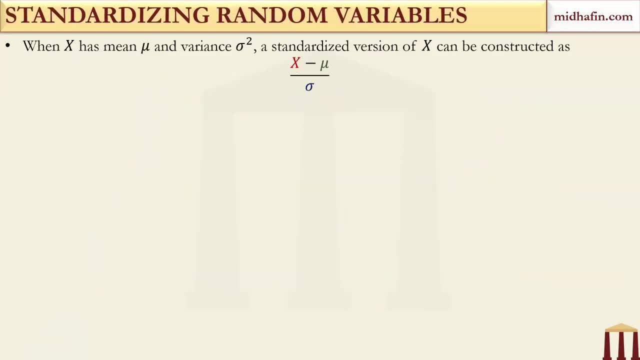 okay, now how to standardize random variables. now standardizing random variables, what you can do? you subtract it. subtract the mean from the value. if x has mean, mu and variance of sigma square, you can construct a standardized version by subtracting the mean and dividing it by the. 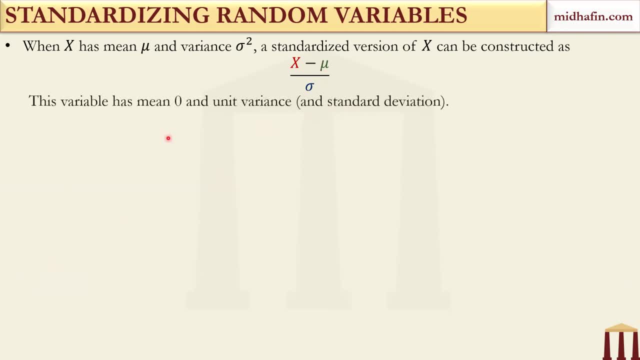 standardized version. now, this variable has a mean of zero. this variable has a mean of zero and unit variance, and we have derived this in the video, not using the normal distribution. we have not remember although this is something which is very close to what we are going to study in the standard normal distribution, but till now we have 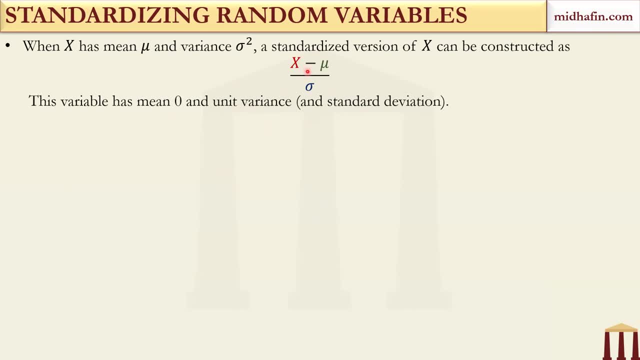 not introduced it. okay, till now we have just introduced it for the purpose of leptok and kurtik, kurtosis and skewness. that's it the mathematical part we have not discussed. so, if you remember, this is also something called as the z value, which we will discuss later. right, 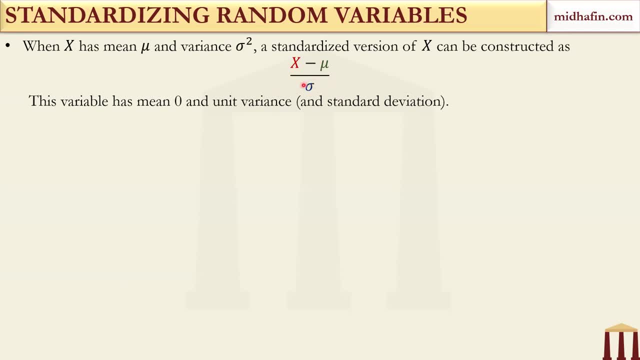 but right now we are just discussing us. if you have to standardize a random variable, subtract the mean divided by sigma square. so this is something which is very close to what we are going to study in the class, and it is guaranteed that this standardized variable has a mean of zero. 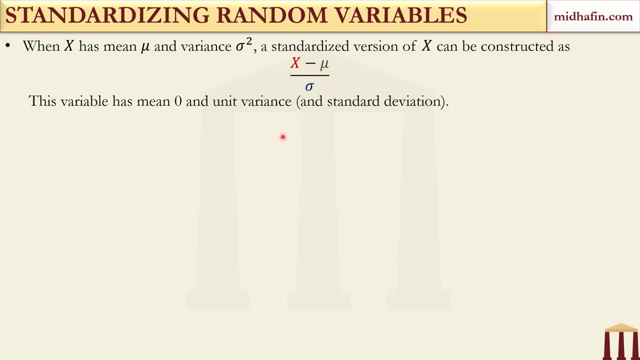 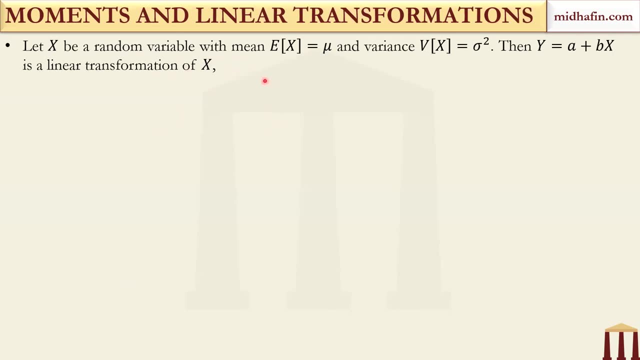 and a variance of one. this is something which we have derived mathematically in the class. okay, now what about transformations? this question was also asked not only in november 2023, but also in may 2000, last year. two times i have heard feedbacks from our candidates that transformations 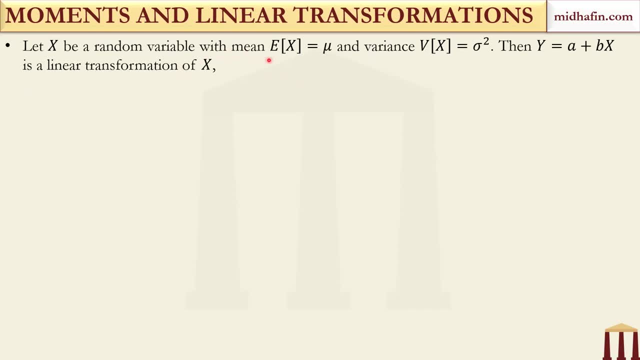 were asked in the exam. so if suppose x is a random variable with mean of mu and variance of sigma square, then you transform this. this y is equal to a plus bx is a linear transformation of x. so what will happen to the moments if you transform the variable? 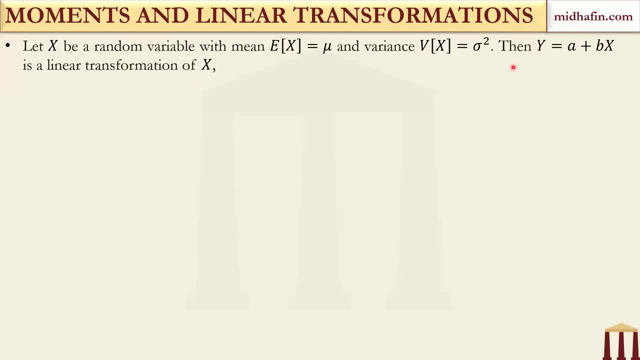 will the moments also be transformed in the same way? let's see. so this is x and this is y. for x, we know the parameters. i am repeating again: for x, we know the parameters mu and sigma square. for y, we don't know the moment parameters. we are about to find out. let us see what will happen. the first moment will be transformed. 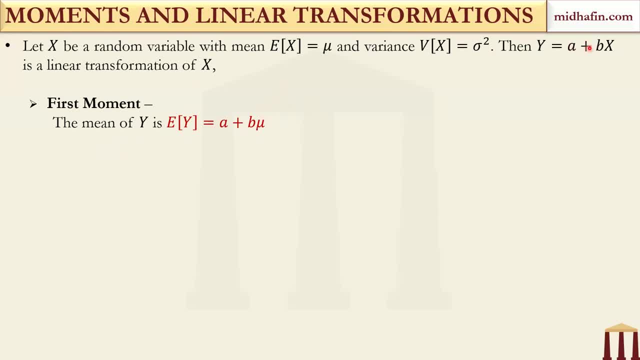 exactly in the same way, a plus bx is the transformation of y, so mu will also become a plus b mu and everything can be derived. you just apply ey. i'm just doing the first one for your convenience, and the remaining, since we have derived in the videos, i'm not going to do it. 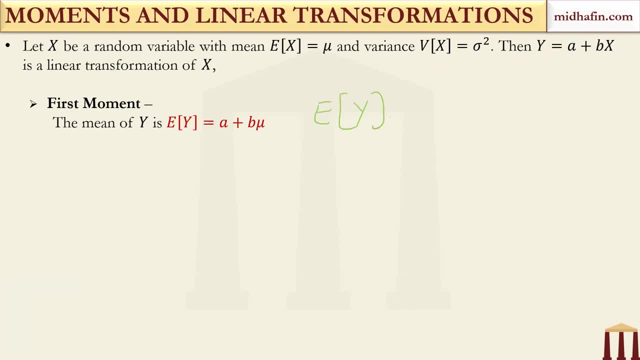 and it's not important also from the point of: so basically, we are just doing this. ey is equal to e of a plus bx, and it's not important also from the point of: so basically, we are just doing the first one for your convenience and so basically we are just doing this. ey is 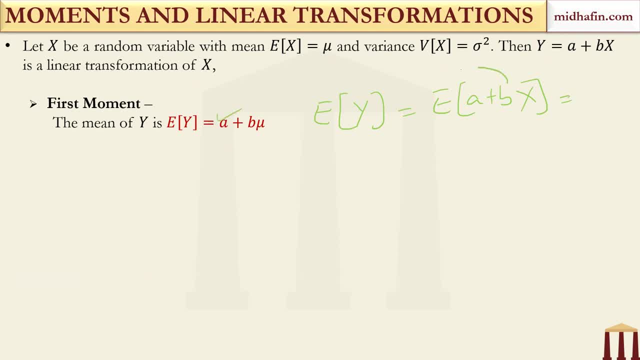 equal to e, of a plus bx. okay, is equal to ea, which is a plus b is. if you remember it was a constant, it will come out. so it becomes b mu, b, mu mu y, because e, x is okay. so this, if we do for everyone, all the moments. so just a quick recollect, can you tell me what will? 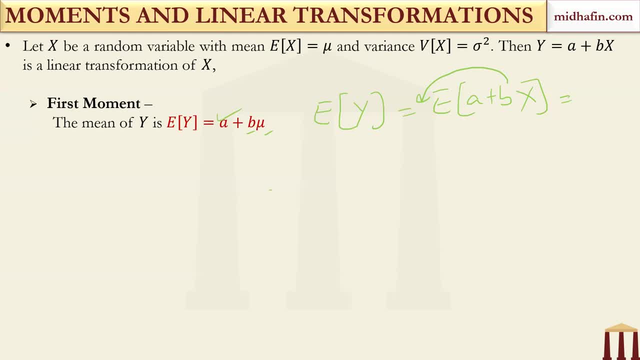 be the second moment? what will be the second moment of why, let's say we are talking about variance, what will be the variance of y? tell me, those would recallak to do for your convenience. that is good for you, see. let us see what will happen to y and. your help, with help with u, can you fly this? the second question is: what will be the second variant to where we are going to define the second variant? let's say i get double interest, but tell me what will be the variance of y. so u have the function no. 1 is 0, so you is Nicht край. 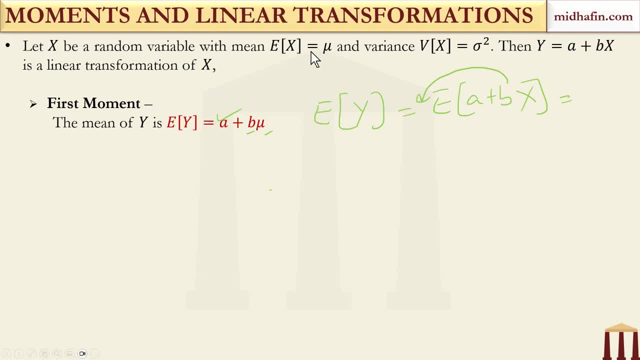 remember, Yes, How to pronounce it? Yes, Very good, Very good, B square, sigma square. Don't say x square, B square, sigma square. Okay, And the standard deviation is square root of B square, sigma square, which is mod B times sigma. So A is gone. So it means that. 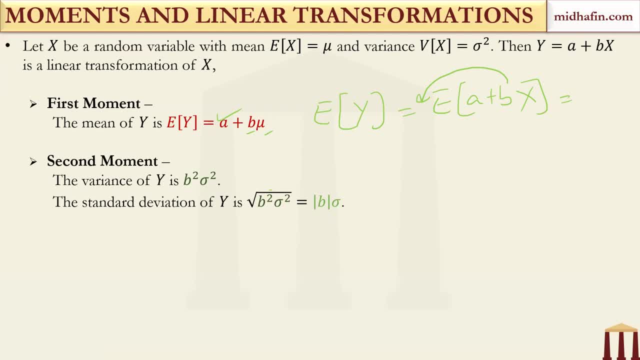 there was no relevance of the location shift. There was no relevance of the location shift when we are talking about variance, Again, the properties of variance, everything can be derived. Just a quick recap Why I added a mod in front of B when I took square root. 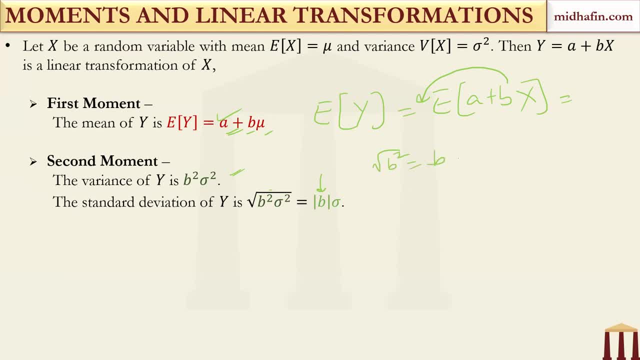 of B square. I should have simply written B, right. Why mod B? Why mod B? Anyone would like to answer. Yes, Sitana, you are right. That is why Platt-Kurtik was having the highest intermediate range Correct In the last case. So why mod B? Why not simply? 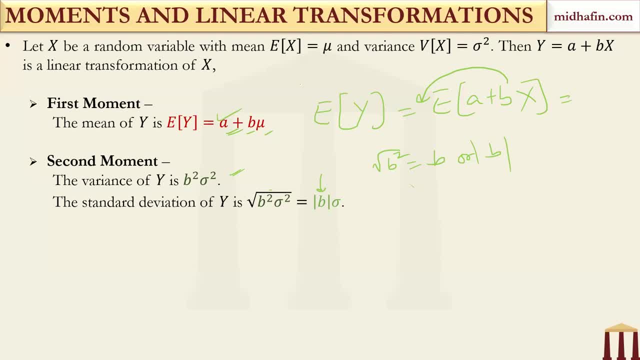 B. Exactly See. the problem is that square root of B square, let us say B, is say negative 3. Okay, And if I do negative 3, square B is going to be negative 3. Okay, So B is going. 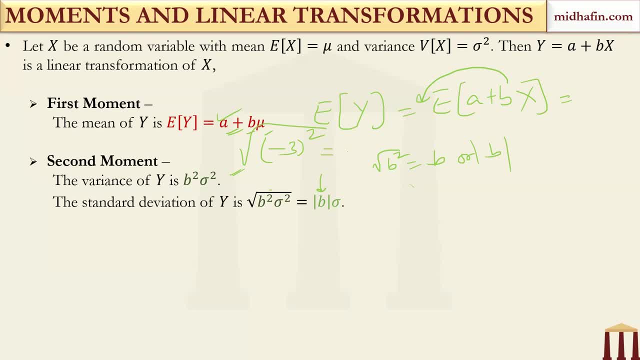 to be negative 3. Okay, So B is going to be negative 3. Okay, So B is going to be negative. 2 square square root. Okay, If I write it, I mean of course it will be a square root. 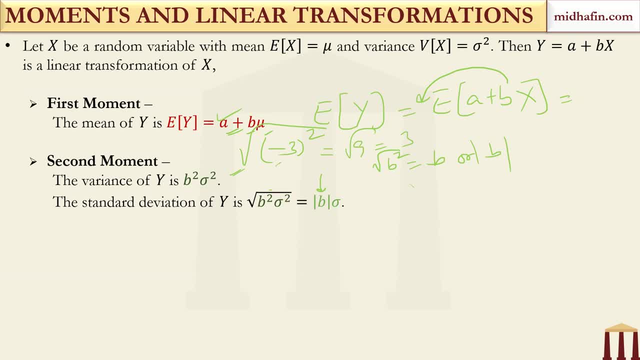 of 9,, which will be 3.. But many of you might say: why not minus 3,? because it was minus 3 square. Why not minus 3?? Because standard deviation cannot be negative. That is the problem. So, even if the transformation, the initial transformation, contains B as a negative, 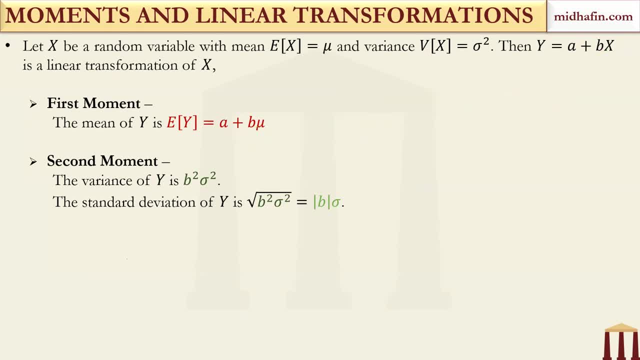 number. Remember, standard deviation cannot be negative Absolutely, So we have to write mod V. And if you remember functions properly from class 11, actually even in function, square root of x square is actually mod x. So that is a different story altogether. We will not discuss. 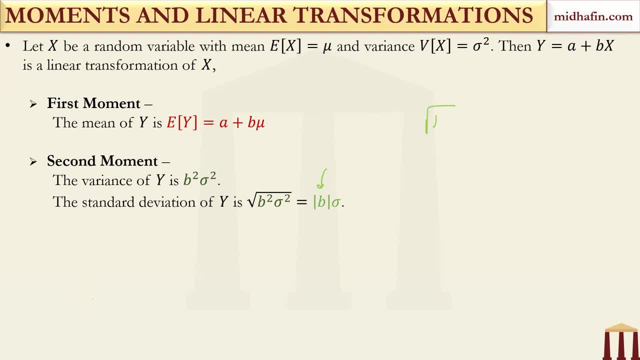 that because the negative part is ignored. Otherwise it will not be a function. There was a problem with one too many and one too many, So one too many problem will happen. It will not be a function. Anyways, that is not a part of the course, So we just have mod V segment. 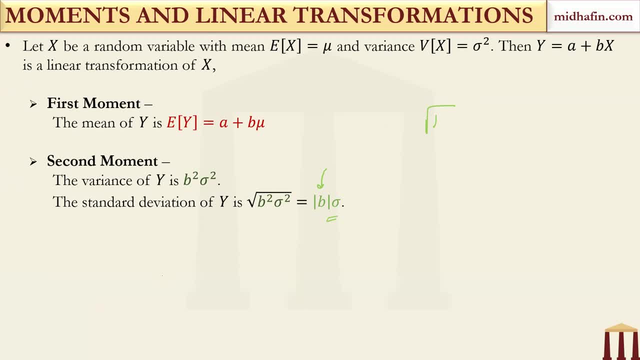 What about third moment? Anyone who can recall what about third moment? So for third moment, skewness of y will be equal to skewness of x if B is positive. So there is again no effect on of A. A only had an effect on the first moment. There was no effect on the second and third moment. 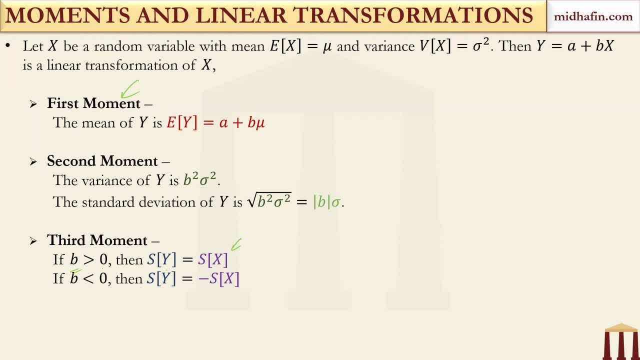 Okay, If B is greater than zero, then B is greater than zero. If B is greater than zero, then B is greater than zero. Then there is no difference in the skewness. Skewness is same. If B is less than zero, the skewness becomes opposite. Magnitude is same in both cases. So 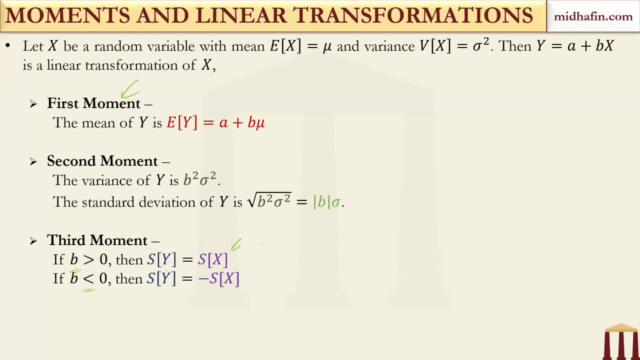 only the sign changes. So you can see that the effect of the parameters A and B are actually decreasing Once you go towards the second moment, then the third moment, then the fourth. In fact, in the fourth moment it will be completely unaffected. 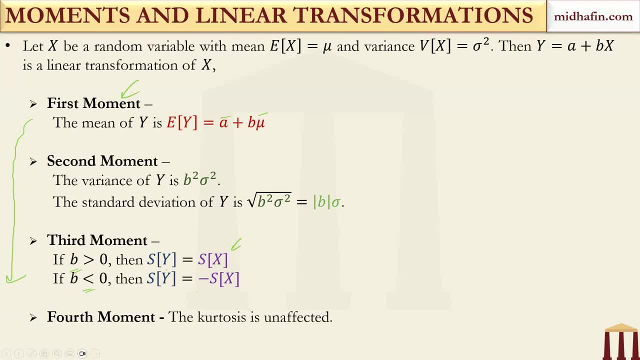 So this slide is very important from the exam point of view, Very conceptual slide. Okay, What happens to the first moment? First moment gets completely transformed in the same fashion. Second moment: only the scale parameter is important, Only B is important. Remember. 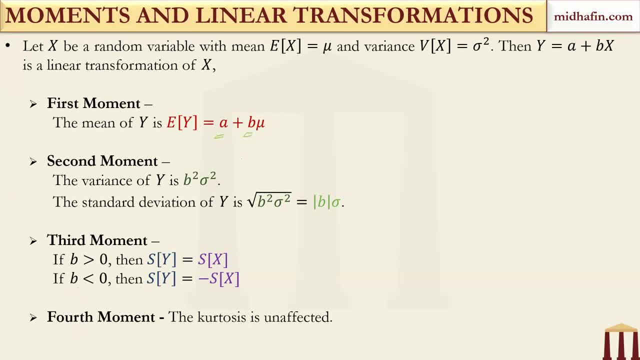 A is known as the location parameter, B is known as the scale parameter. So for second moment only scale parameter is important. For third moment, only sign of the scale parameter is in Positive or negative. For fourth moment, nothing is important, So linear. 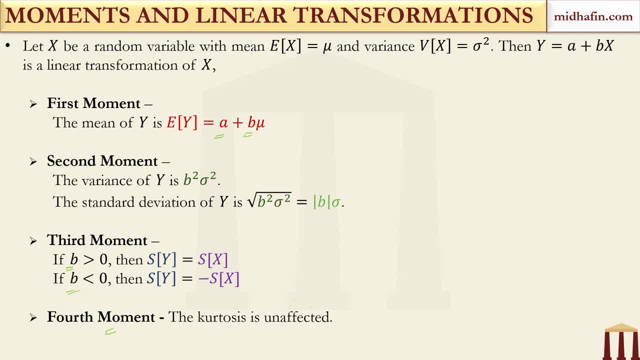 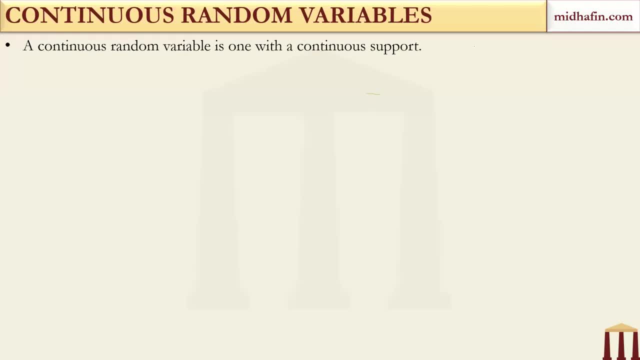 transformation does not affect kurtosis. Okay, Now let us come to continuous random variable. Continuous random variable is a random variable which is having a continuous support. So, for example, if suppose I say all like the example of SMP 500 returns- we discussed Negative 100%. 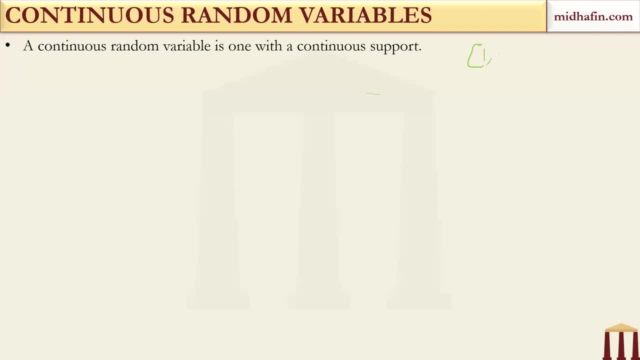 to infinity. Continuous, Let's say all real numbers between 1 and 9.. Continuous, Okay. Now probability of any signal is 0. So if B is greater than zero, then B is greater than 0. So a single value for a continuous random variable is always zero. Can anyone tell me why This? 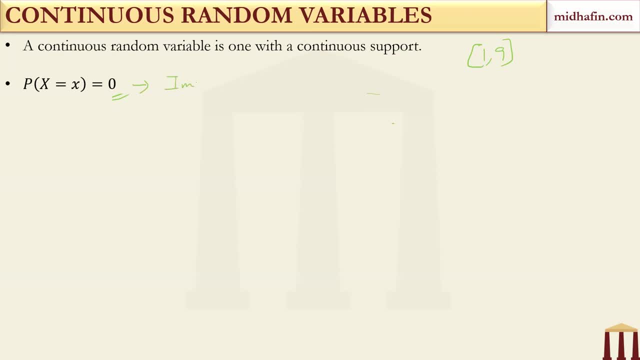 is also extremely, extremely important, And this will be one of the hallmarks of continuous random variable over which we will try to differentiate between PMF and PDA. Can you tell me why? Very good, So can you just send this message to everyone, Sushant? 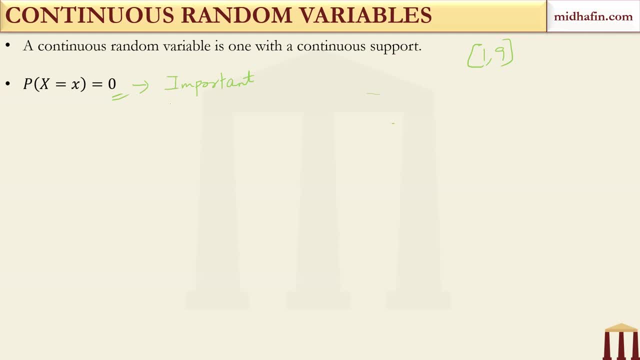 No, Don't say X is very small. So those who have attended our classes, they are answering correctly: Yes, Very good, Because the denominator is infinite. See what did I say? The support is continuous right over here. So if I say all the numbers between 1 and 9, can you tell? 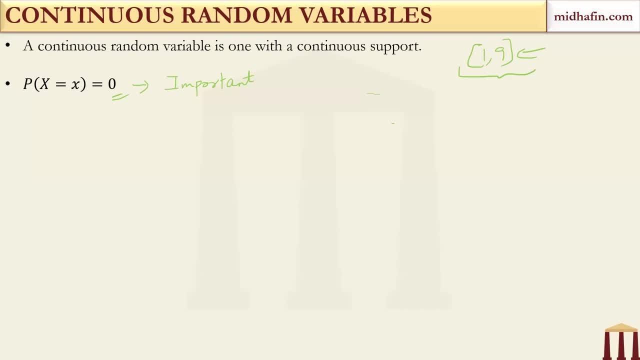 me. how many numbers are there between 1 and 9?? How many real numbers are there between 1 and 9?? How do you calculate probability? This was the formula right of calculating. the probability of any event is equal to NE over NS. How many numbers are there between? 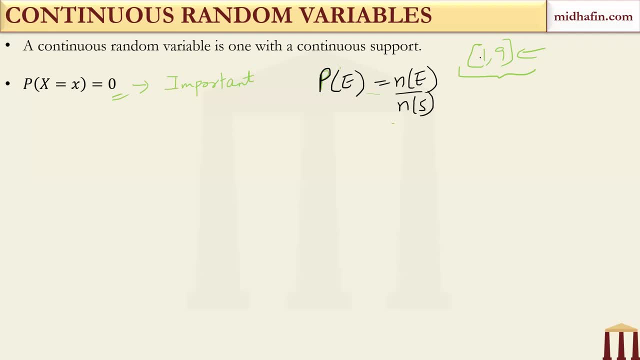 1 and 9? Real numbers, not integers. real numbers For a continuous support. Infinite real numbers because there are infinite real numbers between any two real numbers. Is it clear to everyone that there are infinite real numbers? Okay, So if there are infinite real numbers and 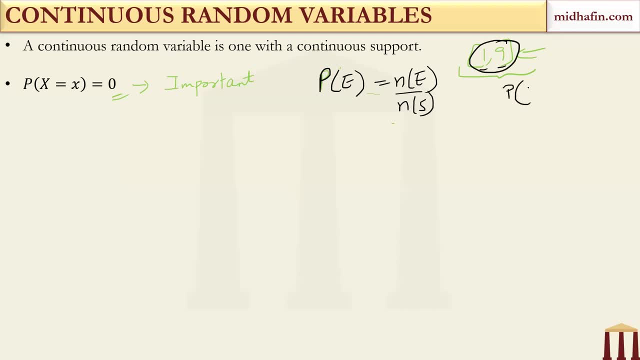 if I ask you, what is the probability of say 10? 2.5.. So 2.5 is only one outcome. So NE will be 1.. Denominator will be infinity. So it will always be the case of finite over infinite. So if the denominator is infinity, this will. 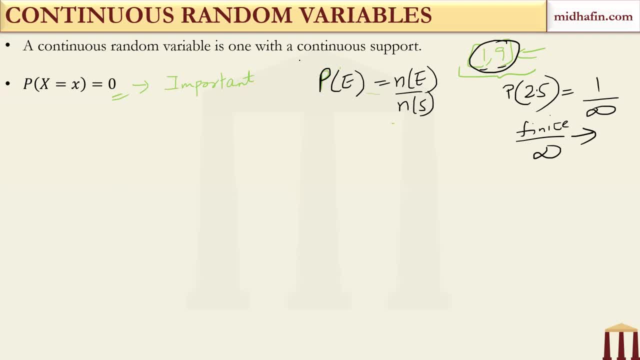 tend to how much. If you divide anything by infinity, what do you get? Theoretically Tends to 0.. So is it clear why probability of any single, any single outcome, any single value in case of a continuous random variable is: 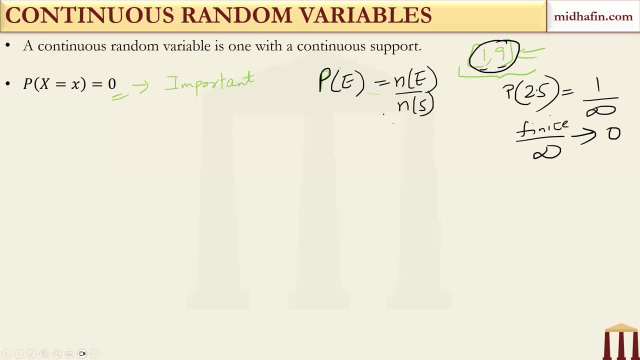 always 0?? Is it clear to everyone? Is it clear to everyone? Great, Okay, Fine, So the CDF is again similarly defined like this: And the interpretation of the PDF right is the same as the CDF: the CDF is the same as the PDF, So the CDF is the same. 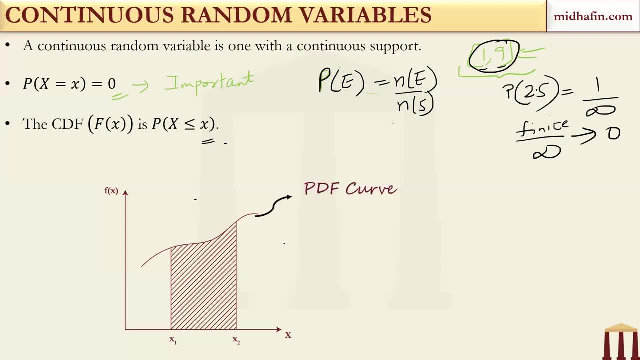 as the PDF. So the CDF is the same as the PDF, So the CDF is the same as the PDF. is something like this: Suppose this is the PDF curve. Now, if you want to find out the area under the curve, this from X1 to X2, this will give you the probability. 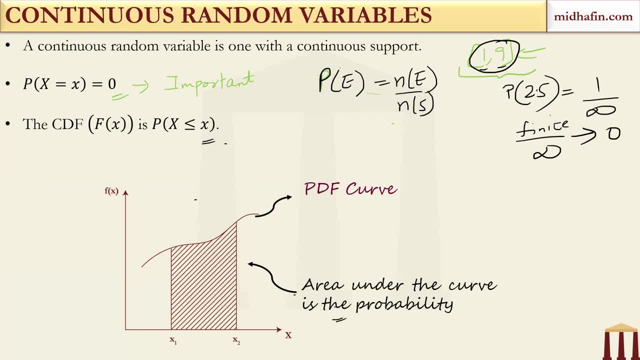 that X1 is between- sorry, X is between X1 to X2.. And how do you find out the area? You perform integration, which is not a part of the course. You don't need to worry about this part. You just need to understand what this part is conveying. It is conveying that the probability 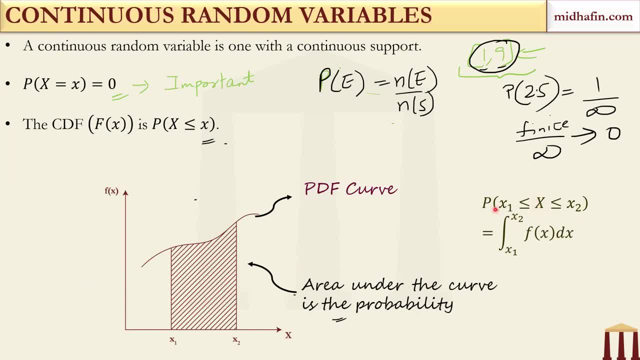 of observing a value X between X1 and X2 is equal to this area under the PDF curve between X1 and X2.. Is the interpretation clear? Formula is not important. Is the interpretation clear? How will you calculate probability To everyone? 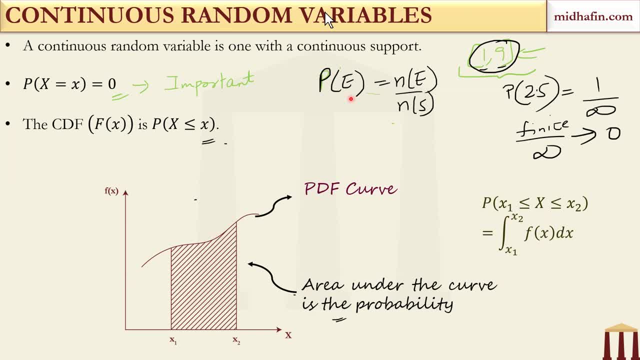 Okay, those who are sending direct messages. please, it is better if you send it to everyone. it will be better. Is the interpretation clear to everyone? Okay, great, Okay, Pooja, I'll explain again. See, if suppose this is the PDF curve. okay, and PDF curve is a continuous curve. 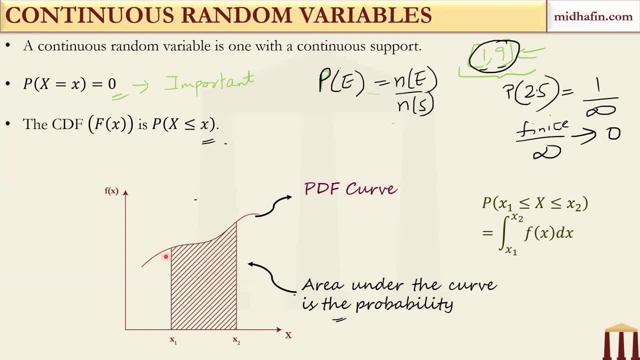 It is a continuous random variable. PDF curve is a continuous curve. If I want to find out the probability, Pooja that X lies between X1 and X2.. So what is the probability that X lies between X1 and X2?? 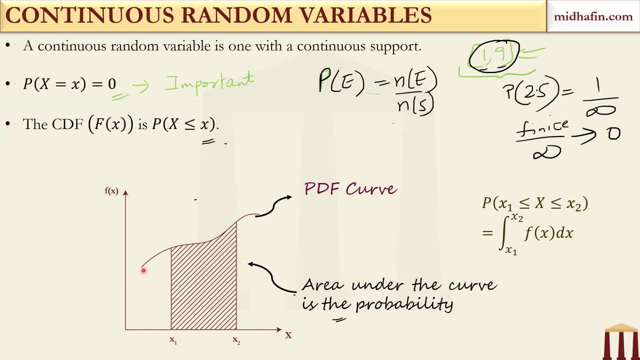 It is given by this area under the PDF function between X1 and X2.. That is what I am trying to say. Okay, so under the PDF, you find out this area between X1 and X2.. This will give you the probability. 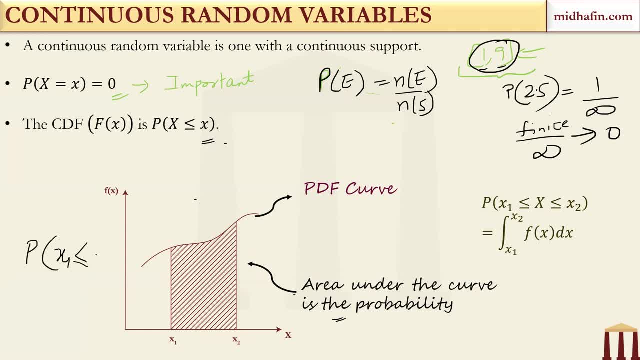 that X is between X1 and X2.. Got it? This area, That is how I am saying it And this is the method to calculate it, which is not in the course. Now Divesh is saying that we don't have integration. 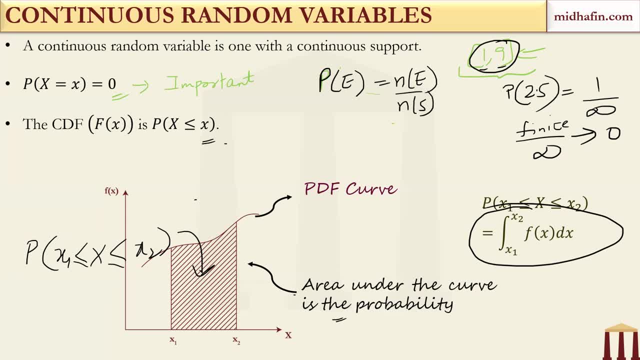 gives me nightmares which I used to have during my 12th. standard Fine, So definitely it's good news. But I'll say that you know you try and revisit those concepts. It might be possible that I mean this is for everyone, not only for Divesh- It might. 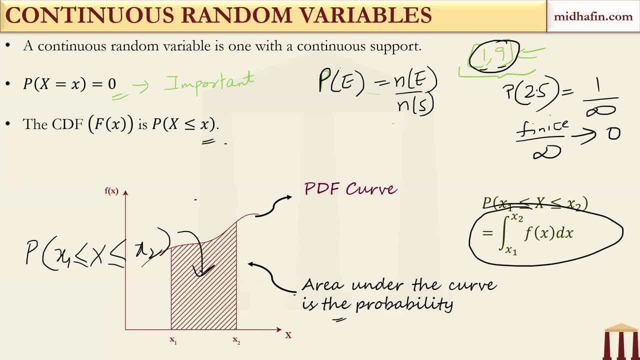 be possible that things might, which were seeming difficult that time, with proper guidance, with proper practice, you might be able to. because, see, I say this all the time to many of my candidates- that right now, the stage at which you are in your career, it's not only about 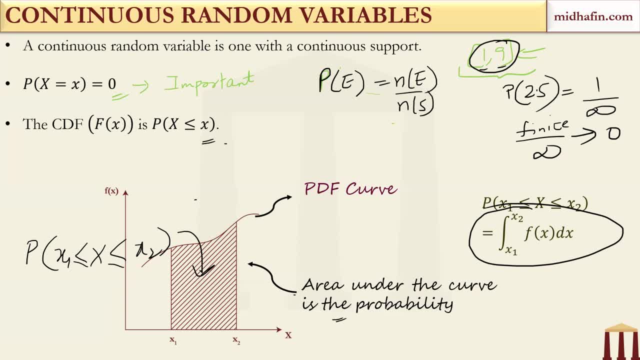 your professional life right. It's about your personal life also. I mean, many of you are freshers, but most of you are working professionals- if I'm not wrong, most of you- And you have a family, Having kids. you have to teach them math, right. So I think it's always better, I mean, take some 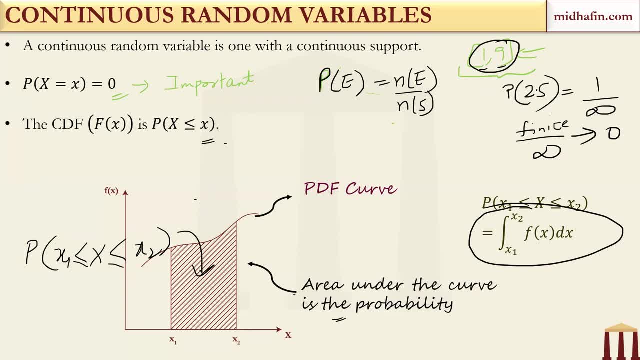 time out, try to revisit those concepts. What is the harm If you're not able to understand? still it's okay. But there's no harm If you're able to recall some things. it is definitely a good thing for you know, teaching your kids Because a good mathematical background, the kind of evolution 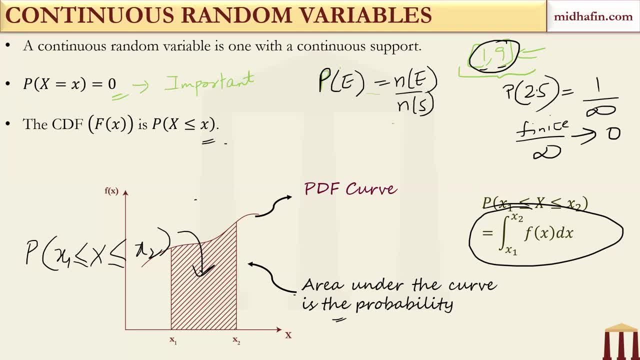 that we are seeing right now in the job market. no, no, no, we will not have integration, 100% integration. Okay, So I was saying the kind of changes that we are seeing with the advent of AI, and we are hearing a lot of discussions right. There have been a lot of debates on both sides. 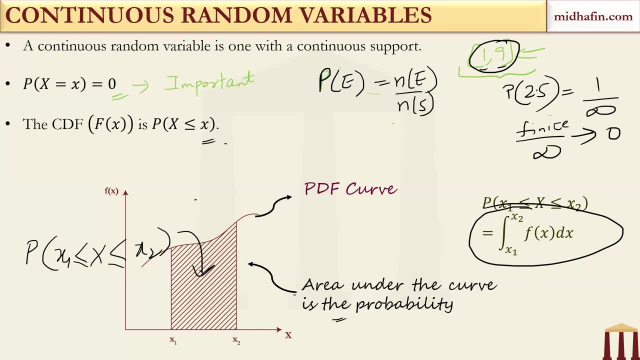 what will happen to jobs and all those things. But anyways, that is a different debate, But in any case, I think in today's world developing a mathematical perspective to everything as much as possible is very, very important. You should definitely try and excel. 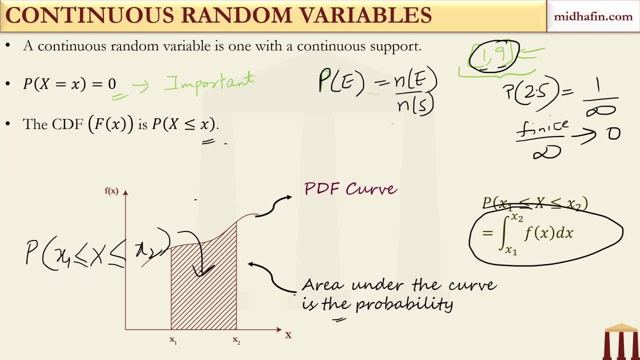 at things as well, And I'm not saying it's the only thing. People might be very good in finance, not very good in math, even that is okay. But I think you should still take a chance, Because if you, let's say, want to learn data science, many of you who are from commerce backgrounds arts. 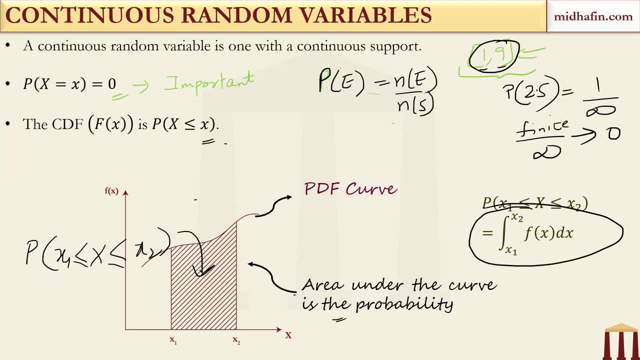 background, say even engineering backgrounds, but did not study engineering properly, did not prepare for JEE properly, switch to commerce background again. there are many of you who actually started with science but then they left and they pursued a career in finance. or it is also possible that you are very good with science. you're very good with math. 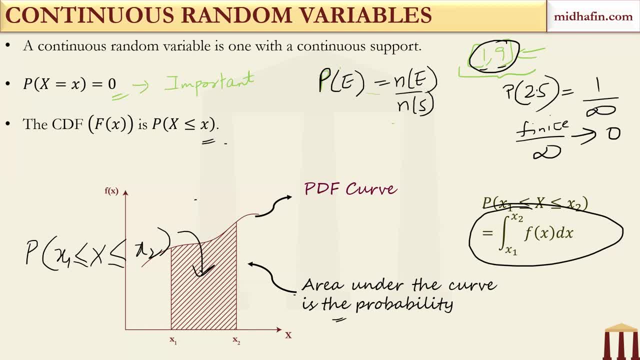 but because of lack of practice, it's been so much time that you are completely out of touch and things seem out of it. But you will definitely admit that if you have tried your hands, learning, say Python, say machine learning or other tools of data, science, mathematical tools, 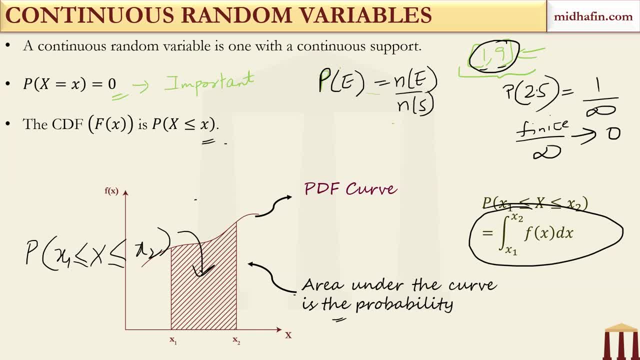 are very important In the beginning. probabilistic and mathematical tools are always taught, So it is a good idea to try and revisit those concepts. You can always take the class 11-12, grade 11-12 books. you can try and have a revisit of those concepts. it will definitely help you. But the good news, 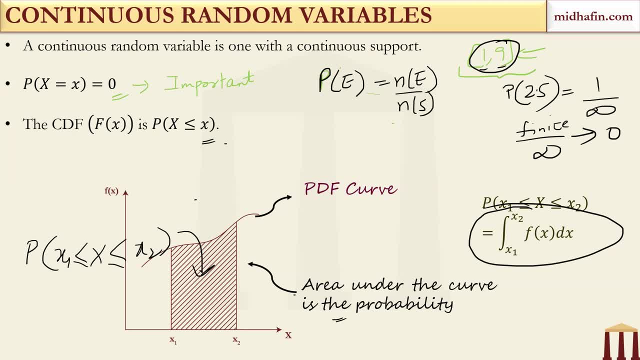 as I said, from the exam point of view, none of these integration concepts are going to be directly tested. only the visual interpretation is affected. Now, as I said, that this part is extremely important, And this is how I'm going to base the difference- This is something which is: 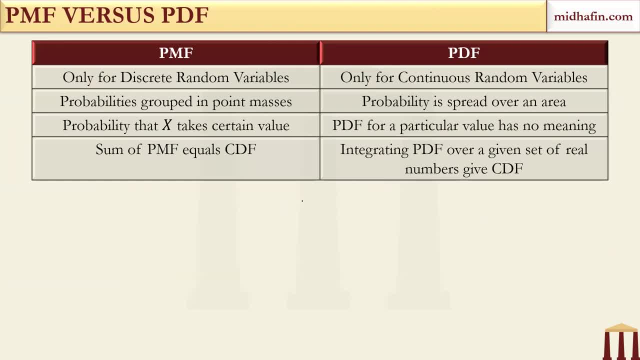 heavily overlooked in the FRM curriculum as well as some other literature also. But I think differentiating between PMF and PDF is something which we should do at all levels wherever possible. So PMF is only applicable probability mass function for discrete random variables- PDF. 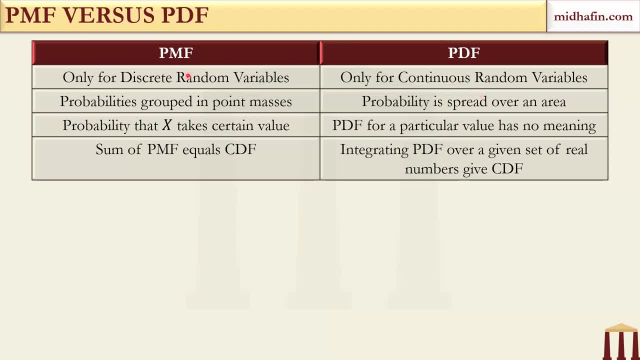 is applicable for continuous random variables. For PMF, the probabilities are grouped into point masses. So for particular values, the probabilities are calculated And the probability for PDF is spread over an area. The third point, I believe is the most important point which you should understand, And this is where even FRM, CFA, past candidates- 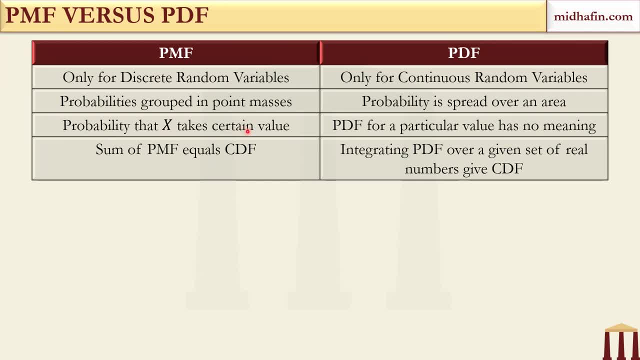 having a lot of experience in the industry, 90% of the candidates will give an incorrect answer. PMF does not. sorry, PDF does not give you probability, whereas PMF you probability. It means that the value of the PMF at any particular point x. 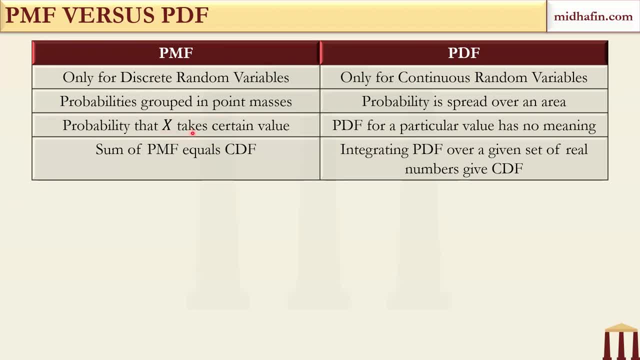 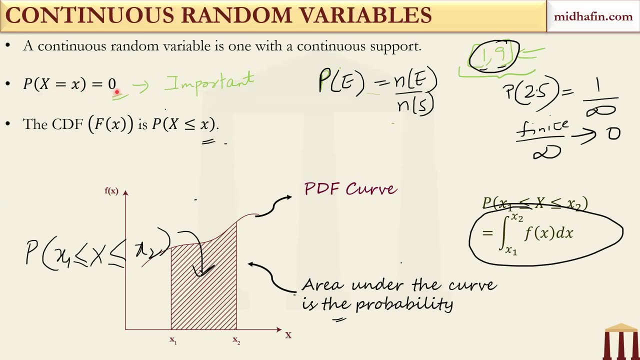 gives the probability that x takes that particular value, Whereas pdf for any particular value has no meaning. Now you will counter question me over it- that right now I said that probability of any single value is equal to zero. Yes, absolutely, I said that. But if you see over here, this is: 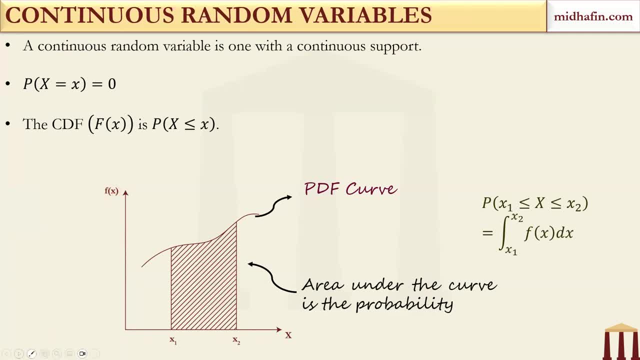 the pdf curve, right. So this fx, these are pdf values, agreed or not? These are pdf values. Okay, so pdf values are having some non-zero values. So these values, this point, let's say this is the point- say at random, I'm saying, say 8.. So f of 8 is having some positive value, correct, Let's say it is 0.14. 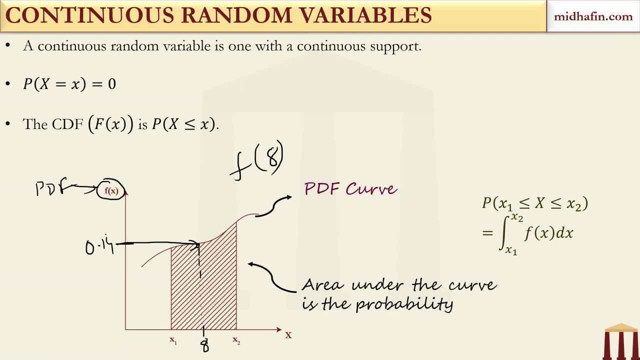 for example. You know what this has: no meaning whatsoever. This has no meaning whatsoever because this 0.14 is not giving you the actual probability that x will be equal to 8. Because we know that from the properties of continuous, random variable probability that x will be equal to 8. 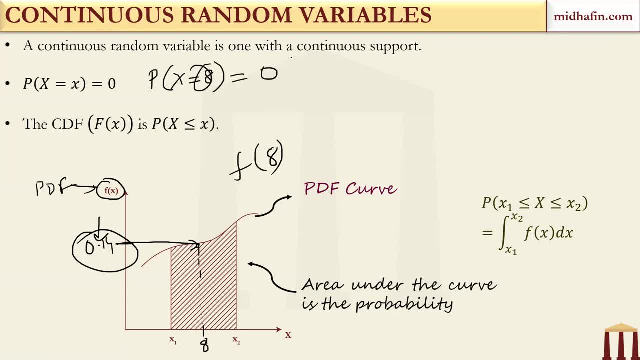 is always 0. It's a single value, So probability of x taking a single value is always 0.. So what is this 0.14 then conveying at point 8? Nothing. It conveys no information. That is the most interesting part: The information is conveyed. if you find out a range over here, Let's say if I. 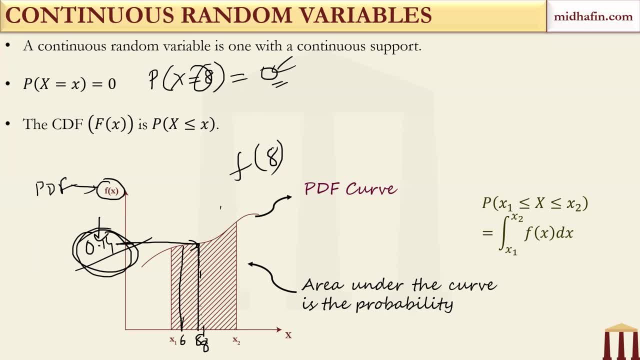 want to find out that x lies between 6 and 8.. If I want to find out the probability that x lies between 6 and 8, I will have to find out this area. This area gives me the probability that x lies between 6 and 8.. But f8,, f6, whatever values they take, they convey no meaning. Okay, at this level. 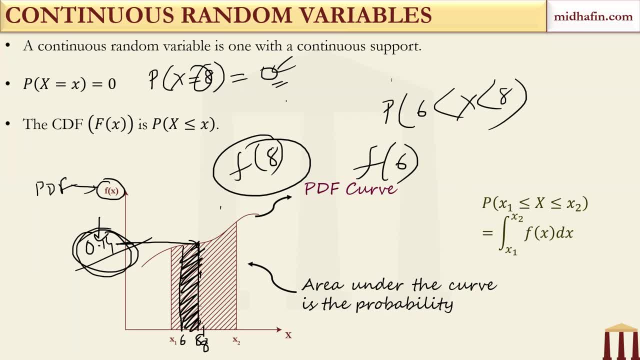 at your level. Again, I am repeating: Okay, so this might sound a bit confusing. That's why I'm I'm repeating: I mentioned that probability of obtaining a 6 or a 8 is how much Is how much? Zero, Correct, But F6, sorry, F6 or F8 might have some positive values. 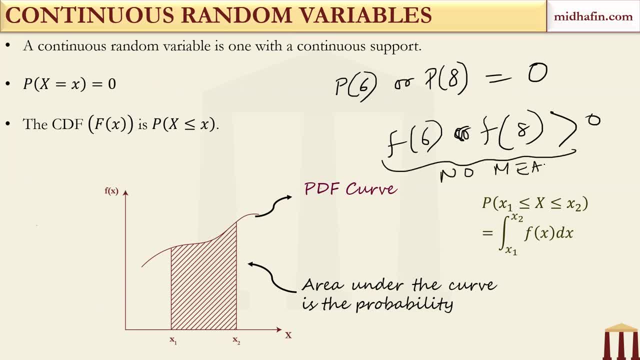 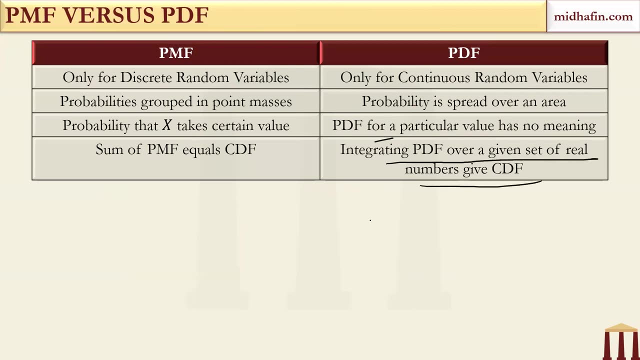 Which have no meaning. So the values of the PDF do not convey you anything. It only becomes meaningful when you integrate a PDF over a given set of real numbers. Okay, When you integrate, then it becomes meaningful. So PDF when integrated over a set of any real. 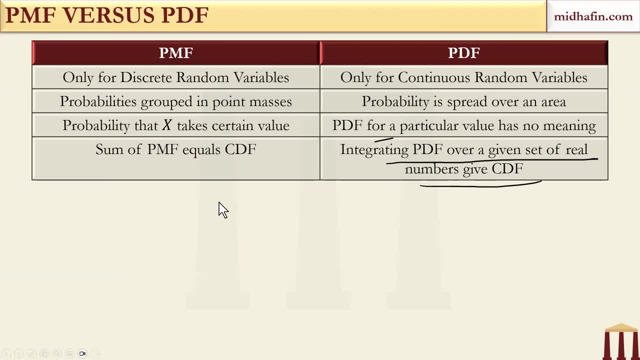 numbers. it gives the problem That X lies between, say, any particular two numbers or in a particular page. Now the last difference, uh, that some of the PDF equals CDF and integration of PDF. sorry, sorry, sum of PMF equals CDF. So summation of PMF equals CDF and integration of PDF equals CDF. 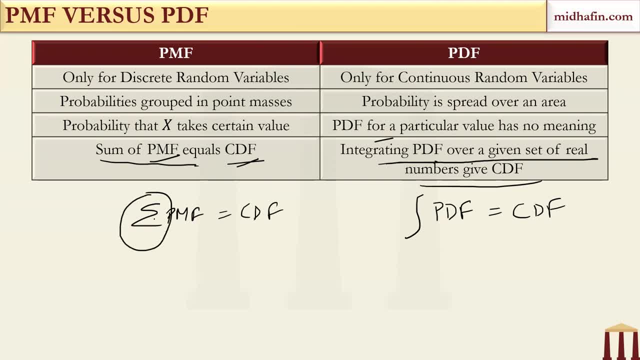 in this case for continuous, Because summation in case of discrete is analogous to integration in case of continuous and vice versa. similarly, differentiation in case of continuous is analogous to difference in subtracting in case of discreet. And that is why, if you remember, I mentioned that to calculate PMF you take a difference. 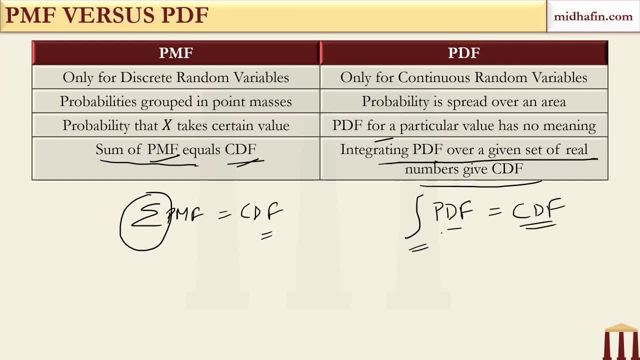 of continuous values Over here. If you differentiate CDF, you will get PDF. If you Really CDF, you get PMF. Okay, So these are conceptual points. This will not be tested except when the PDF is getting Right. 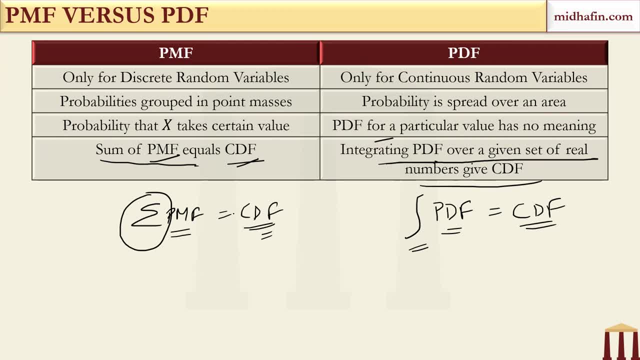 Right not be tested if anything related to integration differentiation, if these words, uh, i'm mentioning they will not be asked in the exam, so don't worry if you don't get okay. so are the differences clear between pmf and pdf? are the differences clear? so, if yes, tell me yes or no. pmf gives the probability. 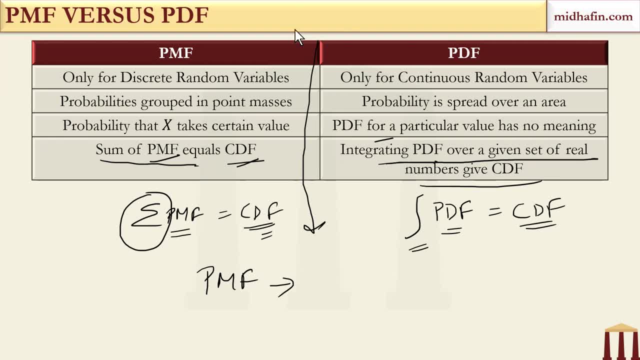 at any point, yes or no. pmf gives the probability at any point, yes or no. okay, very good, yes, correct. next question: pdf gives the probability at any point, yes or no. value of pdf gives the pro: no, very good. so that is the distinction. remember this, okay. 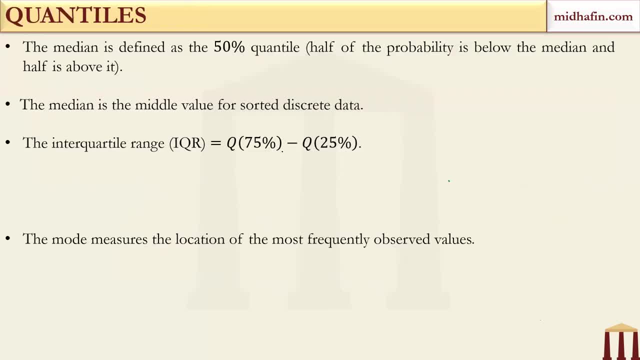 fine. so quantiles, let's discuss again. we are not discussing the quantile function in detail, so it's the inverse of the cdf. we are just discussing the main quantiles. so median is defined as the 50 percent quantile because half of the probability is below the median and half is. 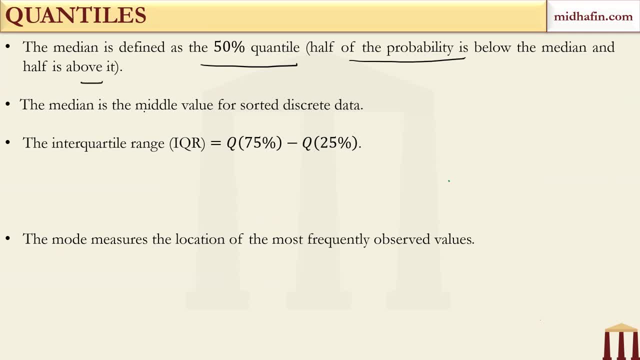 above it. okay, median is the. again i'm mentioning we are not discussing the definition of quantiles and quantiles in details, we are just quickly recapping the main quantiles. median is the middle value for a sorted discrete data. so we have discussed some examples where, if you have discrete data, 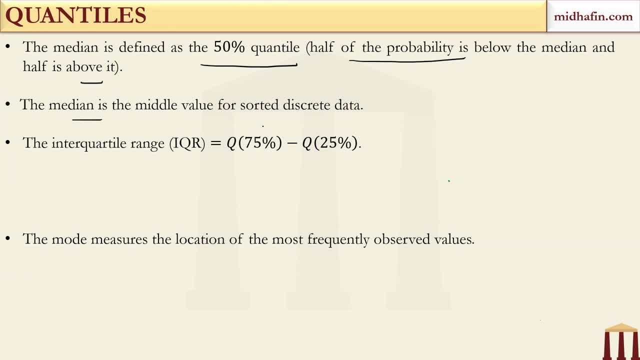 for odd numbers, you will have one middle number and if you have even numbers, you will take the average of the two middle numbers and, of course, for continuous data, it will be the central point where fifty percent of the distribution is to the left hand side, fifty percent of the distribution in terms of areas to the right hand side. 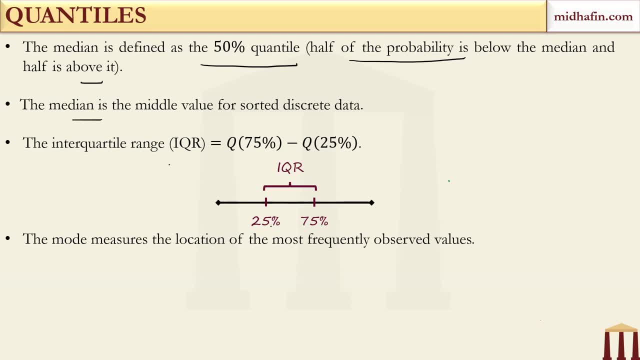 interquartile range. the difference between the 75 percent quantile and 25 percent quantile is a very, very important parameter. okay, and it is actually a very good indicator. uh, just like median, and we'll discuss. in fact, there are some problems with mean. 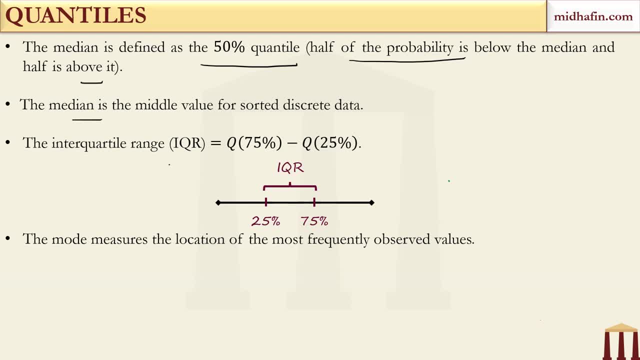 to overcome those problems because median is more robust to outliers. Similarly, IQR is also quite robust to outliers and it is quite a good representation of your average data set And mode measures the location of the most frequently observed value. So you can have unimodal data where you only have one mode. 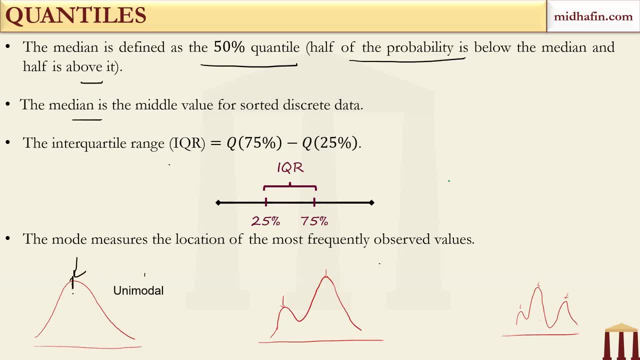 So mode means basically, in a continuous distribution, you're looking at the highest point. So which value of x contains the highest value of the PDF? That is for continuous And for discrete. you will measure which is having the highest frequency. 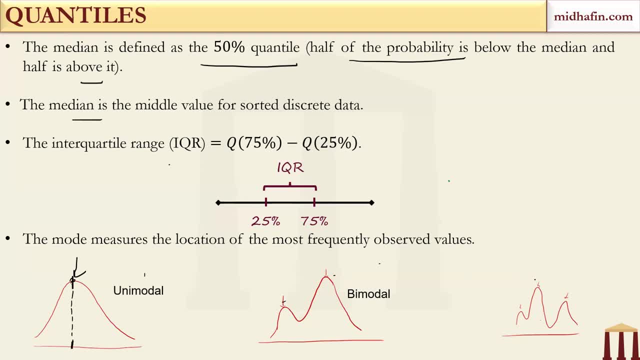 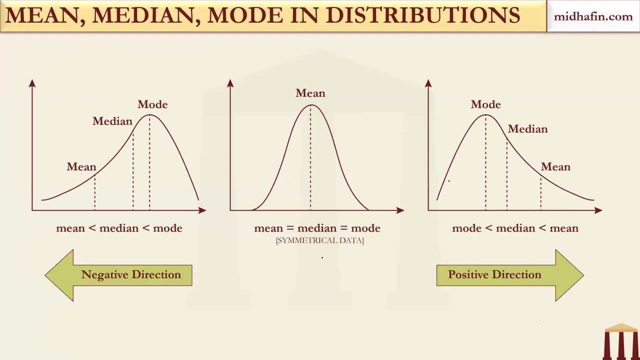 So most frequently observed value. This is bimodal- two modes. This is trimodal- three modes. Now, in distributions, this is the relationship for symmetrical data: Mean will be equal to median, will be equal to mode If the data is skewed. now this is: 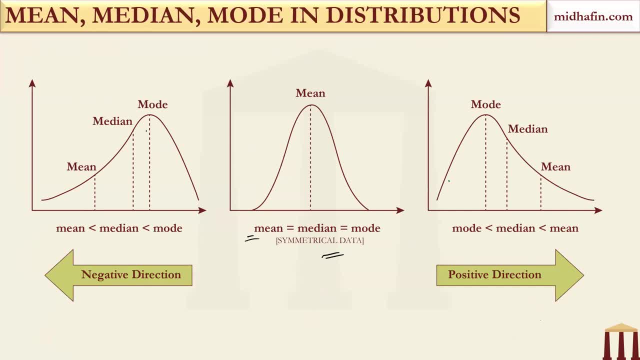 where it becomes interesting. You see which one is pulled the most. See Over here. everything is at the center. in case of symmetrical data, Which of the three parameters- mean, median or mode- is being pulled the most? Tell me, both on the left-hand side and on the right-hand side. 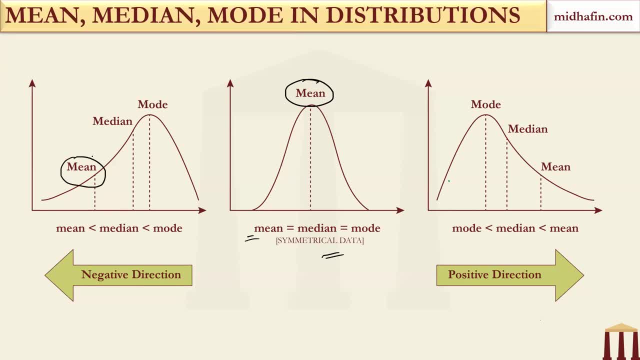 Mean Exactly, You can see. mean is being pulled the most. Mean is being pulled the most towards the left, right, On the right-hand side. also, mean is being pulled towards the right-hand side the most. So mean is more susceptible to outliers. 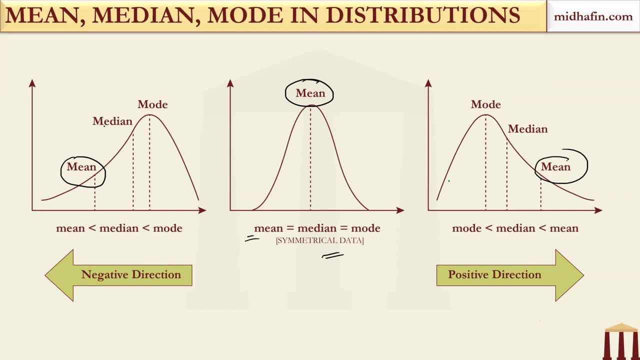 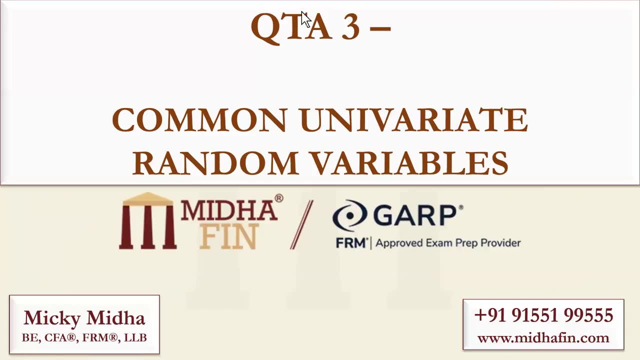 whereas median is more robust to outliers. OK, So remember this, Right. OK, So we'll just take a five-minute break. Please be back by 1.13 PM. I'll not pause the recording. OK, Please be back. 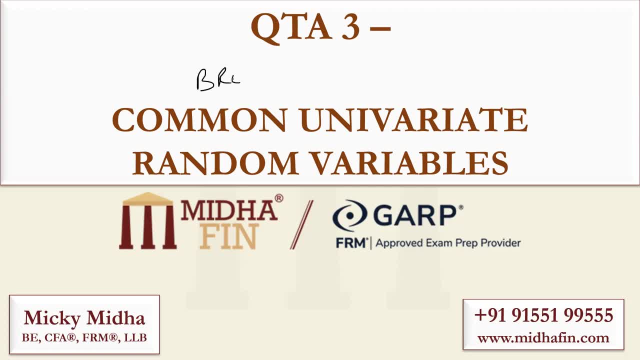 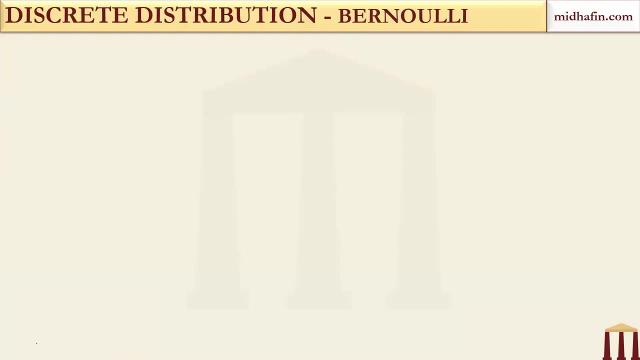 So we start with Bernoulli distributions. So Bernoulli distribution is a discrete distribution for random variables that produce one of these two values: zero or one. It depends on a single parameter, which we call as probability of success or p. 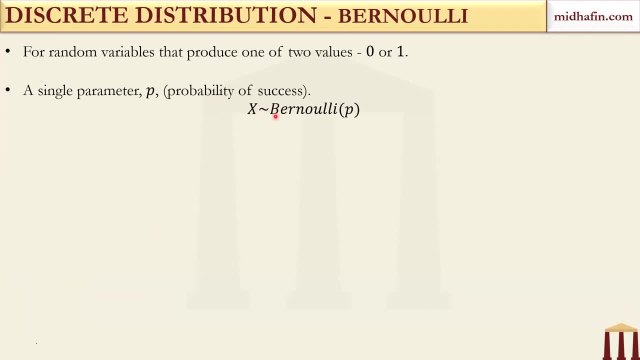 And this is how we represent Bernoulli. x is Bernoulli distributed with a parameter of p. Now, this is the PMF, an example of the PMF of a Bernoulli random review. So there are two possibilities: 0 or 1.. 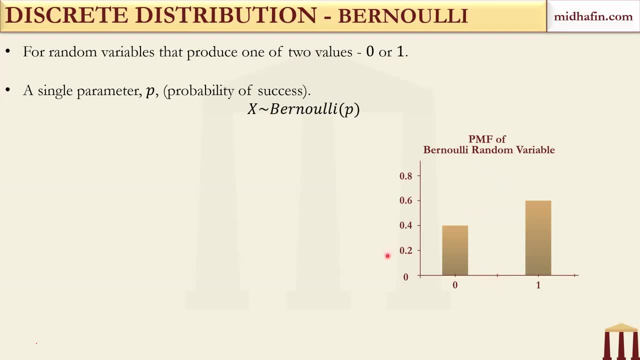 You can call, say, 1 as success and 0 as failure, But the choice is yours. Remember that There is no restriction whatsoever. But the convention is to call 1 as success and 0 as failure, And by success it does not always mean that it should be a good event. 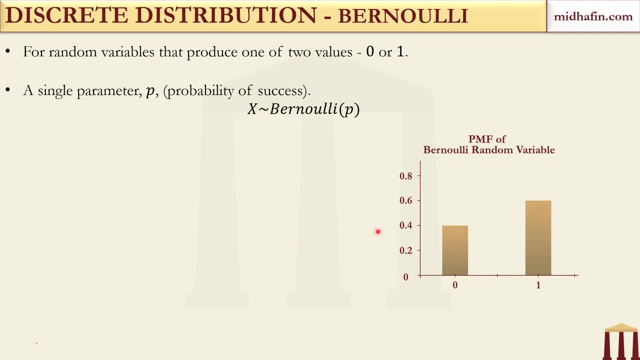 It means that if you're modeling defaults, then default will be your success. OK, so don't worry about these things at all. when you're modeling this mathematically, You can choose anything based on your convenience. So this is an example of a PMF where you can see that if the probability of failure is 0.4,. 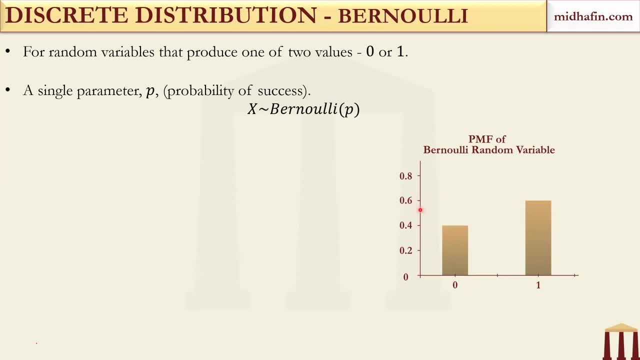 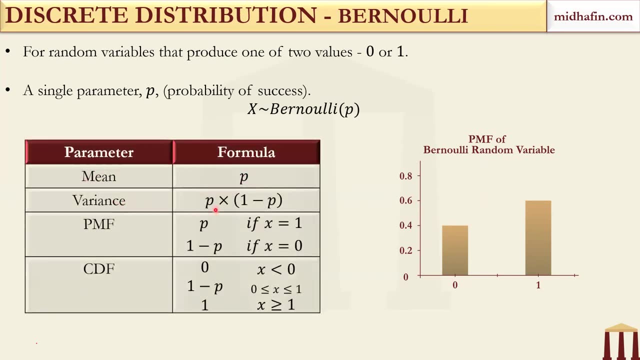 obviously the probability of success will be 0.6 over there. OK, so what are the parameters of Bernoulli? The mean is p, Variance is p times 1 minus p. Again, these questions can be asked directly in the exam. 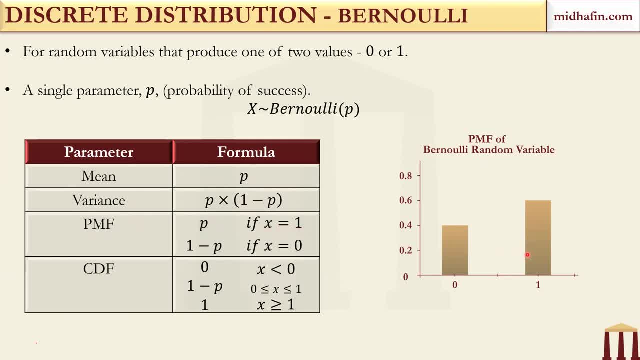 PMF is p if x equal to 1.. It is quite clear over here: PMF is p if x is equal to 1.. And it is equal to 1 minus p if x equal to 0. And this is the CDF. 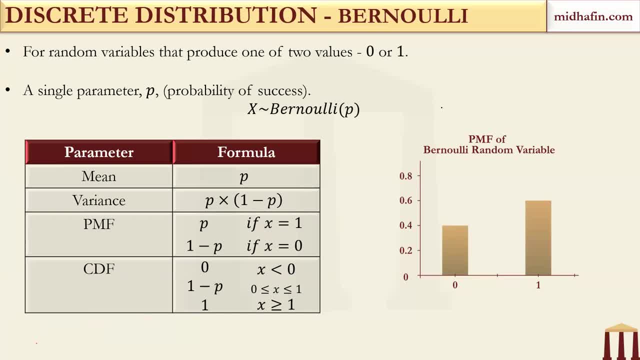 OK, so CDF will be something like a step function for a Bernoulli, a step function So like this. So it will be like this step function. OK, so this is clear, right? Bernoulli is quite simple. 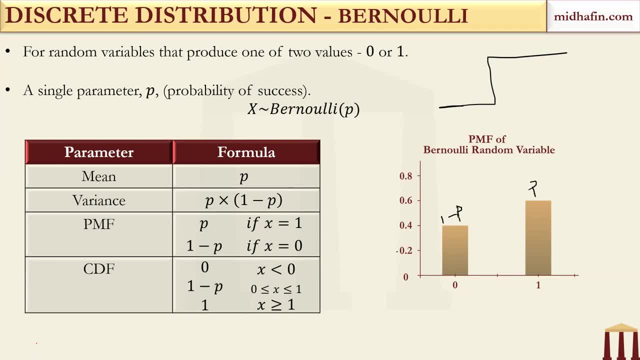 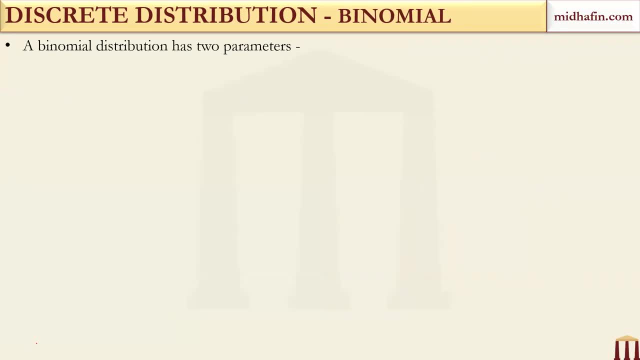 1 minus p. So p is the probability of failure and p is the probability of success. So over here we have taken an example for 0.6.. Then binomial. Binomial has two parameters. You have n, which is the number of independent Bernoulli experiments, and again p, the probability. 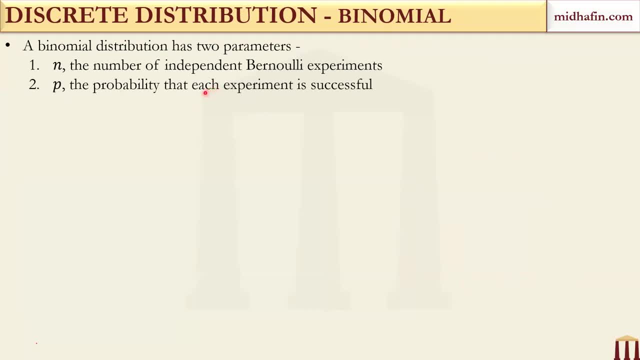 of success. So you can say that binomial is nothing but a collection of n Bernoullis. So this is how you can see. the binomial has been mapped over here. Remember, it's a generalization. It's a generalization. 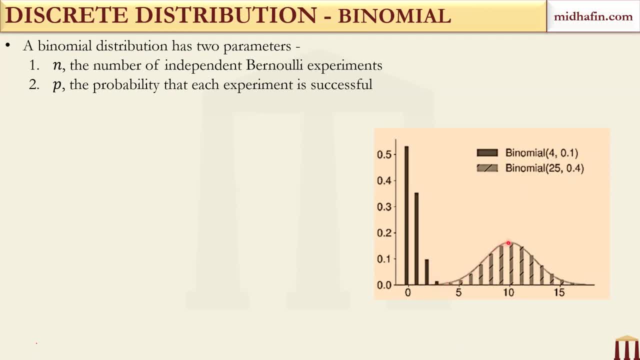 Remember, it's a discrete distribution. So this is just. this curve has just been highlighted over this discrete distribution to convey a message. The message is that when you are increasing the value of n, so earlier n was 4.. So you have these four values of the pn, OK. 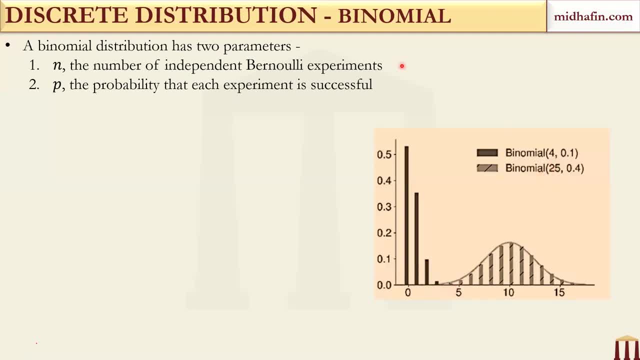 And now you have increased the value of n to 25.. So, as you increase the value of n, any distribution for that matter, whether it is 1,, 2,, 3, 4,, whether it is binomial or not, any distribution, in fact most of the distributions, I'm not. 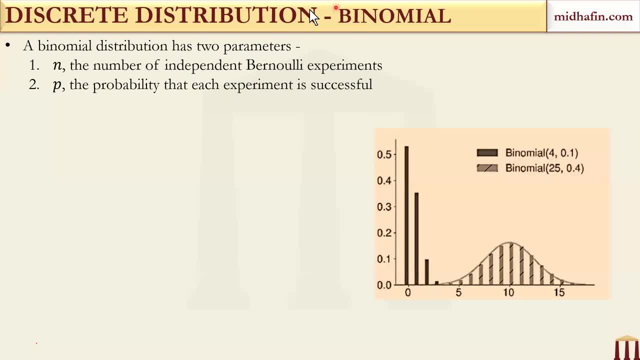 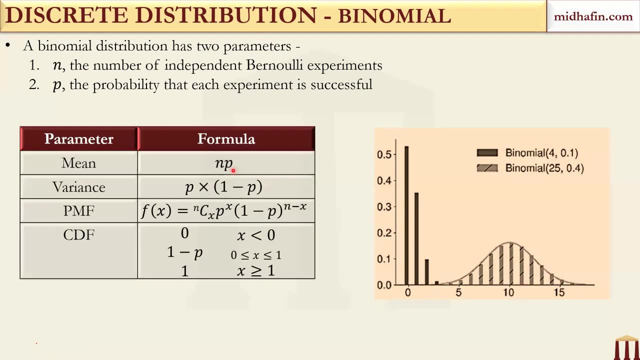 saying most of the distributions which are relevant to the FRM curriculum. they actually converge to the normal distribution And they tend to strike resemblance with the normal distribution. OK, So what are the parameters of binomial Mean? is np variance will be over? here you have, this is missing. this will be np times. 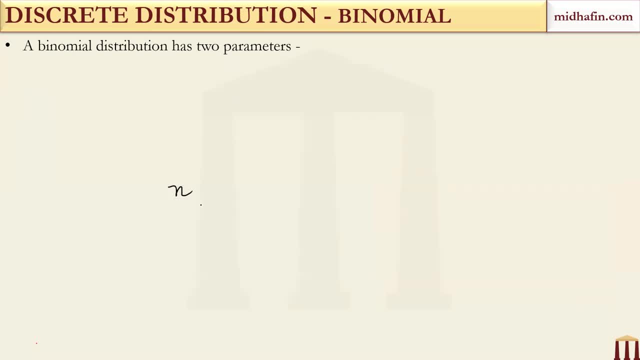 1 minus p. OK, And generalization, And generally what we do is we also call sometimes 1 minus p as q, so sometimes you can call it as nq, also completely your choice. OK, So over here also you can write it as npq. that is what we have told our candidates. 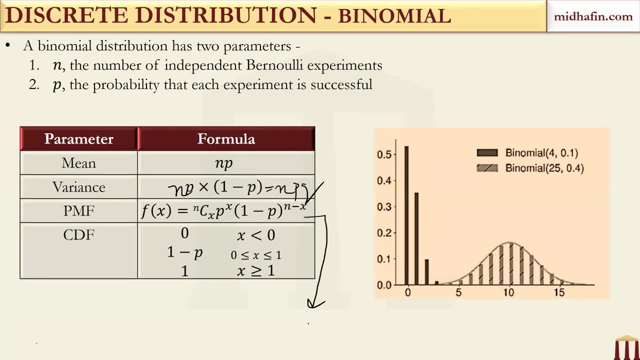 you can remember it like this, because then it is easy to remember the PDF like this, because it is ncx: p to the power x, q to the power n minus x. that is how you can remember. Or directly: 1 minus p. so completely your choice, not a problem. 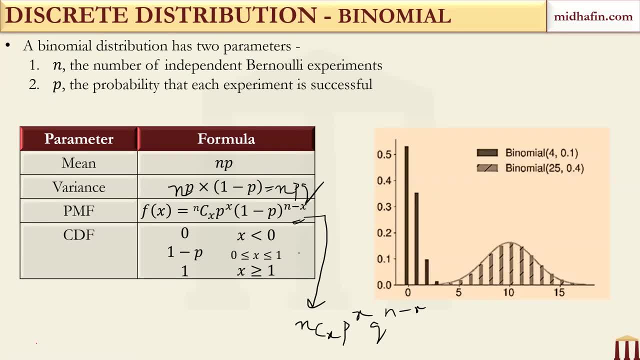 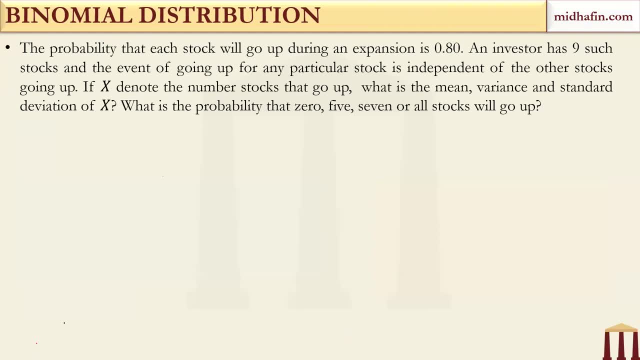 OK, So, based on the PMF of binomial distribution, many questions have been asked in the past, So let's take one of the examples. The probability that each stock will go up during an expansion is 0.8.. Just to make it clear most of the examples that we have, most of them, not all of them. 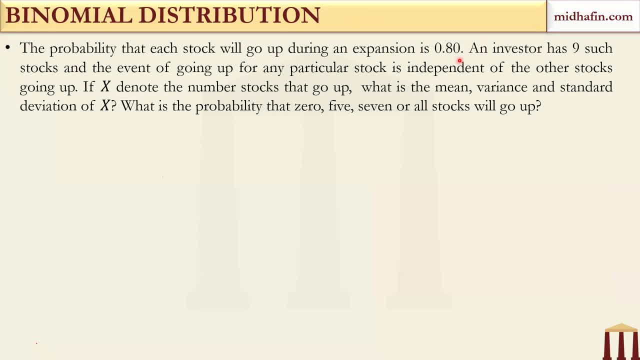 some of them are for card books. also, most of the examples that we are given on this slide- and this is a part of the slides that we have in our class- we have also some of them, So most of the examples are constructed in-house only. 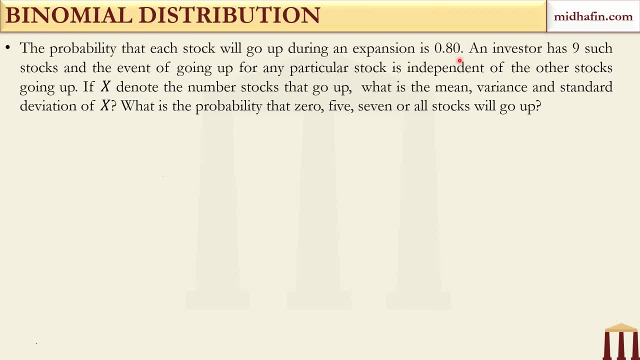 So they are new examples. Many of you might not have encountered these examples and they are not a part of GAR sample papers also, So this is also a chance for you to look into some fresh questions. So this is the probability that each stock will go up during an expansion: that is 0.8.. 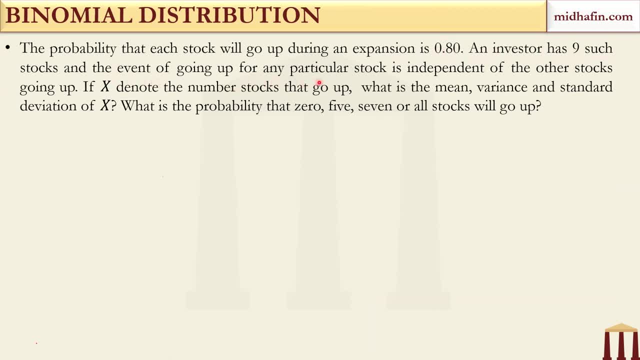 An investor has 9 such stocks and the event of going up for any particular stock is independent of the other stocks going up. If x denotes the number of stocks that go up, what is the mean variance and standard deviation of x And what is the probability that 0,, 5,, 7, or all stocks will go up? 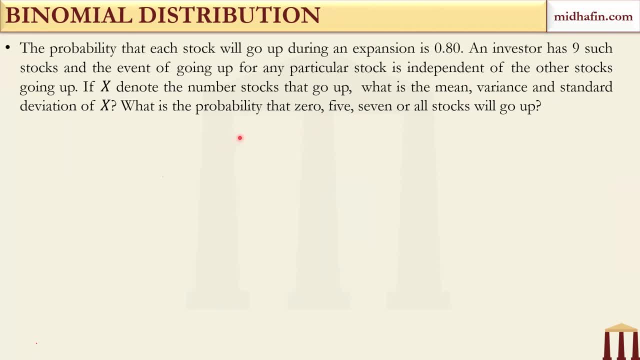 So let's just solve it quickly. So can you tell me what is the value of n over here quickly? What is n? Everyone Correct, Correct, Correct. More answers please, Please be involved. Yes, Nine, Okay. 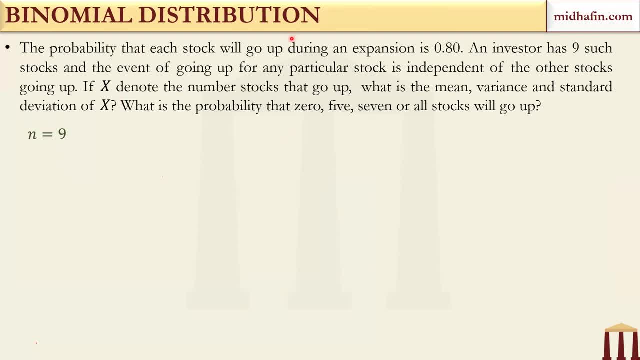 What is p- probability of success? If we term success as the event of the expansion, Correct, Correct, Then the stock will go up. That is my success. let's say, Very good, 0.8.. Okay, So what will be q- the probability of failure? 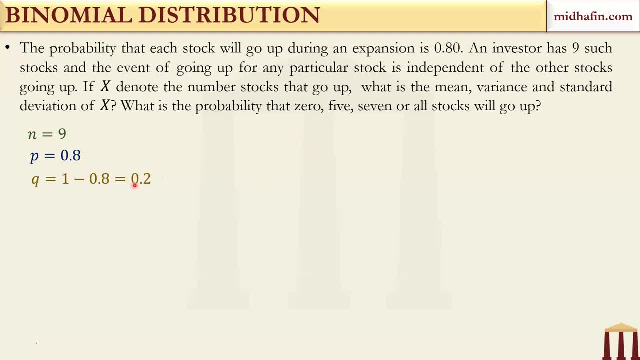 20%, 0.2.. Okay, What will be the mean Mean will be np- We discussed it- 7.2.. And variance will be npq 1.44.. Now, standard deviation will be square root of 1.44, which is 1.4.. 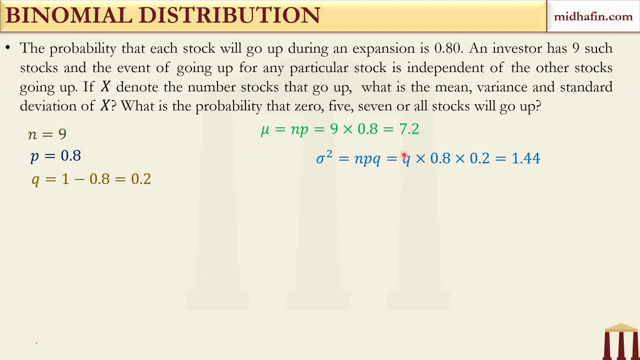 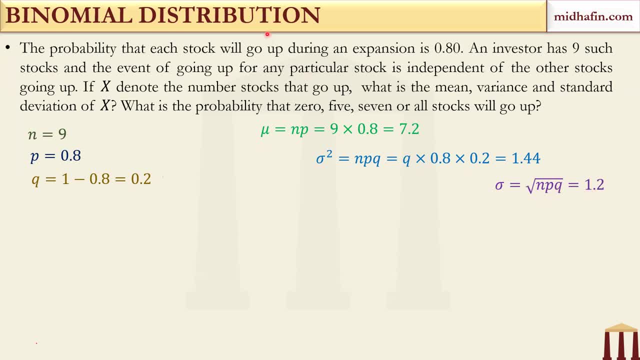 I want to give you a little bit of information. I want to give you a little bit of information. How do you interpret the mean 7.2.. What is the interpretation of this? Because 7.2 is not an integer. 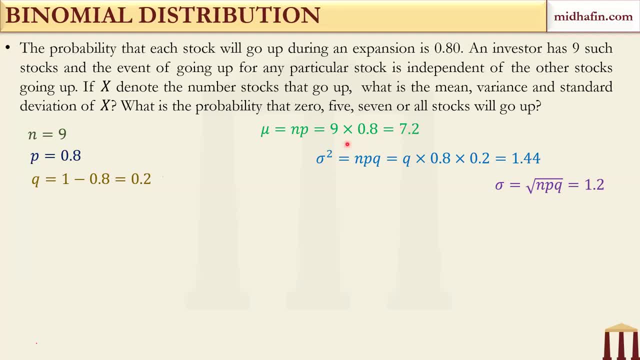 7.2 stocks cannot go up. Do you agree or not? Do you agree or not that 7.2 stocks cannot go up? Okay, So how do you interpret it? You can try and relate it to say some simple examples. 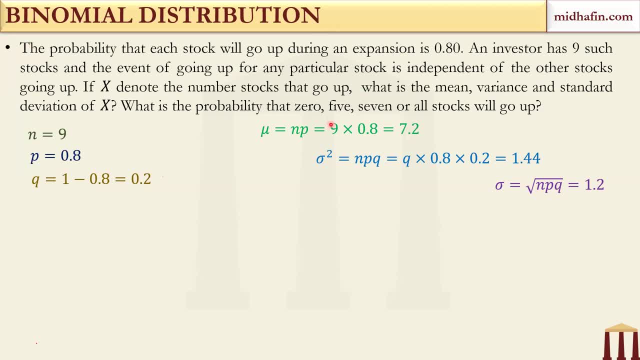 So very good, You can even say: in the long-term average value, the average value of what, In the long-term average value of what. Yes, absolutely correct. So that is a good way to interpret it And that is how probability should be interpreted. 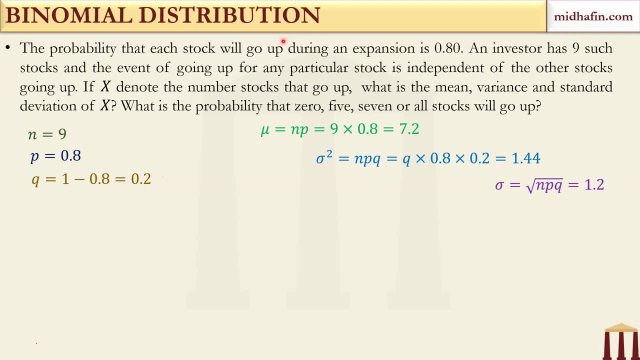 Because if I say that there is a 40% chance that it will rain today- I have calculated, you know, 40% probability- Is it guaranteed? I mean, is it guaranteed that out of 100 days, 40 days it will rain? there is a guarantee. 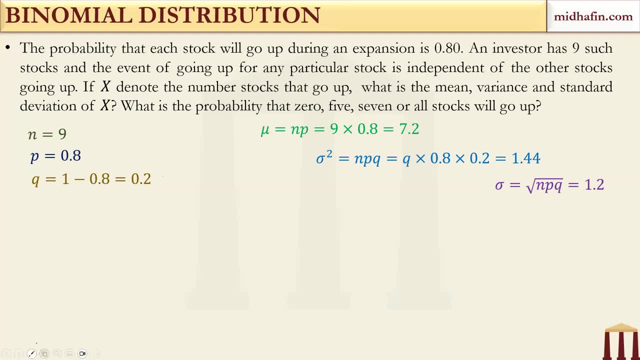 Or let's say, if you take a simple dice, six-sided dice, there are six outcomes: 1,, 2,, 3,, 4,, 5, and 6.. And the probability of each outcome is 1 over 6,, 1 over 6,, 1 over 6.. 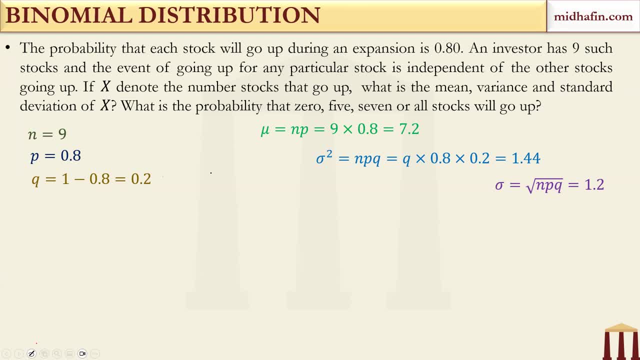 Is it guaranteed that every six times we will have each outcome once? Is it guaranteed? No, You just have to interpret probability. You actually interpret probability like this: that if you carry out the experiment a large number of times, theoretically, it should be an infinite number of times theoretically. 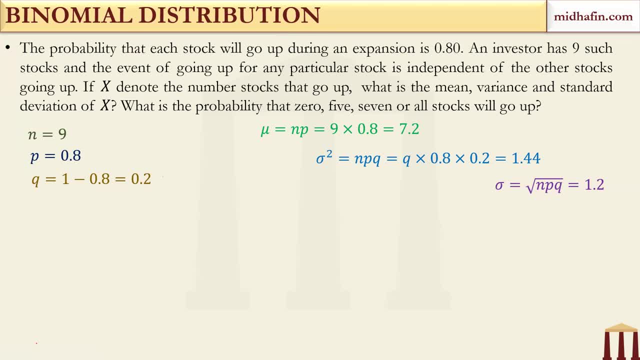 But if you carry out the experiment large number of times, then your actual probabilities, the practical probabilities, the calculated probabilities, will converge to your theoretical probabilities. That is how it should be interpreted. So if you say: roll the dice only ten times, 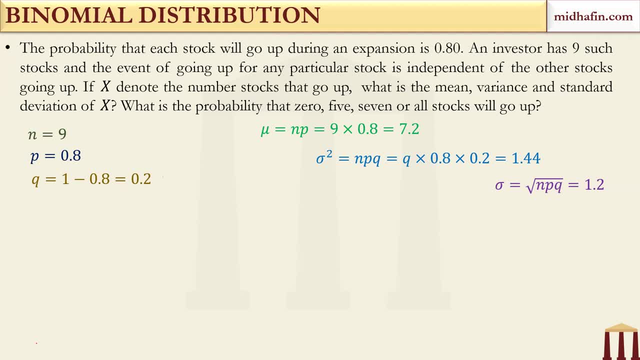 Then calculate the number of outcomes that you got. say, number of times you got one, two. they will be very different from the theoretical probabilities of one over six. one over six: if you roll the dice hundred times, they will become better too. they will become a little bit closer to one over six. 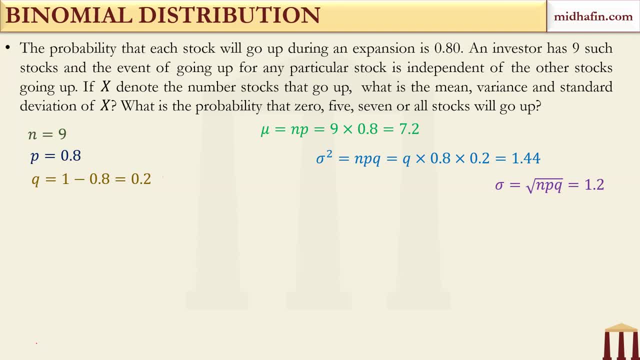 if you roll the dice ten thousand times, million times, billion times, if you roll the die billion times, you will automatically find that the probabilities of all the outcomes they match and they are very, very close to one over six. so this is how it should be interpreted. similarly, expected value. if you find out the expected value of 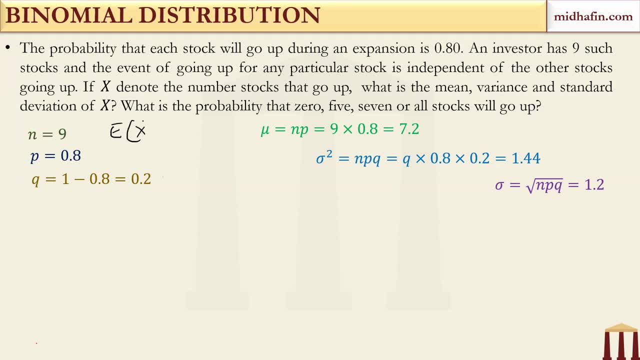 say any random variable, say again in a throw of a die, you'll actually find that for a throw of a die the expected value is 3.5. but 3.5 can never happen. occur on the dice. because if you multiply, say one by six times one plus one by six times two plus dot. 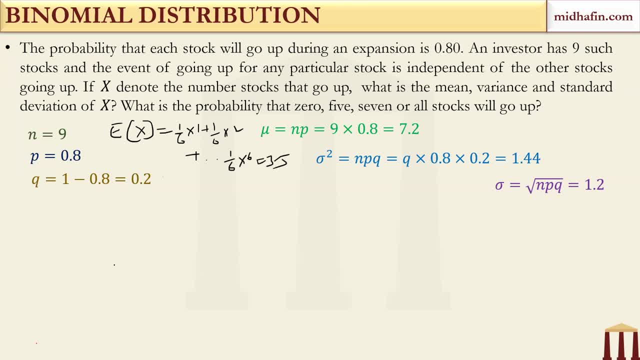 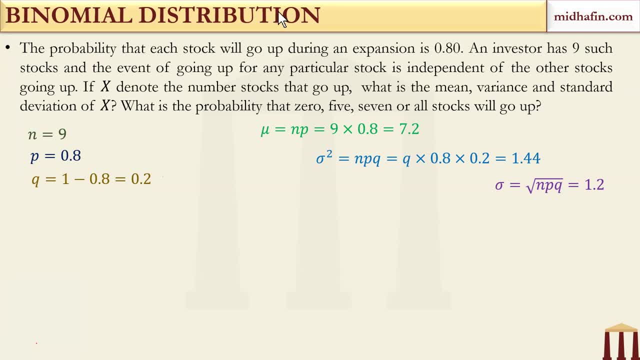 of a die. no, what is the interpretation? interpretation that if you roll the die enough number of times- many number of times say infinite number of time- then the average of all those values will be equal to three. point. similarly over here. okay, in the long run the average value will be seven. okay, 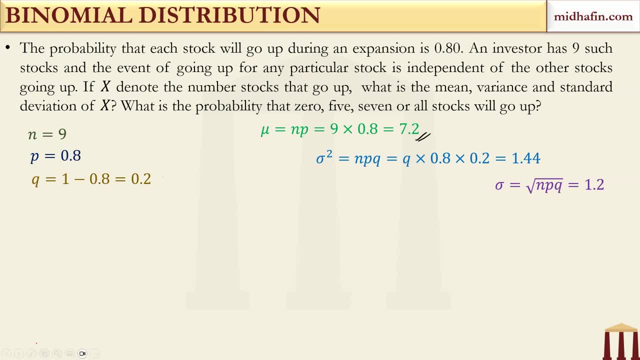 of the number of storms stocks going up. there can be another interpretation also. I'll tell you when I calculate. so tell me one thing: you can have zero stocks going up, one stock going up, two stocks going up, three stocks going up: four, five, six, seven, eight, nine. okay, so there can be ten possible outcomes agreed. 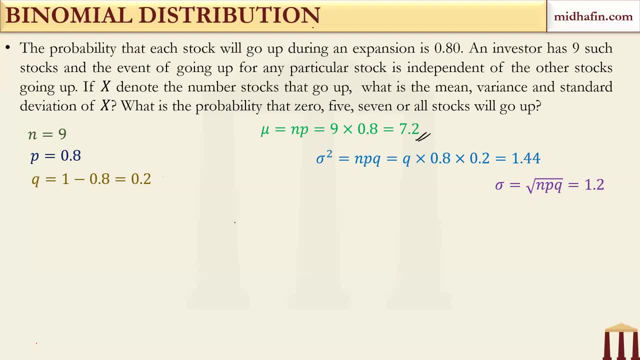 okay. so tell me one thing: what do you think if I find out all these individual probabilities? even how do you form a distribution? you find out all these probabilities and then you map them, okay, where the y-axis is the value of the probability and the x-axis a value of the. 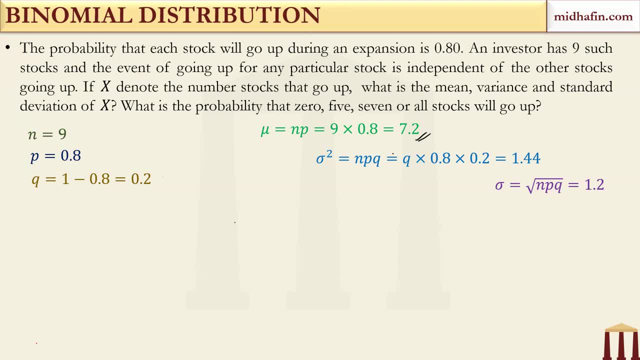 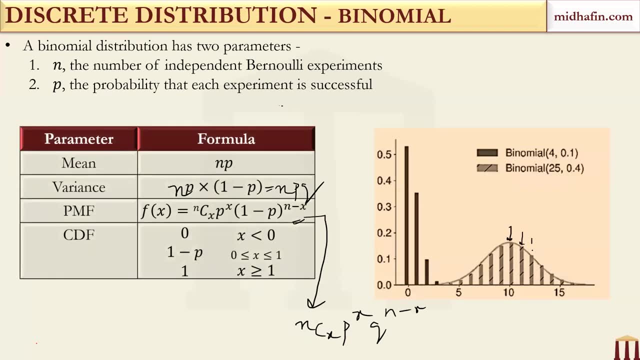 medium. so then you get a distribution just like this. so there are twenty five different probability values over here, times zero, and three- okay, 25- different probability values over here, and these have been mapped. so this is how your distribution is obtained. so that's the difference between distribution and a single probability. 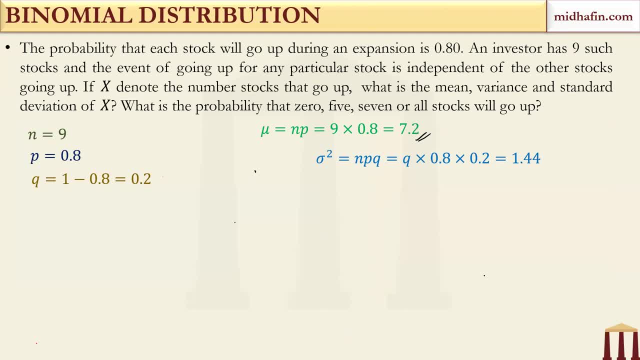 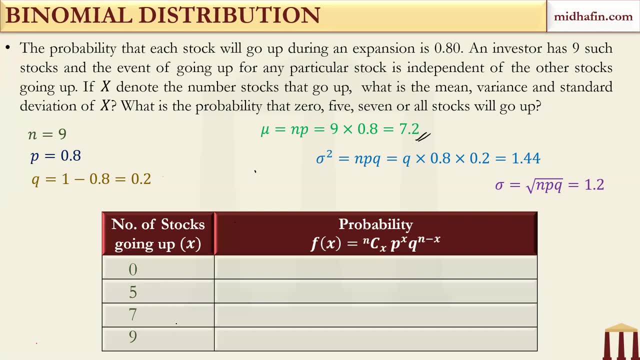 so my question is: if you find out this entire distribution, all the possible values, okay, so let's find out. so we have to find out 0, 5, 7 and 9. what do you think whose probability should be highest? just by looking at this information, can you tell me. see, these are subtle clues, small clues. 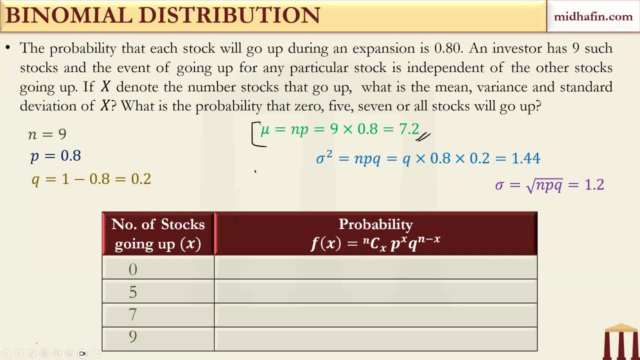 to find out whether you have calculated your answer correct or not. very good again, instead of direct message, please send it to everyone. very good, 7, 7. okay. so this is another interpretation. so even though 7.2 stocks cannot be there, but at least there is a number which is close to 7.2. 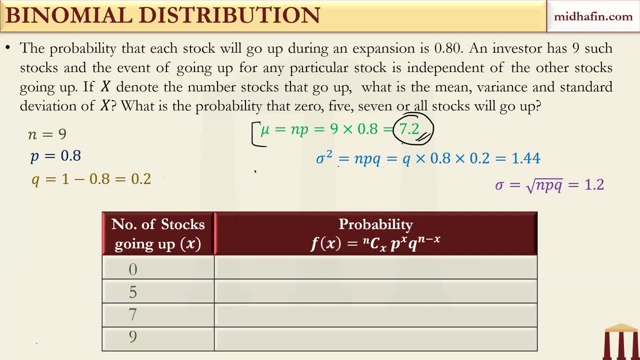 closest is 7.. So we'll have the maximum probability for 7, okay, and the second highest maybe for 8. let's calculate, let's do it for the first one: 9C0 times 0.8 to the positive. so this is a very, very low probability. 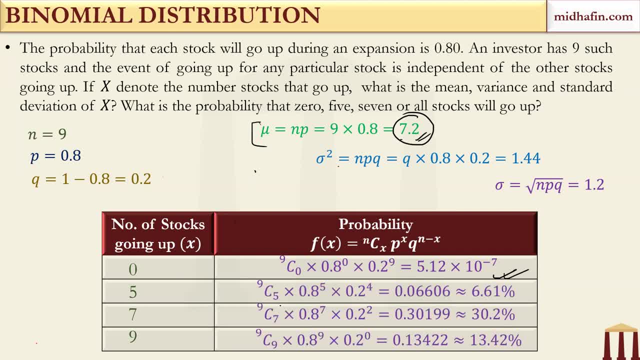 but not 0. similarly, for 5 stocks, 7 stocks and 9 stocks, we have calculated and you can clearly see that for 7 stocks we have a very- you know, I'll not say very, very high, but a very high as compared to others- the highest probability: 30.2 percent. so is the idea clear? 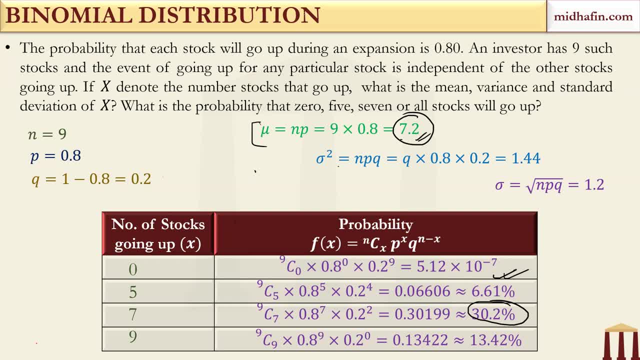 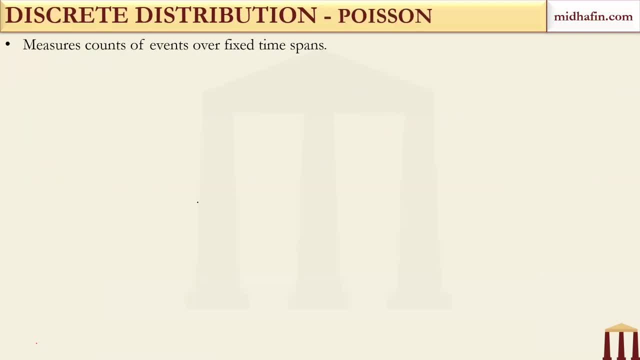 okay, now we have the poison distribution. it measures the counts of events over fixed time spans. so, for example, number of calls in a call center, like that, per minute, something like that. so number of accidents in a road or number of defaults in a month, like that. the random variables are always. 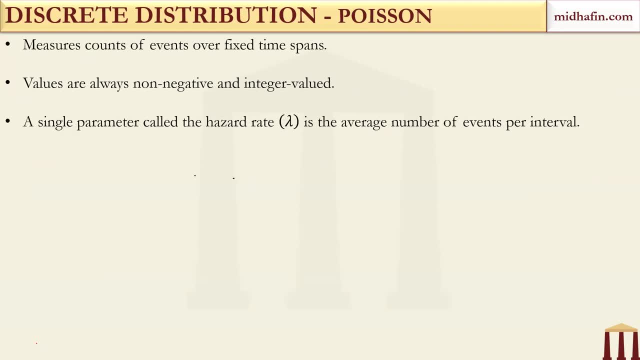 non-int, non-negative and integer valued, and it has a single non-negative and integer value. and it has a single non-negative and integer value. and it has a single parameter called the hazard rate. it is the average number of events per interval. okay, this is the PMF. 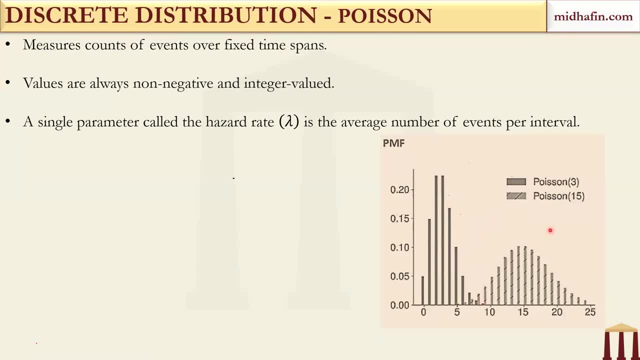 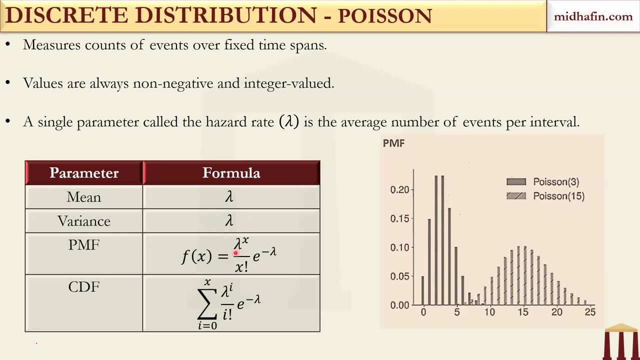 again. you're seeing, I told you, no matter whichever distribution you take, the more number of the parameter values you increase, it tends to get closer and closer to the normal distribution. in this case the parameter is lambda, so the mean of the poison is lambda. the variance is also lambda. PMF is this and CDF of our 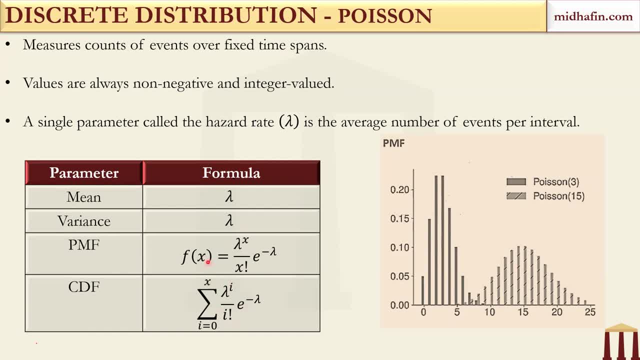 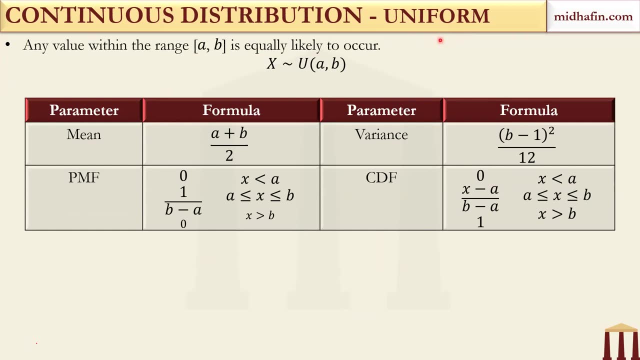 Poisson distribution: is this okay in the class live video and the self-paced video also. we have done some examples based on Poisson distribution also to make the idea more clear. okay, now any value, let's come to a continuous distribution. let's start with uniform distribution. so for a 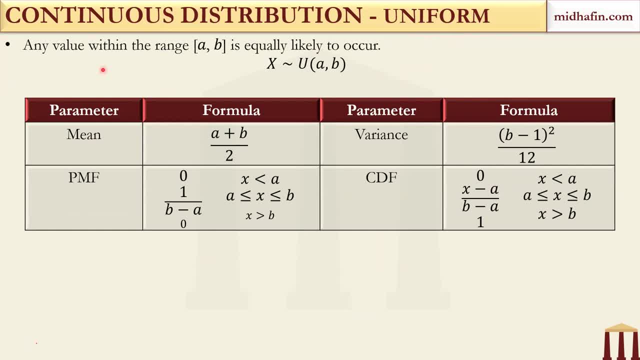 uniform distribution. any value within the range is likely to occur and this is the mean, a plus b by 2. this is the variance, this is the PMF and this is the CDF. now you can remember everything: see mean and variance. you have to remember PMF and CDF. you don't need to remember conceptually. 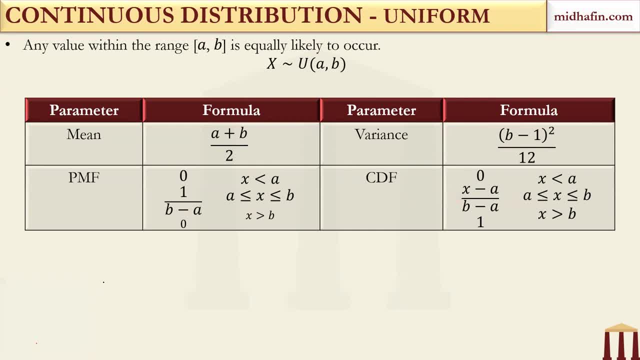 you can understand it quite easily how. when I say uniform, it means any value is equally likely to occur. it means all of them have same probability, correct? so let's say you are having the support is between a and b and you have a, any value is equally likely to occur. it means the PDF will be and in fact there is a mistake over. 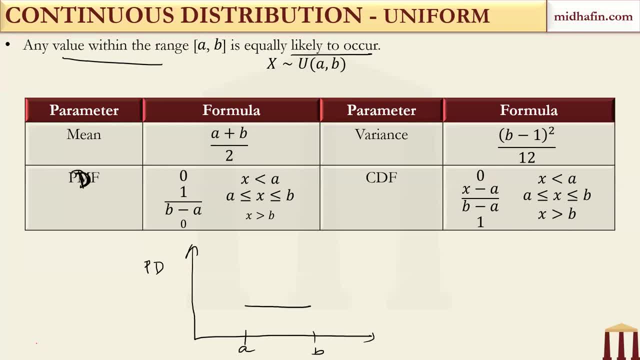 here. it will not be PMF, it will be PDF. why PDF? it's a typo. why PDF? why not PMF? it is continuous, continuous, exactly so these mistakes have to be. in fact, I will expect that you guys there will be. there are any typos. I mean, we had before also there was some typo. 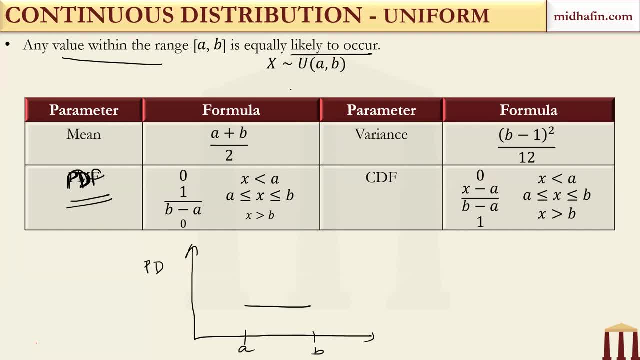 you are spotting it quickly and tell me okay, because this will help you to make your understanding even stronger. so this is PDR. so, since all of the values are equally likely, yes, variance is also. there's a typo- very good, it should be b minus a whole square, correct that? 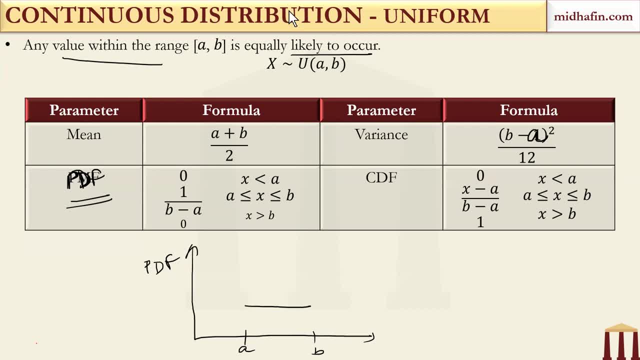 was the video, so there are some typos. wherever you find a typo, please let me. is it correct now? b minus a whole square. yes, okay, so this is the PDF. ok, now tell me one thing. if I want to just reduce this y, it should be 1 by b. the idea is very simple. 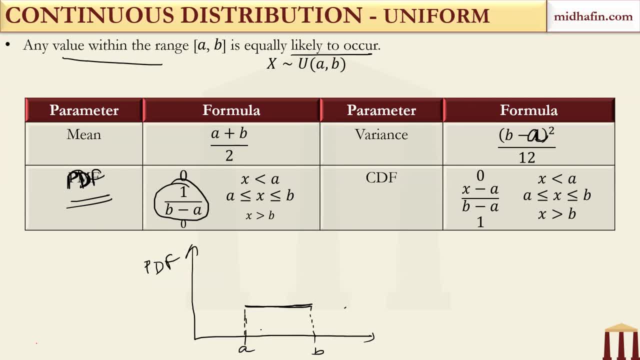 is this a rectangle? is this a rectangle? ok? what is the length of the secondabling edge, traffic- reunions? oh, okay, perfect of this rectangle. What is the length of this rectangle? Correct v-a. And we know that the sum of all probabilities has to be 1.. So the total area should be how much So area. 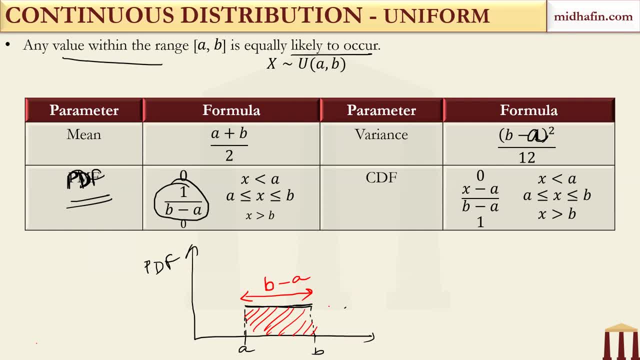 of rectangle should be how much? 1.. So if you know the height you can calculate the area. But if you don't know the height and you know the area, can you calculate the height? Can I say that b-a length times height of this rectangle of breadth? if you want to, 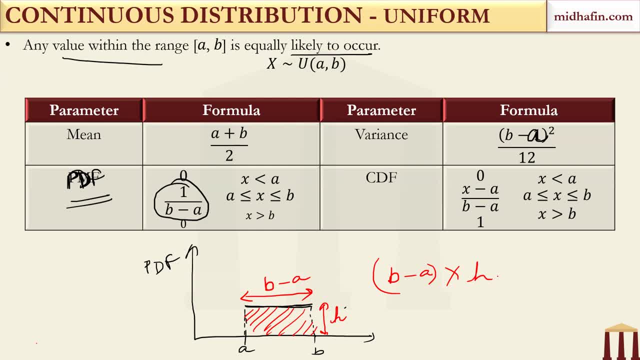 call it. you can call it breadth Height would be better, because we are talking about the PDF values over here vertically. So can I say that this should be equal to 1? Yes or no, Do you agree? The area of the rectangle is always equal to 1.. So what is h? What is? 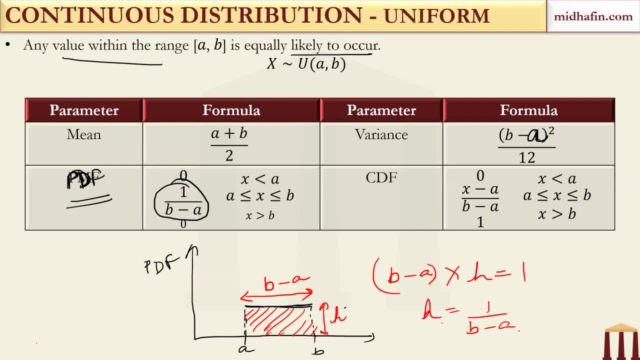 h, 1 over b-a. So this value is nothing but 1 over b-a. So between a and b, that is what is written over here. So between a and b, the PDF is 1 over b-a. Before a and b, the 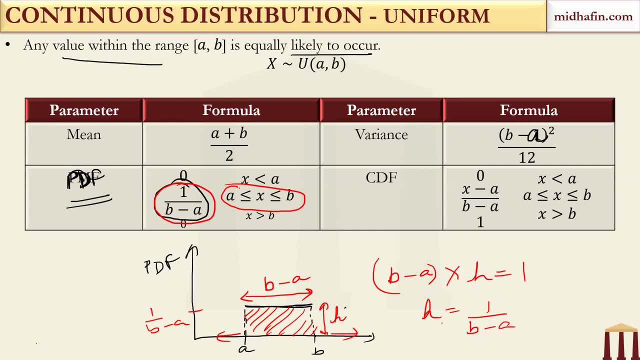 number a, it is 0. After b also, it is 0. So is it clear how to derive it, how to… In fact, the derivation also will not be difficult in the exam. Detailed derivations we are not doing, but these are obvious things. These things we can quite easily interpret in the 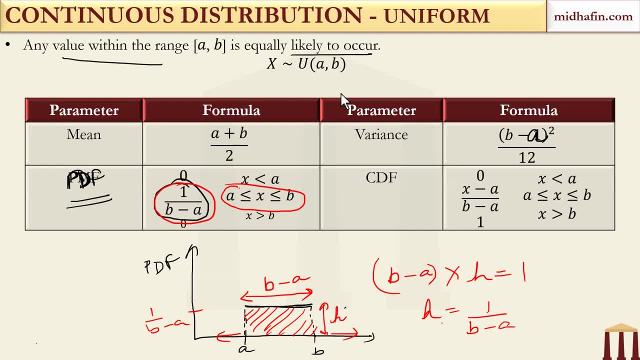 exam rather than remembering the stuff. So if you have a uniform distribution- let's say numbers are given to you- then it will become even easier. You just remember that the total area should be equal to 1. And these are figures for which area can be easily calculated. 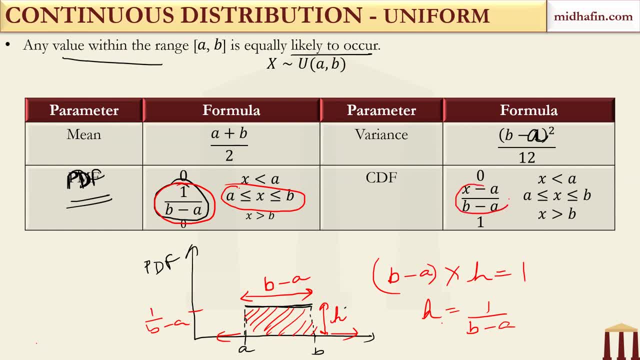 Similarly over here, x minus a by b minus a. This also can be quite easily interpreted and derived quite easily. So if x is any value over here between a and b, and CDF means what CDF means from the minimum value up to x. So what is the minimum value over here? 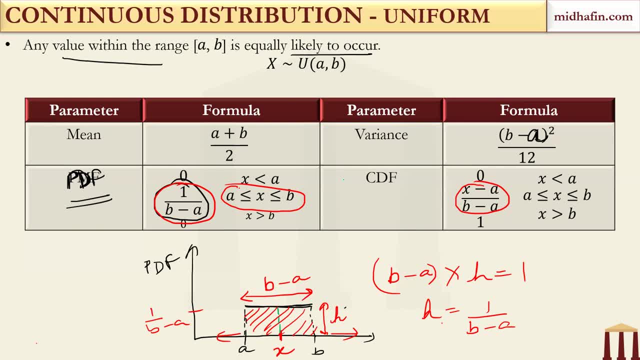 a correct. So up to x. It means you have to calculate this area, agreed or not. for CDF, For a particular value of x, you have to calculate the green area, agreed or not. What is the length of this rectangle? x minus a? You have already calculated the height. 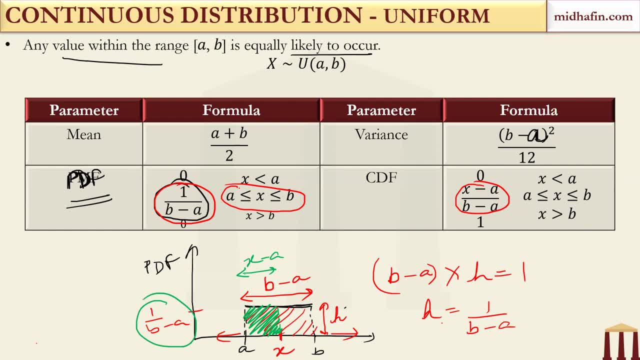 of this rectangle Correct? So if you multiply length by height, will you get this, Yes or no? Is the CDF clear To everyone? everyone should answer this. If there is any doubt, please ask. Okay, so this is how you have to interpret these things, quite simply, in the exams. 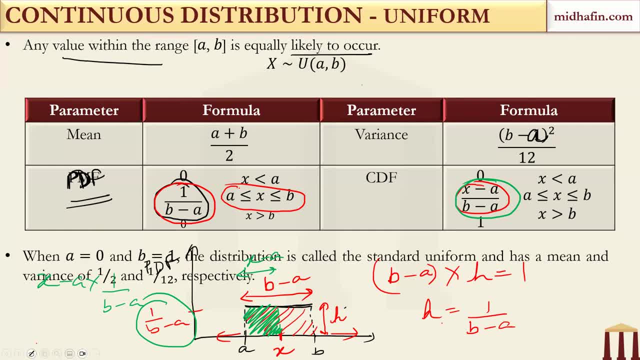 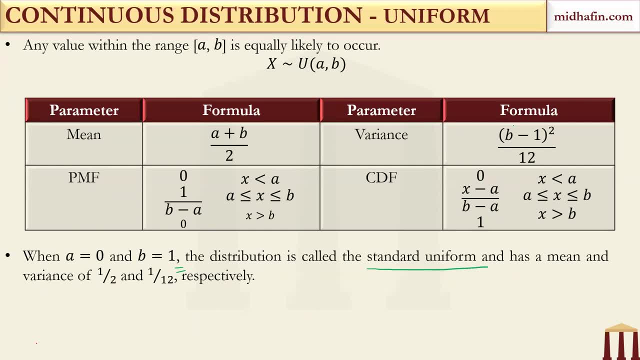 Okay Now, if a is 0 and b is 1, then it is known as the standard uniform distribution And, as I said, this will be a which has a mean and variance of half and 1 over 12.. So 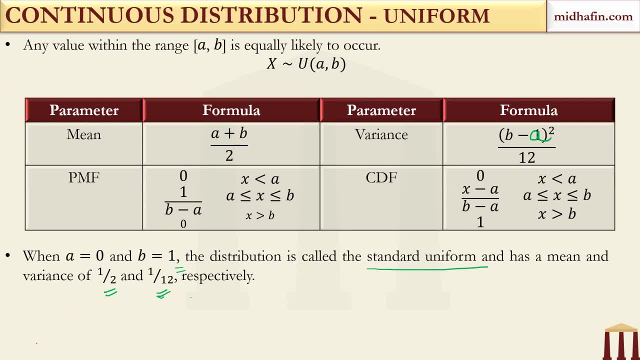 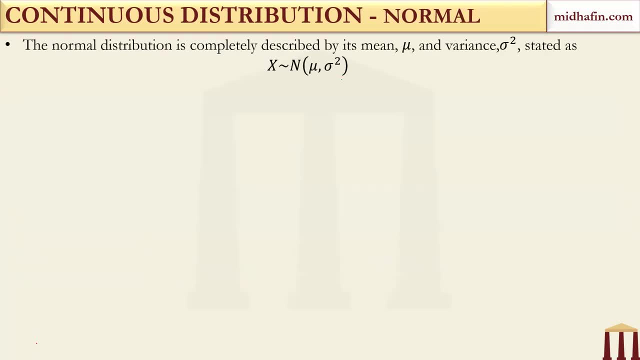 obviously, if a is 0 and b is 1, then 0 plus 1 by 2 half variance will be 1 over 12.. Now let us come to one of the most important distributions that we have to do: normal distribution. So 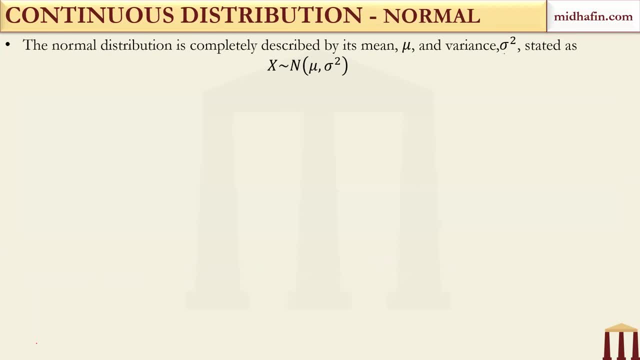 it is completely described by its mean mu and variance sigma square. This is how we write it. Expected value is mu. variance is sigma square. What is the skewness of this distribution? What is the skewness of this distribution Zero? 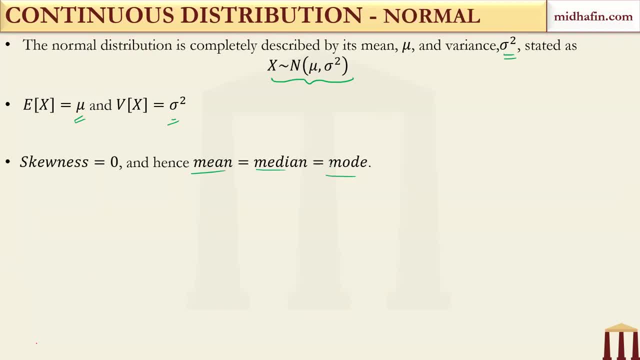 Very good, zero. So can I say that mean equal to median, equal to mode? Okay, And what will be the kurtosis of this distribution Three? What is the kurtosis? Very good, three. Excess kurtosis was zero, correct? 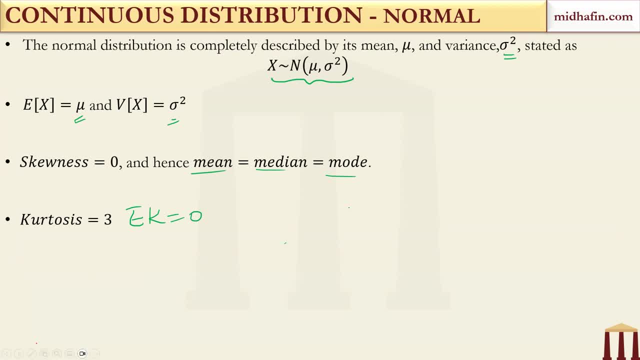 Now one point which is very important from the point of view of the exam, which, again, is overlooked over here sometimes, because this part, though, everyone knows. But what about if there are two normally distributed variables, x1 and x2? Both are having different. 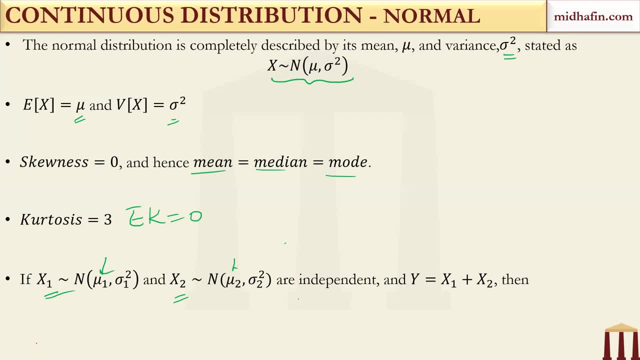 means and different variances. If these normally distributed variables, if they are independent of each other- this question was directly asked in the exam. directly- If they are independent of each other and you construct a third variable, y, which is the sum of these two normally distributed variables, then you can easily prove that. 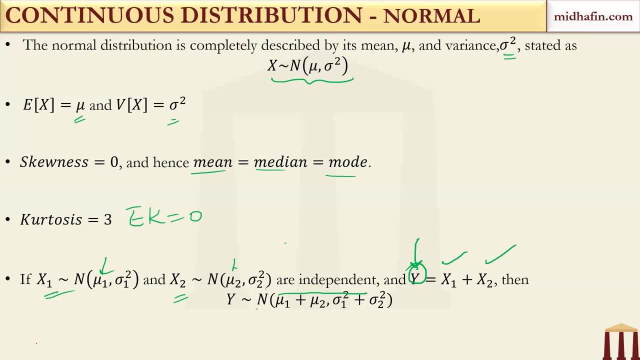 this new variable y will also be normally distributed with the mean of mu1 plus mu2 and variance of sigma1 square plus sigma2 square. Very important point, okay for the exam perspective. Is it clear? Is the last point clear, Not the derivation, Will you? 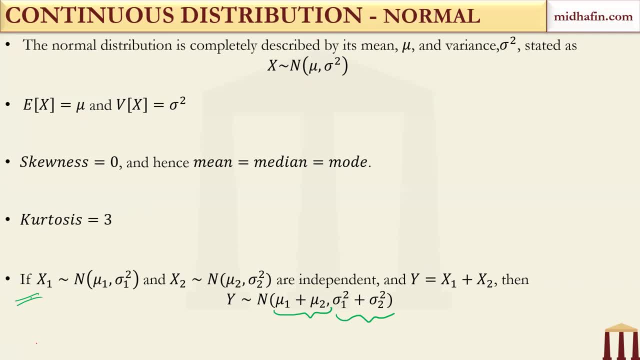 be able to remember this. If there are two independent, normally distributed, random variables, then the sum of those variables is also normally distributed, with the mean of mu1 plus mu2 and variance of sigma1 square plus sigma2 square. Okay, And this is how a normal distribution 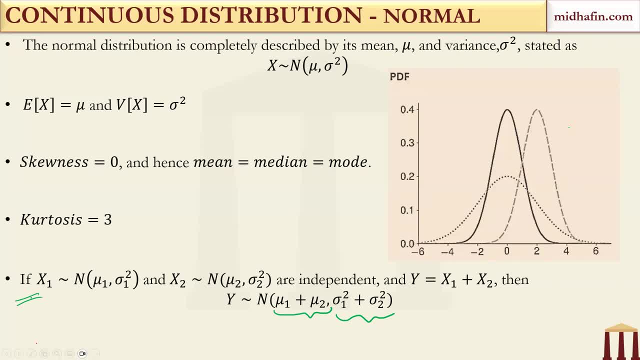 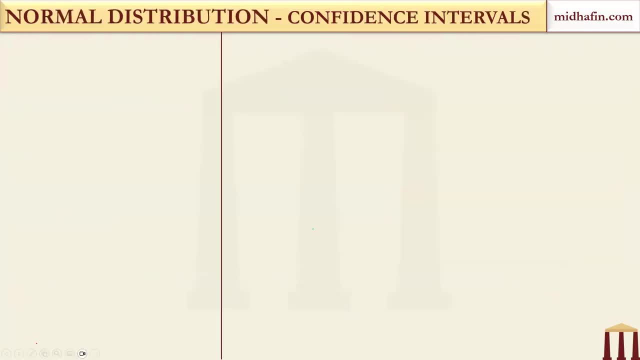 looks like for different values of mu and sigma. Okay, and how will the CDF look like? CDF will always be a non-decreasing function like this. Okay, now let's come to confidence intervals. We have four confidence intervals which are very important. We have 68% confidence interval: mu minus sigma to mu plus sigma. We have 90%. 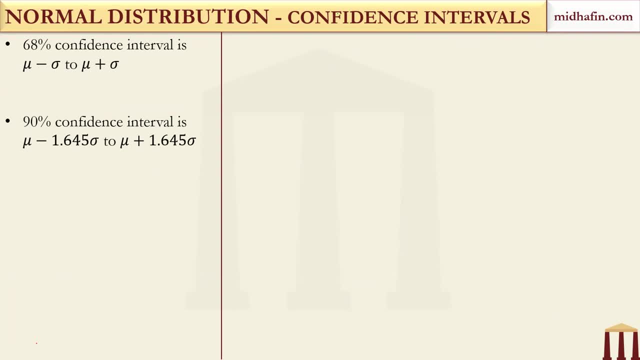 confidence interval: mu minus 1.645 sigma to mu plus 1.645 sigma. We have 95% confidence interval- mu minus 1.96 sigma to mu plus 1.96 sigma Understand and 6 sigma and we have 99 percent confidence interval. So the meaning basically of this: 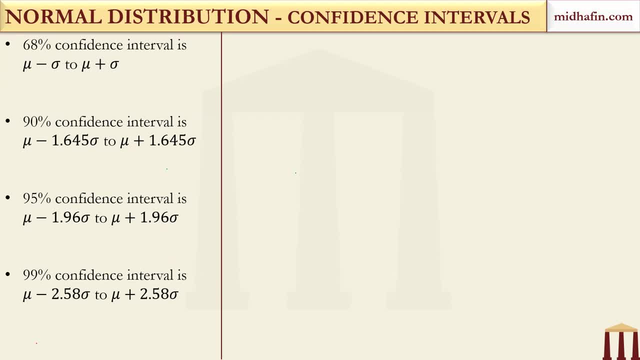 confidence interval, layman interpretation. again, I am saying not the theoretical correct interpretation, because the theoretical correct interpretation is quite detailed. The layman interpretation is that if suppose you are talking about, say, 90 percent confidence interval, it means that you can be reasonably confident that 90 percent of your observations 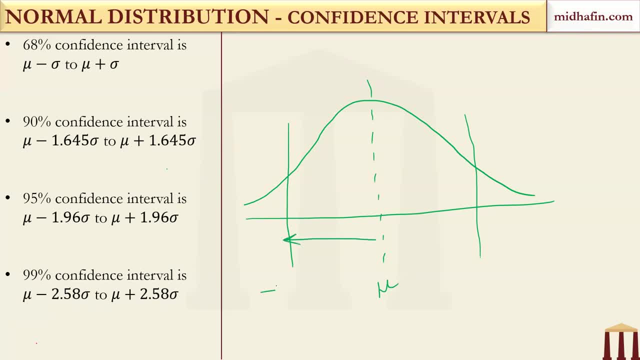 are between these two values: mu minus 1.645 sigma and mu plus 1.645 sigma. So this area contains 90 percent of your observations. Similarly for the other confidence intervals. That was the interpretation, layman interpretation, not the correct interpretation. Again, I am. 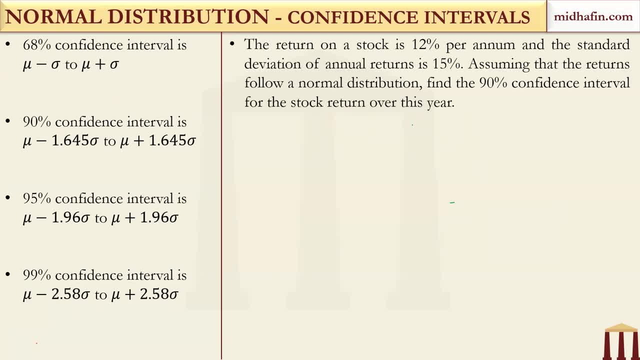 repeating. So let us solve an example. The return on a stock is 12 percent Per annum And the standard deviation of annual return is 15 percent. Assume that the returns follow a normal distribution, find the 90 percent confidence interval. So 90 percent is from mu. 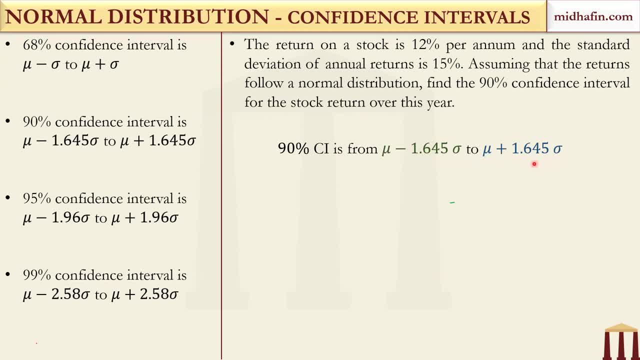 minus 1.645 sigma to mu, plus 1.645 sigma, which is 12 percent minus this times this. So you get straightforward answers. You can be 90 percent confident that your returns under these conditions, your annual returns, will be between negative. 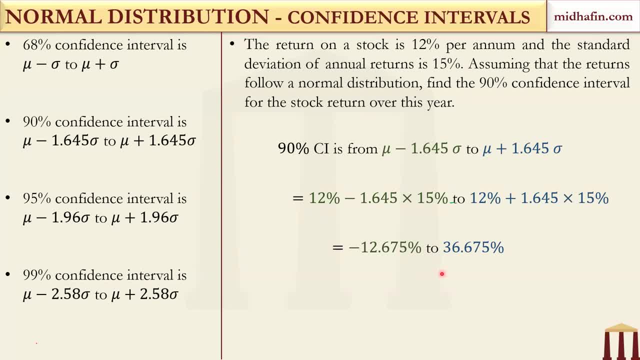 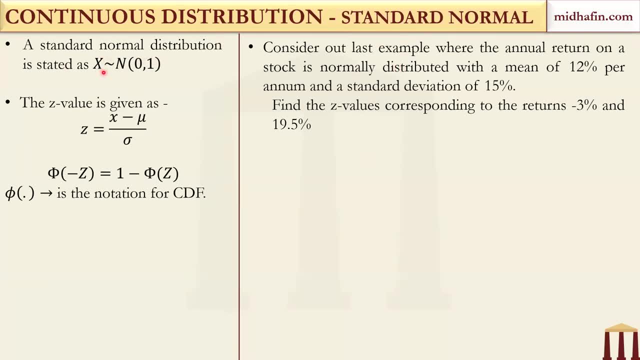 12.675 to positive 36.675 percent. Now let us do standard normal. So standard normal distribution is stated like this: It has a mean of 0 and variance of 1.. And this is the Z value which we actually map for the standard normal. 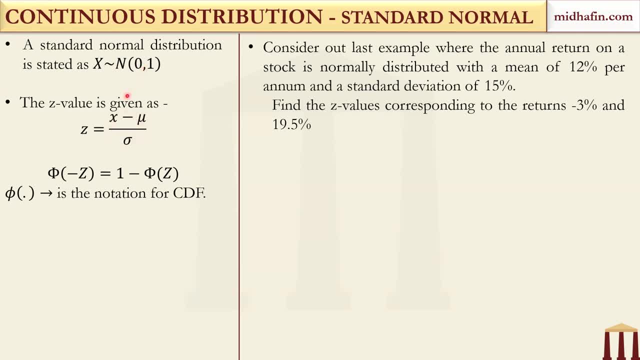 distribution. Now, I told you remember earlier that this is also the standard normal distribution. Now, I told you remember earlier that this is also the standard normal distribution, a standardized version of any random variable, and this has a mean of 0 and variance of 1,. 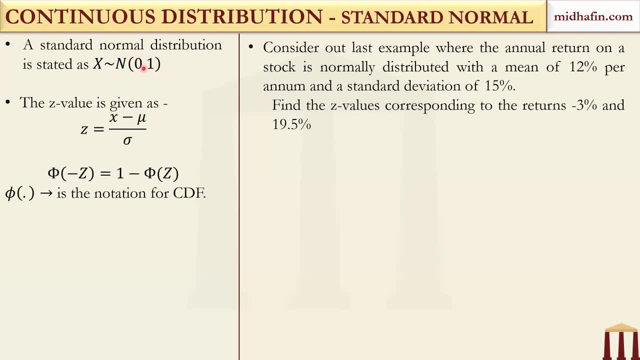 standard deviation also of 1.. So the same thing follows here. This can easily be proved that it has a mean of 0 and variance of 1.. So remember, this is the Z value. this is the standard normal distribution. See in the class we have in fact for only multivariate random variables for probability. 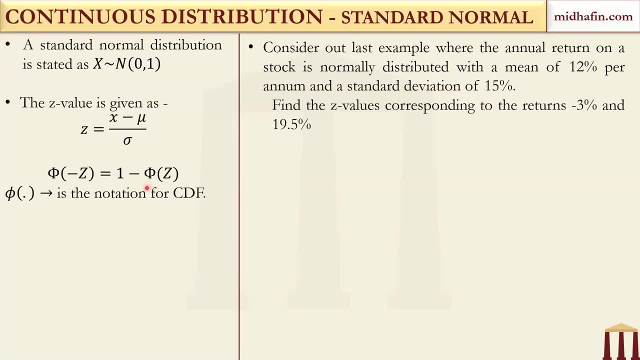 we have three and a half hours, four hours of video for one chapter. So we are trying to cover these things in 30 minutes to one hour. So that is why we are actually rushing. But again, I am repeating, I am assuming for those who have joined late. I am assuming. 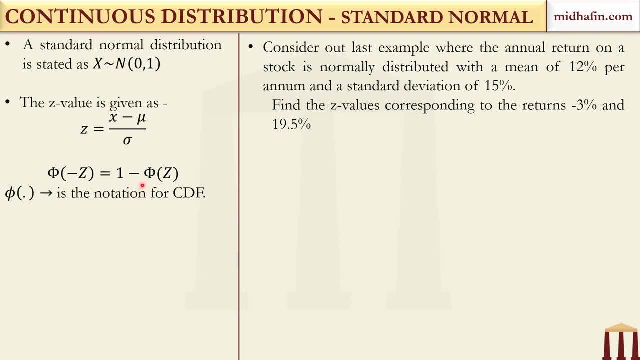 that you are already through with the course at least once, and this is just a revision session for you. Now, this last part: phi negative Z is equal to 1 minus phi Z. This is a property which uses the symmetricity of the normal distribution, the symmetrical 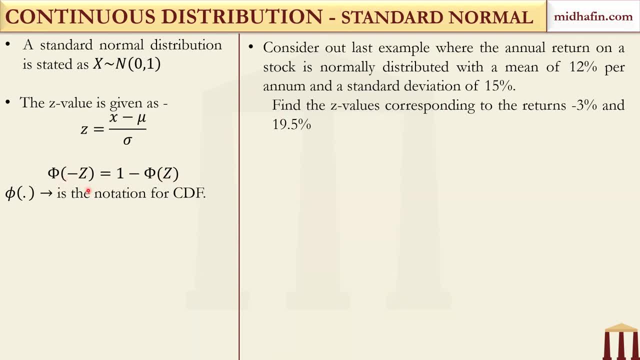 properties of the normal distribution And can you tell me where this is utilized heavily, this property, when this will be helpful for you in the future? When will this be helpful for you in the exam? When you will be given a Z table? let's say you are given a Z table which does not contain. 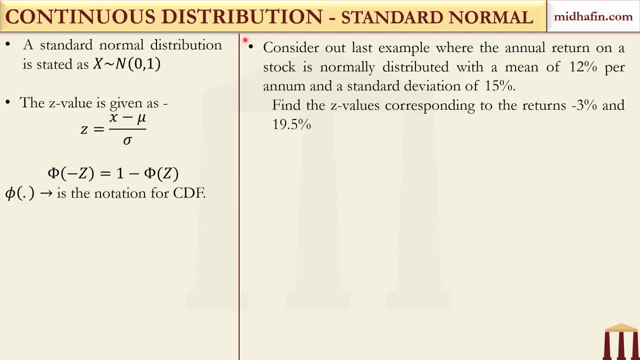 any negative values And you have to find out the phi values corresponding to the lower tail, correct, Shashank? So this property, you see, if you directly have a Z table where you can find out the phi value directly, okay then there is no problem. 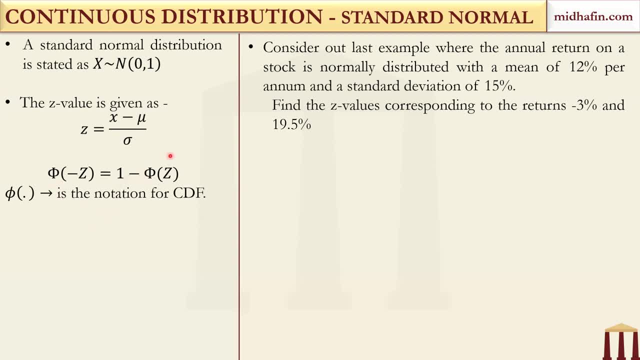 But what if you don't have it? Then you use the positive values only And you apply the symmetric properties of the normal distribution. okay, So consider our last example, where the annual return on a stock is normally distributed with the mean of 12% per annum, standard deviation 15, same examples. 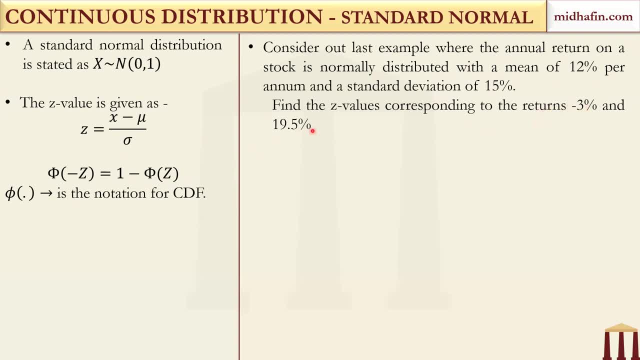 What will be the Z value corresponding to negative 3 and 19.5%? So first case I said X is negative 3, Z value will be negative 1.. So what does it mean? It means that- listen to this very carefully, the interpretation. 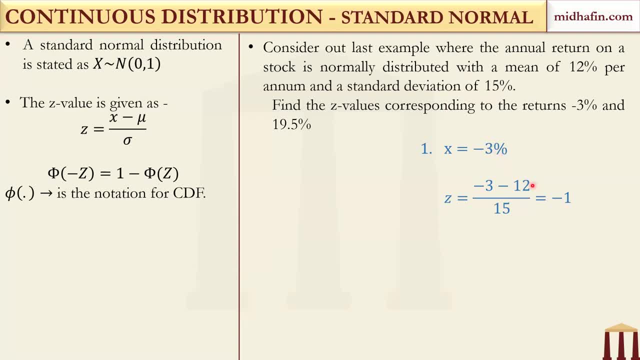 It means that negative 3% is one standard deviation away from the mean, which is 12% on the left-hand side, because it is having a negative sign. okay, So this negative 3, when you compare it in terms of distance, okay, this is 12%, I'm. 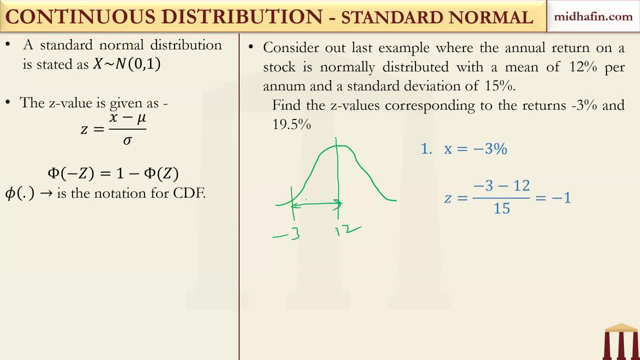 not writing percent over here. Okay. So distance, if you compare this, distance is one standard deviation. So this is basically the meaning of Z value. It tells you how many standard deviations away and observation is away from the mean and on which side. okay, 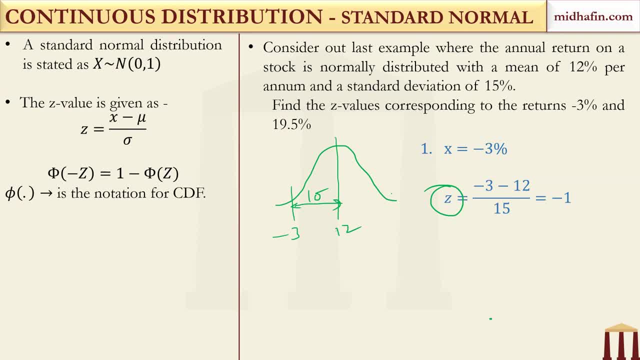 That is the interpretation of Z value. How many standard deviations are there? Similarly for 19.5, can anyone tell me how many standard deviations away you are getting? You solve this quickly. quickly, because it's very simple. What is the Z value corresponding to 19.5?? 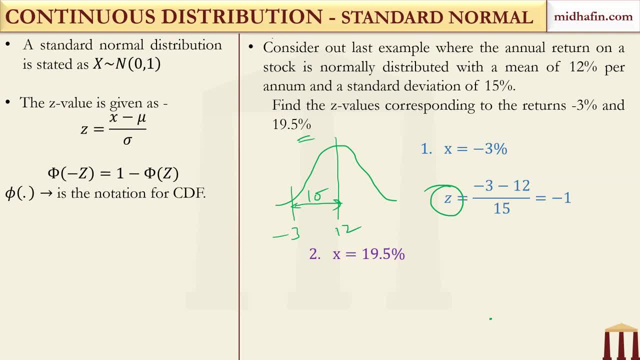 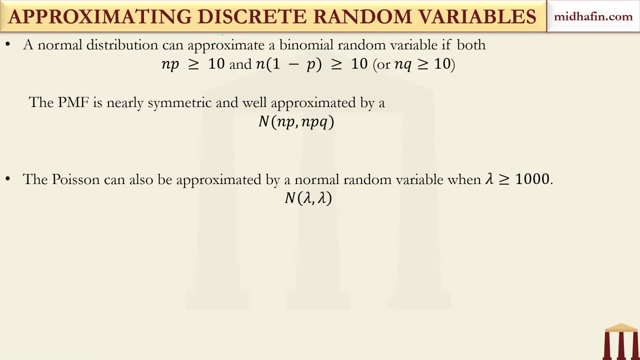 Very good, 0.5.. So 19.5 is 0.5 standard deviations away from the mean of 12% on the right-hand side. okay, That is the interpretation. Now if suppose you want to approximate discrete random variables to normal distribution. 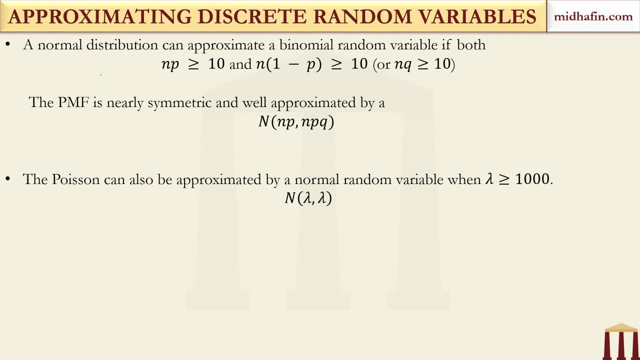 So there are some conditions. One is for binomial, the other one is for Poisson, So for a binomial random variable. if both these conditions are satisfied, Np is greater than equal to 10, Npq- you should write Np, yeah. 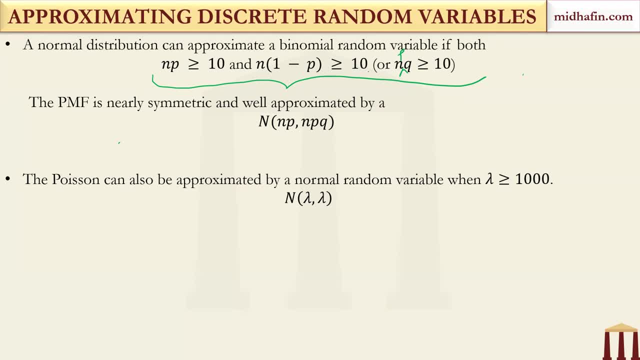 If Np is greater than equal to 10, in fact there was a condition for Npq also, There is a condition for Npq also, So Npq should be also greater than equal to 10 actually. then it makes a better distribution. 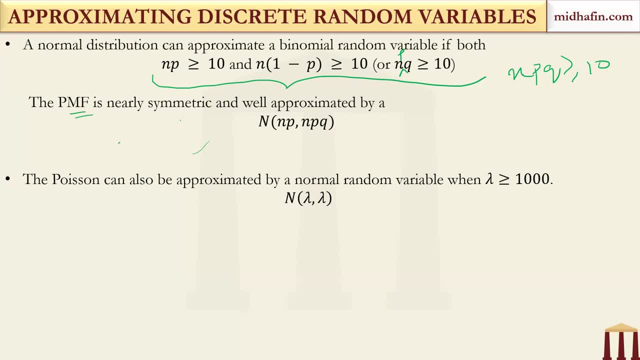 okay. Now the PMF is nearly symmetric and well approximated by this. in that case, It means you will get a normal distribution with a mean of Np and variance of Npq. okay, But these two conditions are more important: Np is greater than equal to 10 and Nq is also greater than equal to 10.. 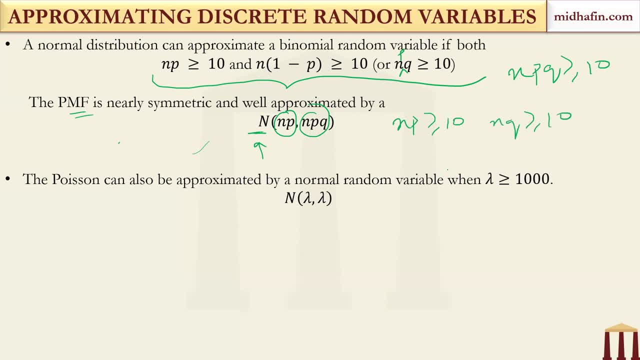 So this is the distribution. Okay, Thank you. And in some literature, as I said, you will find some conditions with respect to Npq also. In fact, Npq is greater than equal to 5 is also acceptable sometimes, okay. 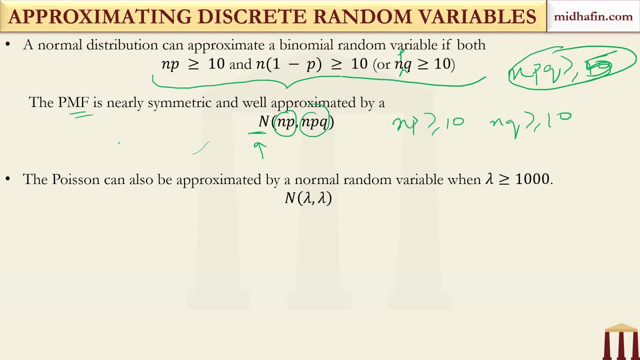 So if these conditions are satisfied, a binomial distribution can be approximated to a normal distribution. Also, a Poisson distribution can be approximated by a normal random variable where lambda is greater than equal to 1000. In that case you will get a normal distribution with a mean of lambda and variance of Np. 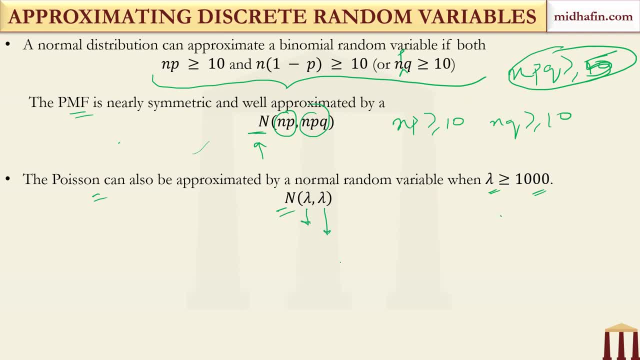 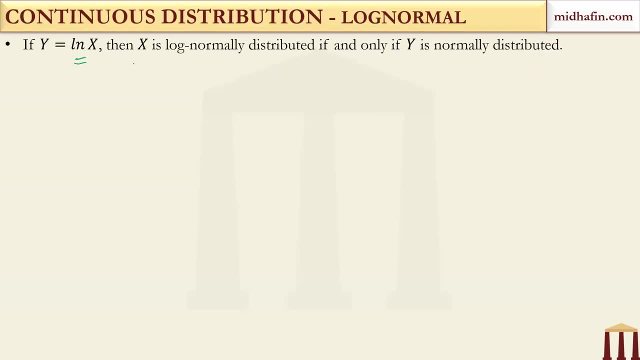 Okay, So if these conditions are satisfied, a binomial distribution can be approximated to a normal distribution. Now, log-normal distribution. If suppose y is equal to lnx, then x is log-normally distributed, if y is normally distributed. So if suppose y is defined as natural log of x and if y is normally distributed, then 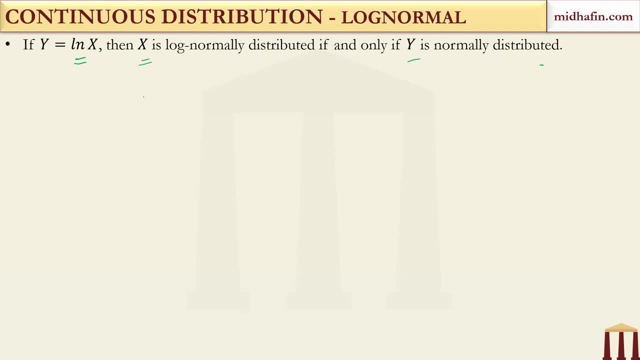 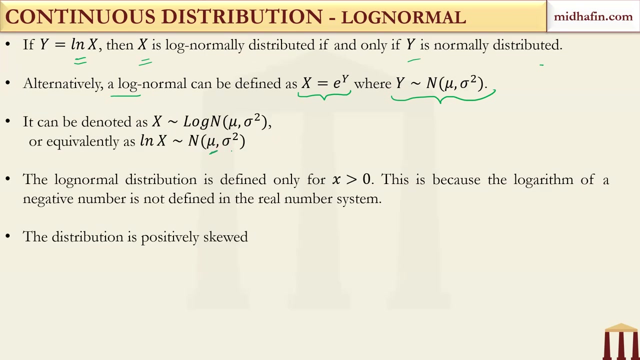 we will say that x is log-normally distributed. There is an other way to define it. Alternatively, a log-normal distribution can be defined like this: x is equal to e, raise to the power y, Where, Where the matrix y is. 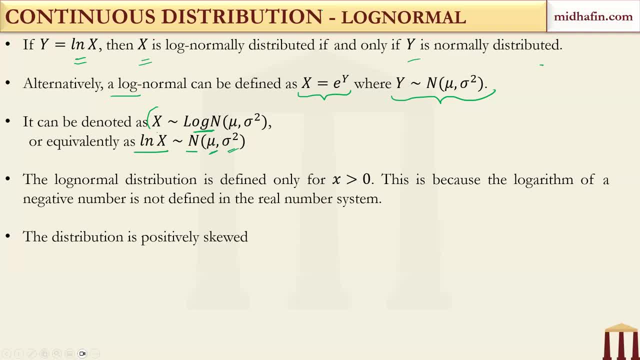 of x. So in that case we can calculate log of x. That'sGood, Let's For ger. log normally distributed means log of x is normally distributed, and over here by log I mean natural log. Now log, normal distribution. you all know that it is only defined for x greater than. 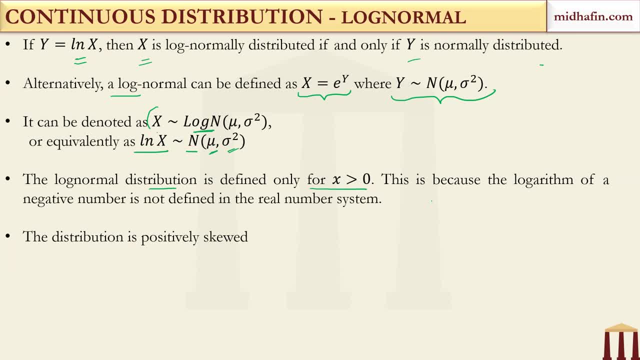 0. So it does not take negative values. it is not defined for negative values for of x. This is because logarithm of a negative number is not defined in the real number system. Can you tell me a good part about this property, a practical application of this property? Which instruments? 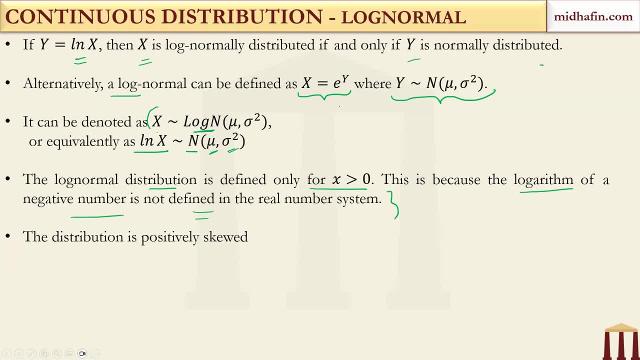 which financial instruments Prices can be log normal, Your voice is not very clear. Prices, Prices, Perfect. So yeah, Divesh has mentioned. Divesh notes, not stock returns, Stock prices, because returns can be negative also right, Got it. But prices cannot be negative, Correct Again, this is also a question, a very easy question. 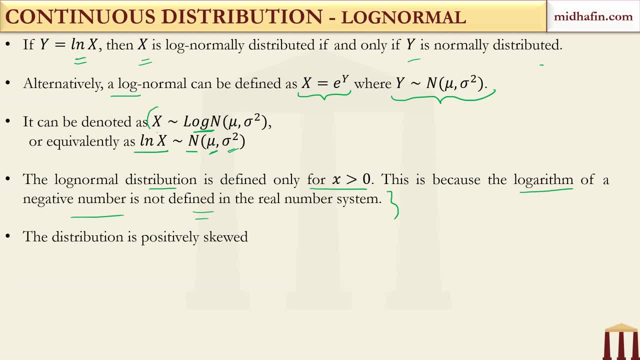 which has been asked, not recently, but in 2015-16. this question was asked two, three times continuously because the GARP has this tendency of earlier. in fact, they had this heavy tendency of repeating questions, at least eight or ten In fact. I'll also give some good news over here. 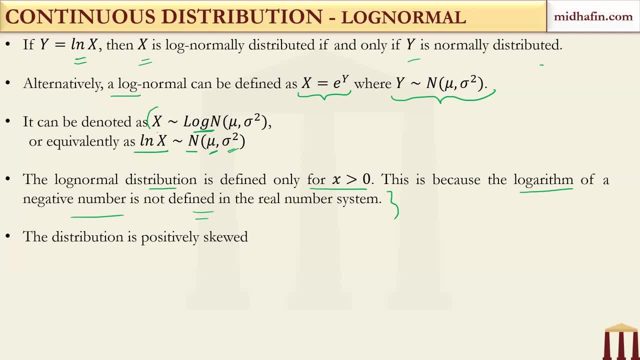 with respect to sample Sample papers. if you have gotten access to the 2024 sample papers in your GARP dashboard in your portal, then there is a good chance that at least eight questions will be almost similar to what are given in the sample paper- questions almost or even identical. When I say almost, they might just 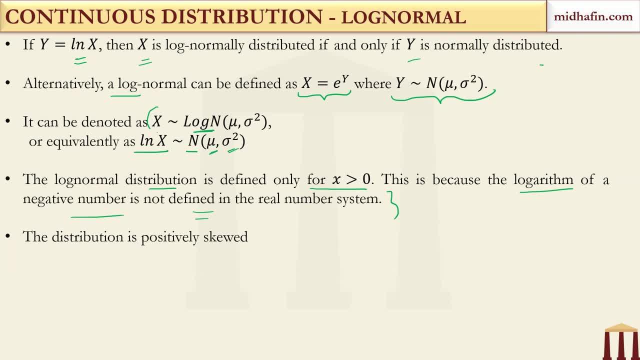 change the numbers a little bit, tweak it a little bit, but more or less you will find that eight questions will almost match. So practice the sample papers. yes, yes, including both notes. yes, Including both. at least, I am saying at least. so if this batch is lucky, then maybe 10,, 12,, 15, who knows? 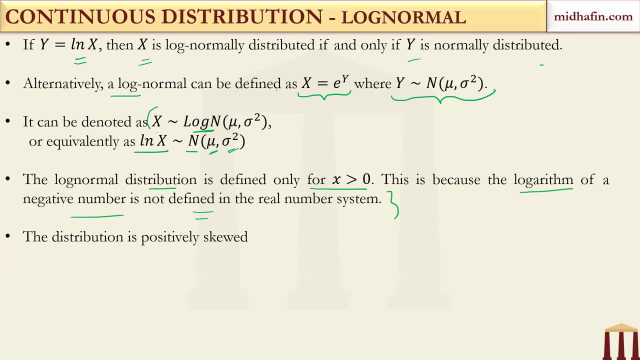 but practice them properly. okay, because they are a very good reflection of what is going to be not exactly tested. but how GARP is, you know, changing the pattern towards more theoretical questions or conceptual questions, what they intend to ask this year. Okay, so practice the sample paper questions without fail. 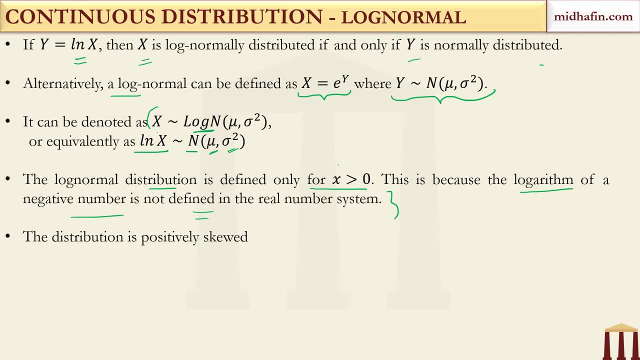 So the application of this problem is very simple. So the application of this problem is very simple. So the application of this problem is very simple. The property is that it is very useful to model stock prices. Yes, Rohit, see, actually we give our candidates the past sample paper questions of the last 15 years. 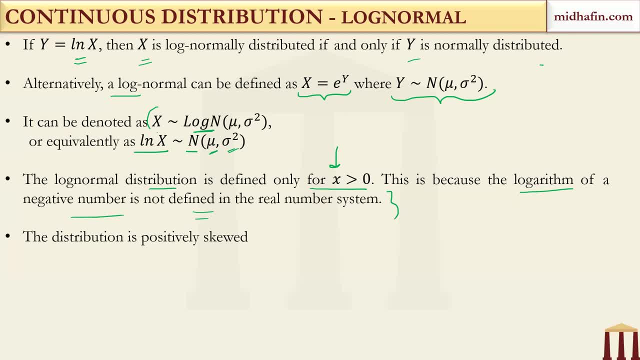 and we don't just give them as pdfs. no, we have actually taken a lot of time and we have filtered those questions, module wise, and we have omitted the questions which are not relevant from the current syllabus point of view, module wise, we have filtered so that you can get everything in one place. 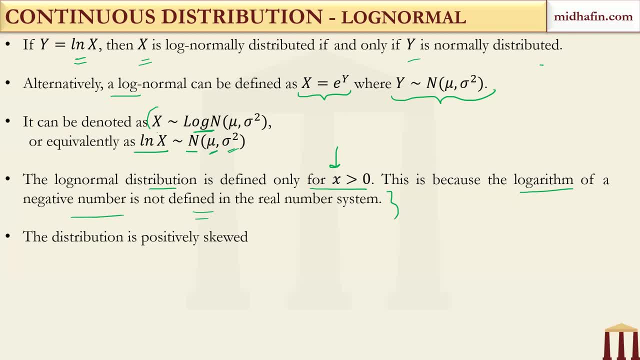 Okay, and mapping is very important. Yes, mapping according to the learning objective also has been done and if there are some mistakes, also in the solutions, yes. so instead of last five years, Rohit, don't solve this pdf separately. use our that the main known pdfs for the past samples of the 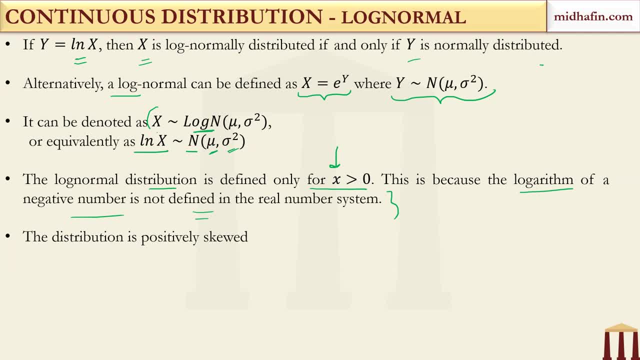 question. that's what i'll say and of course, there might be a little bit some, or maybe once in, say, 100 pages or once in 50 pages. there might be some typos, notify us, but use them on the which we have provided. Okay, But for current year papers- 2024, that you can use it from. 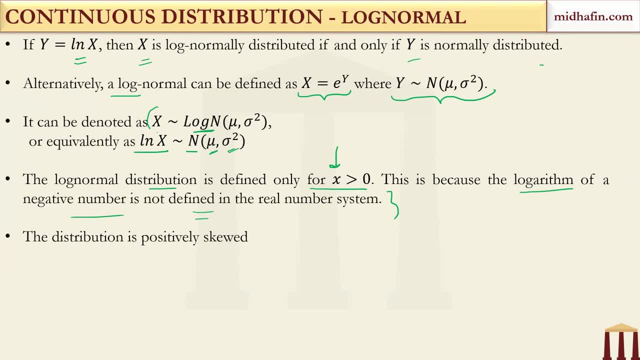 the GARB cash paper. So that would be advisable. Okay, So the distribution is positively skewed. So log normal distribution is actually positively skewed. It has a long right tail, So there are outliers on the right hand side. Then chi-square distribution. they are defined. again the details: 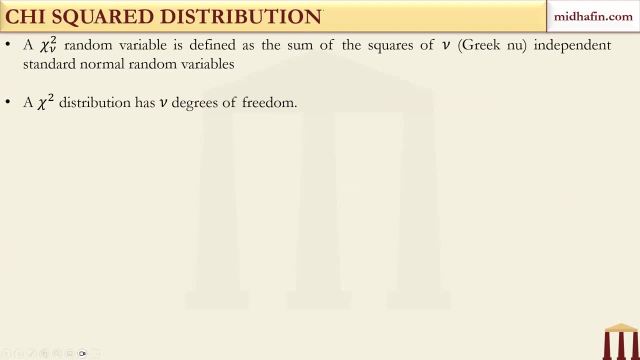 of these distributions were there earlier, prior to the 2020 curriculum. Since 2020, the details have been omitted. In fact, in hypothesis testing, even the chi-square test, F test, were discussed extensively, which has been omitted now from the syllabus. Now, a very basic intro has been given. 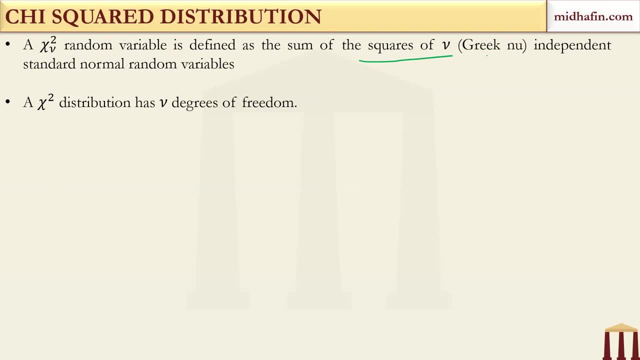 Chi-square is defined as the sum of squares of new, independent, standard, normal, random variables. Sum of squares. Remember how is chi-square defined? Sum of square of normal variables: Okay, It has new degrees of freedom. This is how it looks like, And this is sorry. this is how it looks like. 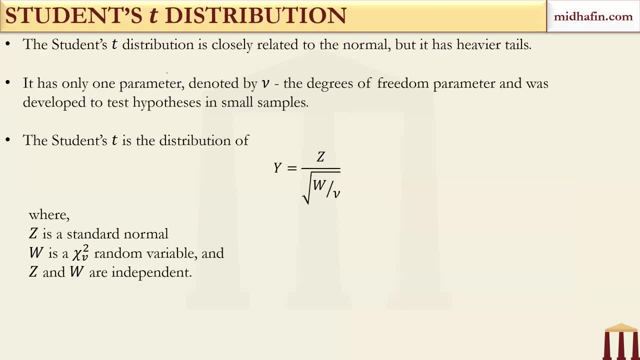 That's it. That is what you have to cover in chi-square, nothing more than Then. T distribution is closely related to the normal distribution, but it has heavier tails. Okay, Now one thing which I think is not very clear in the GARB curriculum- and they have asked questions also- 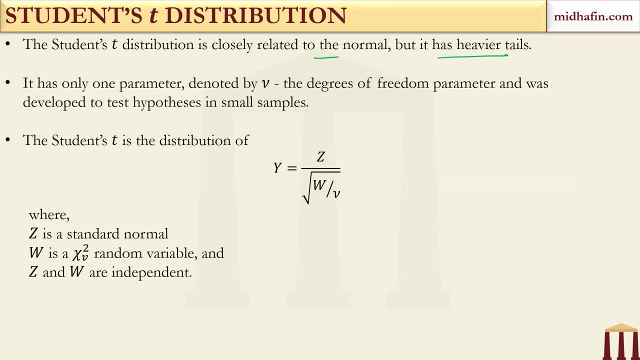 and it might be incorrect, but that is what you have to choose in the exam. Let's say, they give you leptokurtic distribution and you find that T distribution is the only option which has heavier tails. So you'll obviously you'll have to choose the T distribution, right? So T distribution is. 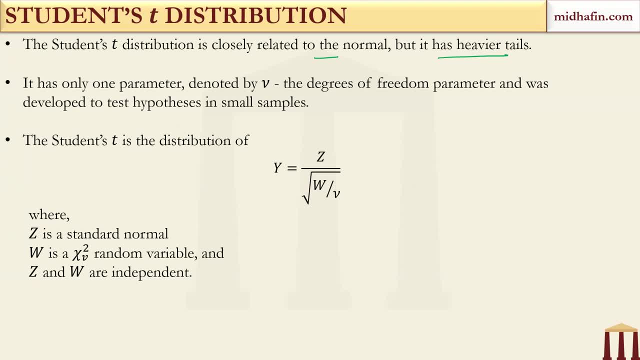 leptokurtic, But there is still a debate with respect to T distribution, although it has heavier tails. but what about the central region? Okay, But mostly T distribution is also having a higher central region. So you can safely say in the exam, even if it's not a hundred percent correct, but 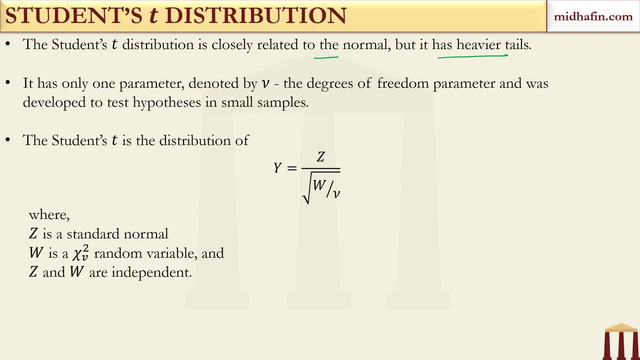 for most of the cases, T distribution is a leptokurtic distribution. That is what you have to assume for the exam point of view. So it has one parameter again, and it is a distribution. of Y is equal to Z divided by square. 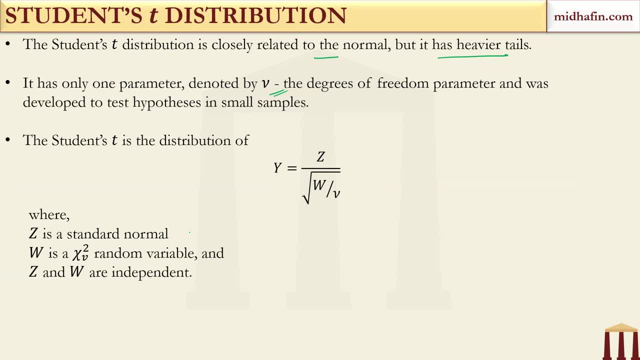 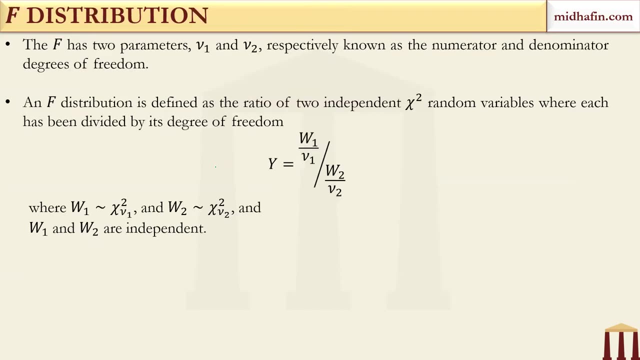 root of W by nu. Where Z is a standard normal, W is a chi-square, random variable. Z and W are independent. Generally, I have not seen questions based on T distribution, chi-square distribution and this is how it looks like, Okay, And F distribution in the past few years, Okay. 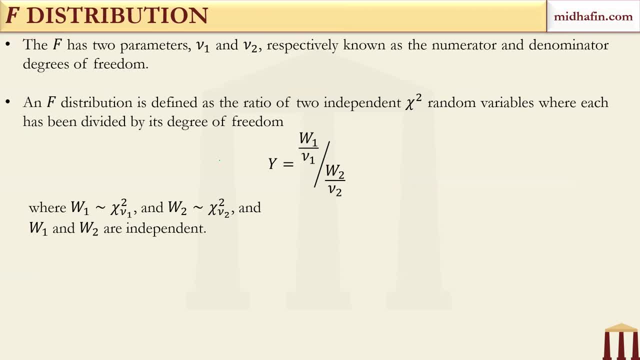 Generally, in the last two, three years I have not seen questions based on T distribution and even the candidates have not given any feedback that these kinds of questions were asked in the exam. So this part you can just go through the PDF that we'll provide you, Okay. 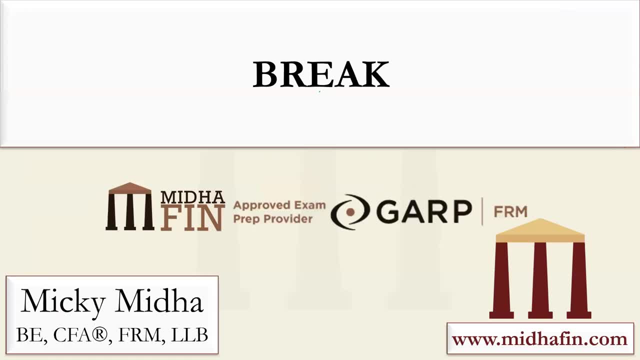 So okay. So that's it for the first three chapters. Let's take a break right now and we can resume in 20 minutes, Is that okay? At 2.10.. As I said, we'll take four long breaks and 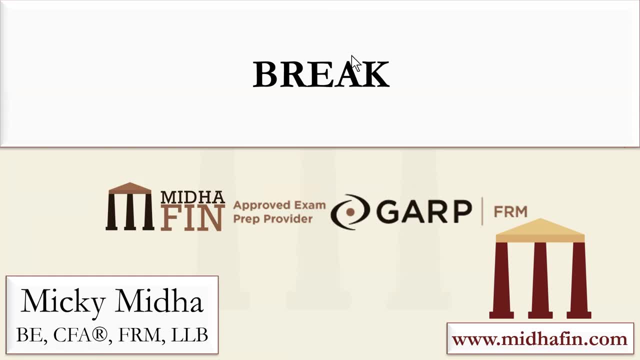 some short breaks, five minutes each, Okay, So 20 minutes break. have your lunch Be back by 2.10 PM. Okay, Now, this time what I'll do I'll with respect to recording. okay, if we are having 20 minutes. Okay, So I'll resume the recording later on, Right, No problem. 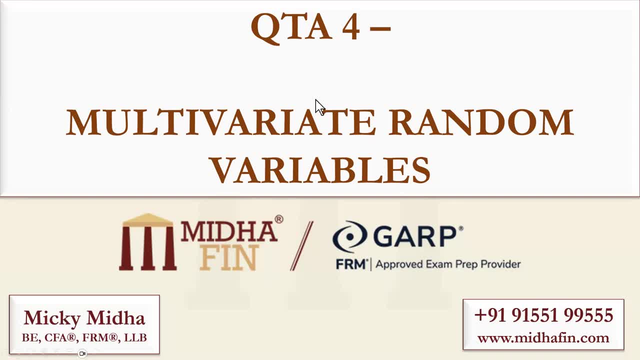 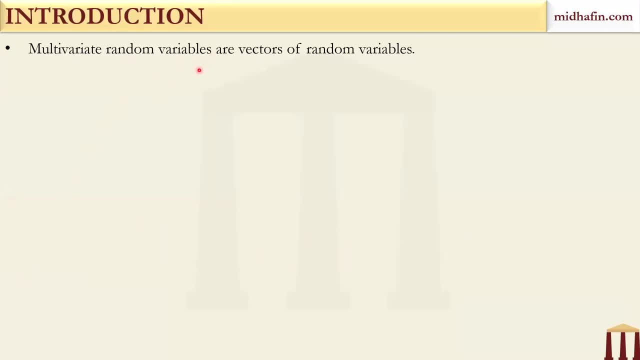 So we start QTF4 now. Now multivariate random variables. they are vectors of random, So basically they are extending the concept of a single random variable so that measures of dependence can be included between two or more random variables. Okay, Example is bivariate random variables. Now 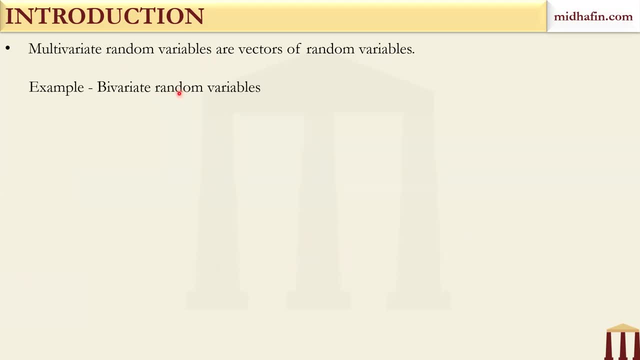 each component of a multivariate random variable is a univariate random variable. They can be discrete or continuous, just like univariate variables. For discrete, remember, we had PMF. For continuous, we had PDF And CDF was common to both. Okay, Now, as I said, they are vectors of random variables, So for 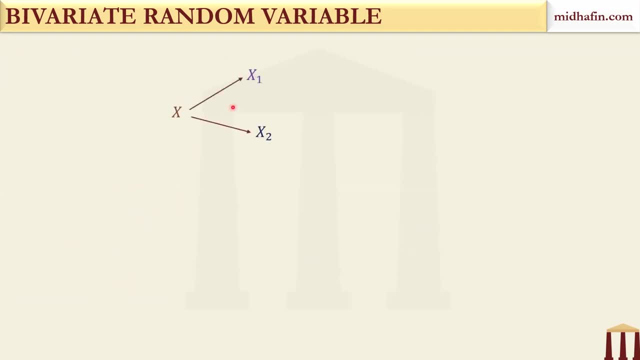 example, if you consider a bivariate, random variable, So X will be a vector. Okay, With two components: X1 and X2.. Okay, And it's realization. Now there is something called as a vector And, of course, it's value. Generally, we denote the vector as X or the function as 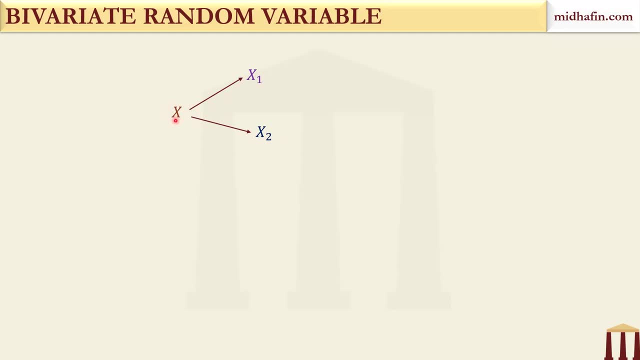 capital letters. If you remember, earlier also we used the capital letters X, X for the random variable And the realization of the random variable was denoted as small x. So this is the random variable, the two components of that and the realizations and the two components. 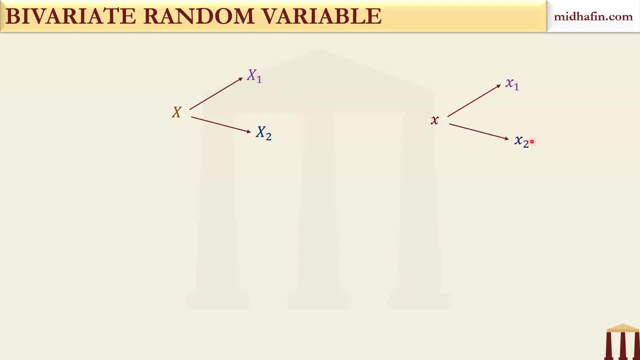 of that. So X1 is a realization from capital X1, small x2 is a realization from capital X2.. Okay, So this is the PMF of a discrete random variable bivariate. So basically this is how we denote it: F, X1, X2.. When we write F? X1, X2, it simply means that probability 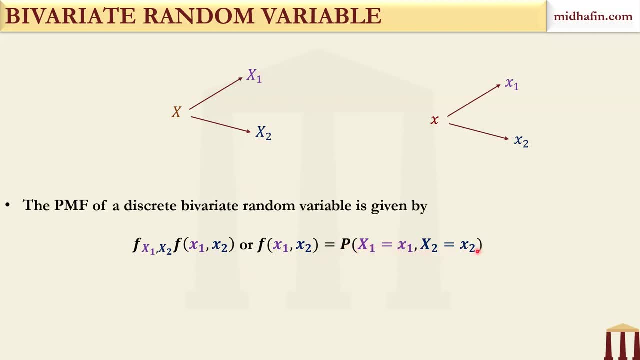 that X1 will be taking the value of X1, and X2 will be taking the value of X2.. And CDF returns the total probability that each component is less than or equal to a given value. So everything, the key ideas, are same. They have just been extended to include one more component. 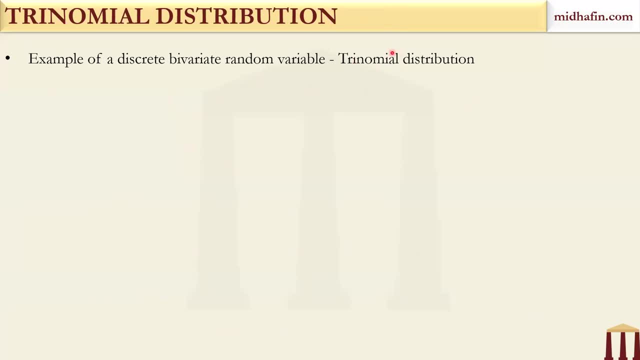 So one of the examples is trinomial distribution. For a bivariate random variable, the example is trinomial. Remember, for a univariate random variable the example was binomial. Okay, And for a bivariate it is trinomial. So you might be wondering. you know it was uni and 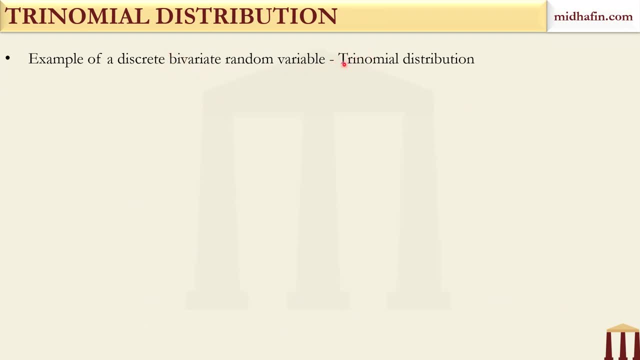 the distribution was bi. over here it is bi and the distribution is tri. So basically, one is being added right. when you're talking about distribution, You'll understand why. You'll just understand why. So let's take an example. So there are two components in 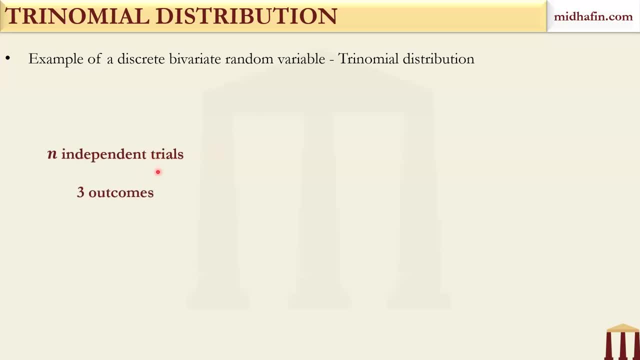 fact of a trinomial, There are n independent trials And we talk about three outcomes. Since it's a trinomial distribution, we will discuss three outcomes. of course, in case of binomial- In binomial we were discussing two outcomes- So we can model these three outcomes using 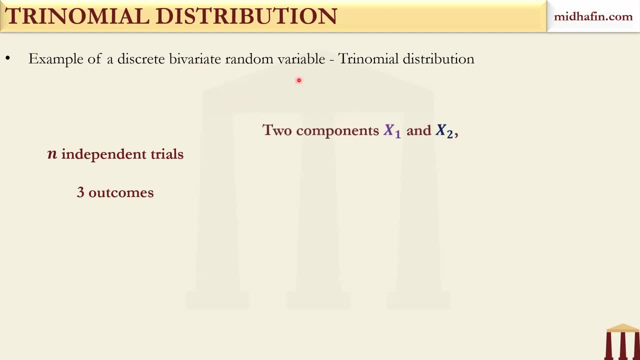 actually two components only. That is why it is a bivariate random variable but a trinomial distribution, Trinomial distribution for three outcomes. but it can be modeled using two components. That's why it is bivariate. Earlier also in case of binomial also see it was. 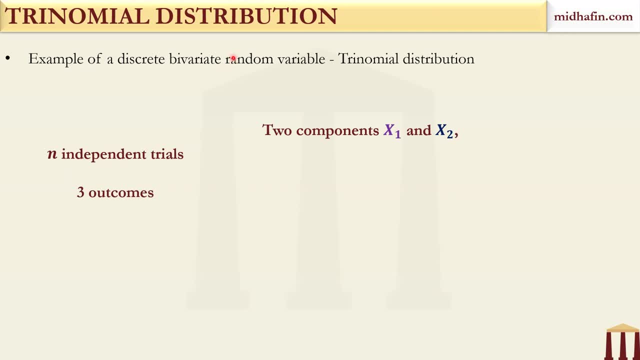 modeled only using the success parameter. right, because the failure parameter was implied as 1-1.. So over here, if suppose there are two components, x1 is the number of realization of outcome 1,, x2 is the number of realization of outcome 2, and you know that there are total n independent. 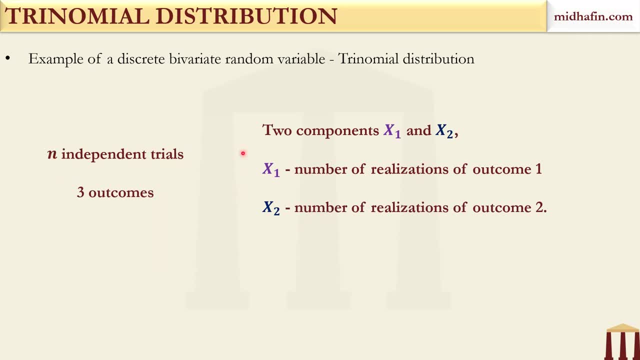 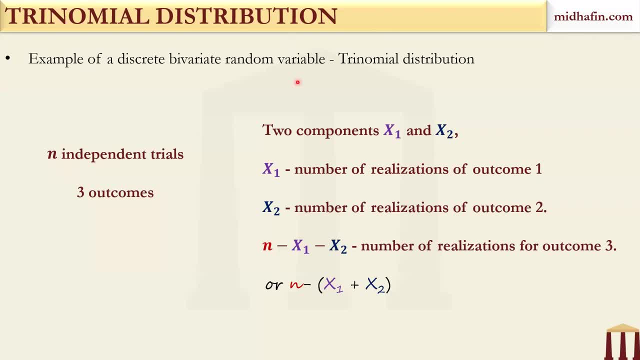 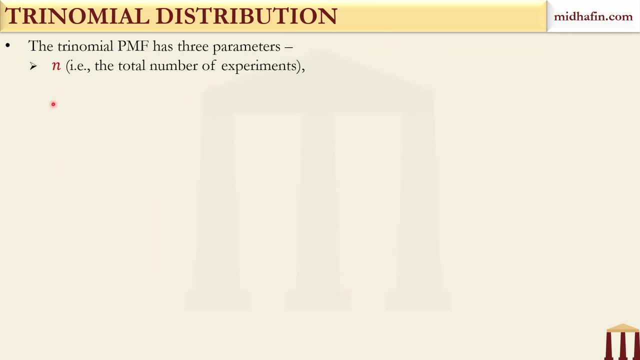 No, No, No. Now, what perhaps you have to do here is simply: you have to come and we will give you the introduction. Look for the distribution. Okay, and you will have 3 parameters: One over here, one behind that. 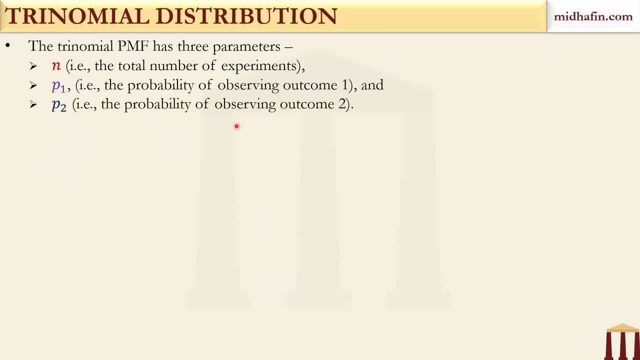 One above here, One above above, One above Okay, one above And one below Okay, one above No. P2 will be the probability of observing outcome 2 and probability of outcome 3 can simply be calculated as 1 minus P2 minus P1, which is nothing but 1 minus P1 plus P2.. 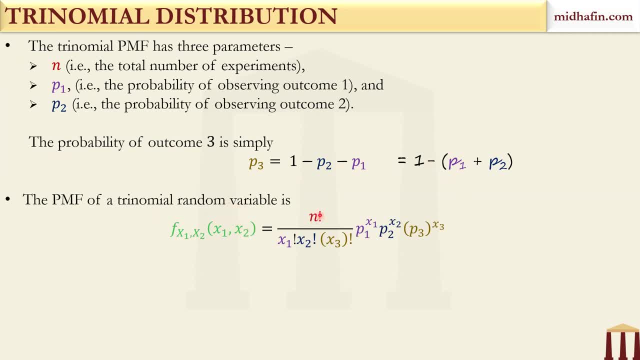 And this is the PMF of a trinomial n factorial divided by x1, factorial, x2, factorial, x3, factorial times P1 to the power x1, P2 to the power x2, P3 to the power x3. Now we have written x3 and P3 separately because it makes the memorization of the PMF easier. 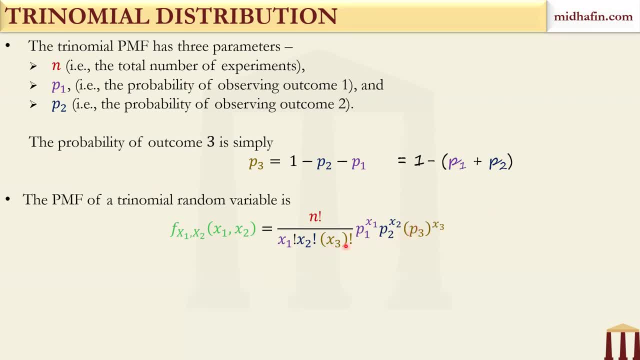 Because if you have, let's say, 1 minus P2 minus P1 over here and you have n minus x1 minus x2, it will make your job a bit difficult in terms of memorization. So that's why just write x3, but it should be implied. what is x3?? 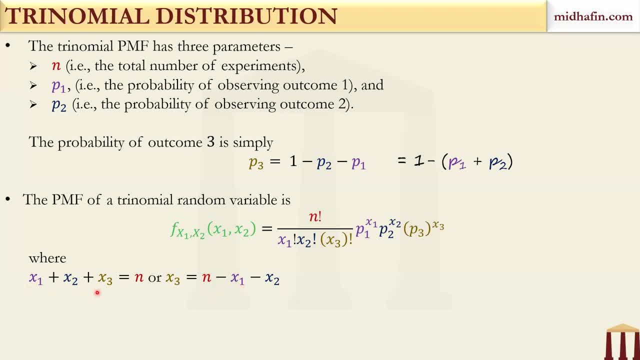 X3 is nothing but n minus x1 minus x2, because x1 plus x2 plus x3 is n. Okay And simply P3 is also 1.. So 1 minus P2 minus P1, okay. So I have reproduced this definition over here and let's solve an example. 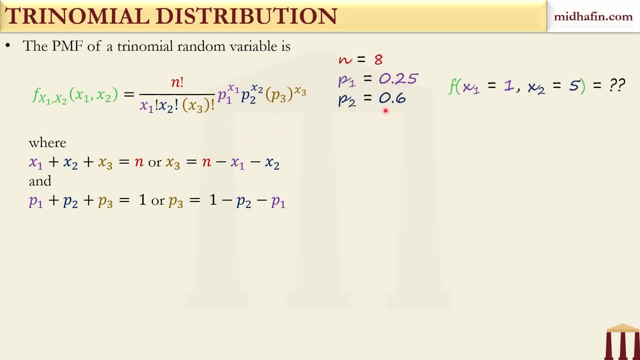 So if n is 8, P1 is 0.25, P2 is 0.6, I have to find out the probability that. what is the probability that x1 will take a value of 1 and x2 will take a value of 5, if this is, 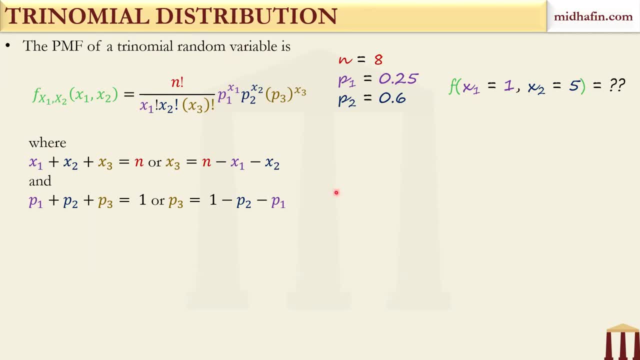 what I have to find out. So, technically, I am telling you, technically, this should be capital N again. See these things, although people tend to ignore. but see, because 1 is the real, this is actually small x1.. This is, this should be capital X and this should be capital X2.. 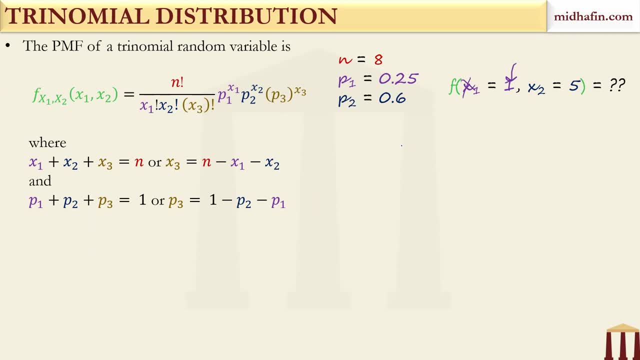 Anyways, don't worry about all these things from an exam point of view, but technically, capital X1 is the random variable and the small x1, this is the realization. Okay, Anyways, let's continue. So tell me what will be x3 over here. 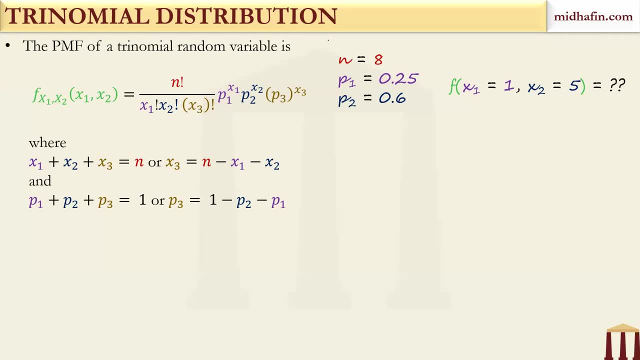 What will be x3?? What will be x3?? Quickly, 2.. 2. Very good, So we can use this to find out x3. Absolutely So x3 is 2.. What is P3?? What is P3?? 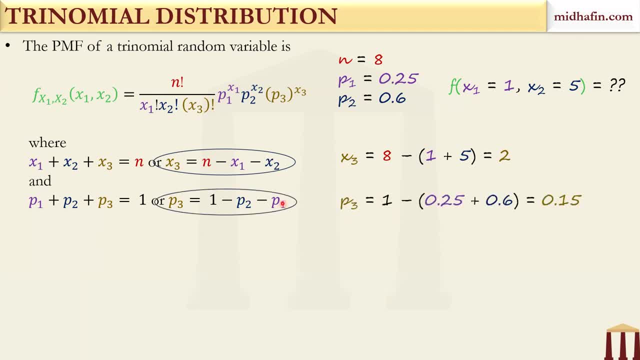 Perfect 0.15.. Yes, 0.15.. So we can use this to find out P3, which means my F, 1 comma 5.. So this can be simplified to. if you want to write it in a condensed manner, you can write: 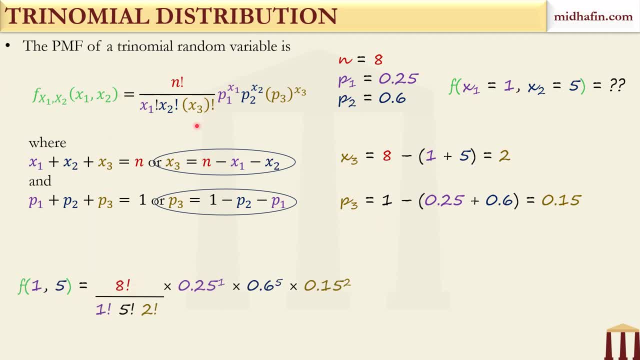 F1 comma 5 simply is equal to. we use the PMF of the trinomial and we get the result as 7.35%. So the interpretation is that under these conditions, the probability of x1 taking a value of 1 and x2 taking a value of 5 is equal to 7.35%. 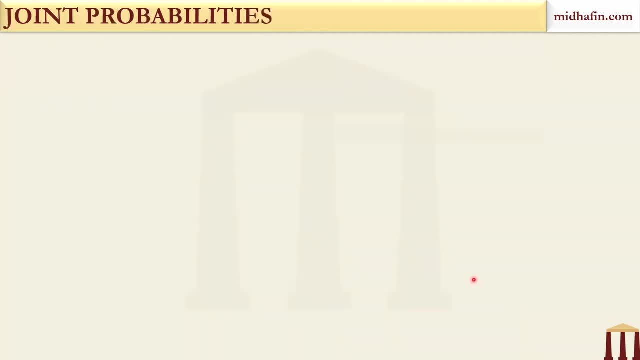 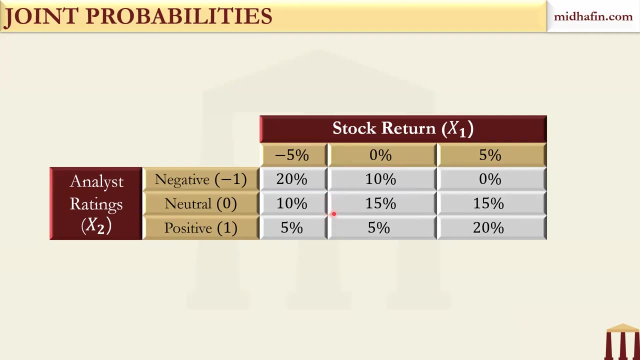 Now let's come to joint probabilities. So let's take an example over here Now. discrete distributions: if they are defined over a finite set of values, they can be described using this kind of a probability matrix. It simply relates the realizations that we were talking about, these three realizations. 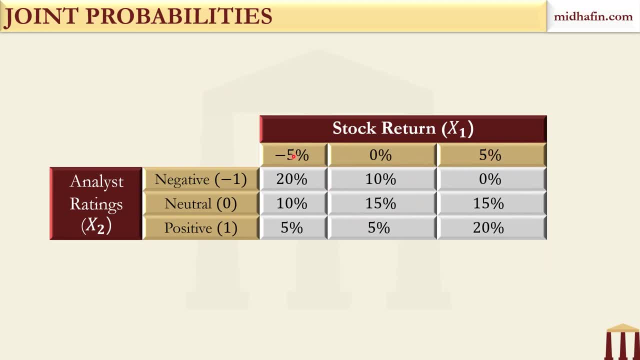 to these probabilities, And these are joint probabilities, basically a tabular representation of the PMF. you can say. So what is the meaning of the numbers in this table? These are giving you the joint probabilities. So, for example, yeah, Okay, 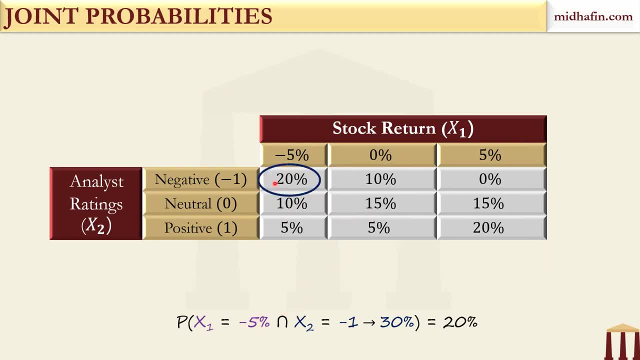 probability. say this: one of X1 taking a value of negative 5% and X2 taking a value of negative 1 is 20%. So this 20% is the joint probability that the stock return will be negative 5% and the analyst rating will be negative. Remember this is not the conditional probability. 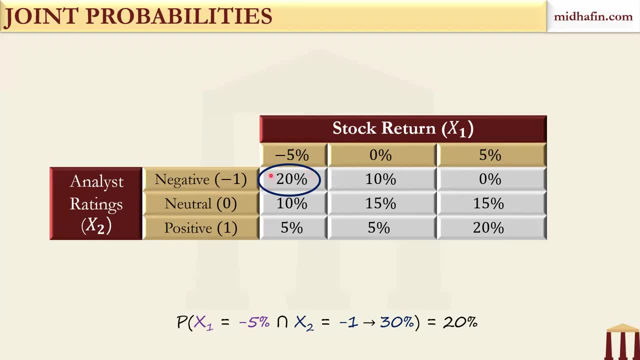 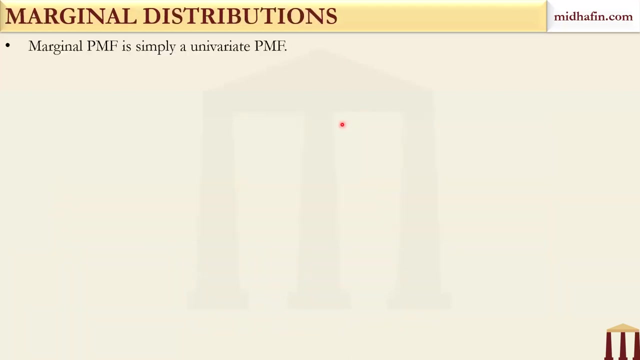 Conditional will be calculated later. This is the joint probability. So all these numbers in these cells are the joint probabilities. Is it clear? These are joint probabilities. Is it clear? Now, what if I want to deduce the marginal PMF from these joint probabilities? 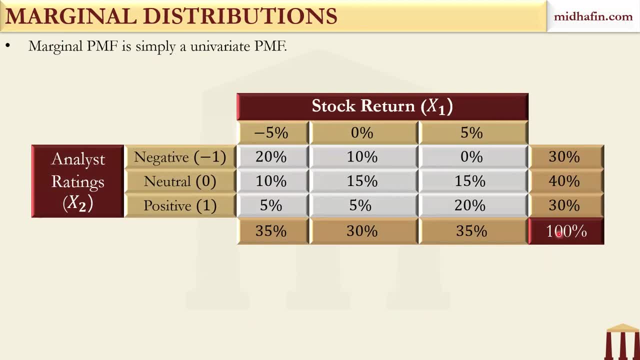 So now the same table I've just extended to include one more extra column, one more row where we are actually summing the entries of these cells. So basically, if I want to find out, the unconditional- see marginal- also implies unconditional. So unconditional in this case. in this case, not always, in this case- for probabilities. 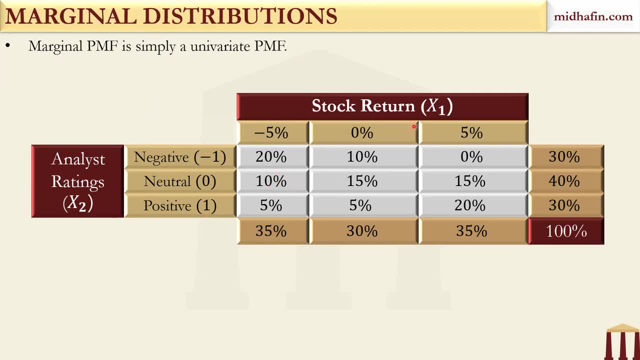 So when I want to find out the unconditional or marginal probability that the stock return is negative 5%, what is the probability that the stock return is negative 5%, simply? So we will just add all the entries over here. So for negative 5% we have three entries: 20%, 10%, 5%. 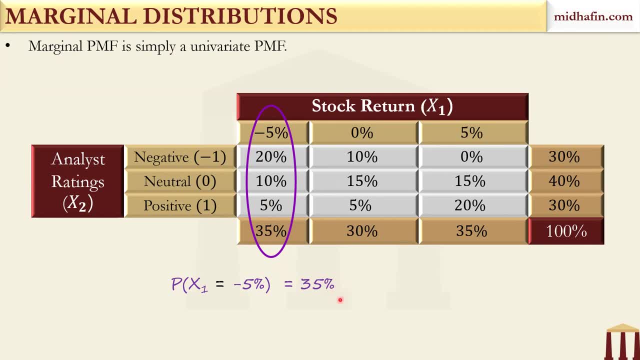 What is the summation? 35%, Okay. Similarly, can you tell me what is the probability that analyst rating is neutral? What is the probability that analyst rating is neutral? Everyone, not only one or two answers. What is the probability that analyst rating is neutral? 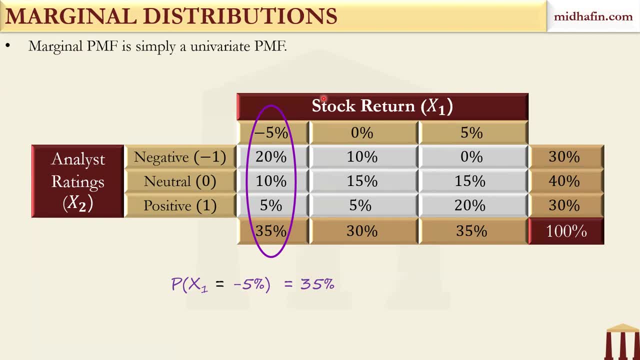 Correct, Absolutely, So you will sum across the second row. This is your neutral, So this is your probability over here. Okay, To make it more precise, I can also include either this part or I can remove this, But anyways, that's just a diagrammatic representation, but the idea is clear. 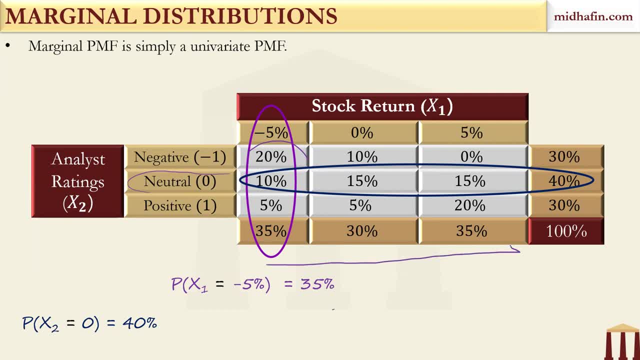 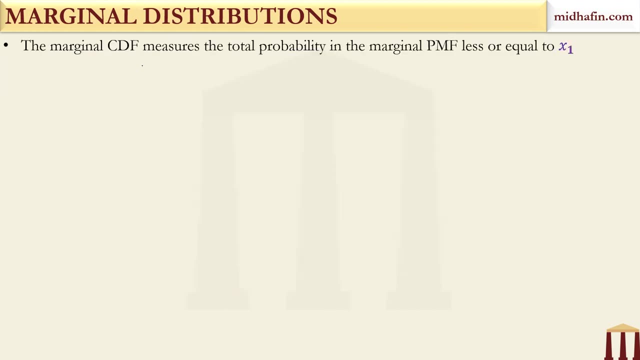 Now one more important aspect you're observing is: either you sum across these cells or you sum across these cells. The total will always be equal to 100%. So this is how you derive marginal probabilities from joint probabilities using this joint probability matrix. Now the marginal CDF measures the total probability in the marginal PMF less than or equal to. 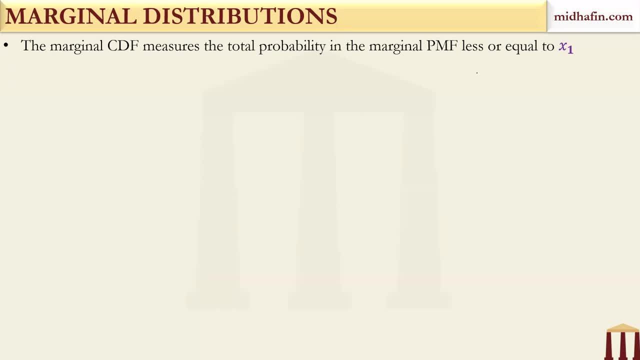 X1.. So similarly, in a very similar fashion, that we defined the CDF over here also, it's the same thing. So let's say, if I want to find out the marginal CDF Corresponding to X1 at 0%. 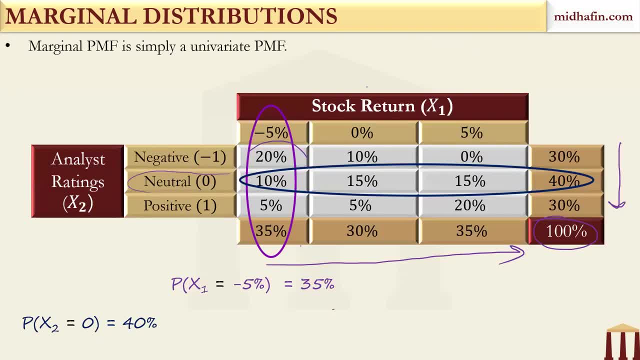 It means that if I want to find out that the stock return will be less than or equal to 0%. So less than or equal to 0 means what? Either this or this. So I'll find out the marginal probability of this and I'll find out the marginal probability. 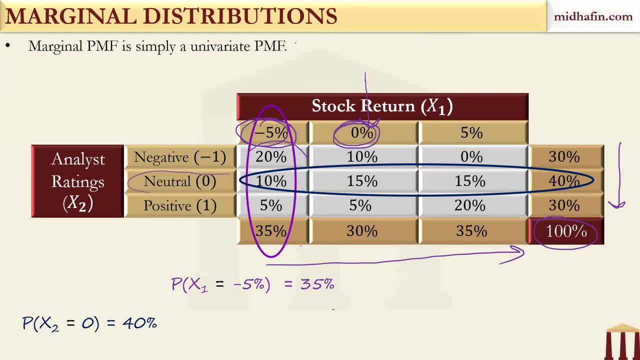 of this and I'll just add them both. So can you tell me what will be the CDF, defined in a way such that I want to find out the probability that the stock return will be less than or equal to 0%? Tell me. 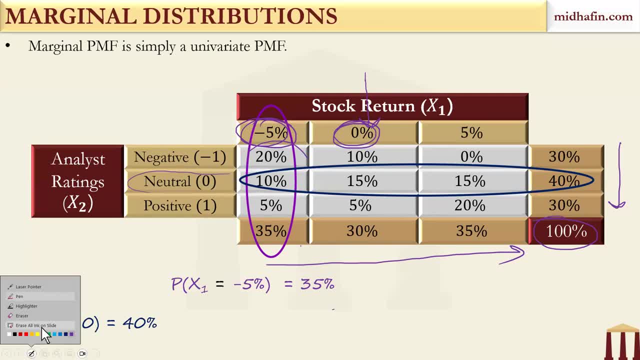 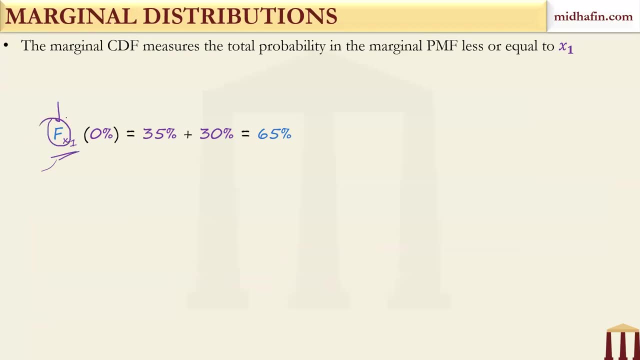 Correct, Absolutely correct, Okay. So basically, we are going to add this and this: for 0%, you have 30,. for negative 5%, you have 35. So this is your CDF. That's why capital F is written here. 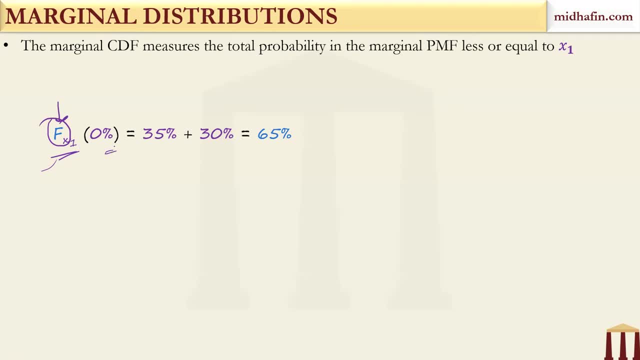 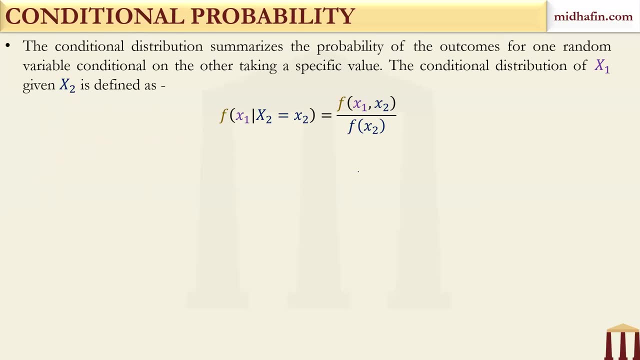 CDF. So this gives you the probability that stock return is less than or equal to 0%. Okay, Now conditional probability, Again in the same way that we calculated conditional probability earlier. only the notations have changed a little bit. Okay. 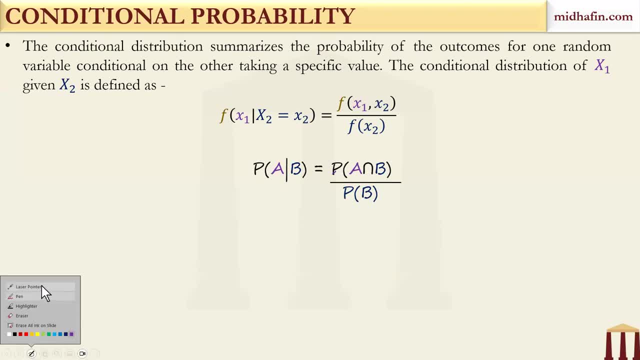 So, if you remember, this was the formula for conditional probability earlier, right? So in the numerator you have joint probability. over here also, you have joint probability. Okay, In the numerator you have the marginal probability. over here also, you have the marginal probability. 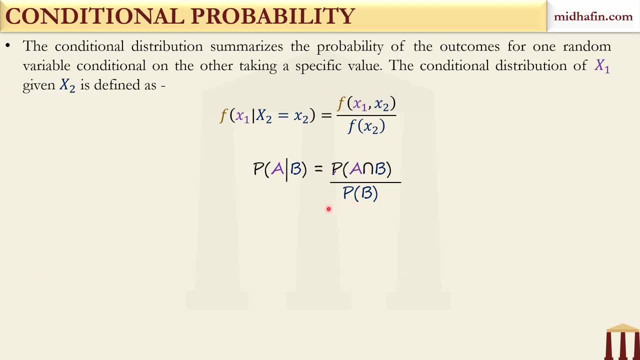 So let's take an example: Using the same table. Using the same table, If I want to find out the conditional probability, this question can be asked in the example, Because they'll give you a table, let's say and joint. they'll definitely not ask because 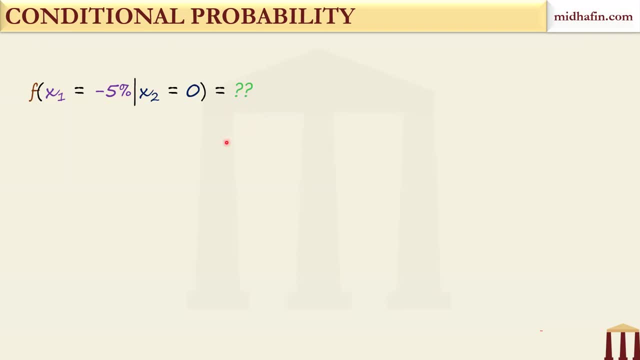 it will be way too simple. Marginal also is way too simple. So what they can ask is, I think, this kind of question where you are assuming that X2 has already occurred. If you're assuming that X2 has already happened, Okay. 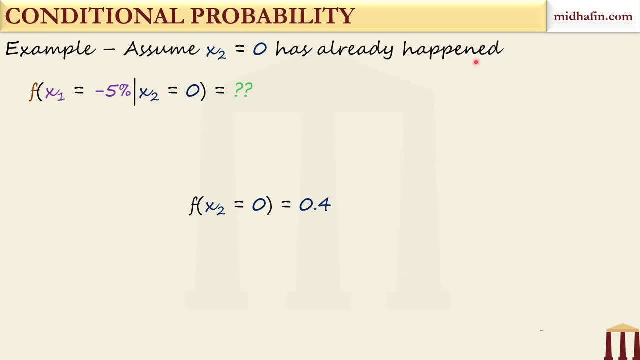 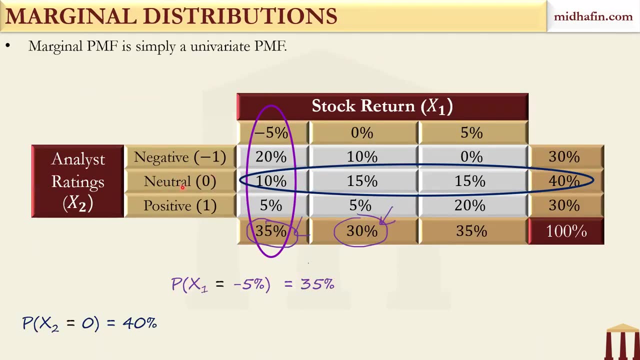 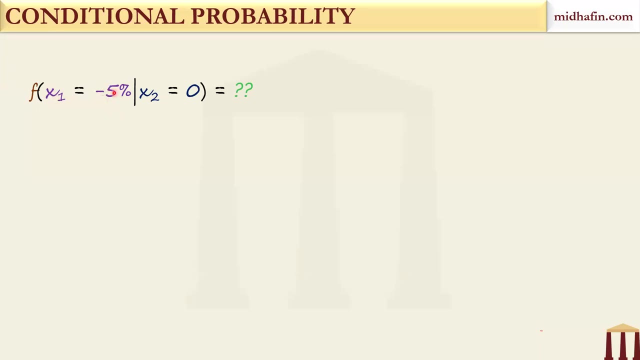 Okay, Okay. So if X2 equal to zero has already happened, it means that it is given that analyst has already given a neutral rating. So, given that analyst has given a neutral rating, what is the probability that the stock return will be negative 5%? if this is what I have to find out, 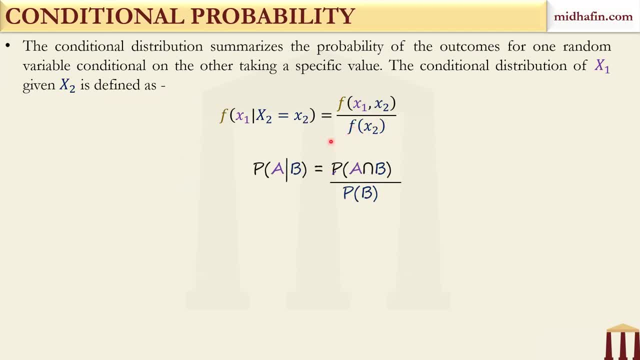 So what is in the denominator: Marginal probability. Now, earlier, in the case of the theorem of total probability, when we studied this for the first time, I said that the denominator generally Should be calculated using the theorem of total value. add all the probabilities for 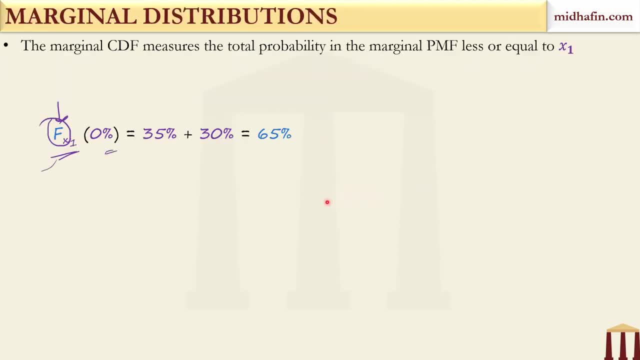 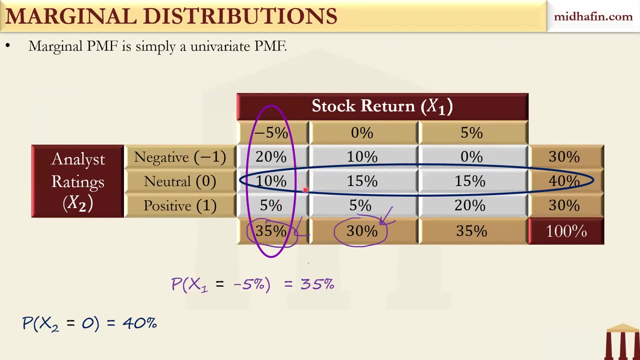 the denominator right The corresponding over here. Also, you're doing the same thing. You're adding across the rows, So only the representation is different. You are adding across the rows and the columns. Okay, So tell me one thing. 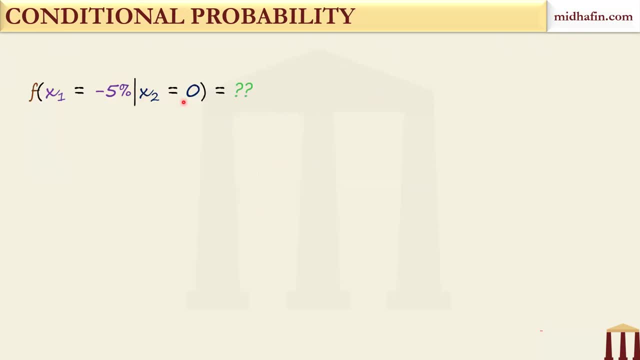 First, I want to find out the marginal probability of X2 equal to zero. So what is the marginal probability of X2 equal to zero? We have already calculated What is the marginal probability that X2 will be equal to zero Absolutely. 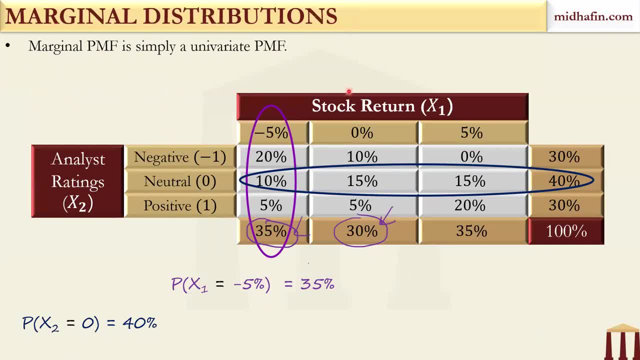 40%. Okay, This blue oval, add all the probabilities: 10, 15, 15.. 40%, 40%. We have already calculated it. So the denominator will be how much? What will be the denominator for this? 0.4 only. 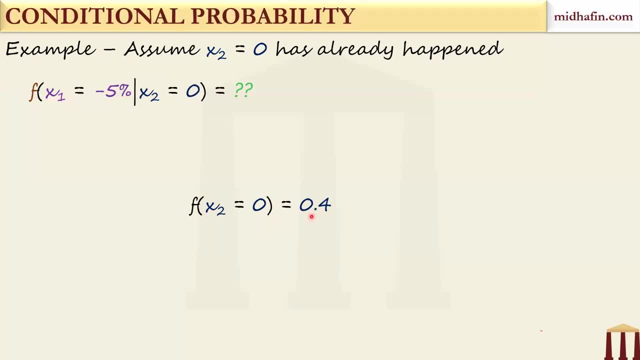 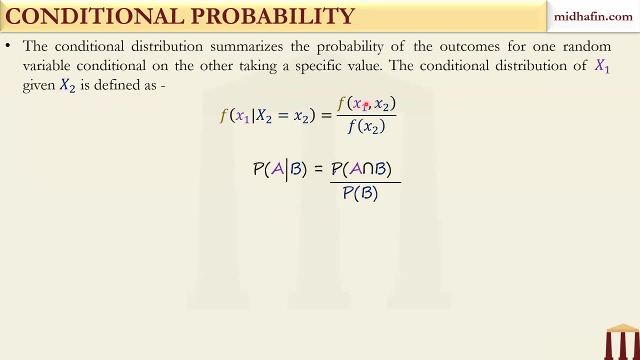 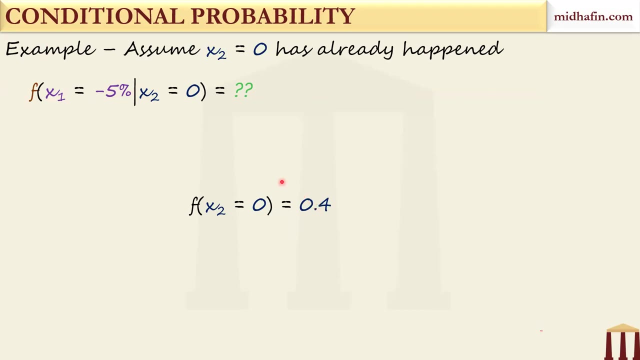 Based on the denominator? Yeah, Based on our definition. so this is our definition of conditional probability. this one, f divided by f. So joint divided by marginal, Joint divided by marginal. So look at the table and tell me what is the joint for these two. 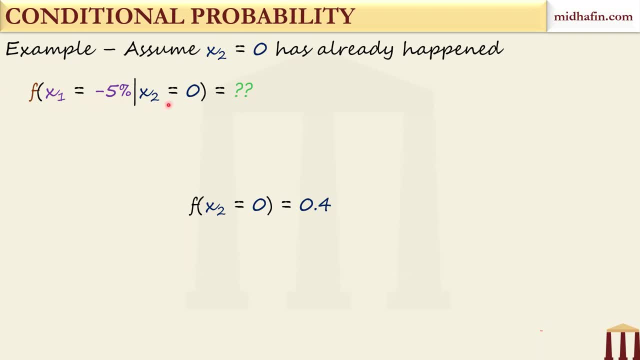 What is the joint for x1 equal to minus 5 and x2 equal to 0?? Let us go back to the table. See the question carefully, and I am going back to the table. Find the joint of these two outcomes: x1 equal to negative 5, x2 equal to 0. first, 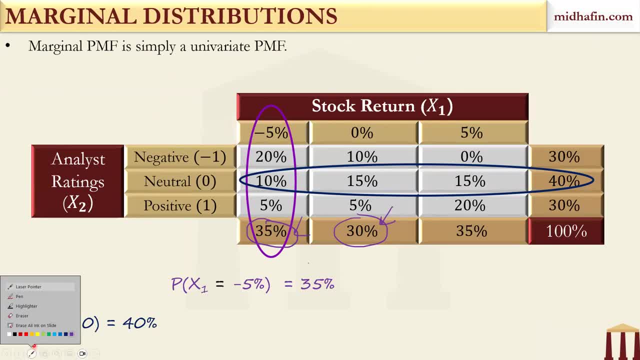 x1 equal to negative 5 and x2 equal to 0.. What is the joint? Correct: 0.1.. So this is the joint, this one, This cell. we are talking about This cell. Okay, So over here. 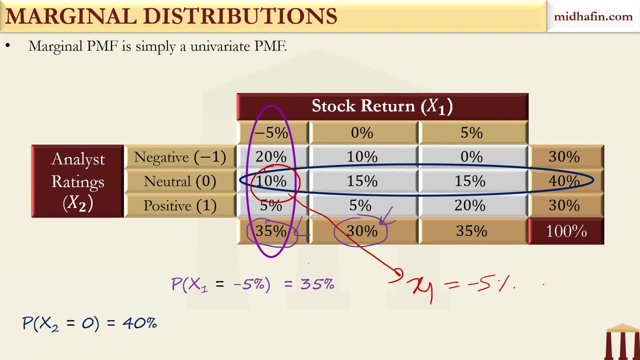 x1 equal to 0.1.. x2 equal to minus 5 percent and x2 equal to 0.. So analyst neutral grating and so joint probability is 10.. So joint is 10, marginal was 0.4.. 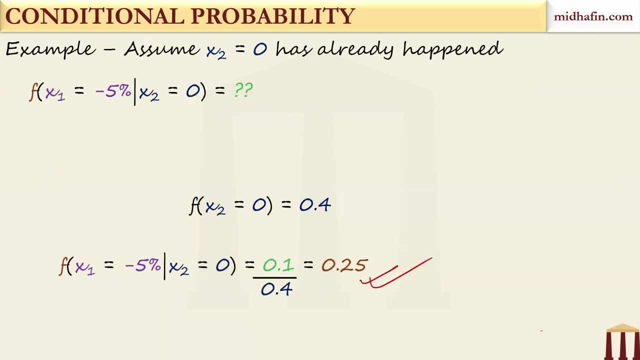 So what will be your answer? 0.25.. As simple as that. So is it clear how to calculate conditional probability from the table. to everyone, Everyone, Okay. So I think the animations were not in correct order. Actually, they should have been before. 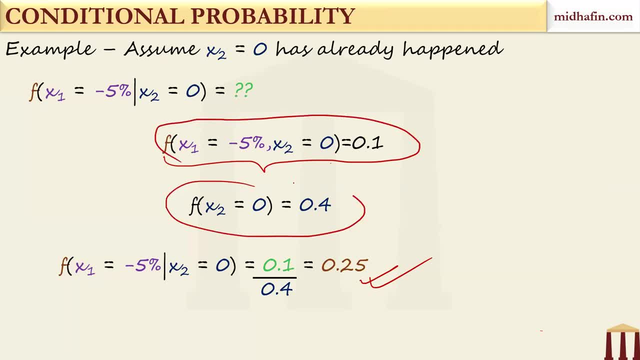 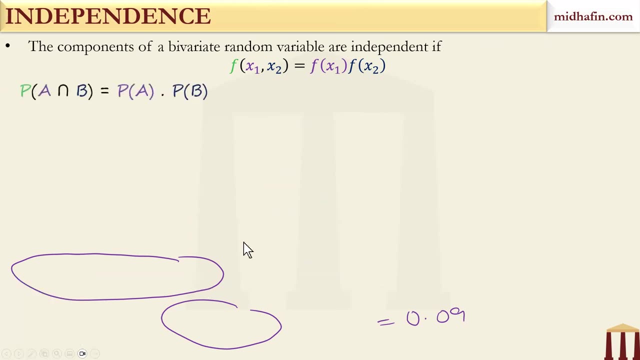 Okay, So this is the joint probability, This is the marginal probability and this is the final probability. This animation was missed, I think. Okay, Fine, No problem Now. Anyways, So the two components of bivariant, bivariate random variable: they are independent if f is equal to f times. 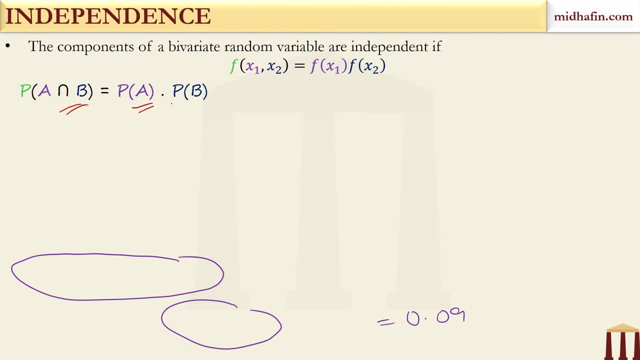 error. This is similar to the joint probability being the multiplication of the individual probability. That was the independence condition. Remember this from probabilities: It's exactly the same thing, which is written just in a slightly different notation. The same thing is written in a slightly different notation and we know that. 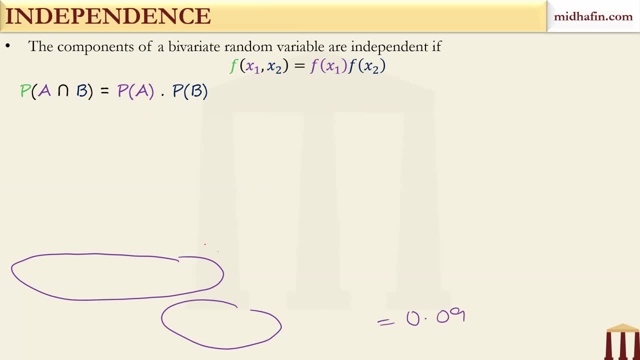 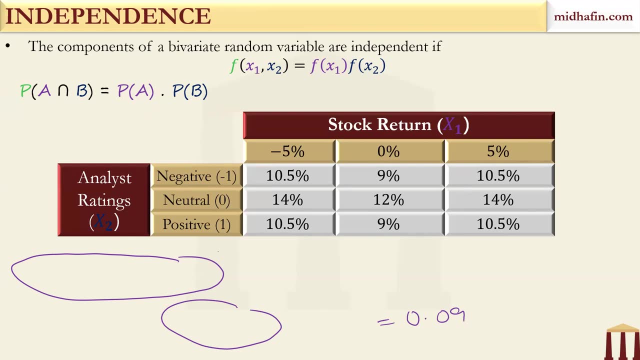 this was the condition for independence, Okay, So tell me one thing. this is the example over here, Okay, And the numbers have been changed. Okay, Just for this example. So first let's find out the marginal probabilities, Let's add across these three rows. 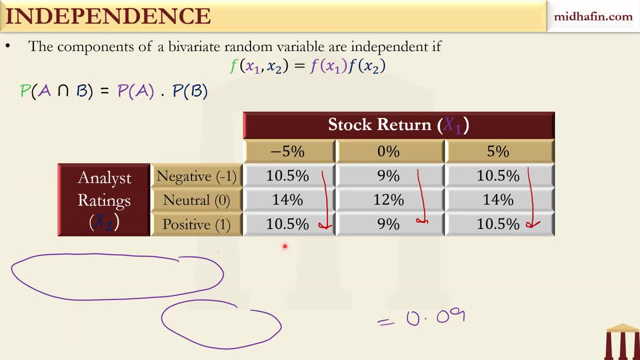 If we add across these three rows- just check the calculations- Will you get 35, 30 and 35? Yes or no, Is it correct? Okay Now, across the columns, you get 35, 30 and 35.. Across the rows, you will get 30, 40 and 30.. Correct. 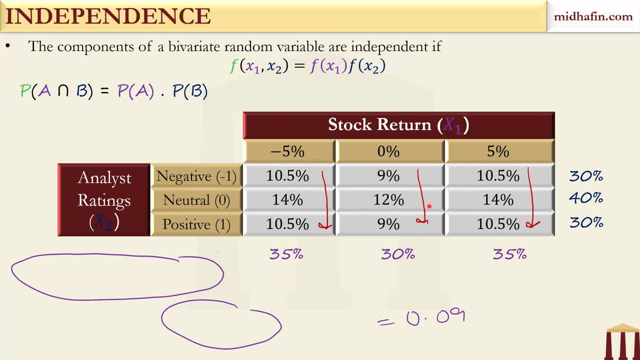 If you add these three entries: 30, 40, 30.. Correct Now, if I have to check the joint probability, that x1 equal to 0% and x2 equal to negative 1. If I have to check this, is it 9%? this one? 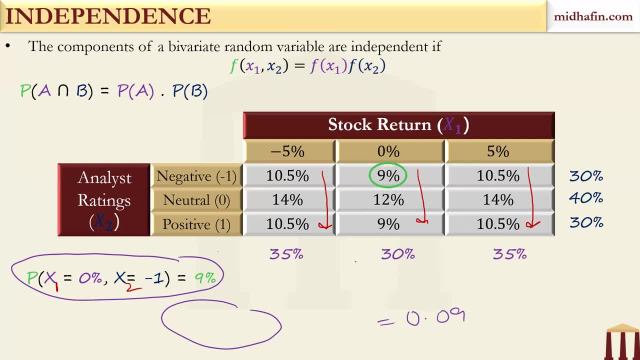 Agreed. Is this correct? The joint probability: Okay. So what is the product of marginal sober? The joint probability of x1 being equal to 0% and the analyst rating being negative, that is, x2 being equal to negative, 1 is 9%. 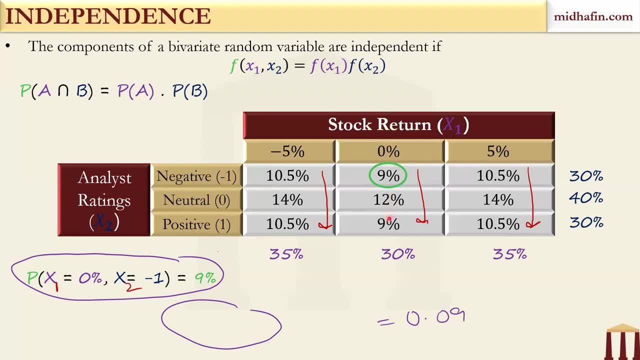 But the product of marginals. let's calculate that also. So for 0,, x1 equal to 0,, the marginal is 30. Right, And for x2 equal to negative 1, the marginal is 30. So over here, PA times, PV is also 0.3 into 0.3,, which is nothing but 0.09 or 9%. Are these equal? 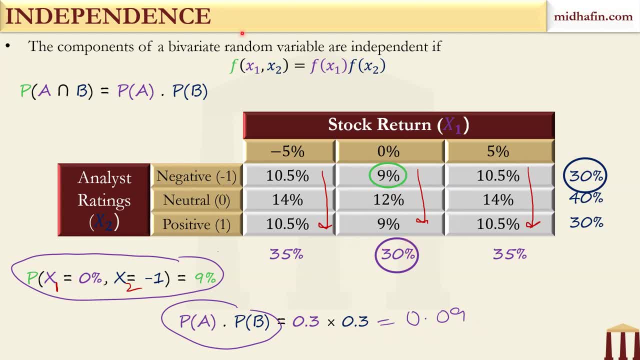 Is the joint equal to the product of marginals. Is the so short, 0.09, right. Do not miss it, because these silly mistakes will be very costly, You know, even if you say miss one or two questions because of these silly mistakes. 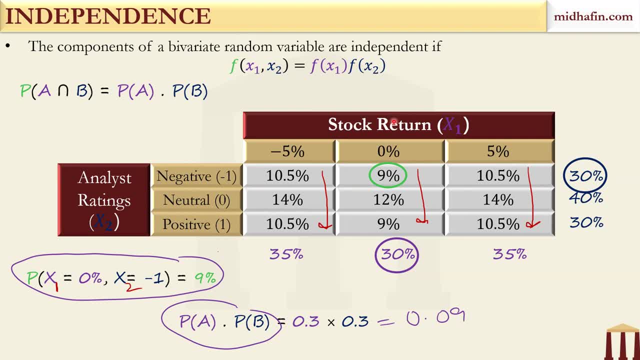 it will be So as of now. you just have to compare. but maybe in a calculated question, instead of 0.09, you mention 0.9, it will be a disaster, Right? So please do the calculations very, very carefully in the exam. So is the joint equal to the product of marginals? Is the joint equal to the 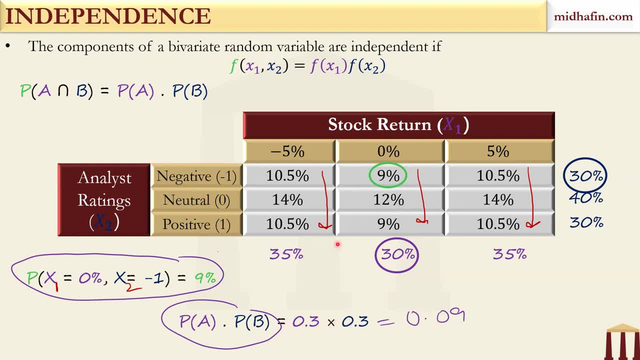 product of the marginals. Yes, Is it true for all cells? Can you check that randomly for any one cell? Because since all of you will be checking and there are around 50 candidates right now, 47 candidates, So if all of you are checking, I'm assuming everyone will check. 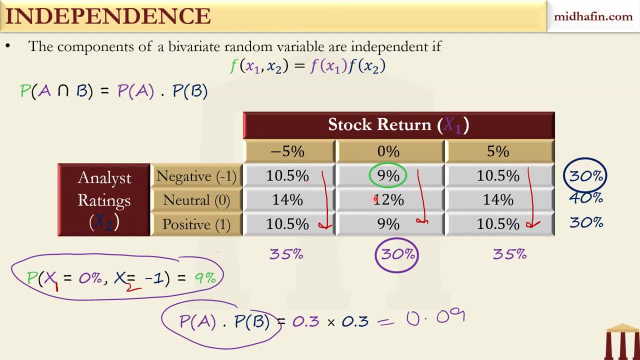 say, any random cell on their own. So all the cells will be checked. Just check any one random cell and check if the product of marginals is equal to joined on for any other cell. Yes, Every cell. Correct, Absolutely. So even if it is not applicable for a single. 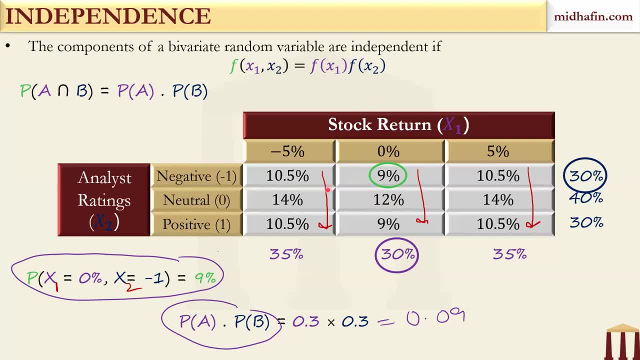 cell, the independence condition will be violated. So that's why these numbers have been chosen very carefully by Garth. Okay, So that this example is clear to me. Got it Fine. So expectations Now, instead of writing the formula for expectations, 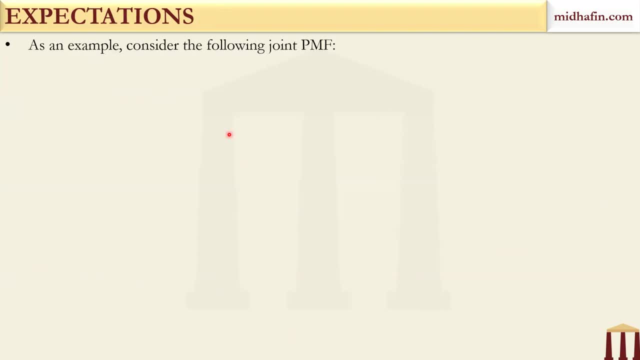 I thought that it would be better to explain expectations directly using an example over here, because we know what is expectation. Expectation was nothing but summation PIXI. Even in case of Y-variate, it works in a very similar. So let's see an example. So let's. 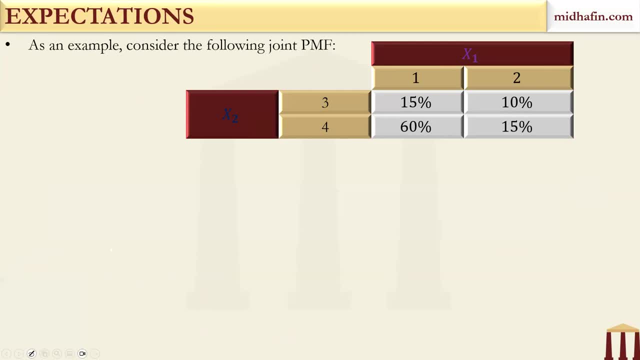 say you have X1.. Okay, It's not visible. I'll use a different ink over here. This is X1.. Okay, And this is X2.. So X1 is taking the value one and two and X2 is taking the values. 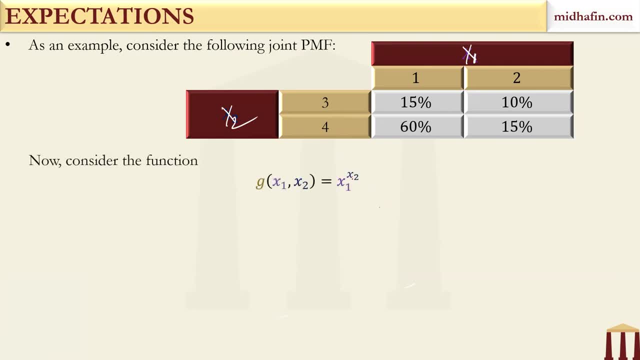 three and four. Now consider this function: X1 to the power X2. So there are four possible outcomes for this function, because there are two values for X1, two values for X2. So that's why there are four possible outcomes, two times two. What are those four outcomes? These 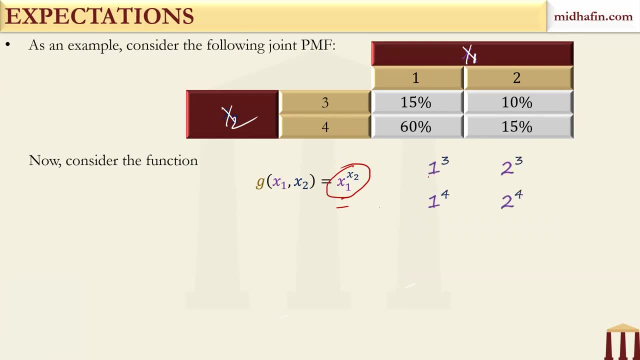 are the four outcomes, Do you agree? Do you agree? these are the four outcomes: One to the power three, two to the power three, one to the power four, two to the power four. X1 is only having one and two. X2 is only having three and four values. So, if I want, 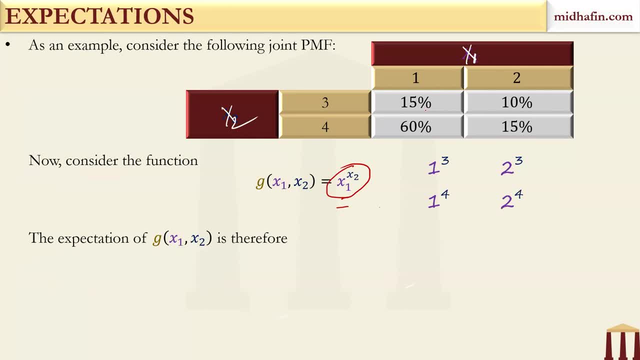 to find out the expectation of G. and these are the probabilities which are given the joint probabilities. And of course I have to use joint probabilities because, see, when will X1 to the power X2 take a value of one to the power three? It will only take a value. 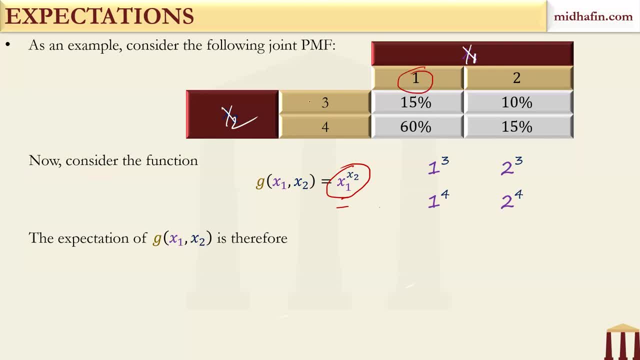 of one to the power three when X1 is one and X2 is three, Correct. So if I want to find out the expected value of X1 to the power X2, these types of questions can be asked in the exam. If I want to find out the value of X1 to the power X2, what will I do? I will 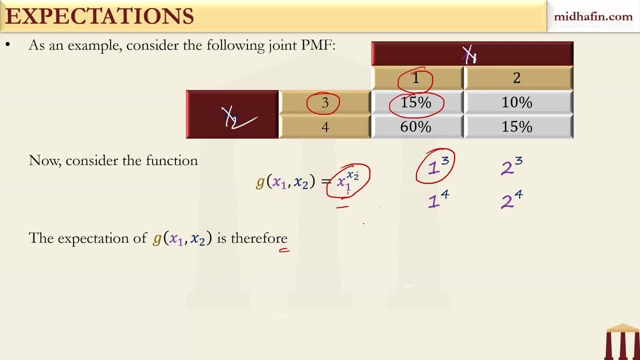 multiply these individual probabilities by this value of the function. the realized value of the function Agreed. So 15% will be multiplied with one to the power three. Can you tell me? two to the power three will be multiplied with which probability? Two to the power three? 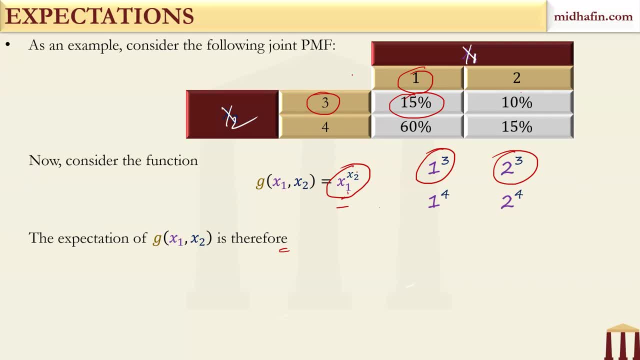 will be multiplied with which probability: Two to the power three will be multiplied with which probability: Correct, correct, correct, 10%. Two to the power four will be multiplied with which probability: Very good: 15%. And finally, one to the power four. 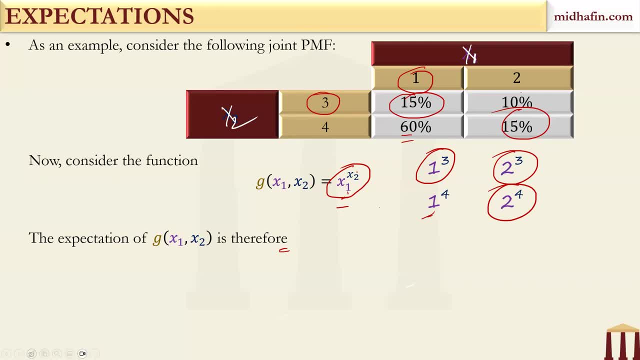 will be multiplied by 60%. So if we do this, we are able to find out the expected value of X1 to the power X2 like this, which is 3.92.. Is it clear? Will you be able to calculate the expected value of a function in case of by one to the power three? Yes, you can, So. 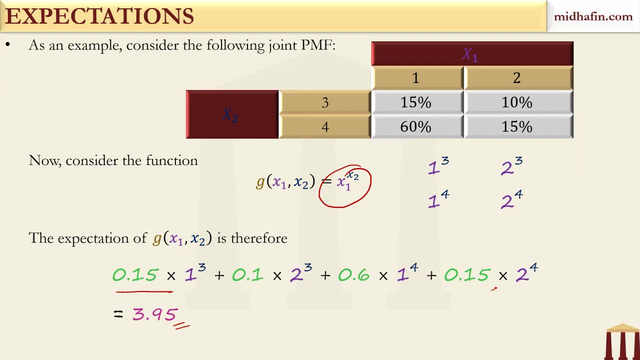 you can calculate the expected value of X1 to the power X2 like this, which is 3.92.. Can you see the by variate variable now? Will you be able to calculate it in the exam? Okay, very straightforward, just multiply the probabilities by the realized outcomes. 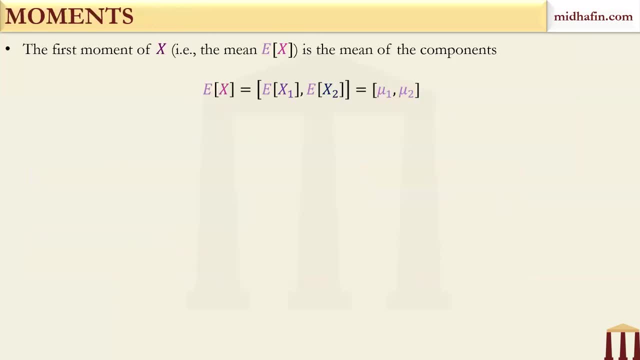 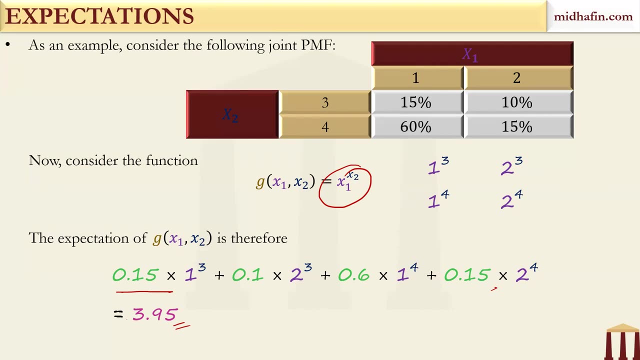 that's it, Okay, See, one thing I just want to point out over here, Since this is a crash course. I said we are taking very limited examples, But- and initially also I said that solving will be very difficult and query discussion will be very difficult. but in case of 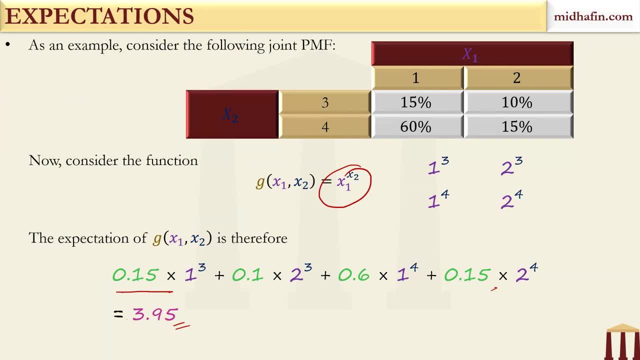 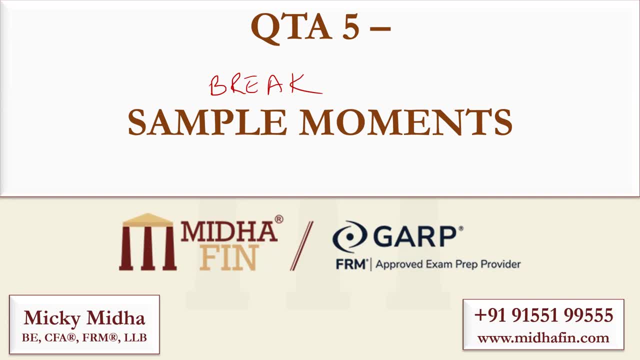 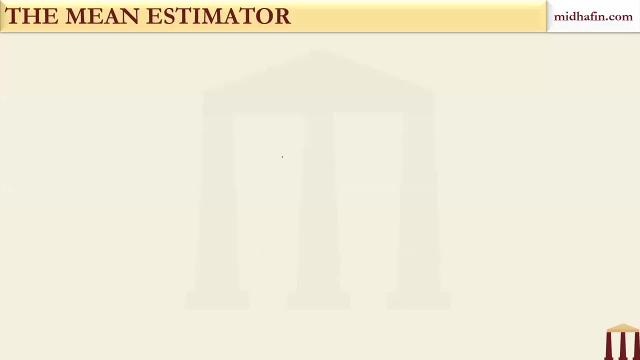 plus 3 plus 4 plus 5 by 5, which is 3.. What is the median Median is also 3.. Okay, So let's say now what I do, is I add an outlier to this distribution, say 200.. What is the? 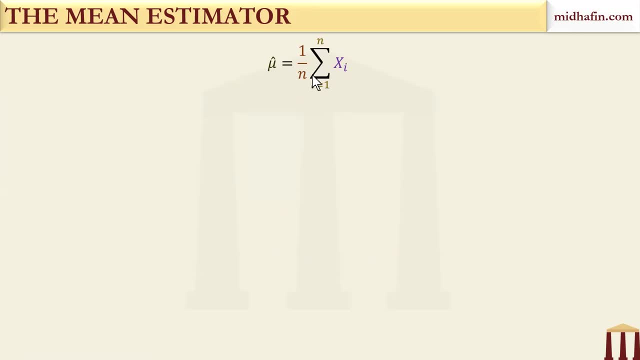 mean of this distribution? What is the mean of this distribution now, Equally weighted again, What is the mean of this distribution? 35 point, something, right, Okay, What is the median of this distribution? The average of these two, correct? 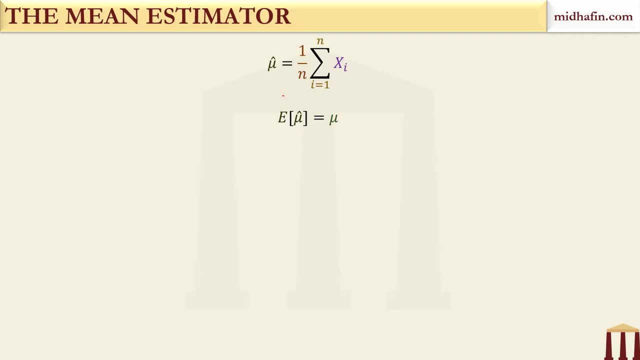 Okay, Now tell me, is the new mean of 35.83 in any way a good representation of the sample? Is it even close to any of the points? not even 1,, 2,, 3,, 4, 5,, not even 200? Are you? 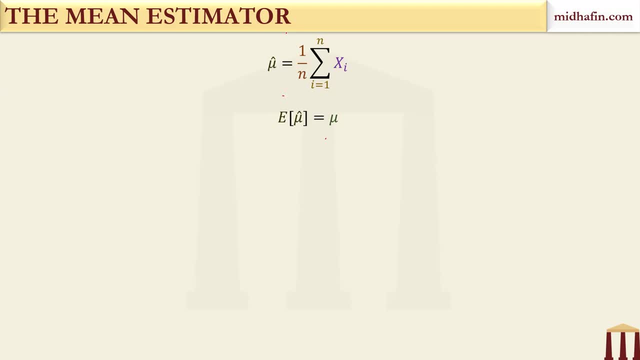 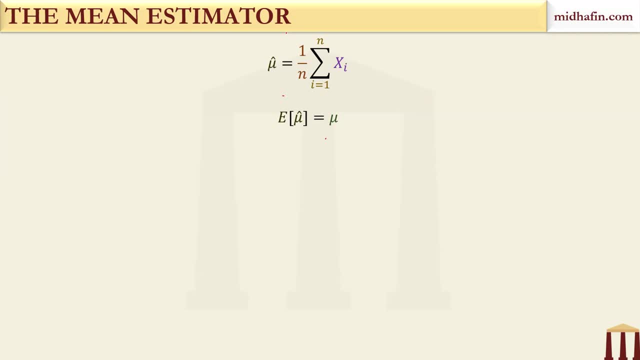 Okay, Okay, Okay, Okay, Okay, Okay. So is it a good representation? Is it a good representation, guys? 35.83 of the sample points? No, But is median still a good representation? Is that still, close to these five points, at least? Right, Yeah, Median still, even though it. 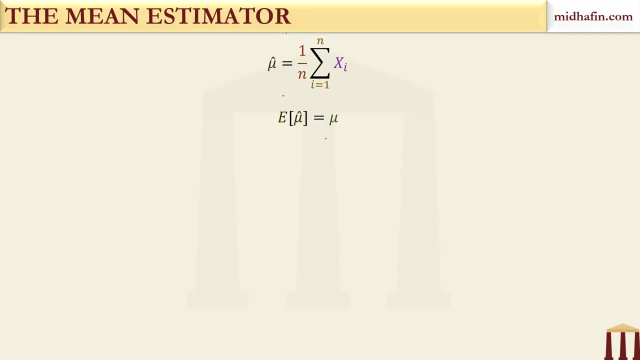 is not close to the outlier. it will not be. So which one is more robust to outliers? mean, Which one is more robust to outliers? Obviously median is more robust to outliers. Okay, so that is the very attractive property of median. Now this is the formula for sample. 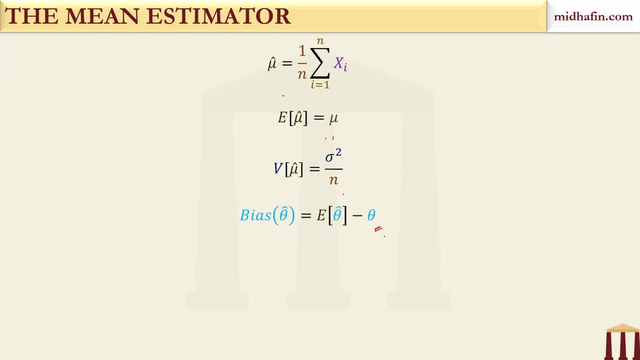 covariance estimator. Again, the crux is that you have 1 minus n, by sorry 1 over n minus 1.. So n minus 1 is in the denominator, which gives you an unbiased estimate, instead of n. Then, in case of multivariate moments, what you can do is you can actually extend the same. 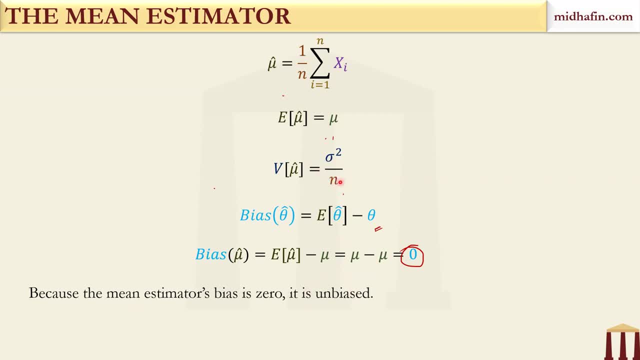 principle that we had in case of univariate, where we had skewness and kurtosis Over here we can have cross moments. So we will have for pth moment we will have p minus 1 different measures. So when we are talking about pth cross moments or cross pth moments, 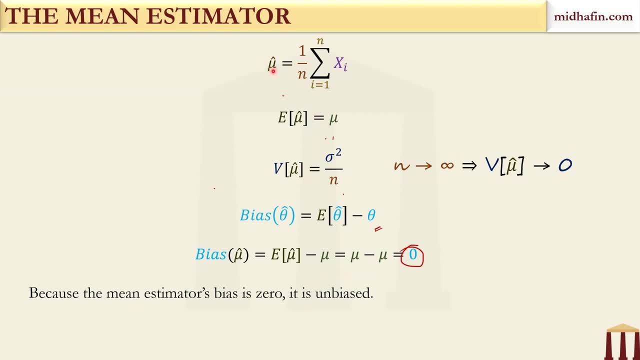 there will be p minus 1 different measures. So what I mean to say is that there will be no cross means. Why no cross means? Because it is the first moment. So p is 1.. So p minus 1 is 0.. So 0 cross means There is one cross variance, which we call as: 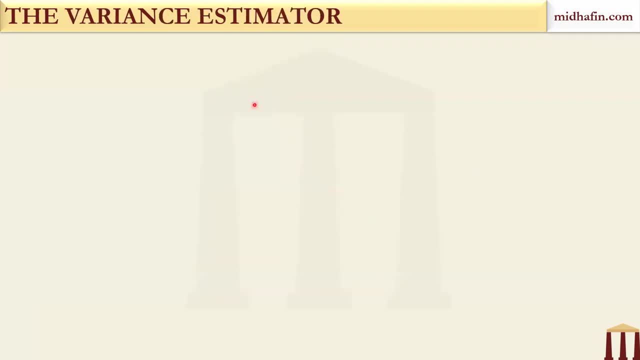 covariance. There is only one covariance, right Between two observation, two components. if you have two components of a bivariate random variable x1, comma, x2, there is only one covariance, correct, There is not more than one covariance. So, since we are talking about the second degree, 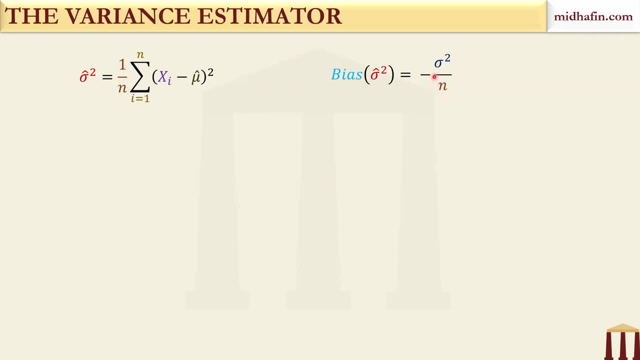 the second moment. So p minus 1 is 1.. There is only one covariance, So this can be verified over here also. What about skewness? How many co-skewness will be there? Two co-skewness will be there. 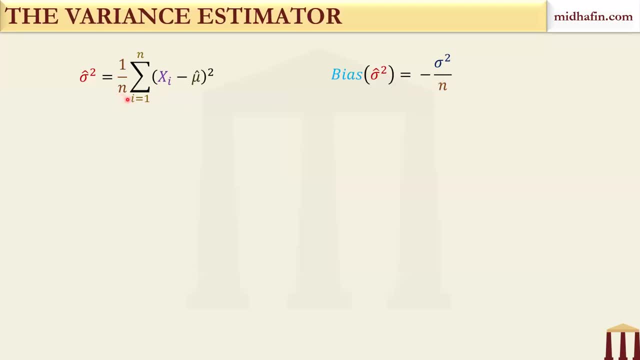 Why, Based on this principle, skewness is the third moment correct. Third standardized central moment, if you remember. So, if it is the third moment, it means p is 3. So p minus 1 is 2. So 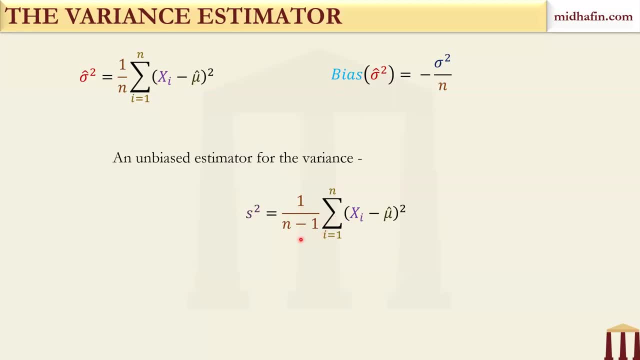 there are two co-skewnesses, And how many co-kurtosis measures will it take? So p minus 1 is 1.. So p minus 1 is 2.. So there are two co-skewnesses And how many co-kurtosis measures? 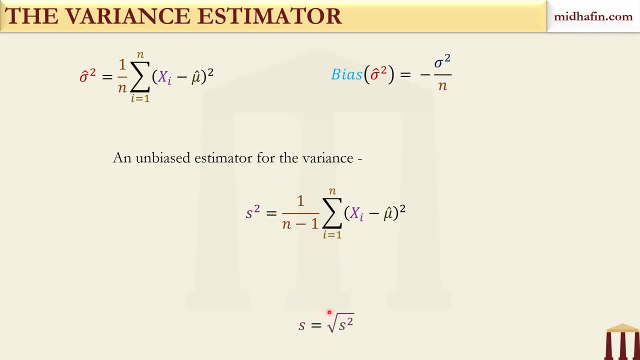 will be there based on this rule of thumb, I should say, or convention, How many co-kurtosis measures should be there according to you? Very good, It should be 3.. So there is one covariance, two co-skewnesses and three co-kurtosis. 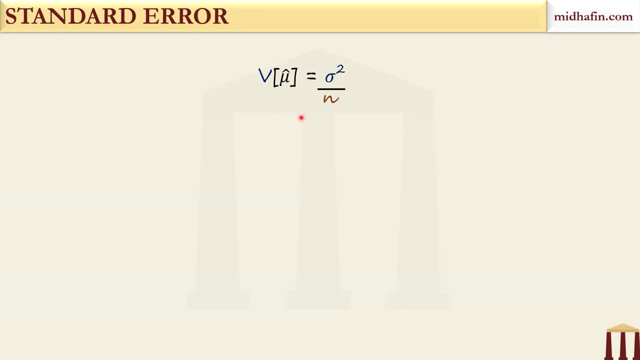 okay, There is an example in the video. we have done that. If you want, we can add that in the PDF also, where we have this Co Co-skewness measurement. have interpreted the co-skewness and co-curtosis with respect to gold prices and stock prices. 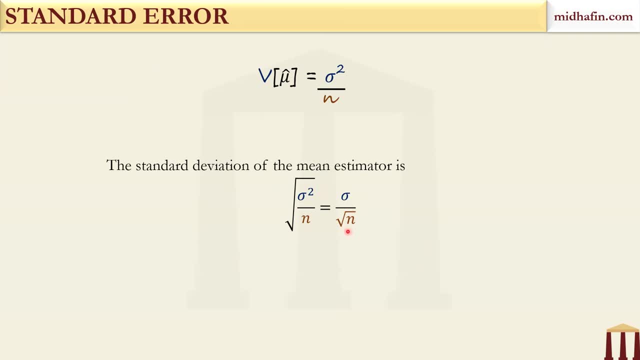 and bond prices and crude oil prices. So four instruments were taken and the interpretation was done properly. okay, You can refer to the guard book also for that Same example was taken. okay, Or, if you want, we can add it in this revision video for you, fine. 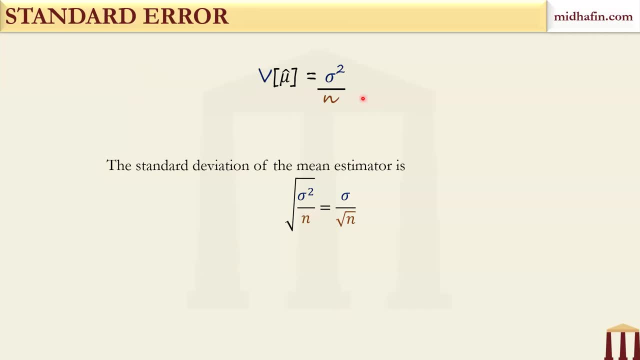 Okay, so let us take a short five-minute break. We can resume at 3.27.. Hypothesis testing is a very important topic, So we will discuss from 3.27.. It might take a little more time than the previous topic. 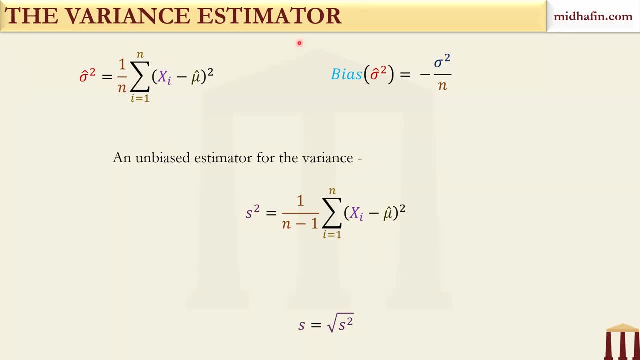 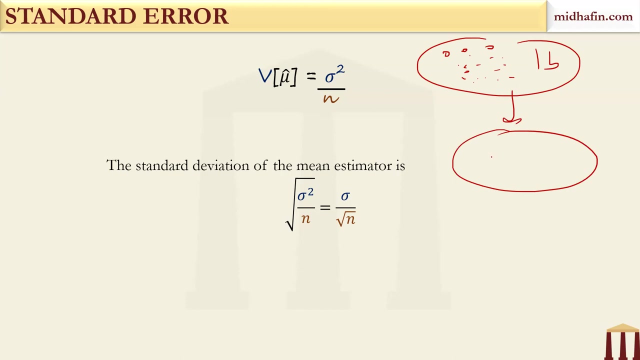 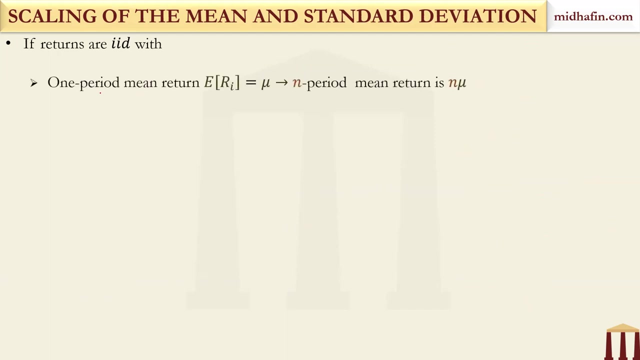 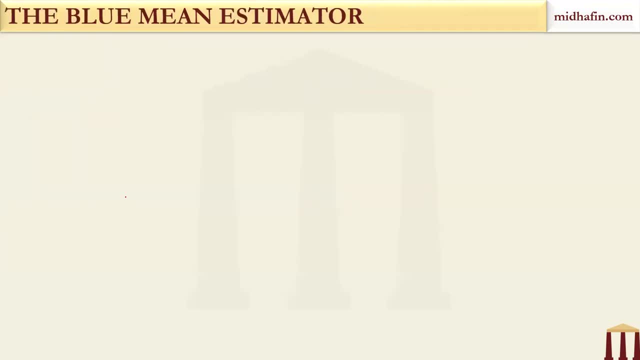 For this also, I think we will cover quickly. We will just discuss some examples, Because the standard, normal distribution and everything has already been covered. Okay, now confidence intervals. Okay Again, we are not discussing this in detail, So we are relating specifically to direct questions or concepts which can be asked in the exam. 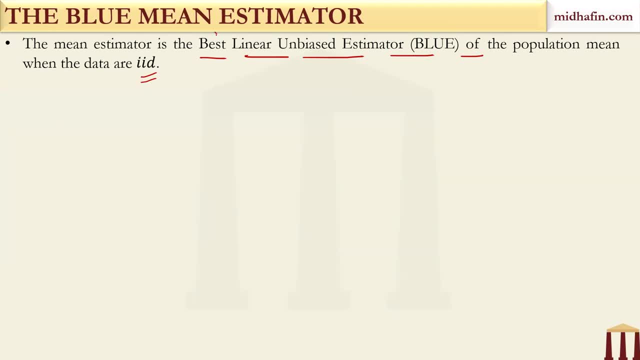 So what are confidence intervals? Confidence intervals: they take on the following form Because confidence intervals we already introduced in when we discussed normal distribution right 95% confidence interval, 68, the 99, and 90. So they take this form: point estimate plus minus reliability factor times, standard error. 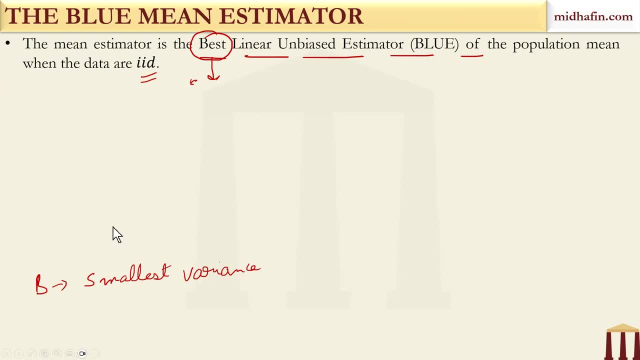 Okay, now let us say, if you are having normal distribution with a known variance, then a confidence interval for the population mean can be calculated like this: In this case, the reliability factor becomes the critical value of the Z-statistic. And since we are talking about confidence interval, are we interested in one-tailed critical value or two-tailed critical value? 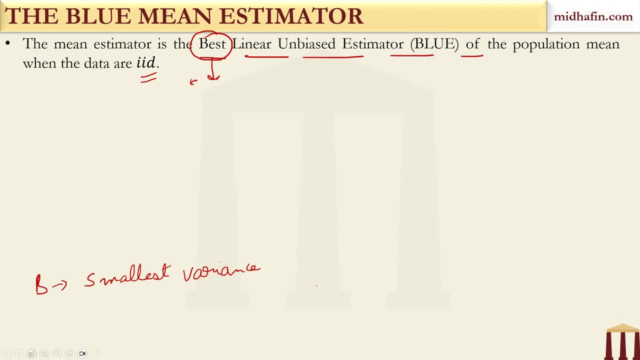 What do you think? Okay, Generally we are interested in two-tailed critical value for a confidence interval, But you would be surprised to know that even confidence intervals can be created from negative infinity up to a particular value. So in fact, we can also have one-tailed critical value usage as well. 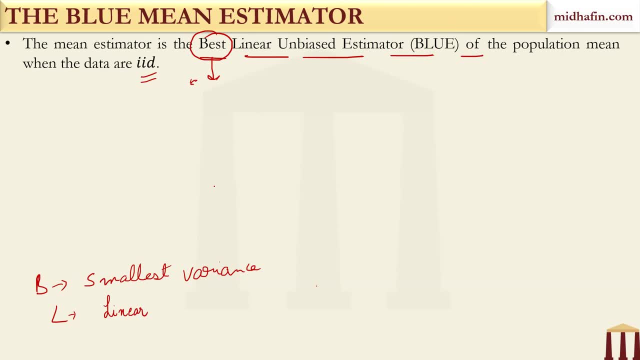 Okay, Although those kind of questions are not asked in the barium curricula. But even that is possible Because the interval means I mean you can also start from negative infinity up to a certain point. That is also an interval. 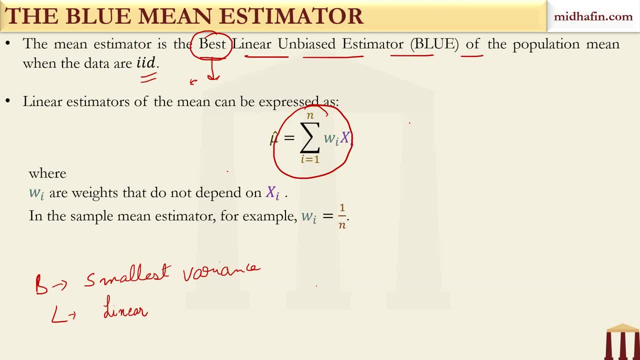 So this is what confidence interval for Normal distribution will look like. Now, which critical value to use, Z or T? There is always a choice between the Z-statistic and the T-statistic. Now this is a table which summarizes what kind of statistics should be used: which is preferable, which is permissible. 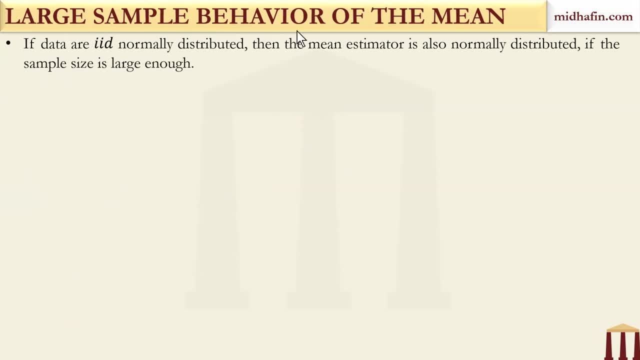 Now, if distribution type is normal and population variance is known, then in that case, irrespective of the sample size- because you already know that the distribution is normal, So there is no problem with the sample size- You can directly use the Z-statistic. 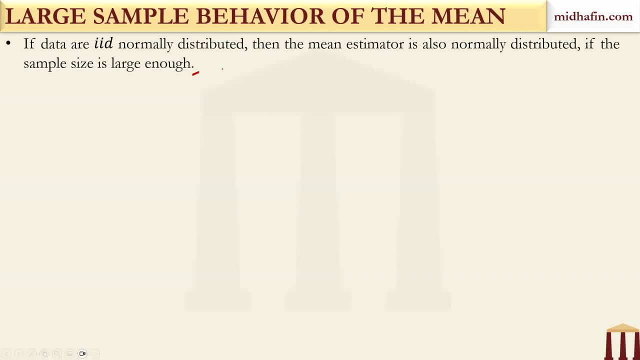 Population variance is also known. So you can also use the Z-statistic If the distribution type is non-normal and the population variance is known. in that case you have to check what is the sample size. If sample size is greater than or equal to 30, then based on the central limit theorem, 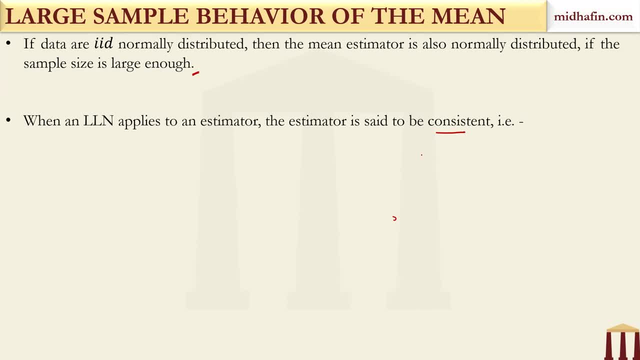 you can approximate that it will behave like a normal distribution. So in that case also Z-statistic can be applied. But what if N is less than 30? In that case you cannot apply any of the statistics because the distribution type is non-normal and N is less than 30.. 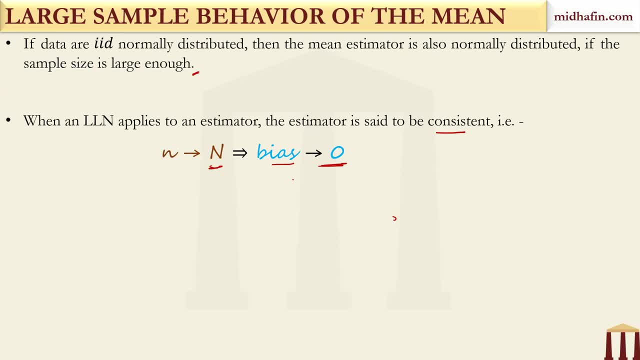 So it is not possible for you to apply any statistic If the distribution type is normal, but the population variance is unknown, in that case this is preferable. T-statistic Is preferable, But Z is also permissible. Okay, And in this case, if N is less than 30, then you have to use the T-statistic. 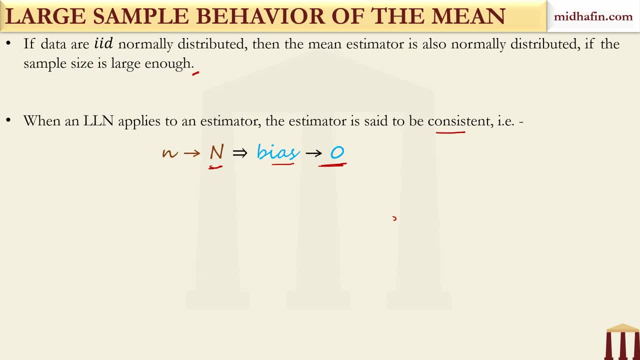 If the population is non-normal, population variance is unknown, sample size is greater than or equal to 30, again the same thing: T-statistic is preferable, T-statistic is preferable, Z is permissible, And if N is less than 30, then you cannot apply any of the statistics. 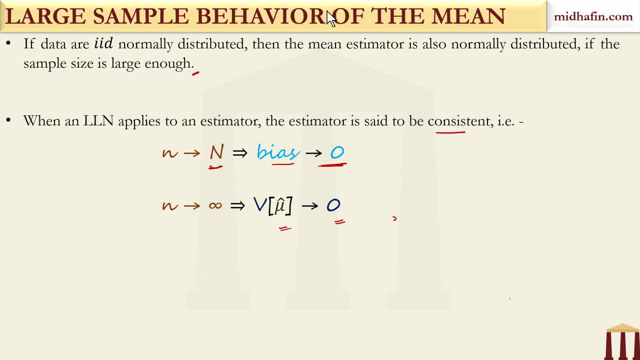 Now remember one thing: that in this particular chapter we are only dealing with Z-stats. T-statistic hypothesis testing is going to be discussed and is applied in case of hypothesis testing of linear regression parameters, slope and intercept. So when we test for slope and intercept in case of linear regression, then we use the T-test most of the time and we use the critical value. 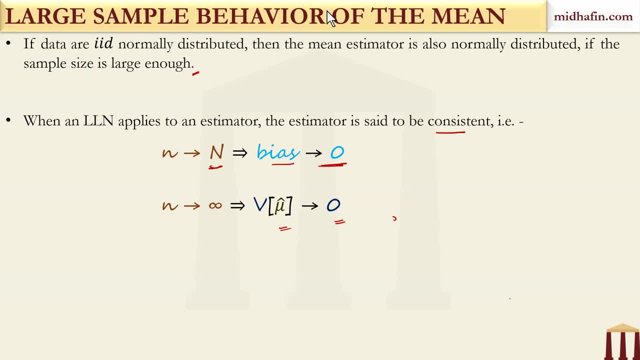 with the T-statistic. Okay Now, although it is not necessary, but the null hypothesis H0 is generally constructed, which the researcher wants to reject. So, for example, if I believe, if I'm a researcher and I believe that the mean return of any stock is greater than 10%, or say 5%, 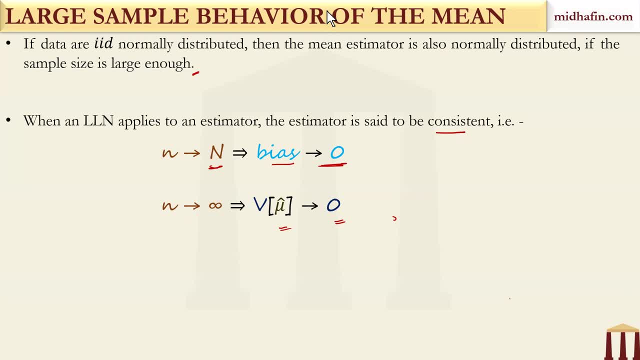 then how? Then? how will I construct the null hypothesis If I believe that the return is greater than 5%? that is my belief. So I will construct the null just opposite to that. So this will be my null hypothesis: HA less than equal to 5 or 10, whatever. if you believe 10% it. 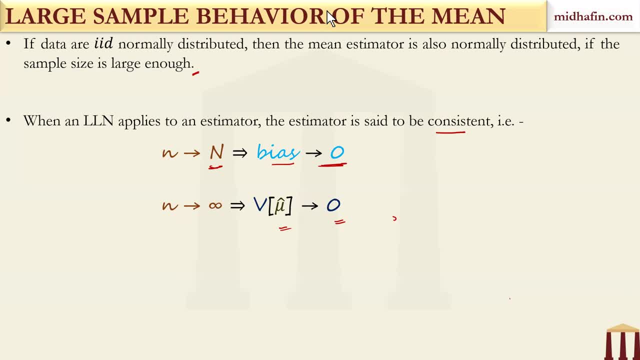 will be 10%. Got it So less than equal to 10% or 5%? Okay, Now, based on the results of the test, if there is a very high probability of the return being greater than 5%, then you can reject this null And you will say that, okay, you were reasonably confident. 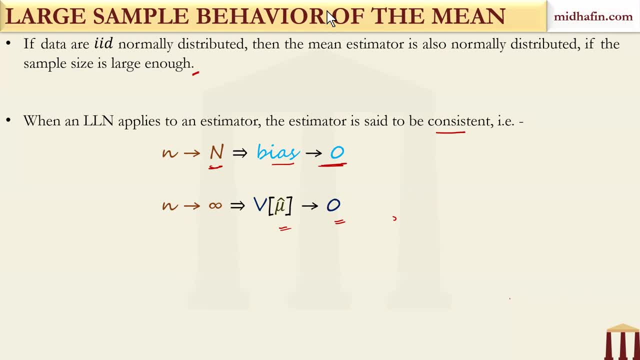 that your return. your belief is not incorrect. Your belief is correct. Okay, Now, one thing is very, very important: The null hypothesis is never accepted, Never. We never say we accept the null hypothesis. It is either rejected or fail to reject. 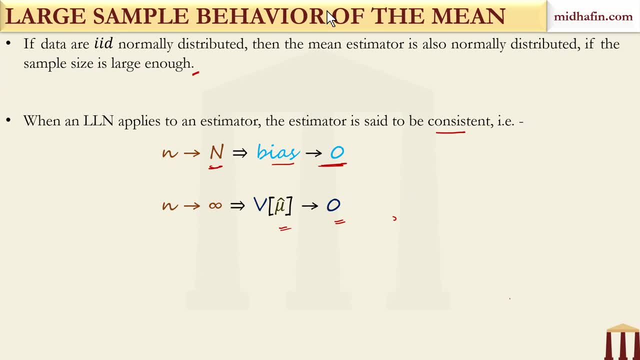 You never say if you could not reject it. you will never say you accepted it, You will say you fail to reject it. I always use a courtroom example for this And it's the best example, I think. to start with, because when any accused is not convicted, the accused 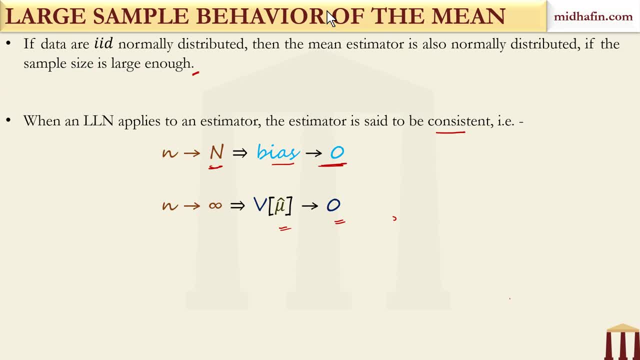 is coming to the court and the accused is not convicted, Then what does the court pronounce? Does the court pronounce that the accused is not guilty? the accused is innocent. The court, in fact. you've seen many movies: Hindi, English or any other language: The 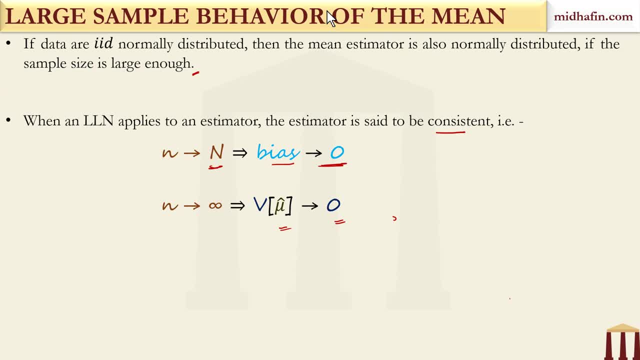 court never pronounces that the accused is innocent. We are letting go of the accused because we believe that the accused is innocent. Never, The court says that, yes, due to lack of reasonable evidence. Okay, Because the accused has to be accepted. The court says: 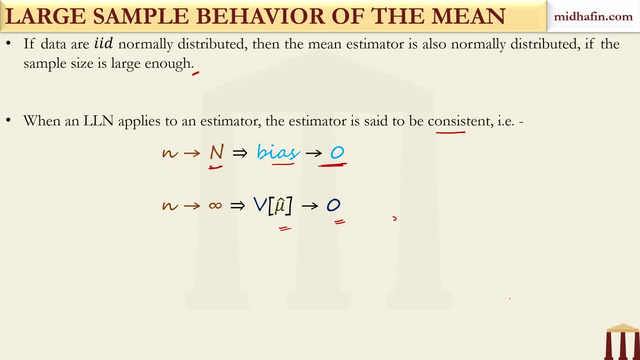 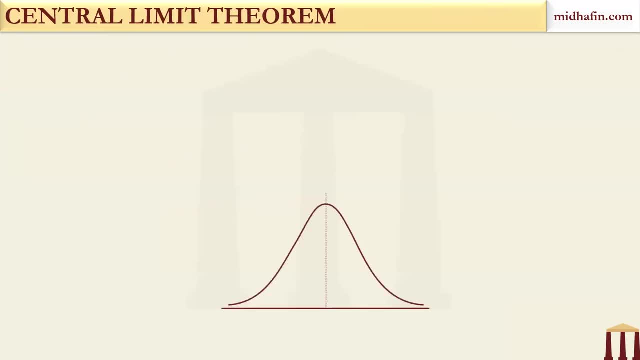 that the accused is not guilty. It is established as guilty beyond a reasonable degree of doubt. So the court will never say that the accused is innocent. That's why the court is releasing the accused, No, The accused. there is a lack of evidence. The prosecution may be failed. 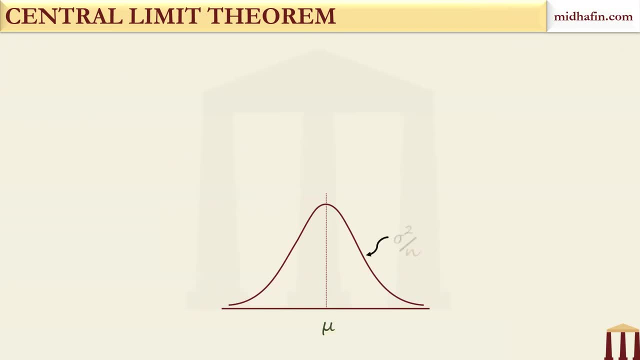 to give sufficient evidence. So, due to lack of evidence, the guilt of the accused cannot be proved beyond a reasonable degree of confidence. Okay, The alternative hypothesis is that if the accused is not guilty, then a reasonable degree of doubt everything that you've said in the whole case, but the argument continues, however. 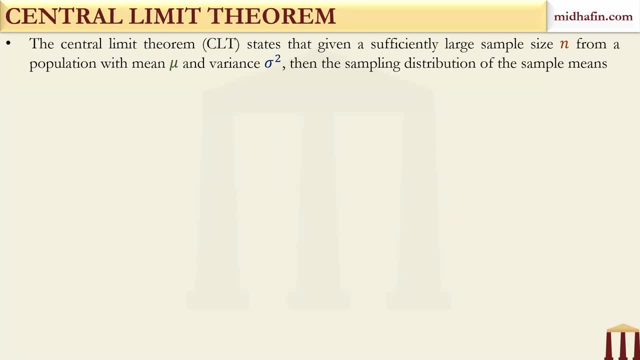 seventy thousand for the εκ ép 8, 18 over 40 рек48ères per year. Let's try to run through it. Let's go through it first one thing with a very typical one, which is that the court provides, written in exactly opposite terms, as the null hypothesis and is concluded if there is enough. 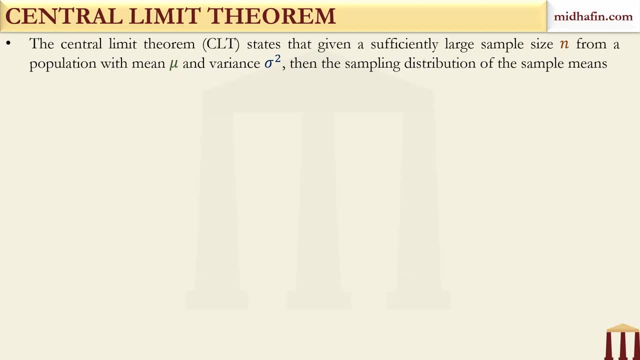 evidence to reject the null hypothesis. so in this case, alternative will be greater than five percent. okay, now. two-tailed test for a one-tailed test. so let's talk about two-tailed test. let's talk about a 95 confidence or a five percent significance. two-tailed test now. earlier the 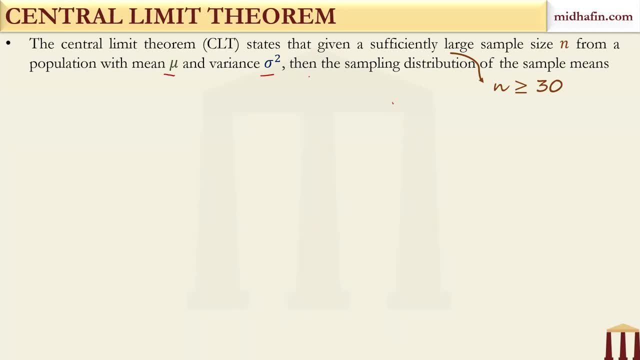 confidence level was if 95, then this five percent was termed as significance level. in the new curriculum they have termed this as a term, this as the test size. so remember, whether it is significance level or the test size, the implication is the same and i don't think there. 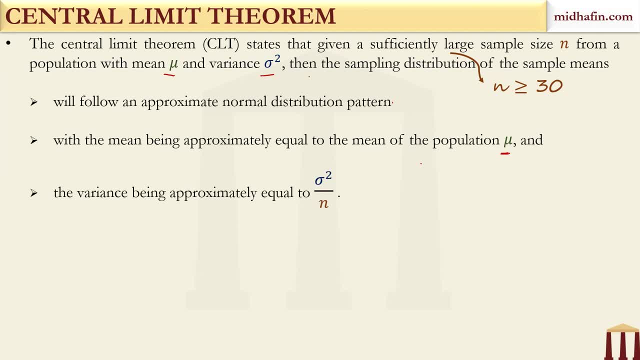 was any reason to change the usually adopted convention of significance, because mostly in most of the cases it's mentioned significance level only in most of the other books. so i think it would have been better if they continued to use significance level, but probably they would use test size in the exam. now, what are the keywords? 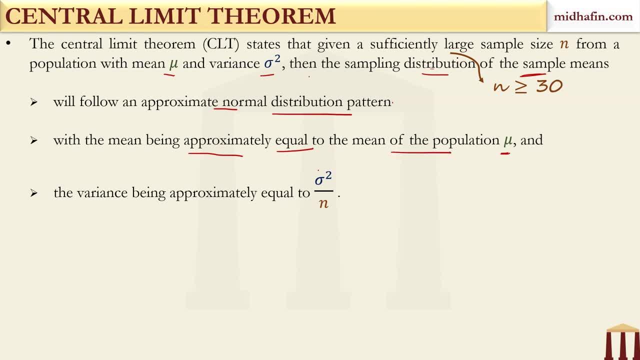 in the question which you can use to identify that this is a two-tailed test. these are the keywords if the question says: test if it is different from something. test if it is not equal to something. test if something had an effect or not so had an effect, can we? 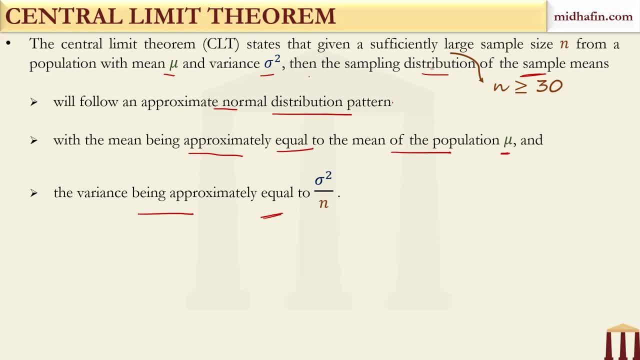 positive effect or negative, not equal to, can be on both sides. greater than or less than different from also can be on both sides. so are you getting the points? these are the keywords which will help you identify which kind of test we are talking about. okay, and this region will be your fail to reject region. this region will be your reject region and. 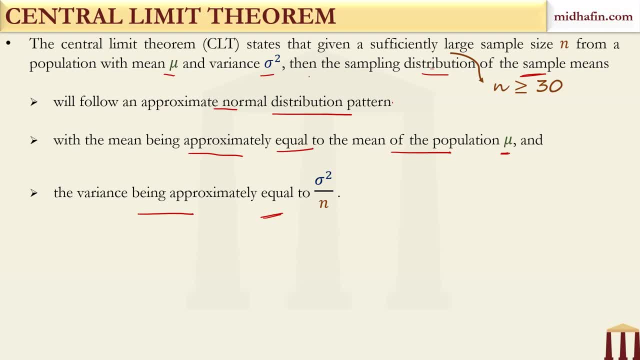 of course, we will discuss one example to make things more clear. so this is the idea behind the two tail test. now let us discuss the idea behind the one tail test, specifically the right tail test. the same idea can be extended to a left tail test. also, what are the keywords? 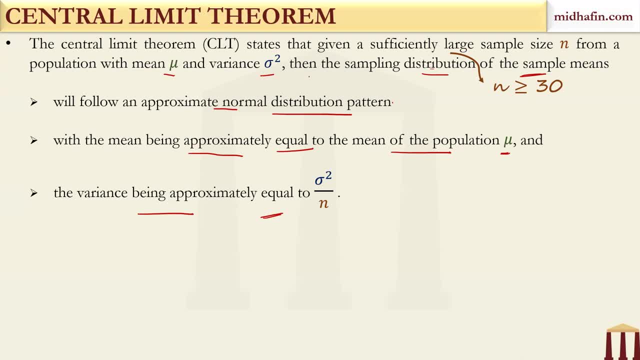 the keywords will be: for a right tail test greater than, and for a left tail test less than, or at least, or at most. all these keywords will be there. even for a right tail test, the keywords can be less than. you have to be very smart and choose. uh, you'll be able to understand. 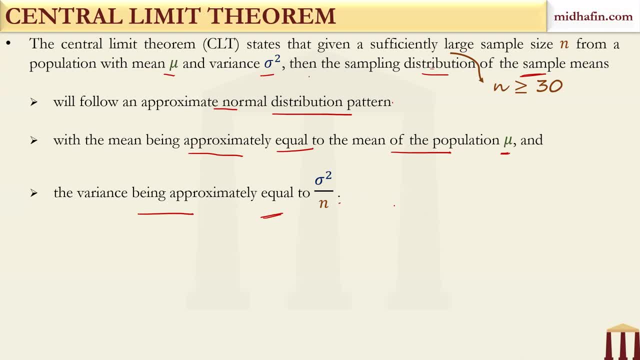 when you look at the question carefully, you'll be able to understand which one is the right tail test. so this is your fail to reject region. this is your reject region. now, these are the steps, steps. i'm not going to go in detail. in fact, i have curated the steps. 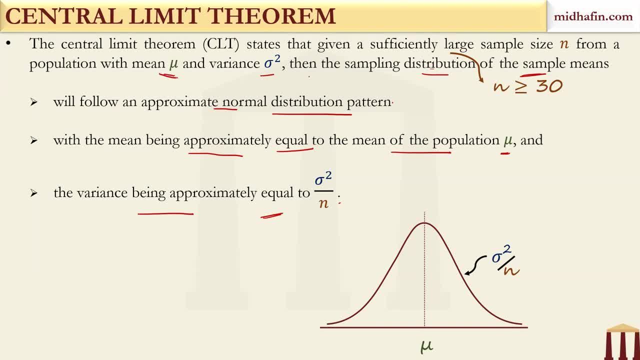 and this. these are not the standard steps which are given in the curriculum or any other book, so i've actually modified the steps a little bit so that steps are included properly, so that you can understand when to go back to which step. okay, select the appropriate test. statistic specify. 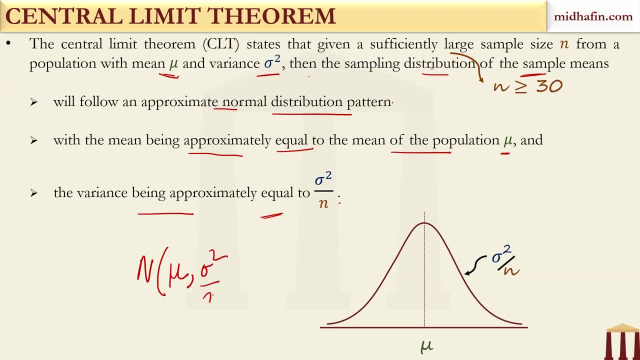 the critical value of the test statistic based on the significance- let us state it in steps two, okay then- and also based on the notion of the test. so, whether it is two tail test or one test, these things are important- then state the decision rule regarding the hypothesis based on the. 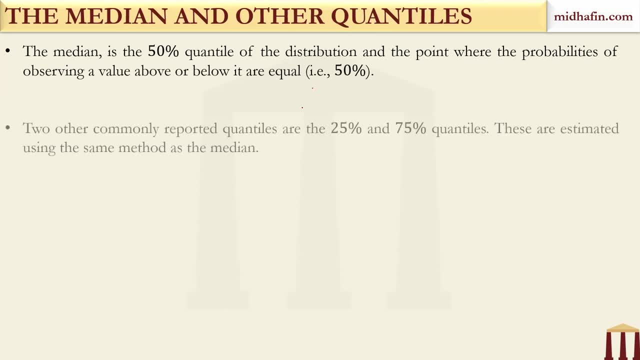 critical values specified in step three. again, you go to step three, then sample test statistic, then make a decision based on which two steps also i've given, then draw a conclusion based on which two steps. so this is a modification. go through this once you get the pdf. okay, we'll directly. 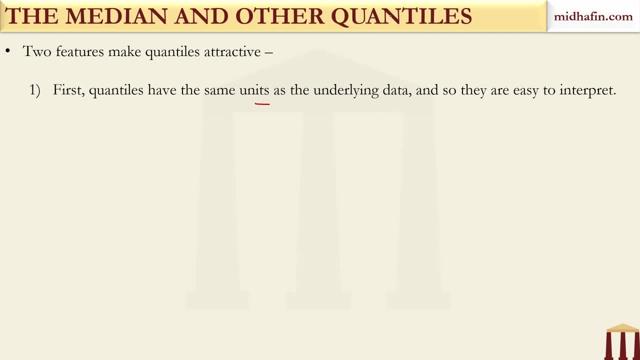 go to the example. so let's discuss only one example, and in the pdf i'll be uh sharing two more examples. okay, a left tail test also, and a two tail test also. so read the question. an electric bulb manufacturer claims that the average lifetime of bulbs produced by it is more than 36 months, with a standard deviation of three. 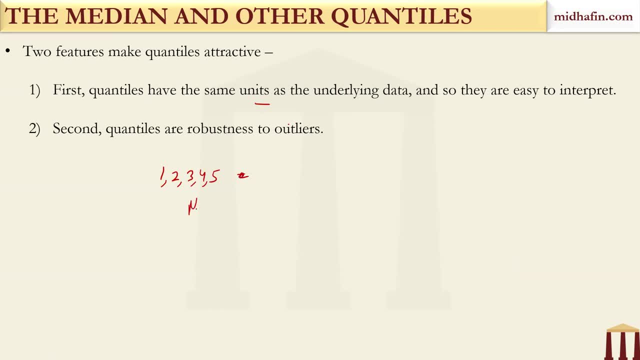 months. a random sample of 50 bulbs was taken and the average lifetime of those bulbs was found to be 37 months. test the manufacturer's claim at 5 percent level of significance. so tell me one thing: if suppose you take a random sample, the claim is: 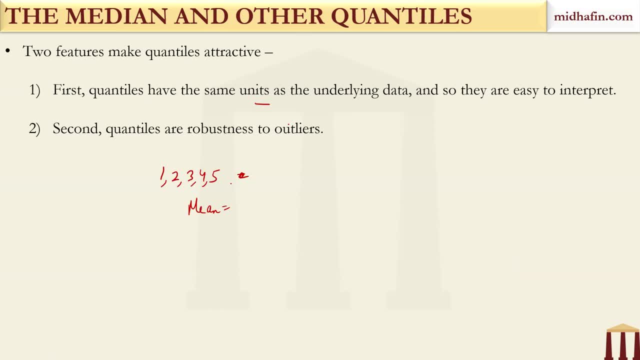 that the average lifetime is more than 36 months. if you take a random sample and if you find that the average lifetime is 33 months, will you even perform the test? will you even care to perform the test in that case? because, see, we always do hypothesis test and all, but do you need to perform it every time? no, in any case, it's the, the. 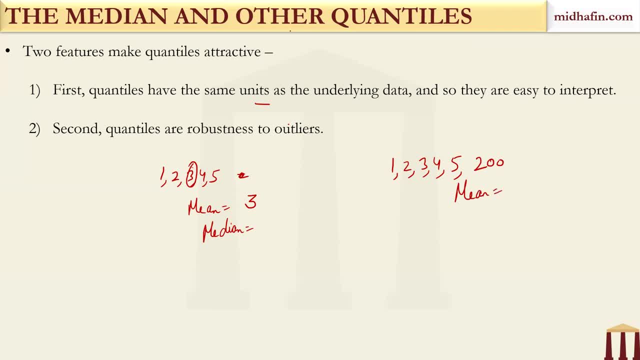 claim has been, you know, violated in the sample. you only perform a hypothesis test. i'm repeating: roid, see, you see, this is the claim: more than 36 months. okay, this is what manufacturer is claiming. you are the person who's testing the claim. okay, you go there and you take a random sample of 50. 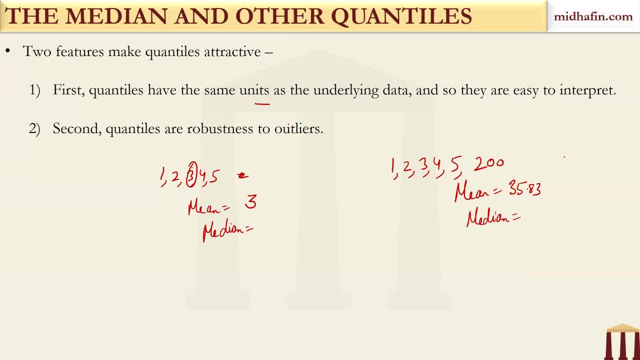 bulbs. you test the average lifetime of those bulbs and you find it to be 37 months. but if i ask you that, instead of 37 months, if the average lifetime was 33 months, would you even perform the test? do you even need to perform the test? no, because the 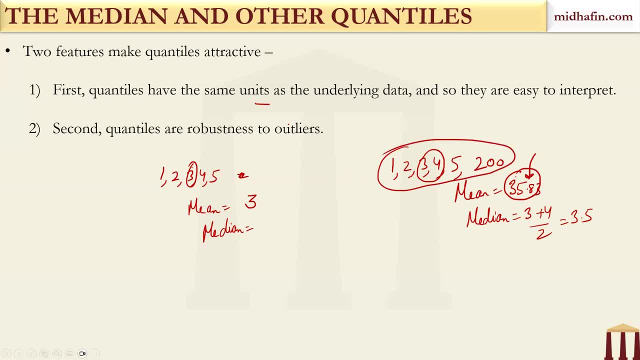 claim is 36. you will, yes, i will, repeat the keywords. absolutely, i will, i will. i will need to do so. why this is a one-tail test. we'll discuss that. so the average lifetime, if it is fine to you be found to be 37 months, it means that you believe that. yes, okay, there is some merit in the. 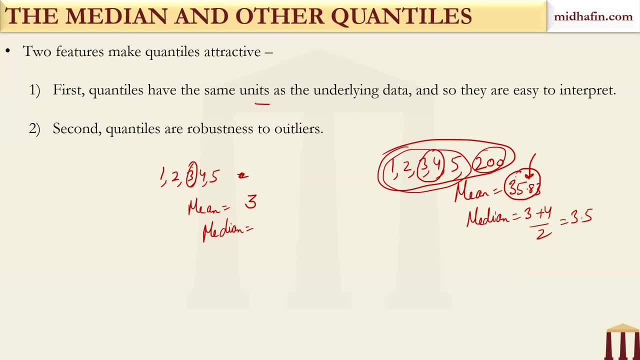 manufacturer's claim. the manufacturer is claiming more than 36. i've got 37, so there is some merit. let's test this claim. okay, now what are the keywords which will tell you that it is a one-tail test? what are the keywords? what? what did we discuss, niyarika? these were the keywords. 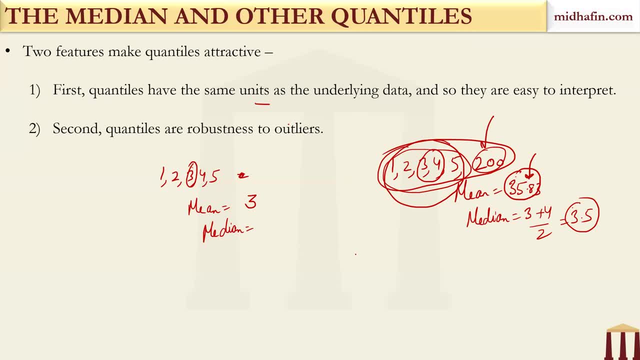 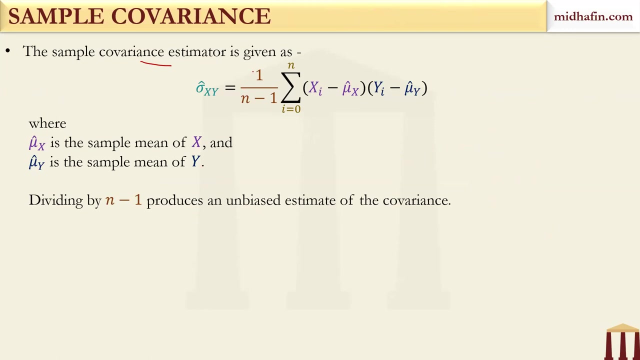 greater than less than, or more than less than, at least at most. okay, so can you see some some related keywords in this example? can you see some related keywords in the first line itself? very good, see, niyarika, got it, got it, niyarika. can you see this more than? 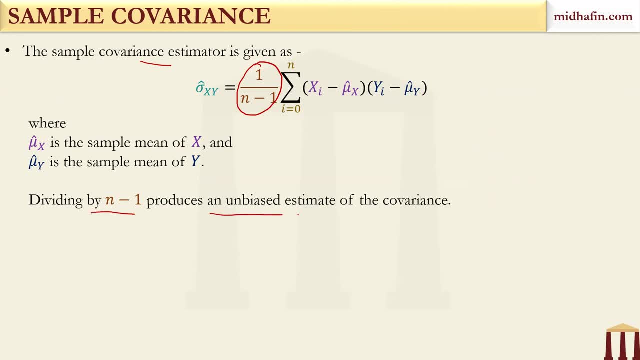 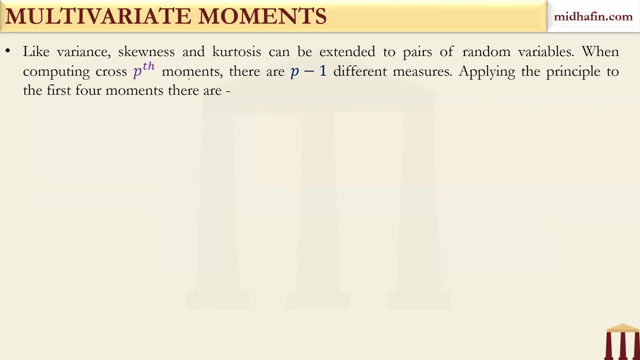 so the claim is that it is more than something. it means you have to test in the right tail. got it okay? so you will perform a right tail test now, you will test and you start by using the first step. so let's go back now. that's why i did not discuss, so we'll discuss it using the example i said. 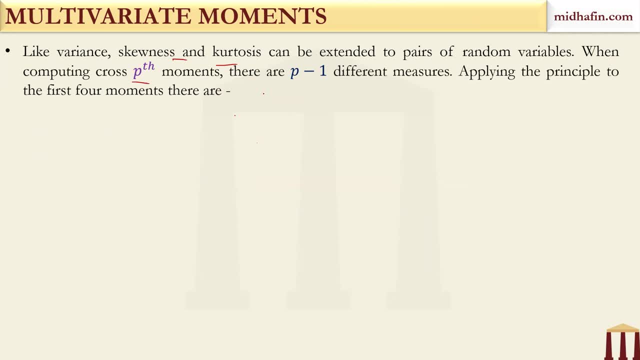 so first step is: state the hypothesis. state the hypothesis. what is your null? what is your belief? tell me if, as a researcher, you have found some merit in the manufacturer's claim. your belief is: maybe the manufacturer is correct, let's test it out. so you also start to believe that, yeah, the 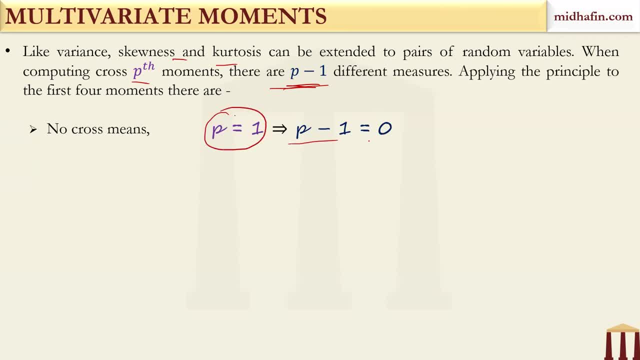 average lifetime is more than 36 months. so what will be your null and what will be your alternate? i said that generally, the null should be something that you want to reject generally, so let's go with the general convention. yes, mu is less than equal to this is what you want to reject. 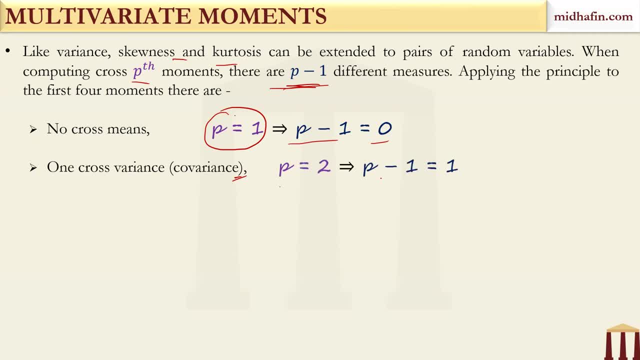 and this is what you want to believe, right? so again, just like i mentioned my way for writing conditional probability, i mentioned that i write given first when i write conditional probability today earlier in the conditional probability discussion. so in this case also, i tend to write the alternative hypothesis. 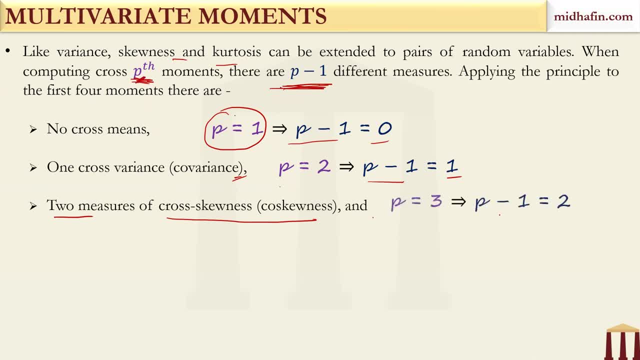 first when, as a student, i am saying when i started studying frm for the first time in 2011, i actually uh, wrote the alternative hypothesis first because it made me more comfortable. i don't know why. so if it works well for you, then it's great, because, whatever you believe, 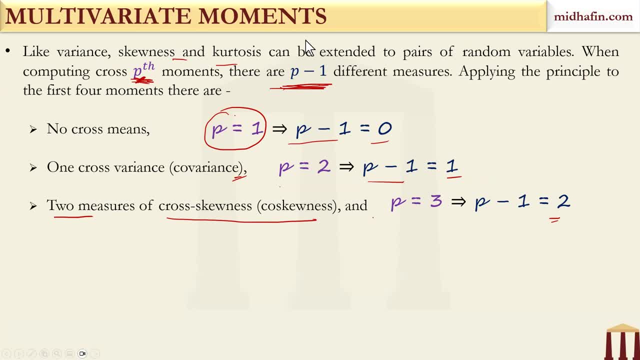 that you have to write in the alternative and the opposite. you're writing the math, so we know that it is a right tail test, so we draw this diagram accordingly. okay, next step. next step is to specify the level of significance, test size. is it given in the question? 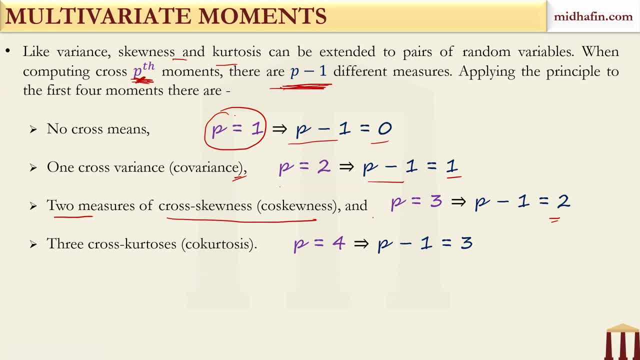 what is the test size? even if it's obvious, please say correct, no, no, test size, significance level: five percent, five percent. see, that is why i said they should not have no changed it to test size. they should have written significance level only. so test size is 0.05 or significance level is 0.7. 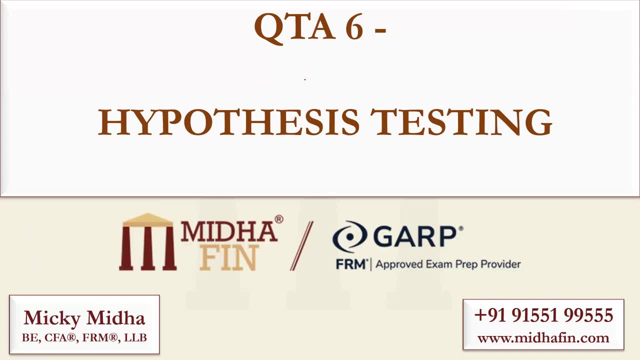 third step: select the appropriate test statistic and specify the test size. so we will specify the critical value of the test statistic based on the significance level stated in step two. so we will specify the critical value based on five percent significance level and also based on the notion of the test, whether it is a two-tail test. so we'll give a two-tail. 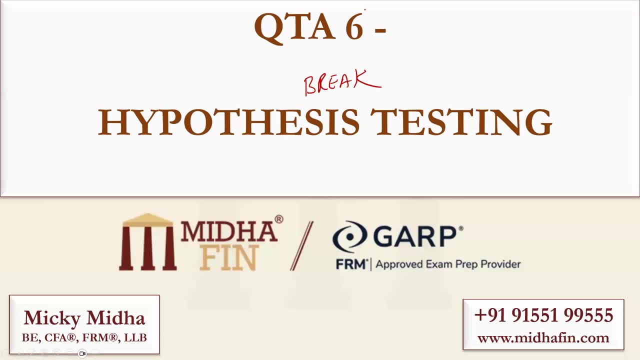 critical value. if it's a one-tail test, we'll give a one-tail critical. now tell me one thing before we proceed, i mean how to decide which test we will use this table, refer to this table for the test. so distribution type, population variance and sample size. now let's go to. 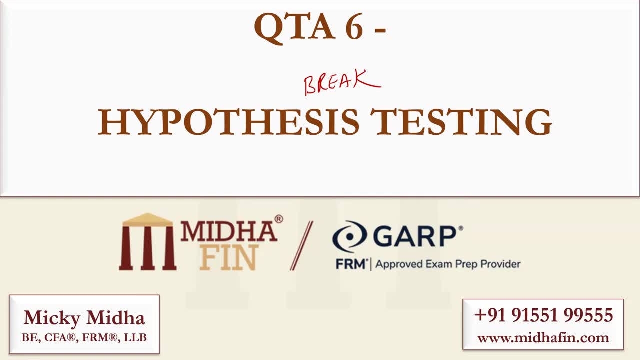 the sample size. is sample size more than 30? is sample size more than 30? yes, it is 15. and also, is the population variance known? also yes, because it is given that this is for the population only. it is not for the sample. see for the sample standard division. 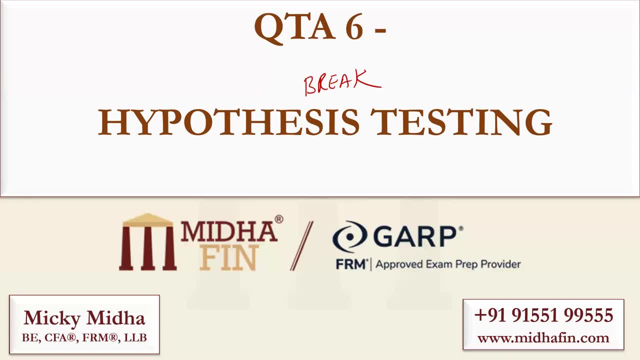 is not given. it is given for the population. only. the manufacturer is claiming that his all the bulbs are having a. the average lifetime of all the bulbs are having a standard division of three months. so you know the population variance, you know the population standard division and you also know that the sample size is greater than equal to 30. you are free to use. 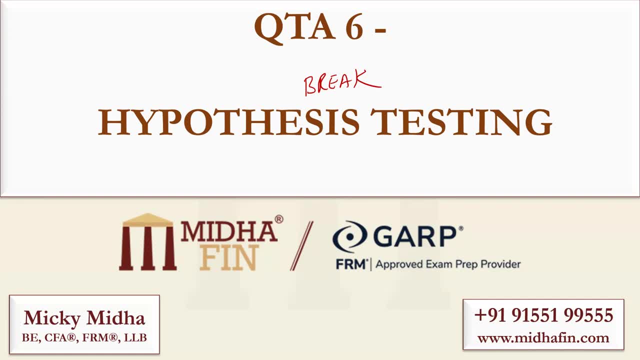 the z test. okay, even if that is not the case in the exam. if they don't give you the t table, perform test only so you have the z test. and can you tell me what is the critical value of the z statistic at five percent level of significance? one tail critical value. 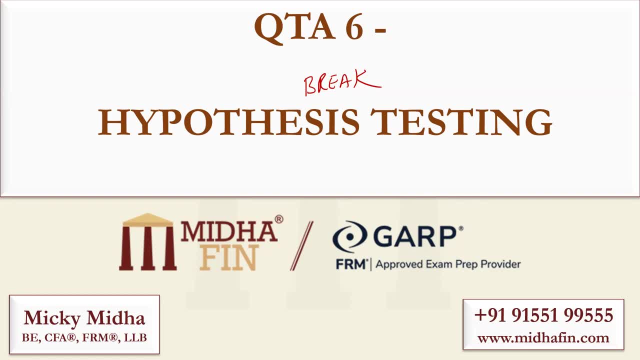 we will use the one tail critical value. one tail critical value. what is the one tail critical value? very good, one point six four five. so one point six four five. so this is one point six four five over. one point six four five. so this is one point six four five. so this is one point six four five. 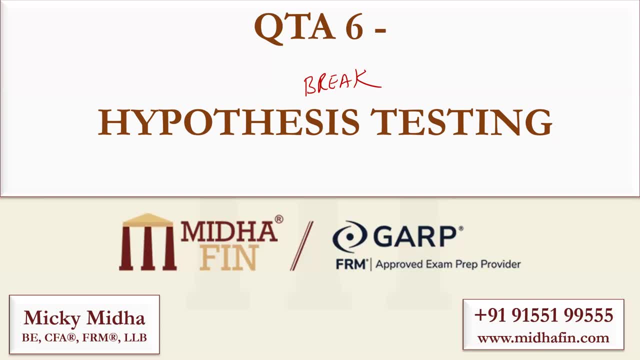 now what is the decision rule? next step is the decision rule. the decision rule regarding the decision rule is that this is the reject region, correct? so reject h naught if my sample test statistic is greater than 1.64. how do i find out the sample test statistic? it is a z test. 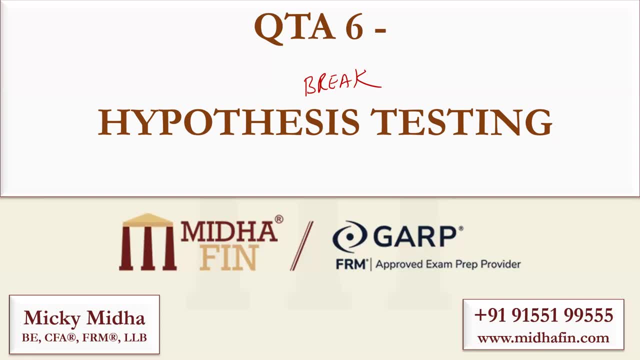 so this will be my sample test statistic: x minus mu naught divided by standard error of x. how do you find out the standard error of x? how do you find out the standard error of x? first, let's find out the denominator. denominator is sx. standard error of x. what was the formula for standard error? 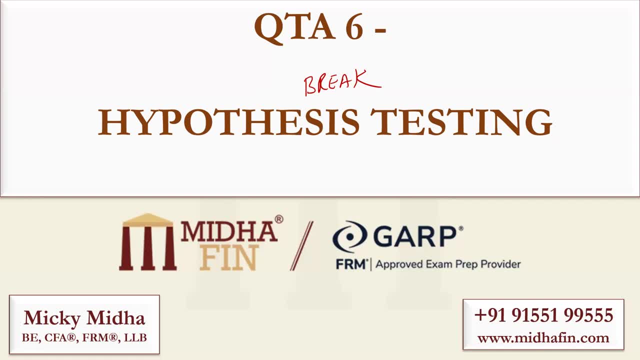 sigma by square root of n. absolutely correct. okay, since sigma is known, you will use sigma directly. if sigma was not known, you you could have used the sample standard division, but the first choice is always sigma. so sigma by root m, which is 3 over root of 50.. 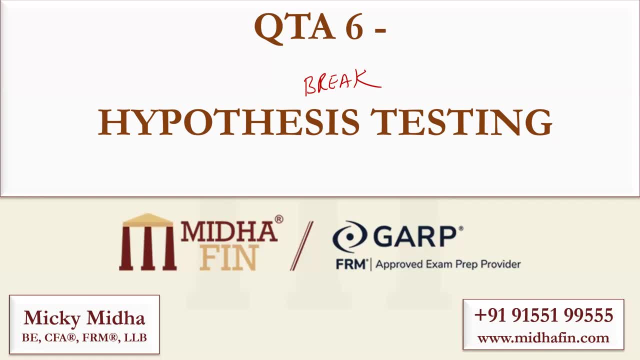 so point four, two, four, two is your sx, the standard error. okay, so let's find out the sample test statistic. now tell me what will be x. see, mu naught is the hypothesized value. remember, mu naught is the hypothesized value. so mu naught is something against which you are testing and it is given in the first step only. 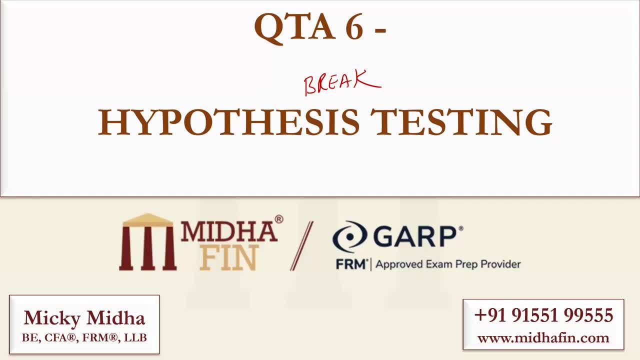 remember if you have to find out mu naught. so there is always a confusion sometimes I see in the minds of the candidates which is x and which is mu. remember mu naught. you will pick from the first step, from the hypotheses, so against the hypothesized value. so mu naught is 36. 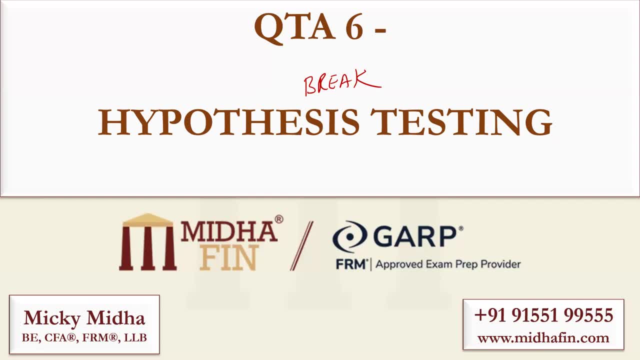 and x you will check from the claim. so what is the claim? sorry, x you will check from the sample. mu naught is from the claim or the hypothesized value x is from the sample. so what is x? absolutely correct, tanuj. it is 37.. 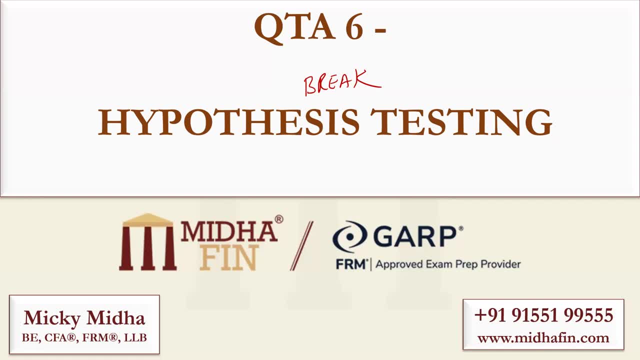 So I am repeating once again: x, you will check from the sample. the data that you got from your sample, mu naught will be your from the claim, or the hypothesized value, whatever you want to call it. So this will be your STS 37 minus 36 divided by 0.4242, which is 2.357. 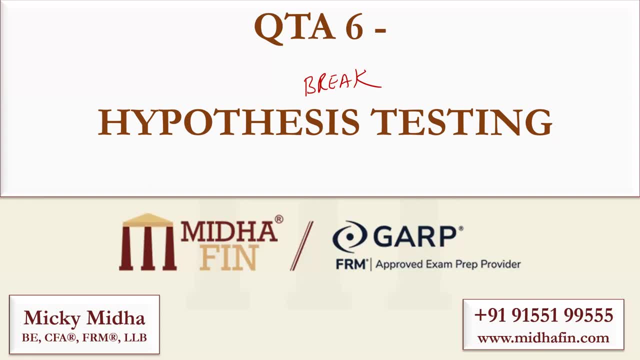 So this is your 2.357.. Is it in the reject zone or fail to reject zone? Reject zone, Reject zone. So, since 2.357 is greater than 1.645, so we will reject the null. Is our question complete or is still one step remaining? 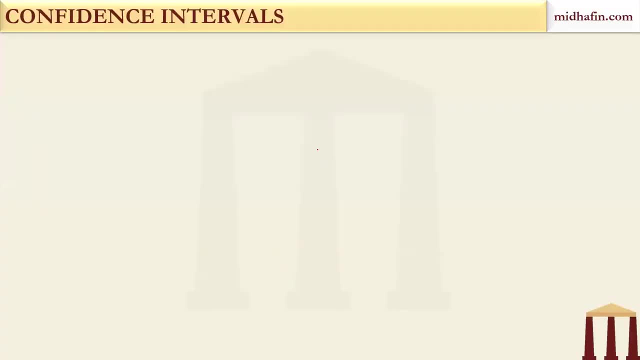 This is only step 6. guys. reject or fail to reject is step 6.. The last step I mentioned: draw a conclusion. So what will be your conclusion? Very good, Very good, Yes. So the conclusion will be that you have sufficient evidence to claim. 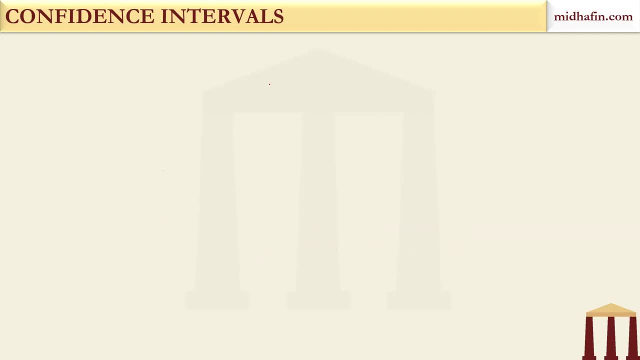 You never see. you should never. I mean being a statistician, you should never give a layman kind of claim that, yeah, manufacturer's claim is correct. Questions might be asked like this in the exam. even options might be like that: 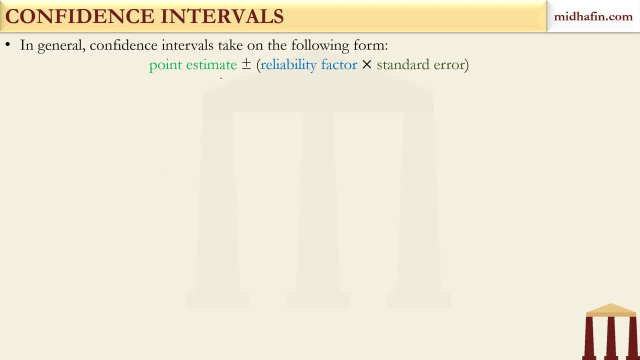 So that is okay for you, but you should always claim like this that you have sufficient evidence to validate the manufacturer's claim at 95% confidence. So this is how you should frame the answer. A few points I want to discuss regarding standard error and sample test statistic over here. 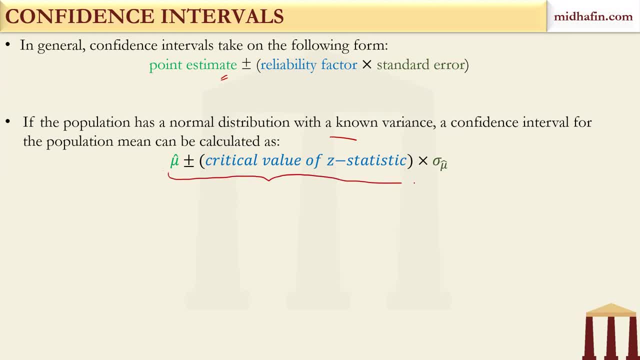 See, if suppose the sample size was decreased to say 35, let's say, If I decrease the sample size to 35, would you be more confident in your results or less confident? What do you think Your degree of confidence will reduce correct? 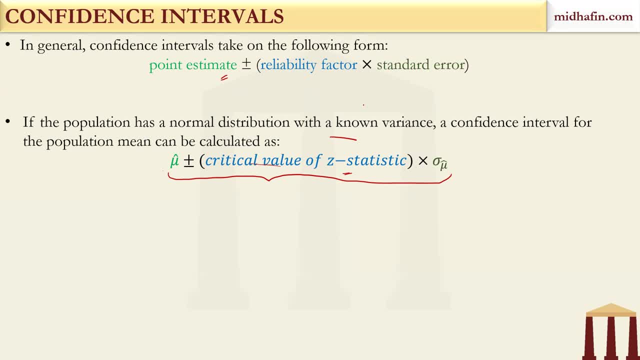 Do you agree or not? The larger sample size you have, the better it is for you And mathematically also it is justified. You see, with standard error, what will happen if n's value is decreased? What will happen to standard error if n is decreased? can you tell me? 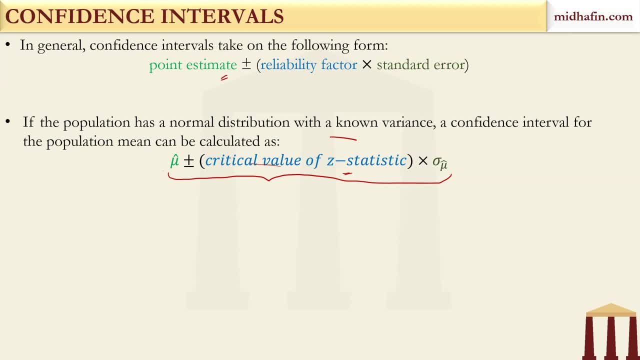 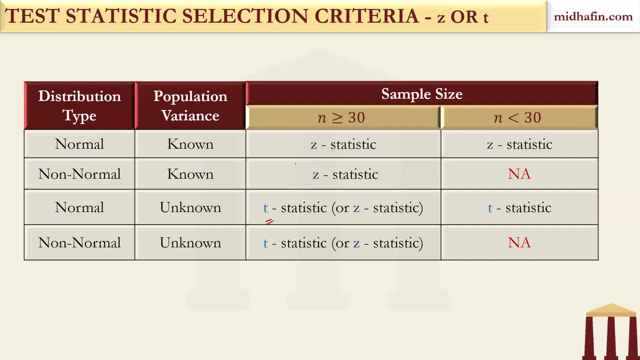 It will increase. It will increase because it is the denominator. So if this increases, it means the denominator increases. and if the denominator increases, what will happen to sample test statistic Decrease? It will decrease, absolutely So because of the sample size decreasing, your sample test statistic also might decrease. 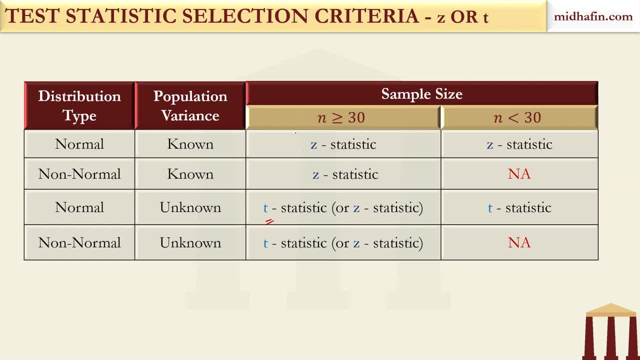 and there is a chance it might fall into the fail to reject zone. Do you agree or not? Because the more number of bulbs you have, the standard error is lesser and lesser, given that sigma is constant. Okay, If it becomes 2.357 over here, maybe your next value will become 2.5 if the sample size 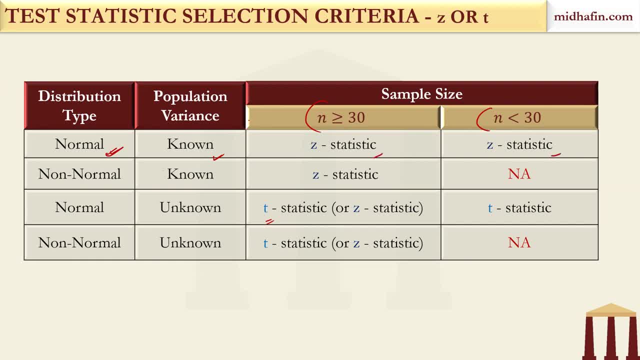 is 60 bulbs. But what if the sample size is 35 bulbs? It will come close to 1.645.. It may even go to the left of 1.645.. So in that case you will fail to reject the null, if that happens, okay. 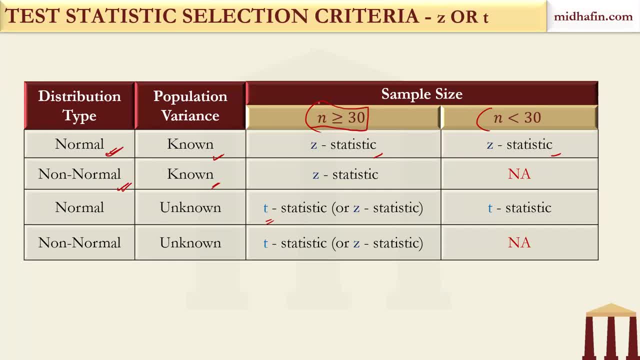 So tell me one thing: If you fail to reject the null hypothetically, what will be your conclusion in that case? That is what I want to ask: Give me a technical conclusion, Okay, Anyone who can say: Give me a technical, proper conclusion. 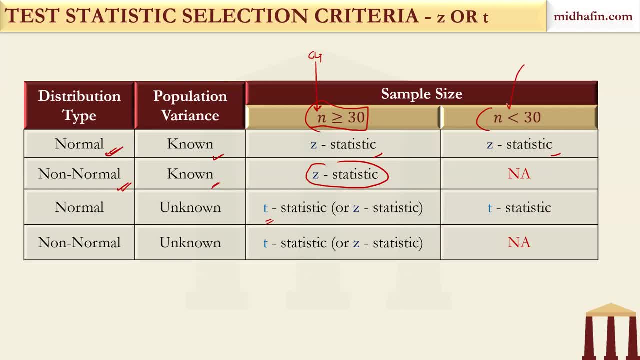 There is sufficient evidence to reject the null. We have Not able to reject the null. Exactly, Exactly. You will never say that manufacturer's claim is not correct. Okay, You will say that you do not have sufficient evidence to support the manufacturer's claim. 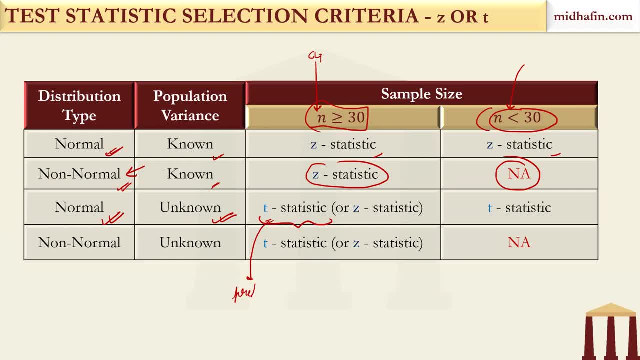 at 95% and confidence. That is the best way to conclude. So that is why we never accept the null. We will never say that we have proved this. No, we don't have sufficient evidence to prove this. We have not proved this, Got it. So that is the whole point. Now one more question I asked you in. 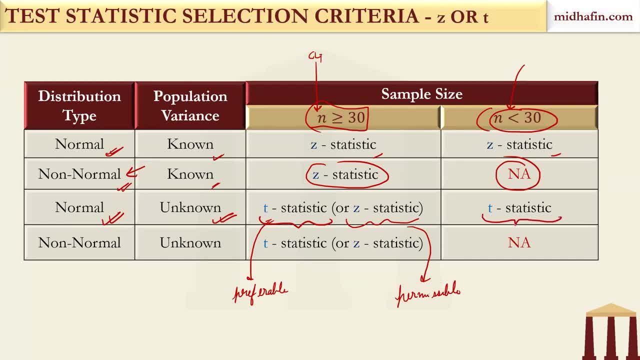 the beginning that if suppose the average lifetime of the sample is 33,, will you even test? You said you will not test and you were absolutely right. Mathematically also it makes sense because if, instead of 37, if it is 33,, what will happen to the numerator? It will become. 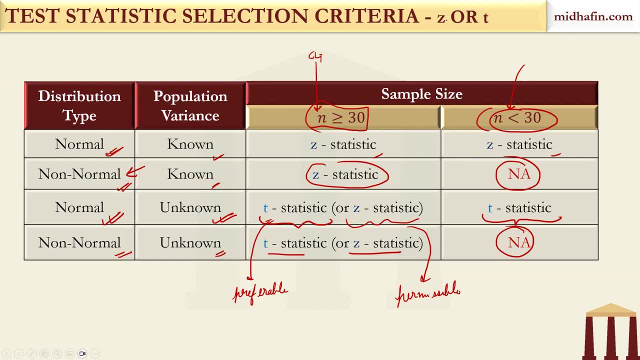 negative. And if it will become negative it will always be in the fail to reject. So there is no point of testing the hypothesis. You will never be able to support the claim right? So mathematically also, everything is justified. Okay, So that is the whole idea behind hypothesis testing. 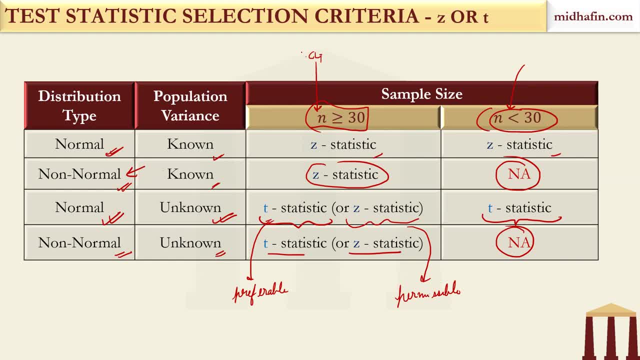 Fine, Now this is another question. I am not going to discuss this right now. Okay, So I am going to quickly go through it. It is a two-tailed test. You can go through it from the PDF. It is better. 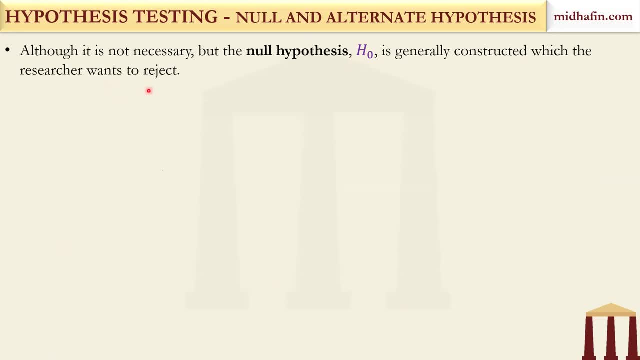 right, Because I think if we have discussed one question, let us proceed to the next part, right? So this is the same way. It is a two-tailed test. The only thing that I want to ask in this question: which keywords Now, Niharika, you tell me which keyword is telling you that it is a two-tailed? 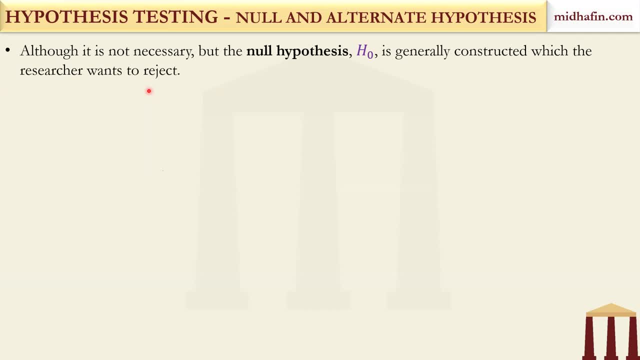 test. Come on, Which keywords are telling you? Keyword or keywords? Niharika, please answer If you are able to fine. If not, then question is open to everyone, Because you had asked about keywords. Do you want me to go back to the keywords slide? I can, No problem. 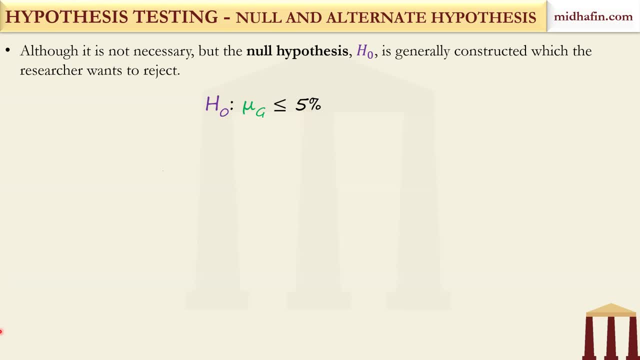 Effect. Very good, Okay, Fine. Someone has already answered. Okay, Fine, Fine, So it had an effect, right, So clear. Yeah, No, it had an effect, Because, see, negative effect means it is only on one side. It is given both positive as well as negative Understood. So over here. 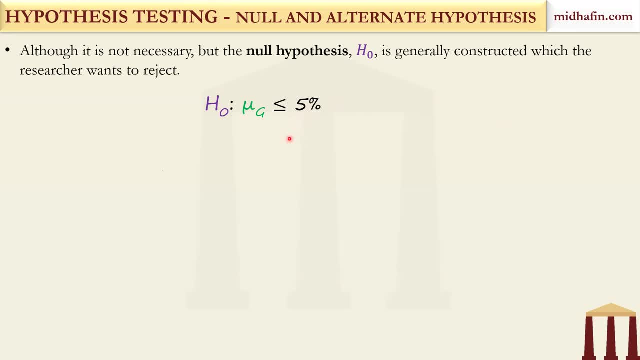 you see, it can have a negative effect or a positive effect, But finally, the main keyword I will say is this, Although over here also in the question, it has been given. But if suppose even these things were not given to you, then it is not given to you, So it is not given to you. 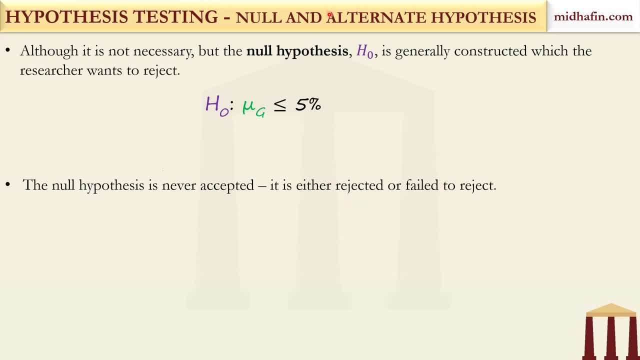 Had an effect is a keyword, because it can have a positive as well as negative effect, And if you go back to the keywords, you will clearly see that one of the keywords was had an effect. Got it Okay, So let us move on. 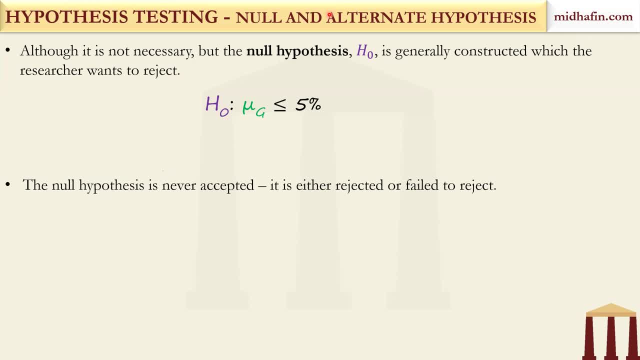 to type 1 and type 2 errors. Type 1 error is rejecting the null hypothesis when it is actually true. And type 2 error is rejecting the null hypothesis when it is actually true. And type 2 error is failure to reject the null hypothesis when it is actually false. Okay, 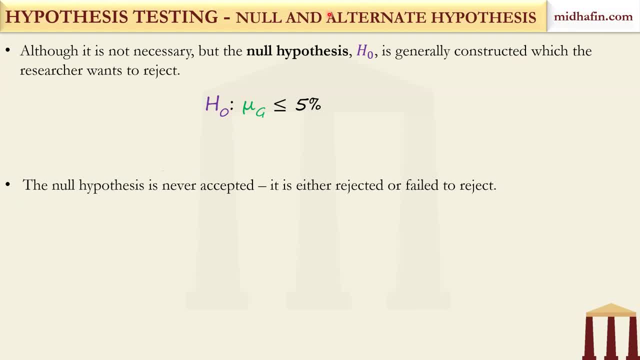 And again in the context of a courtroom example, if suppose an accused, Anyways, I have to state the null and alternative and I have to explain that completely once again. So I will not go into that example. Just remember that rejecting the null when it is actually true. 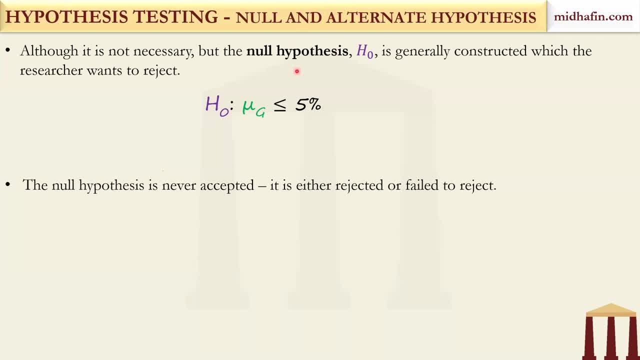 is type 1 error And failure to reject the null when it is actually false is actually type 2 error. So I will not go into that example. Just remember that rejecting the null when it is actually true is type 2 error. Is it clear to everyone? Is anyone having? 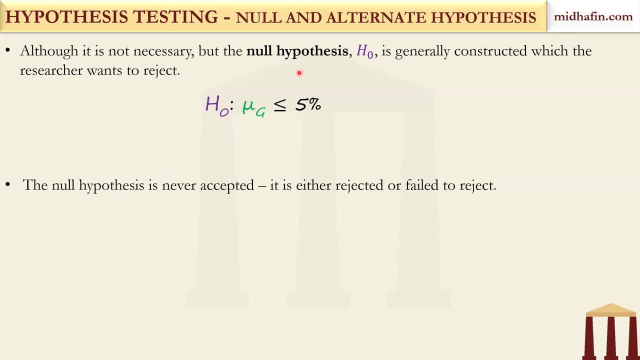 any doubt in type 1, type 2 error. Do you guys need me to explain? anyone who is having any doubt, Then only I will deal with that example, Otherwise I will skip it. Shall we proceed to the next part? Oh, it is. I mean use of type 1 and type 2 error. Absolutely very useful, Because see. 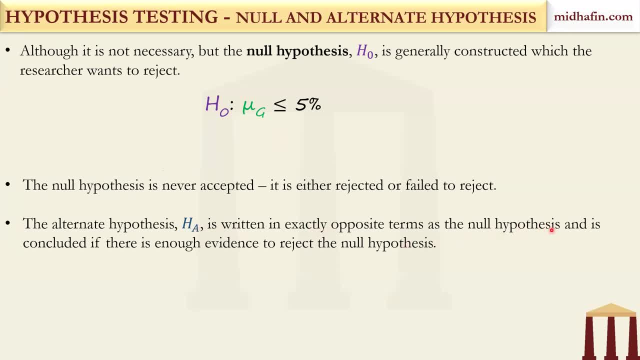 if you are performing a hypothesis, it is still a test, right? You are just being 95% confident, Right, Rohit? So yes, with Redman I am proceeding And I am just explaining this point. that why it is. 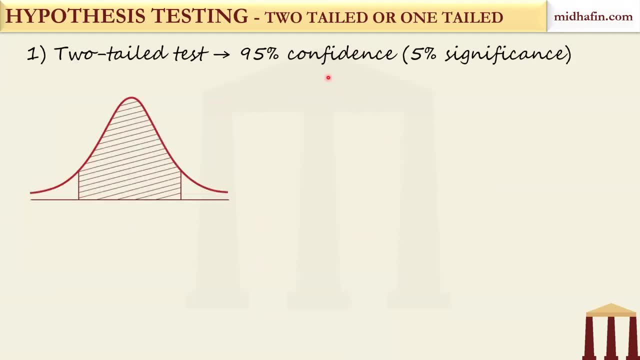 useful, So you are just performing a test. You are not giving a 100% guarantee. right Even you can be wrong, So maybe you actually let us take this example. I think it is a very relevant question. That is why I am giving you a 100% guarantee, So maybe you actually let us take. 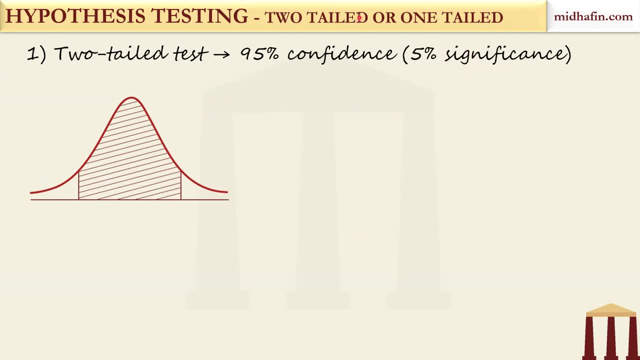 this example. I think it is a very relevant question. That is why I am giving you a 100% guarantee. We should discuss this. So let us say this example: okay, So you actually have rejected the null in this case, okay, But then some other researcher comes and takes out another sample. In that case, 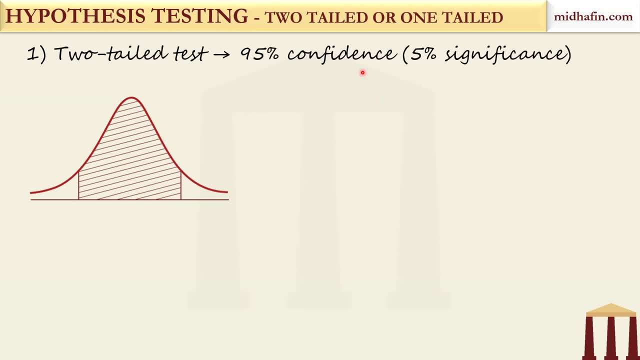 the average lifetime is less than 36.. Another researcher comes: the average lifetime is more than 36,, but the Z statistic is sorry, the sample test statistic is less than 1.645.. Again, the researcher fails to reject. Another researcher, again fails to reject. So it means your results were wrong, Understood. 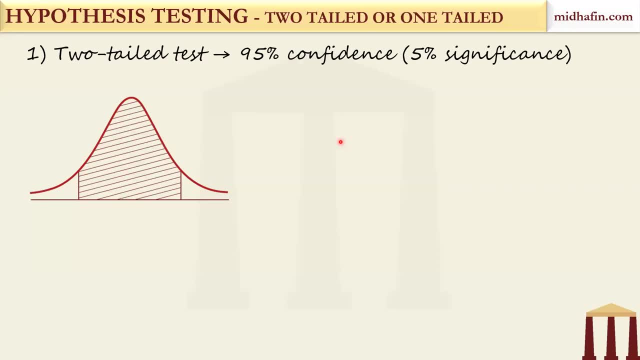 So it is possible that even in a hypothesis test you might be wrong. So these errors are actually telling you, okay, that if suppose you are rejecting the null, then you should not have rejected. So if the court is pronouncing an accused guilty when the accused was innocent, 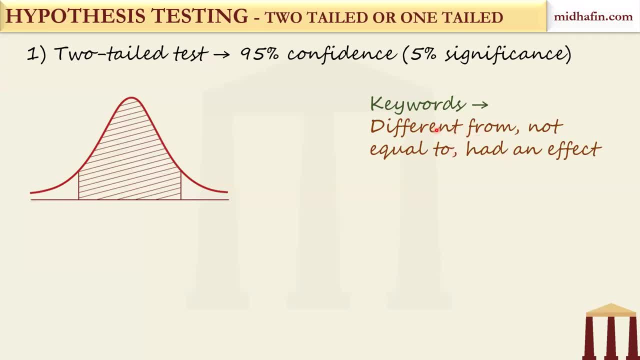 let us say in reality, I mean again, it depends on what is your null and what is your alternative, Because in a courtroom example we always presume- see, you might have heard this term- that innocent until proven guilty. Any accused, if brought to court, that accused is always assumed to be innocent until proven guilty. 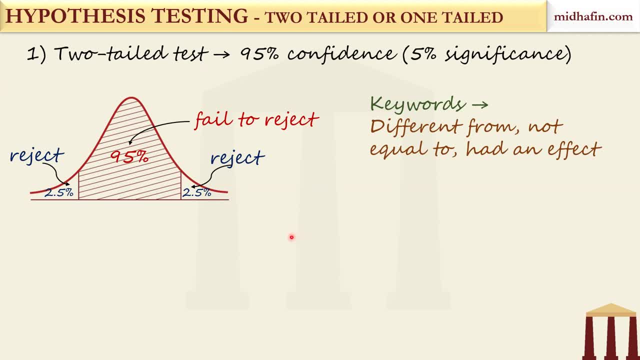 So, based on the prosecution and based on the defense, the null and alternative might be different, but there is always a standardization to it. We actually, when we construct the null- that is why I said about the null and alternative, we always assume that the null and alternative are. 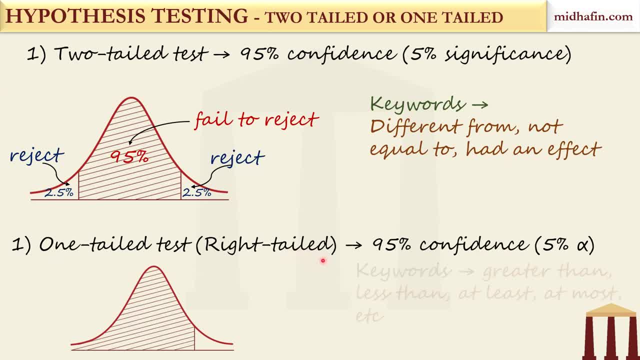 And I have to go into that example. It will take some time, But just remember this, at least the last part of the example. I am not going to the example in detail, But at least remember the last part of the example. So if you are, if suppose someone is innocent and the court has pronounced them guilty. 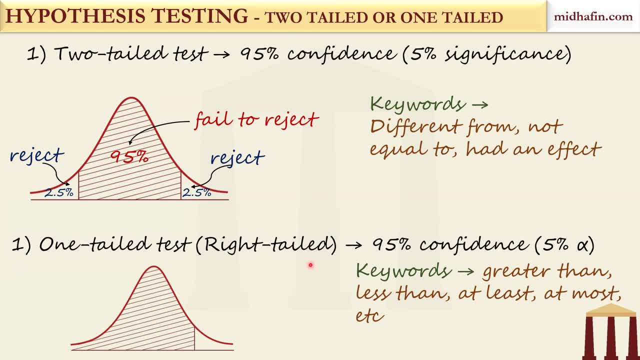 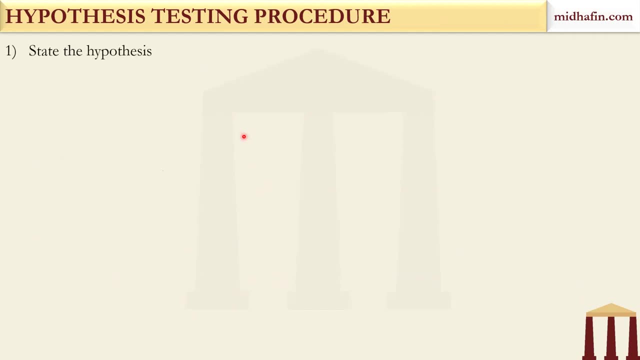 they are making an error right And if someone is actually has committed a crime which even the public knows, maybe there are some celebrities for whom we probably are aware, But the court will not have reasonable evidence right to prove that they are guilty. 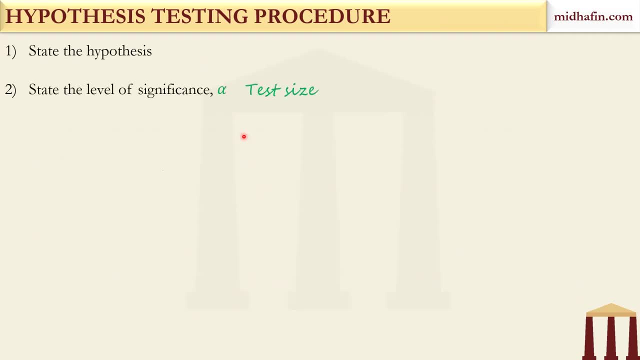 So that is another type of error And, again, depending upon what is your null and alternative, it will depend if it is a type 1 error or type 2 error. Got it. So just understand that if you are rejecting a true null hypothesis, 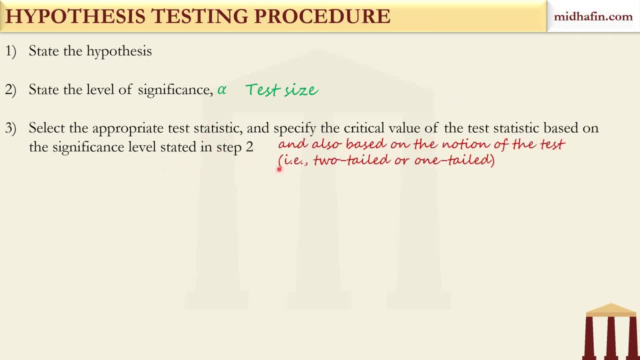 it is a type 1 error. Again, I did not say accepting hypothesis, I said rejecting a true null. it means the null is actually true. It does not mean I am accepting null, So true. Don't get confused with the terminology. 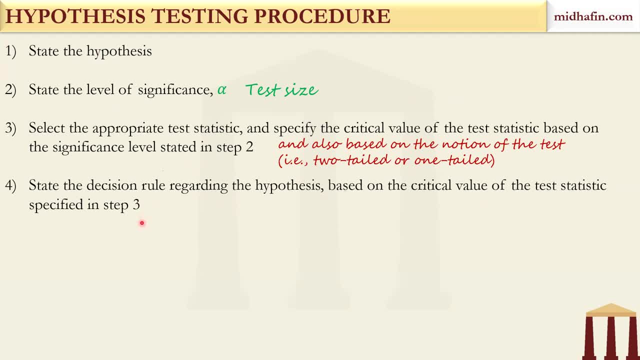 And the second one. if suppose the null is false but you are not able to reject it, then it's a type 2 error. So that is the use. Okay, then the significance level is the probability of making a type 1 error. 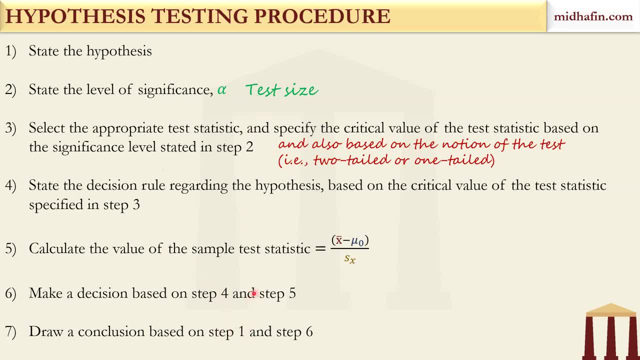 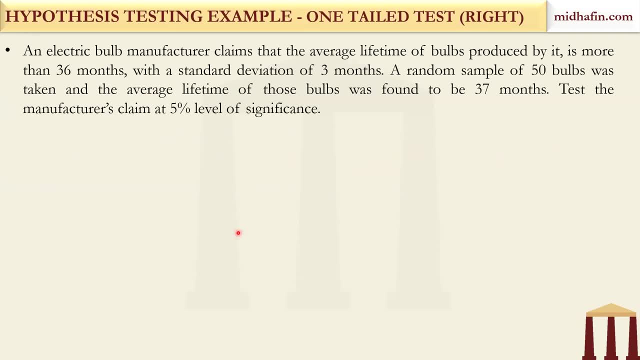 Remember that. So if the significance level is 5%, there is always a 5% chance of making an error And probability of type 1 error is significance level And power of a test is 1 minus probability of making a type 2 error. 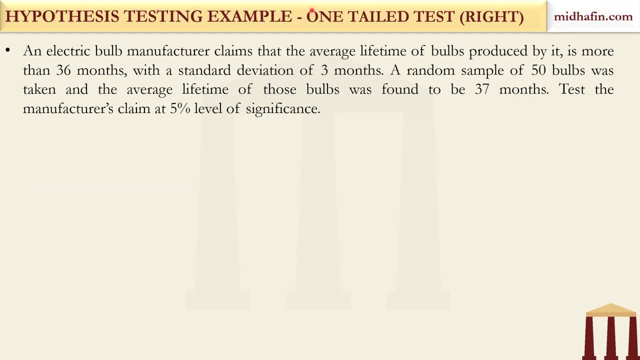 Okay, Now what is the p-value? The p-value is the minimum level of significance at which the null hypothesis can be rejected. And I'll tell you the usage of p-value also from the exam point of view. p-value is the minimum level of significance at which the null hypothesis can be rejected. 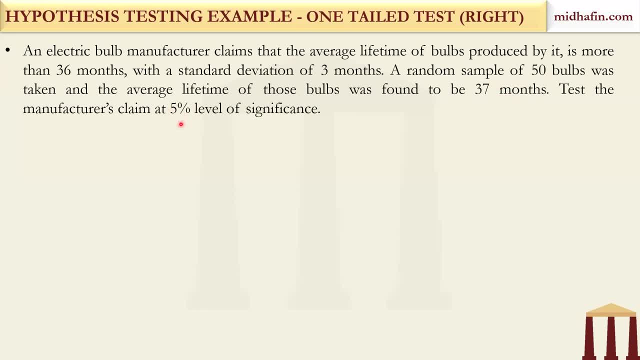 So let's discuss these two cases: one tail and two tail. So in this case you are having 5% on the right-hand side. 1.645 is your critical value. Now let's assume that this is your sample test statistic over here. 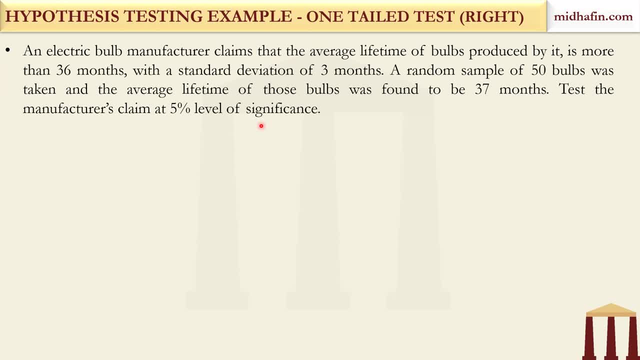 Say: this is 1.8, just hypothetically I'm assuming. Okay, So this is 1.8.. Then, for any critical value- listen to this very carefully- for any critical value which is to the left of 1.8.. 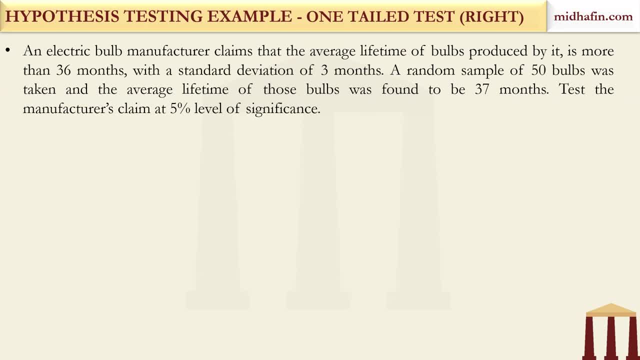 Okay, You can reject the null or no. tell me for any critical value. say this critical value is 1.645. in this case, critical value can be, say, 1.6, also 1.7, or 1 point, depending upon the confidence level. 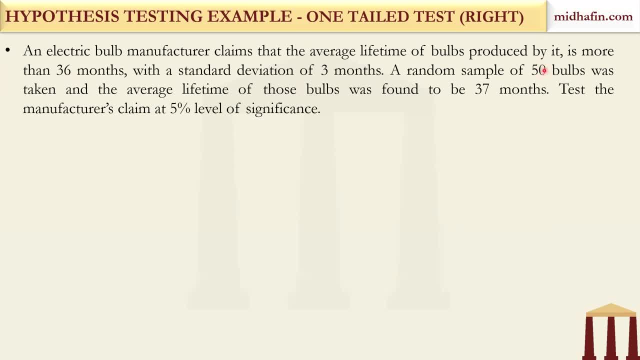 Okay, So any critical value to the left of 1.8, you can reject. So let's take a practical example. 1.645 is the One tailed critical value for which significance level: 5% significance level. 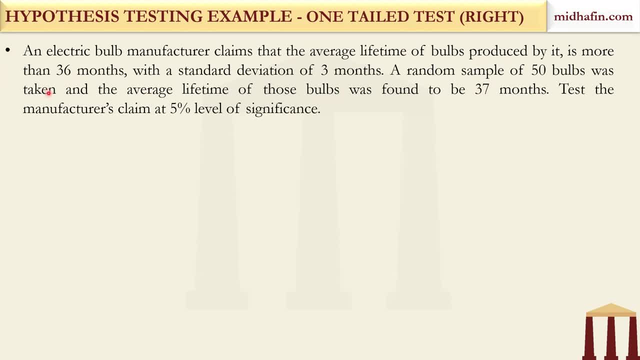 Right. Can you tell me what was the critical value, if anyone remembers, The one tailed critical value for 2.5% significance level, anyone who remembers, Even if you don't remember, you should be easily able to decipher, easily able to derive it right. 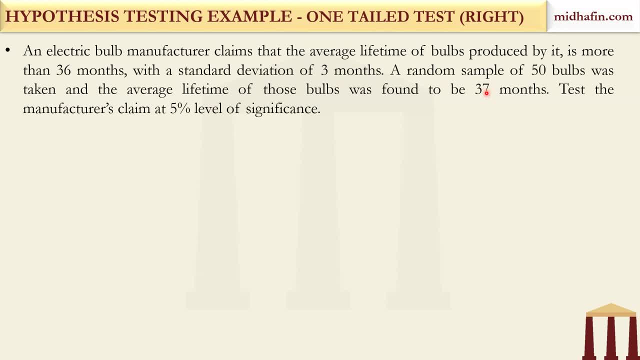 Very good, Because see for two tailed what happens For two tailed, this is 1.96, and this is minus 1.96,, correct? So 2.5% area is over here and 2.5% area is over here, correct? 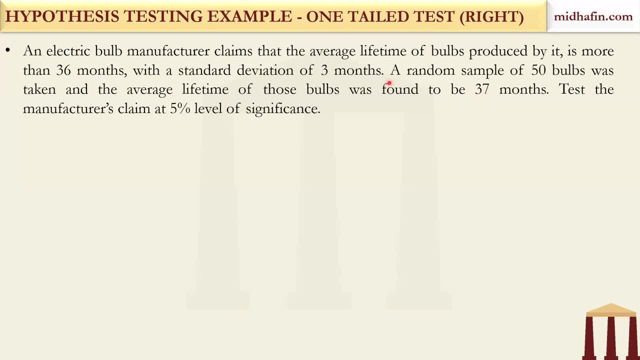 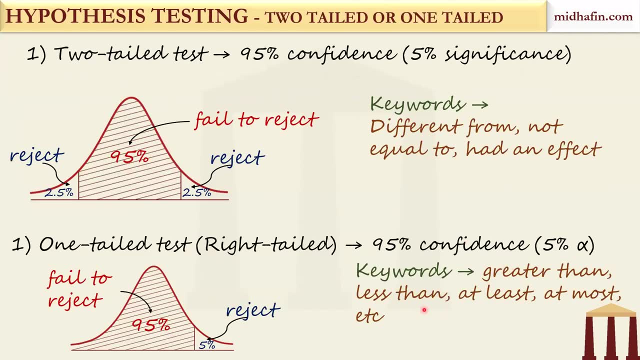 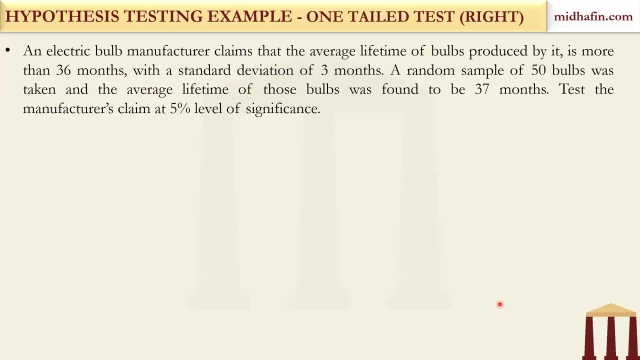 So obviously, if I have 1.96 over here, then it means to the right of 1.96, you have 2.5% of the area, correct, Okay? so everyone is okay with that, great. Now tell me one thing: can you reject the null at 5% level of significance? 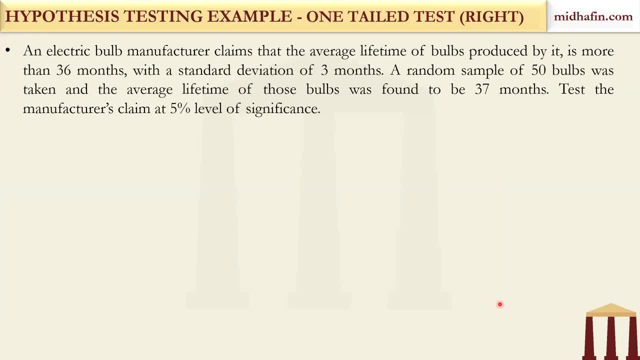 Yes or no in this case, if this is your STS, can you reject the null? can you reject the null at 5% confidence significance: sorry: 1.8,. the sample test statistic is greater than 1.645,. can you reject the null at 95% confidence? 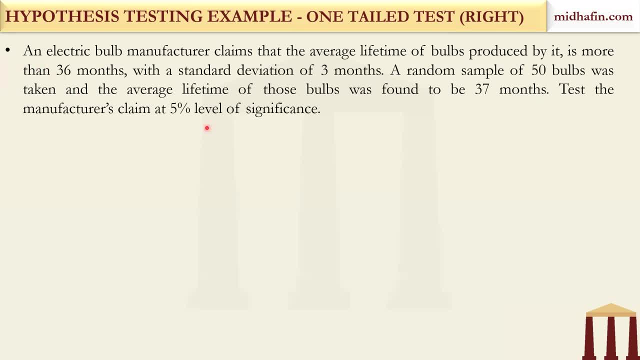 Why not? Obviously? yes, this is the reject zone right, Sushant. The right side is the reject zone. 1.8 is greater than 1.645,. correct, Sushant, clear, Got it. But can you reject the null at 2.5% significance? 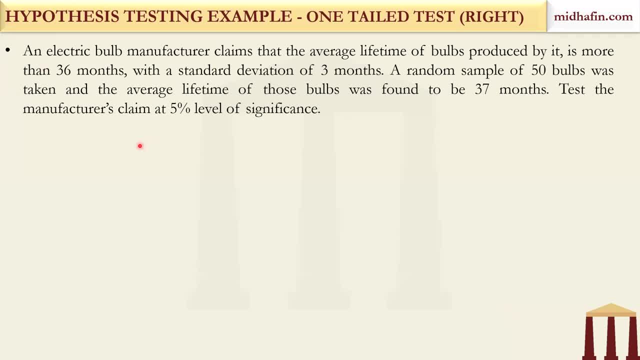 1.8 is less than 1.96.. Can you reject the null at 2.5%? significance: No, So reject at 5%, fail to reject at 2.5%, right? so it means that there is a value between 2.5 and 5, which is the minimum value at which you can reject, and that is known as the p-value. okay, 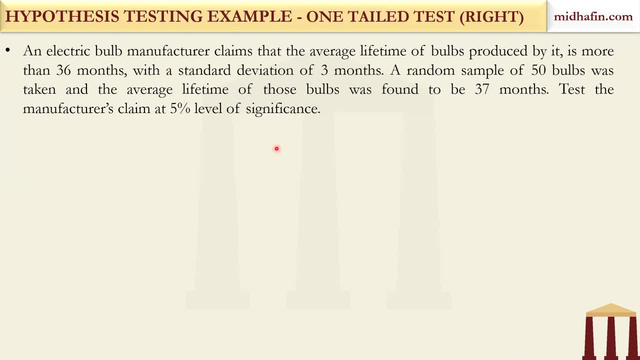 So, basically, any significance value to the left of 1.8, any critical value corresponding to a significance level to the left of 1.8, you can always reject them. okay, And it is very easy to calculate. You calculate it based on the STS only, based on this STS only, or which we can also call as p sometimes. 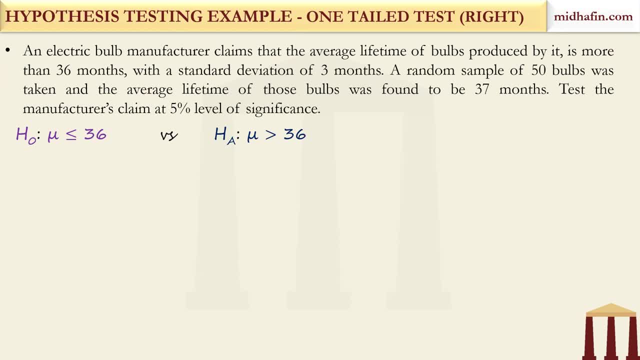 What is the formula? You simply find out the area to the right of this. This is your p-value. The area to the right of the black line is your p-value. understood, Understood, Okay, Okay, Okay, Okay Okay. 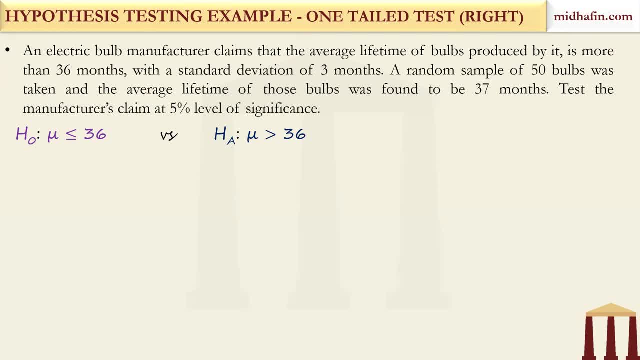 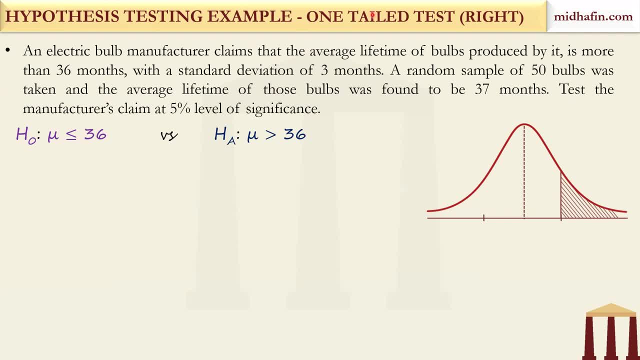 Okay, So in that case you will not be able to reject them. Now. this P-value slide only if you remember those who have attended the classes. I think we devoted around 40 to 45 minutes only to explain each and every aspect of P-value. 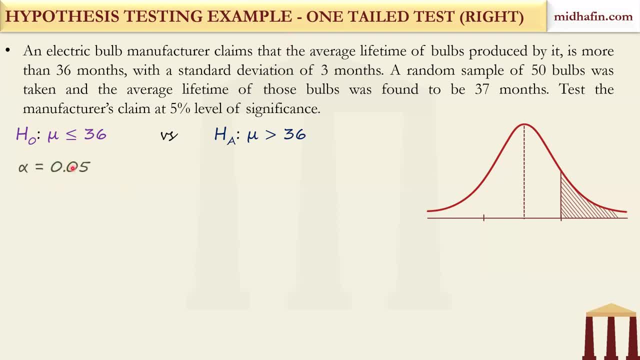 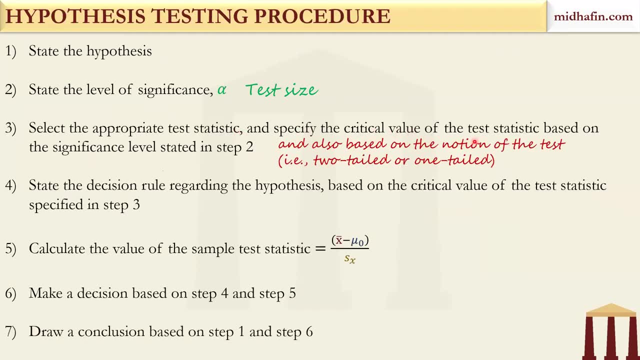 So it takes a lot of time, but I'm trying to explain the crux over here. Is it clear? Yes, you reject in black zone, absolutely. So my point is: if the rejection zone shifts towards the right, you are not able to reject, agreed or not. 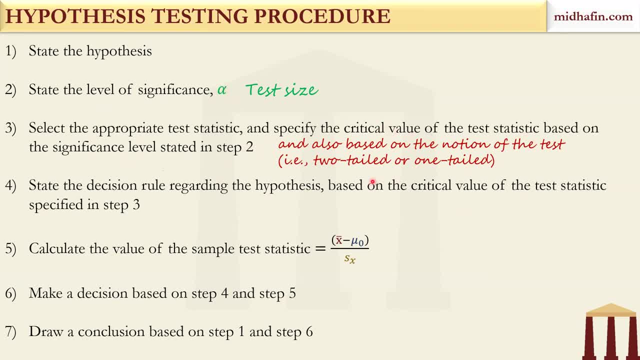 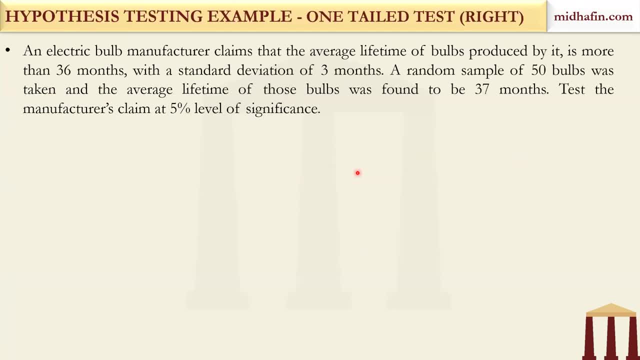 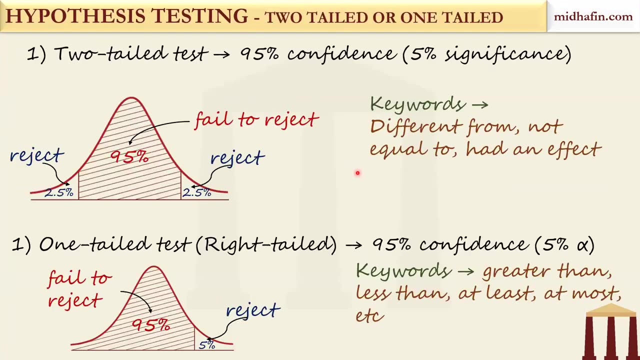 Right. If the rejection zone shifts towards the right of 1.8, you are not able to reject correct. So it means that the rejection zone has to come close to 1.8 first and it has to exactly coincide with 1.8.. 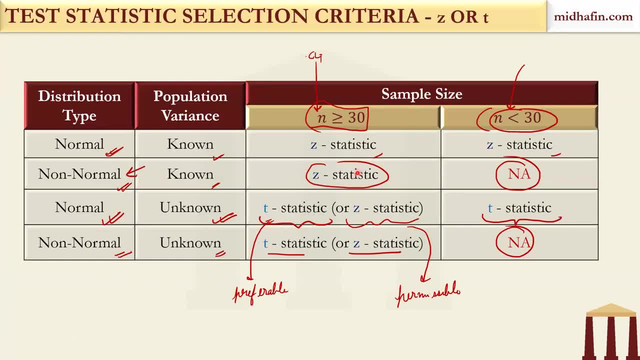 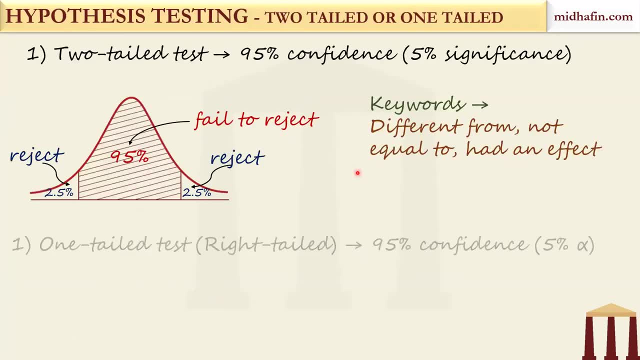 It has to this end point of the rejection zone, the left side has to coincide with 1.8. And as soon as this happens, this is the minimum level of significance at which you can reject the null hand policies Understood. 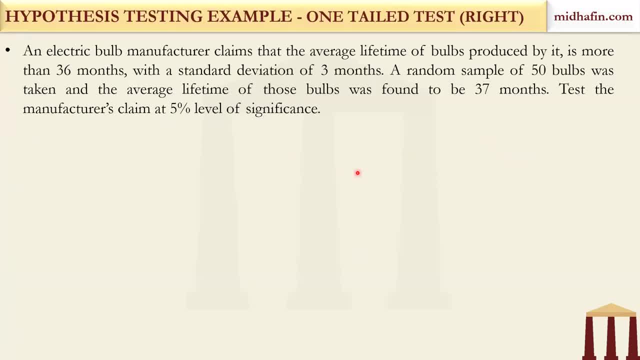 This area is the minimum level of significance at which you can reject the null hand policies. So that is why, if you see again, I'll explain this diagram once more. That is why, if you see this example which we had, this was 1.8 and this was 1.96.. 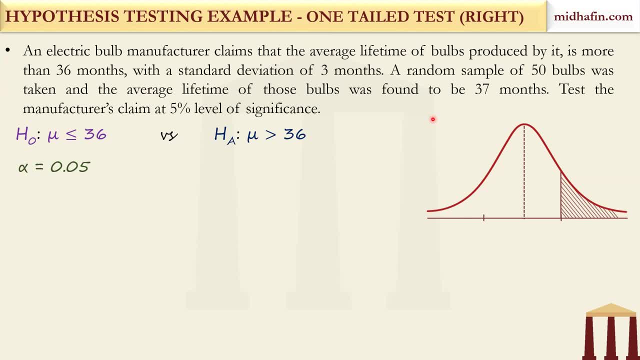 So corresponding to 1.96,. guys, this is the rejection zone, correct? So that is why you are not able to reject at 2.5%, agreed or not, The rejection zone is to the right of 1.8.. 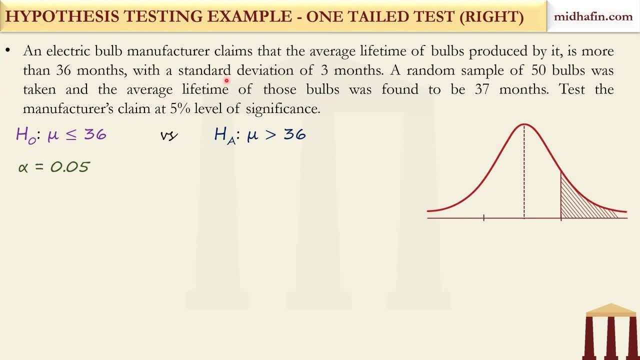 This is clear now To everyone. To everyone, not only to one or two people. to everyone. Is it clear In this case, since the rejection zone is to the right of 1.8, you are not able to reject because. 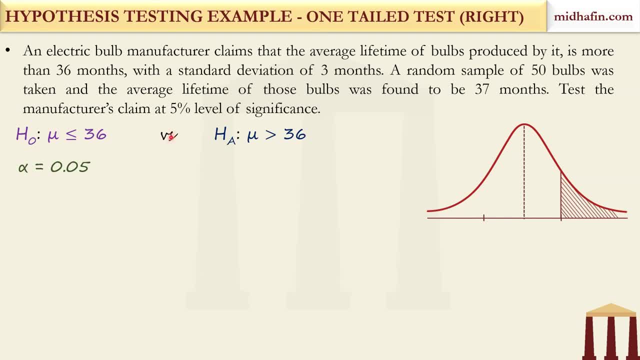 this is the diagram, guys. Let's go back, Let's revisit. yeah, See, reject zone. is this to the right hand side And this is the fail to reject zone? okay, So if the reject zone is to the right side of 1.8. 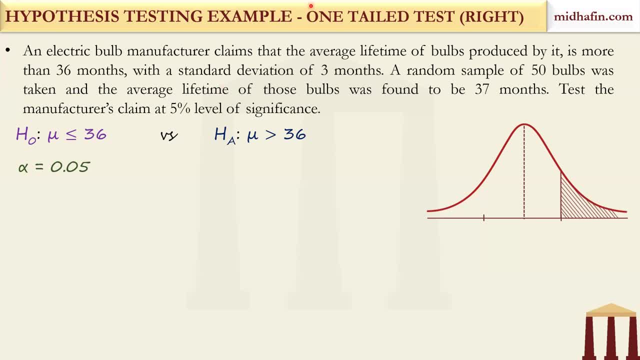 in this example. will you be able to reject? That is my question. Will you be able to reject at 2.5%? I am emphasizing this point again and again Because it is important. Will you be able to reject at 2.5%? 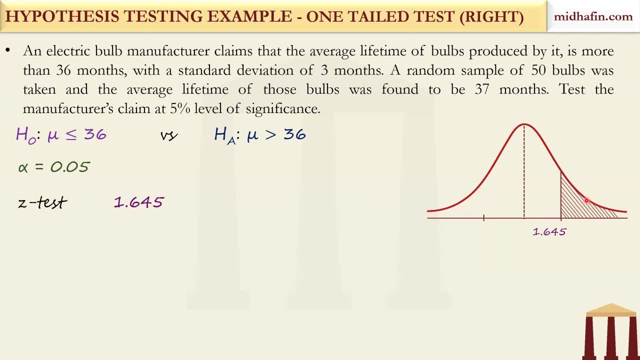 No, No, But are you able to reject at 5%? Yes, Because 1.8 is in the rejection zone as far as 5% is concerned, understood. So p value is the minimum level of significance at which the null hypothesis can be rejected. 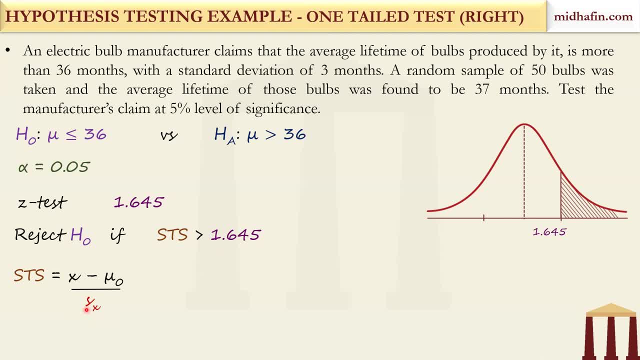 and it is nothing but this area. Okay, so this is the formula: P-values. you just look at the Z-table, This is the formula And for two-tailed, of course, you have to consider both the regions. Now, last part, testing the equality of two means. 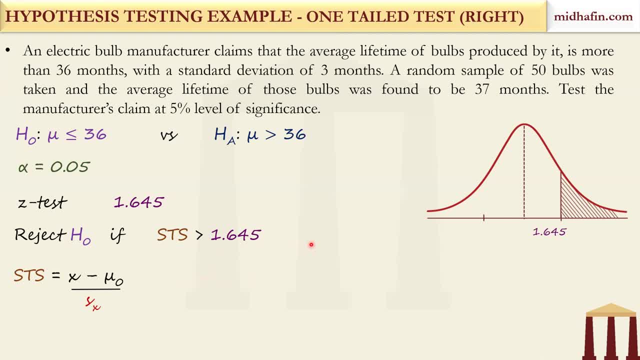 I will not explain the theory, I will not explain how the hypothesis is transformed. I will show you how to solve the question in the exam directly. So see which test statistic has to be used, If suppose this kind of question is asked. 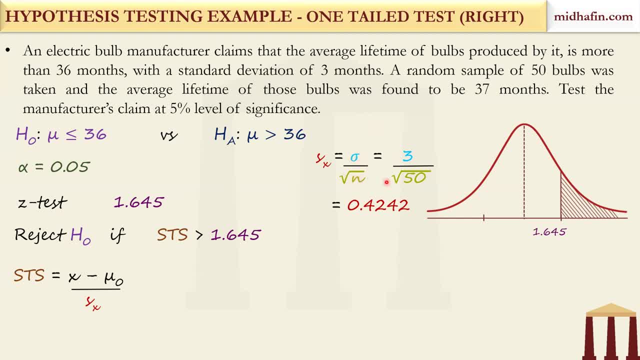 you just remember that you have to use this test statistic, this one. What happened? I think there is a problem with respect to animation. again, Let me just see. Anyways, there is a problem with respect to animation. You see this part first. 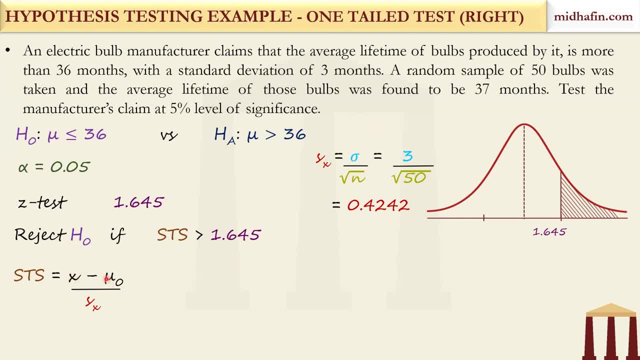 So this is the test statistic that you have to remember: mu x minus mu y, divided by sigma x- square plus sigma y square minus 2 sigma x- y divided by n. Just a quick Question: why cap is there in all these values? 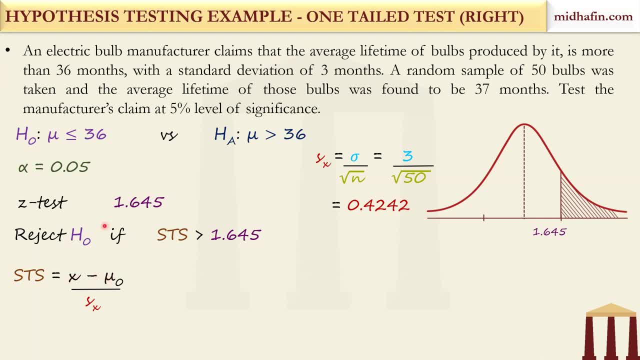 Why a cap? you can see. Can you tell me Why there is a cap first? Yes, these are estimators from the sample. Very good, These are all estimators. These are all estimators, Okay, So if this kind of question is asked, 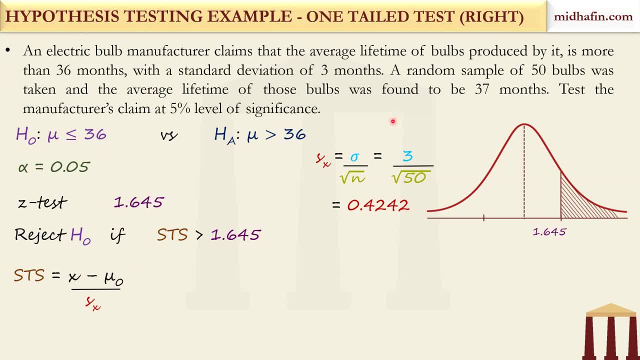 consider two distributions that measure the average rainfall in city X and city Y. Means variances, sample size correlation. this will be given to you in the exam. Using this formula, you calculate the test statistic and then you compare it against the critical value and you directly say: 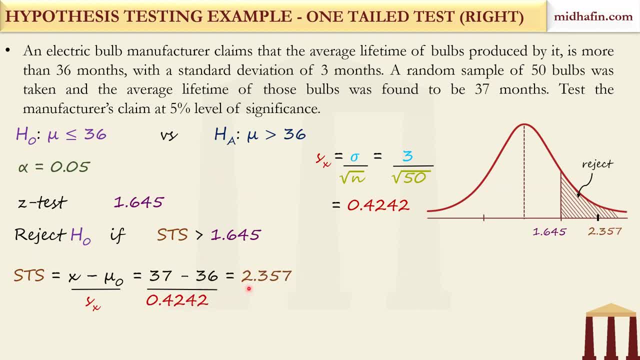 that the null hypothesis can be rejected. So when null can be rejected, it means the population means are not equal, Because if you see the hypothesis, the hypothesis mu x equal to mu y can also be stated as mu x minus mu y is equal to zero. 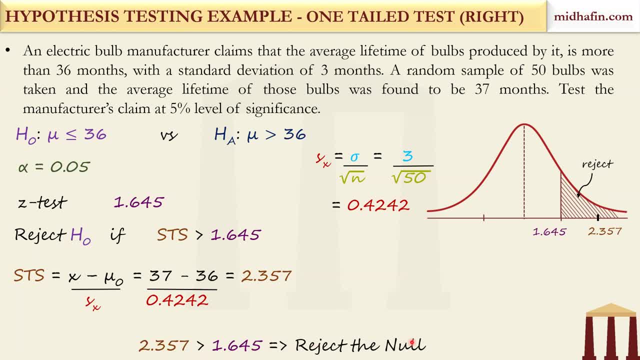 And this is your null, And the alternative is that mu x is not equal to mu y. Okay, so this is how you will perform this question in the exam. No, this will also be z-test. This will also be z-test. 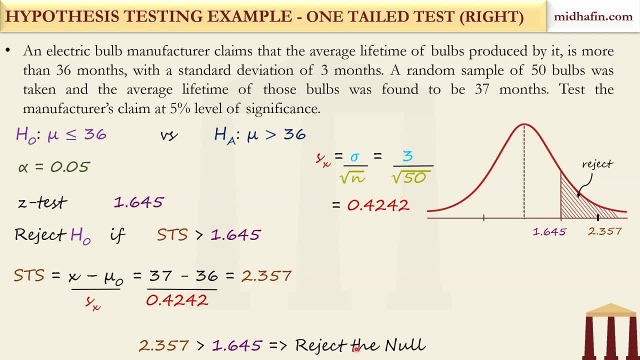 Unless and until they mention because- see, I'll tell you why- The sample size and everything, because the data that has been collected, it is the average rainfall. This has been collected probably based on a data of 200 days, So 200 is a large enough sample to use a z-test. 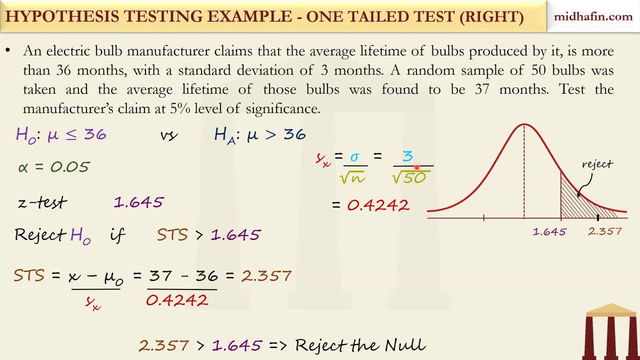 Okay. so just look at the null and alternative hypothesis and take a correct decision. Remember that if you are able to reject the null, the population means they are not equal. It means the average rainfall in city X and Y are not equal in this case. 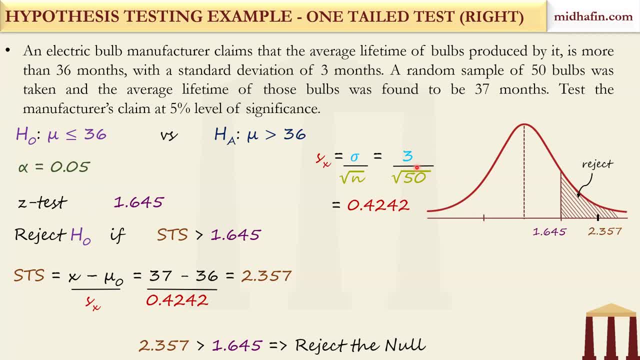 That is how the construction of this test is done. Very smartly, equality test has been transformed into an equal to zero test. Equality between two means has been transformed because- see again, I'm repeating mu x minus mu y You are writing. actually the main test was mu x equal to mu y. 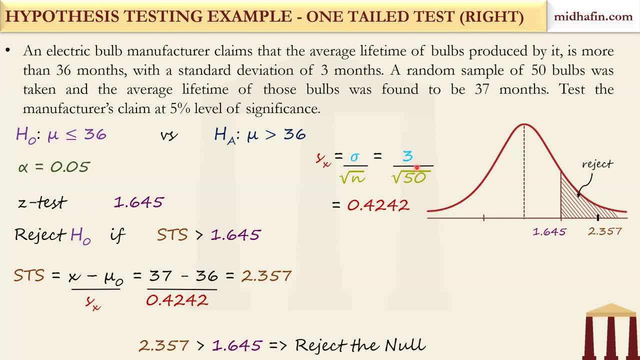 So this was the null hypothesis. So either you test this or can you write the same thing as mu x minus mu y equal to zero, Yes or no? Are these two statements identical or not? Are these two statements identical or not? Yes, because if mu x equal to mu y, then mu x minus mu y equal to zero. 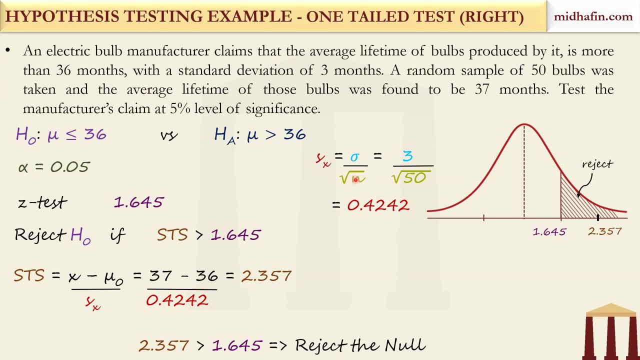 Now, if you have rejected the null, it means you have rejected this. It means you have rejected this. Okay, so rainfall is not equal in both. Got it. So that is the whole idea. Now, one more thing which I want to add that generally you will find: 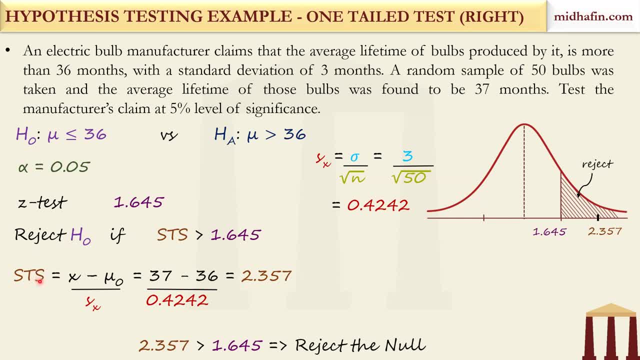 that wherever we have written the null hypothesis, we have always included this equal to sign with it: Equal to sign, whether it is less than equal to or equal to or anything. So null sign. null hypothesis always contains equal to sign. Alternative hypothesis does not contain equal to sign. 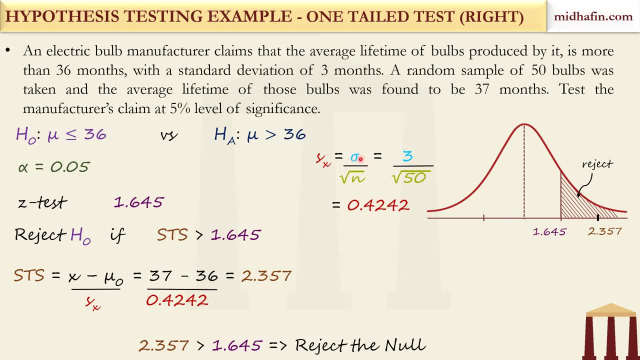 Either it will be greater than, or it will be less than, or it will be not equal to. So this is one of the keys We can use to frame the null and alternative hypothesis. Okay, Okay, so we'll take a break for 20 minutes. 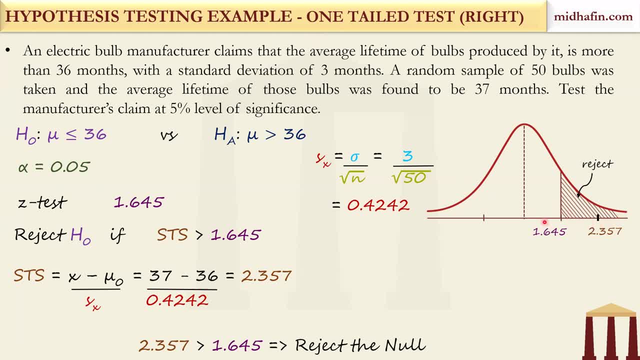 We can be back at 4.30.. Is that okay, Or a shorter break, As you say? I'm completely okay with both. 4.30 is okay. Shorter 15 minutes, fine, 4.25. Okay. 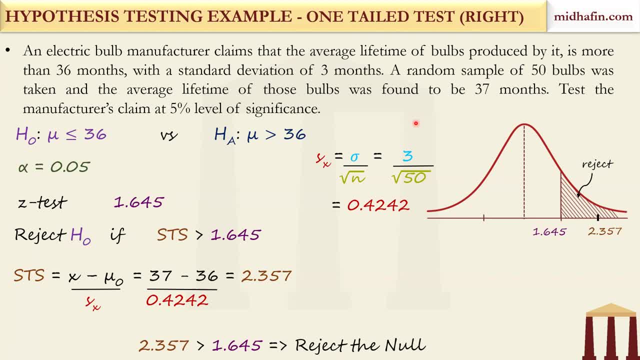 At least revisit the concepts. Revisit the concepts. Okay, Caroline is asking for 20.. Caroline, actually see, the content is very, very long And I agree that you know, even if you are able to say five minutes, it will be better. 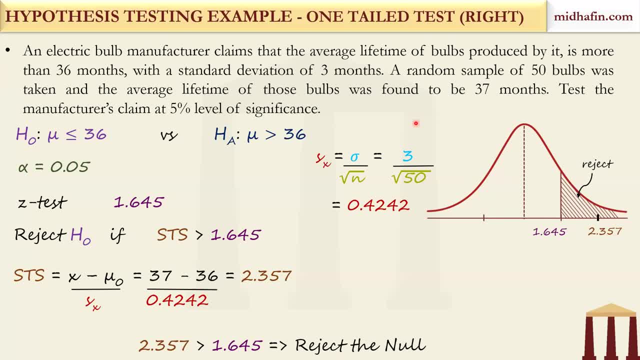 It's already 4.11.. So at least do one thing. We are going to do very important chapters, regression related chapters. So before you resume, at least have a quick brush up of the regression concepts and the formulas quickly So you might. 4.25, 15 minutes. 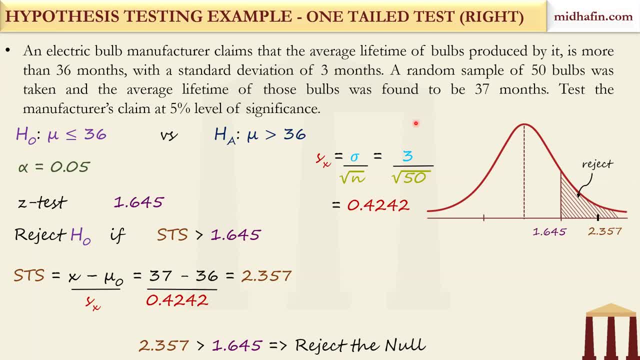 Is that okay, Caroline? Does it work for you? Okay, fine, DMs have also been given, So, anyway, let's start at 4.30.. No problem, So 20 minutes. Fine, Let's start at 4.30.. 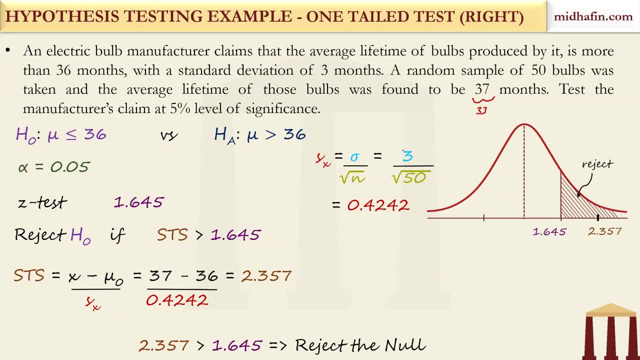 Okay, Thank you, Thank you. So we'll start with now QTA regression. QTA 7, sorry- linear regression. Okay, now linear regression. it assumes the linear relationship between any explanatory variable and a dependent variable, Y. So this is the relationship where beta is the slope or regression coefficient. 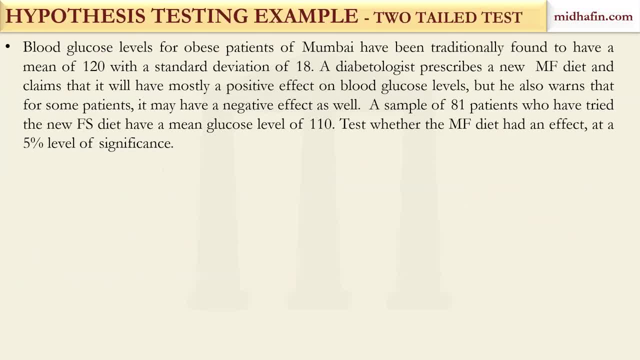 It measures the sensitivity of Y to changes in X. So how we interpret the slope coefficient in a linear regression? Basically it is the change in Y for one unit of change in X. So that is why sensitivity of Y to change in X. 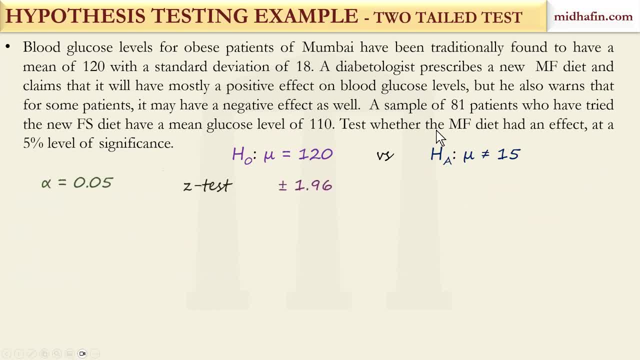 So remember that, And we modify the same interpretation in case of multiple regressors. Okay, And you have alpha, which is the intercept, which is constant, And again, the interpretation of alpha is that The value of Y and the value of the dependent variable when X is zero. 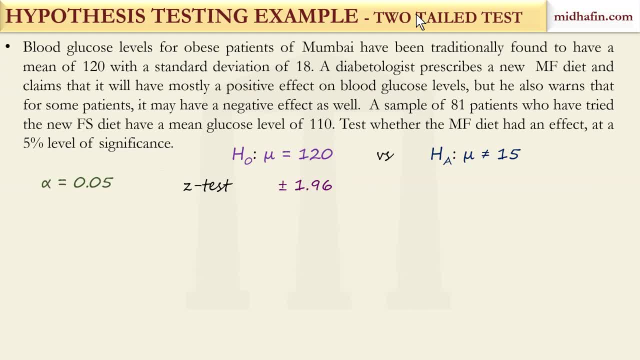 So obviously the expected value of error term is assumed to be zero. So both these terms are zero. If X is also zero, then Y will become alpha, right? So alpha is interpreted as the value of the dependent variable when the independent variable is zero. 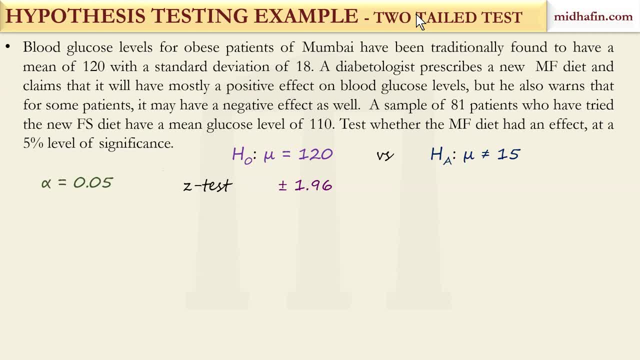 Okay. So just remember this: The interpretation of slope: slope is nothing but the change in Y For one unit, change in X and alpha is nothing but the value of Y when X is zero. Remember this, Okay. So just like straight lines, which we did in class 11.. 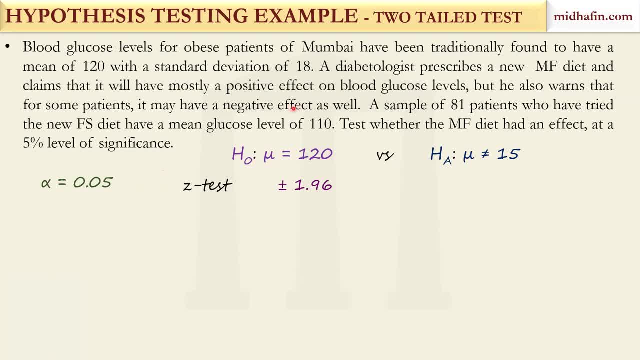 Now E or epsilon is the shock, the innovation or the error term. It represents a component in Y that cannot be explained by X, And the expected value of the error term is always assumed to be zero. So let's take some example. 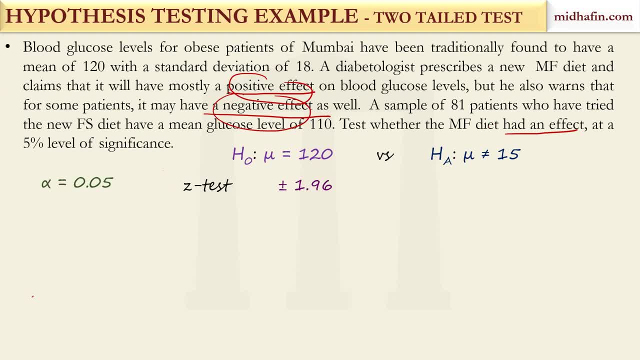 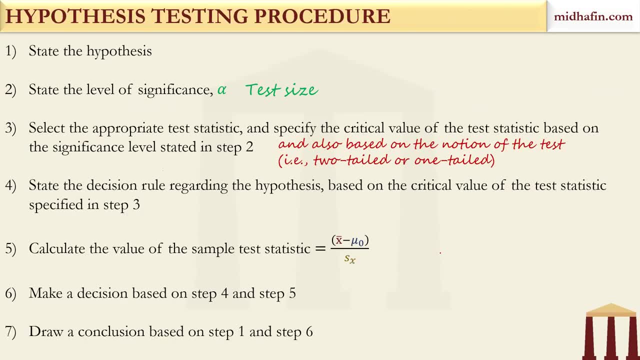 Let's say we take an example of phone sales versus discount. where phone sales is my dependent variable, discount is a dependent variable. We can also have an example of H1 returns versus lock-in period, So Y versus X, And we can have an example of student. 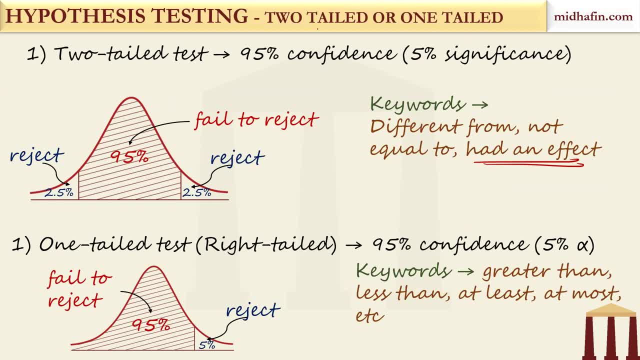 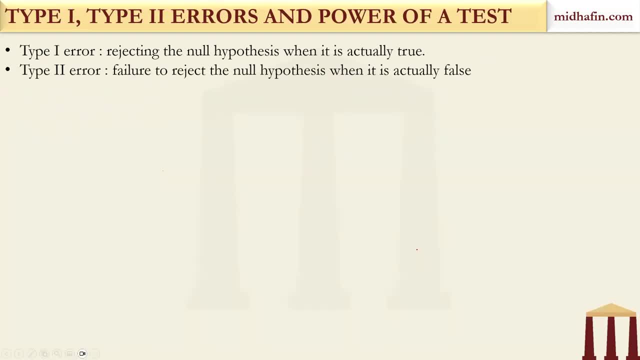 average marks versus student teacher ratio. So one and two. what do you think A positive relationship or a negative relationship between Y and X? In case one and two, a positive relationship or a negative relationship? As discount percentage increases in general, what would you expect for sales? 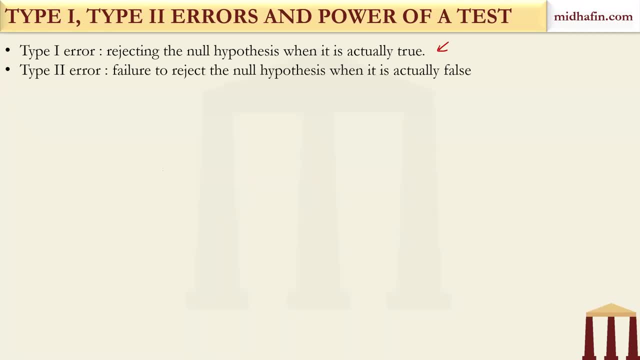 Increase right. Similarly, as lock-in period increases, hedge funds returns tend to increase. The first two relationships are having positive relationships. First two are having positive relationships. first two pairs And the last one. the third one- is actually a case of negative absolutely. 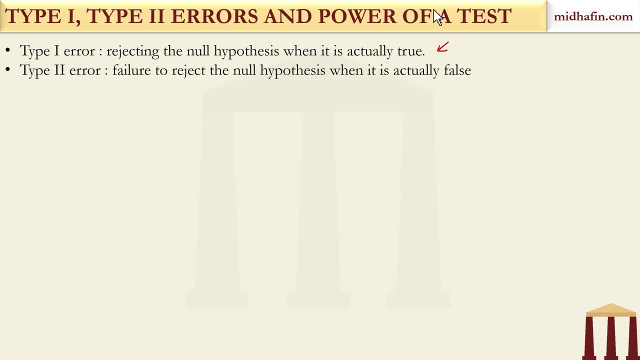 Because if the student teacher ratio is high, if there are more number of students per teacher, if there are 60 students per teacher, and compare it to the situation where there are only 10 students per teacher. So if everything else say is constant, then the marks will, of course. 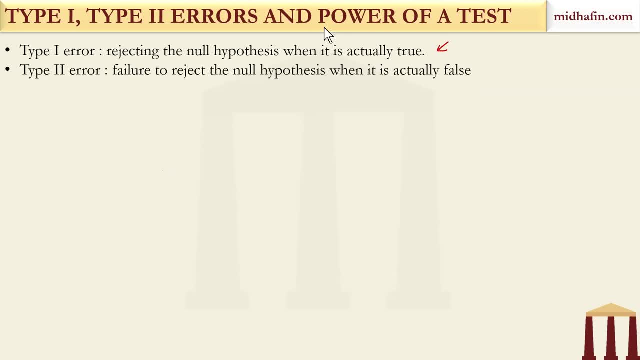 improve for a lower student teacher ratio. It's a negative relationship. Now these parameters: what are the naming conventions? Y is known as the explained variable, or the left hand side variable, or the dependent variable, or sometimes the regressant, And X is explanatory variable, right hand side variable, independent variable or regressor. 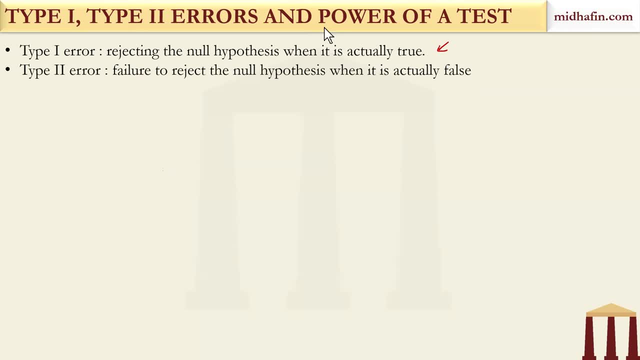 Epsilon or E is the shock or innovation or noise or error or disturbance. OK, Then you have dummy variables. Dummy variables are a special class of variables which we use in linear regression. They are binary and they only take values of zero or one. 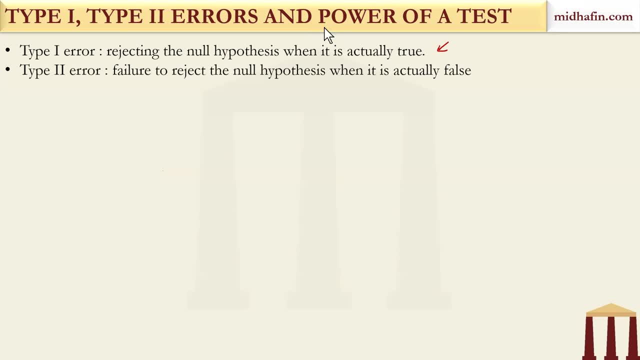 So dummies are used to encode qualitative information, For example a firm's sector or a bond's country of origin. So let's say you might have a case where you are denoting IT sector with a dummy variable of one and anything other than IT. 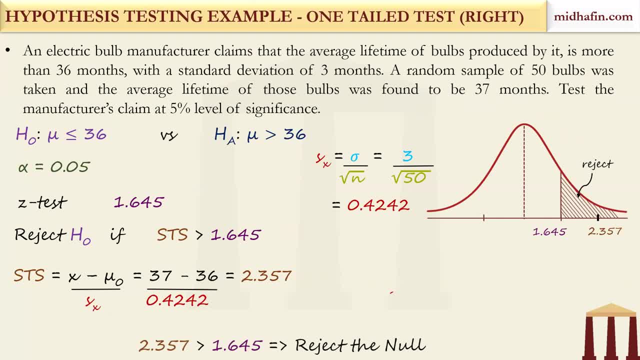 sector is having a dummy variable value of zero. Now let's come to OLS. consider a basic regression model which includes a single explanatory variable, the basic example that we have been taking. Now these alpha and beta can be estimated using OLS estimators. 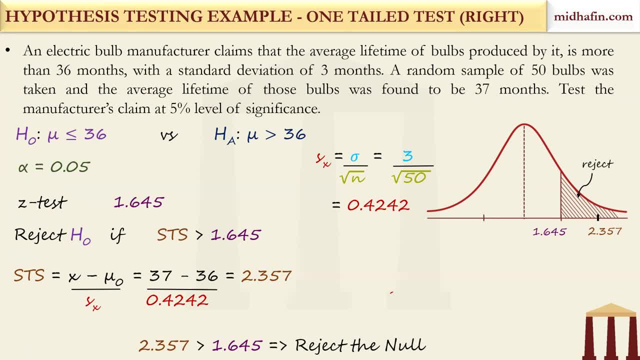 OK, so this is the beta estimator. OK, this, by mistake, is double equal to OK, and this is equal to covariance between X and Y divided by the variance of the independent variable. Remember that in the denominator I have seen candidates making silly mistakes. 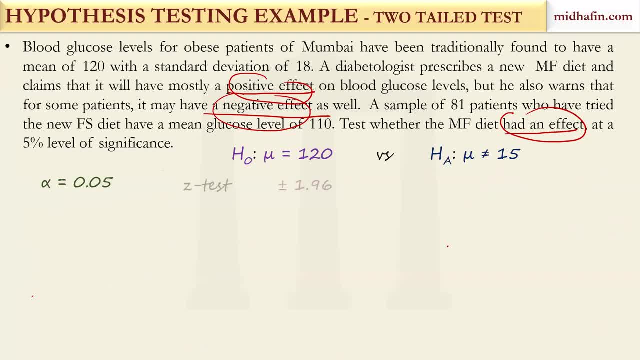 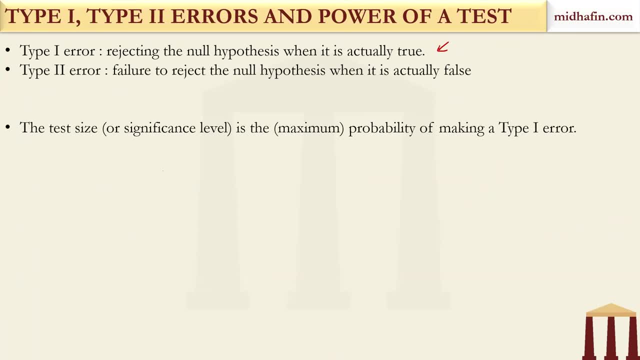 in the exam, where in the denominator they'll write variance of Y, Don't make that mistake. OK. And of course, if you want to frame the same relationship in the form of correlation, this is the relationship over here- OK. this also can be derived by minimizing. 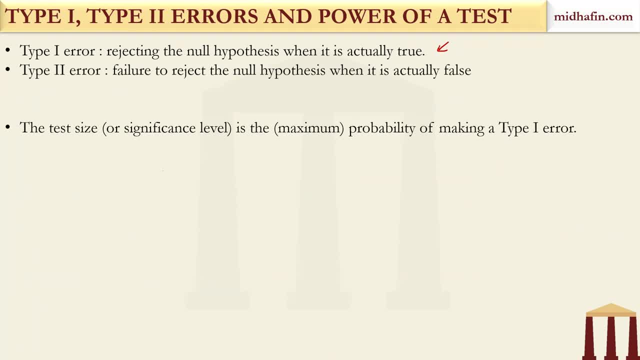 problem using maxima minima in differentiation. OK, you take the function and you minimize it. set the dy, dy, dx equal to zero And basically we are trying to minimize the sum of squared errors. OK, so we get beta hat equal to this. 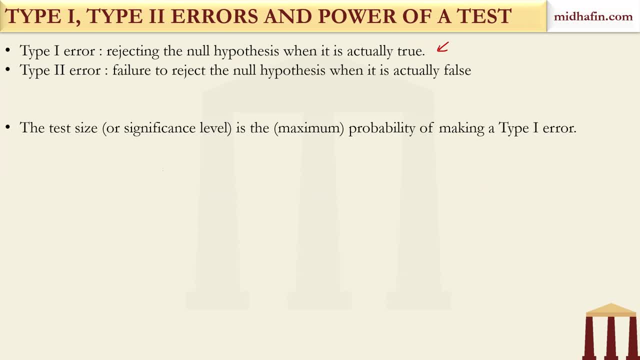 And alpha is estimated using a property of the OLS regression line, that it passes through the mean X bar, Y bar of the values of X and Y. OK, so these are the properties. Again, derivations we are not going to do. 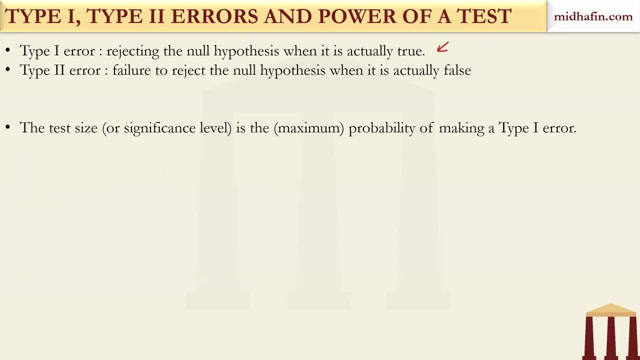 Only formulas are important from the point of view of the exam Derivations we have done in the class. Now let's take an example. Let's say this is an example. This is how you'll be asked in the exam this kind of question. 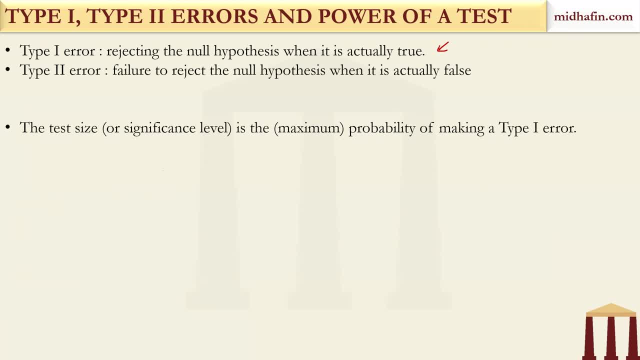 So the covariance matrix will be given to you. X bar is given, Y bar is given. Covariance matrix is given to you. The first job is to find out beta For beta hat. So this was the formula: beta hat equal to this, which gives you 1.5188.. 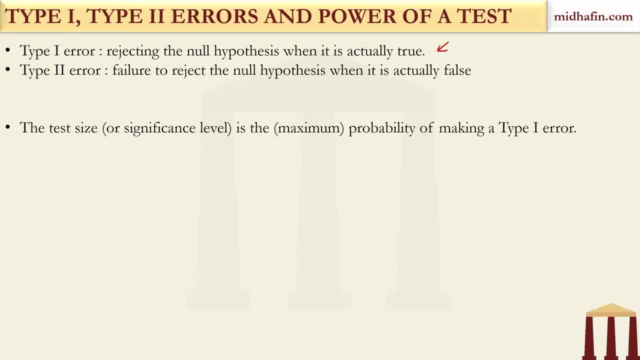 So you can see that these parameters are directly taken from the covariance matrix. 512.3 is the covariance and 337.3 is the variance of X. OK, so what is the interpretation? The interpretation of beta hat: is that the return because we are talking about? 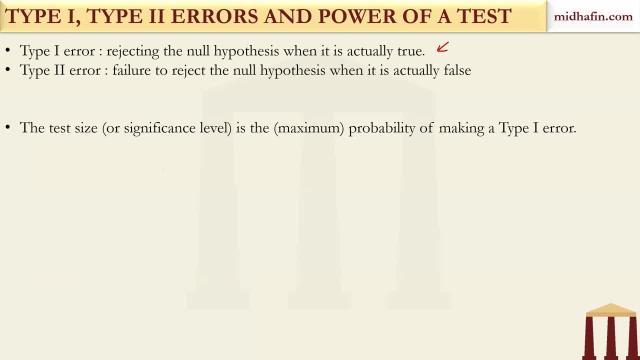 the mining sector, and this has been assumed over a period of 20 years, And these are annual returns. OK, remember that the period is 20 because this will be important later on, So N will be equal to 20.. OK, 20 years later, 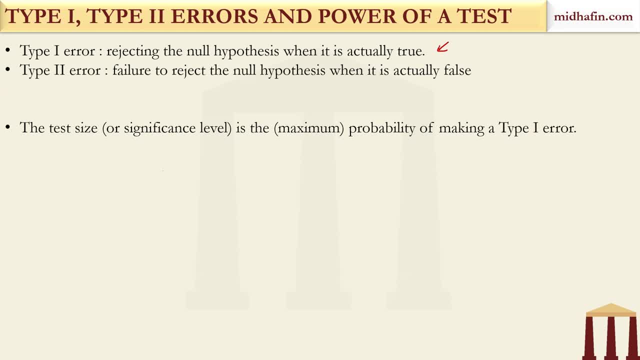 So beta hat equal to 1.5188.. So the interpretation is that the return on the mining sector portfolio, which is my dependent variable, it increases by an average of 1.5188 percent. When the market return on the independent variable, it increases by 1%. 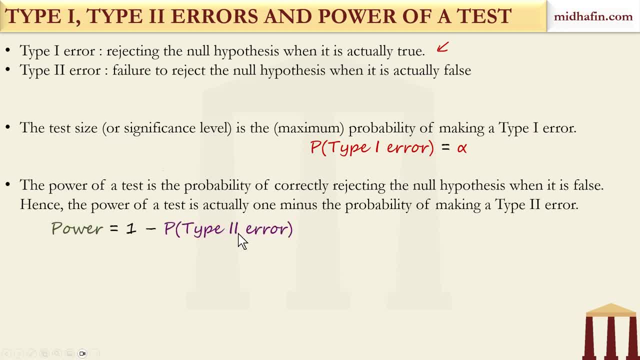 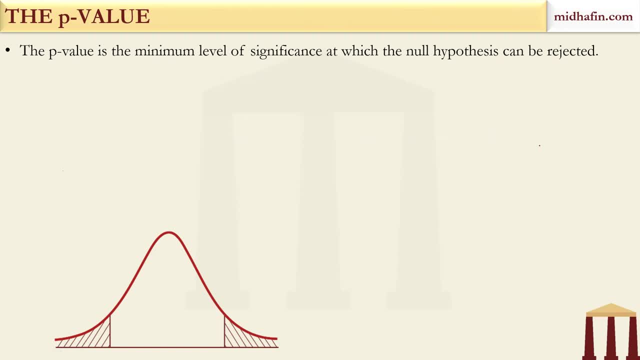 So for every 1% increase in return in the market, the mining sector portfolio increases by 1.5188 percent. OK, so for alpha hat also, we use the formula and we get 3.5989%. What is the interpretation? What did I say for alpha? 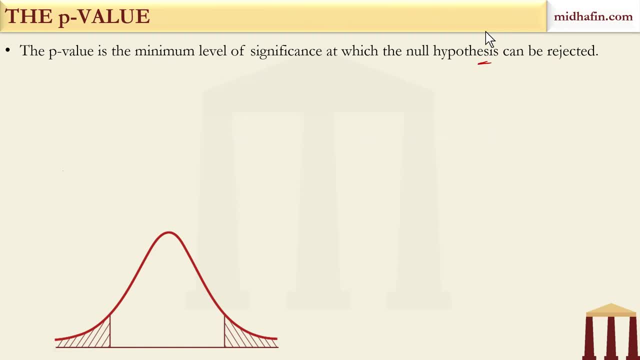 For alpha, the interpretation should be the value when X is zero, right? So this indicates that the portfolio returns are having an average return value of 3.5989%. OK, if there is any calculation mistake, please let us know now or later. 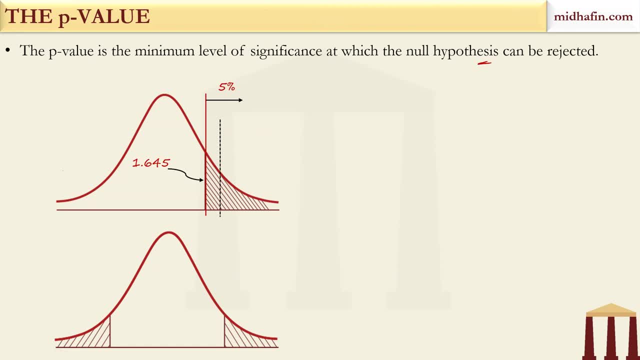 Also, if you have any typo, As I said earlier, it returns an average. the portfolio mining sector portfolio- it returns an average of 3.5989% when the market return is zero. That is even based on interpretation. the questions can be asked, OK. 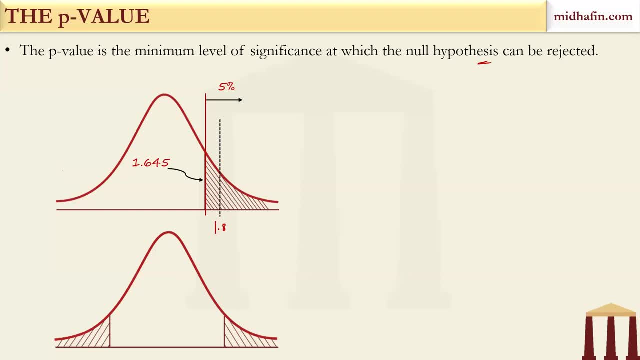 Next, there are three important definitions. Explain sum of squares. So it is the sum of squared deviations of the predicted values from the average value. See the difference Predicted minus average. Sum of squared residuals. Sum of squared residuals. So sum of squared residual is very, very important. 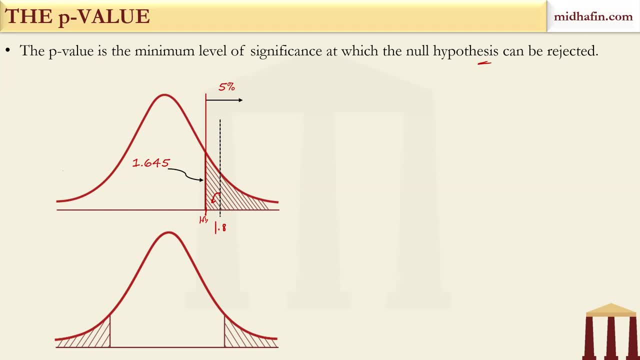 Or you can say residual sum of squares, or RSS, RSS, SSR, whatever you want to call it. So this is the sum of squared deviations of the act, actual values, from the predicted values. So these are basically the error terms, the sum of the error terms. 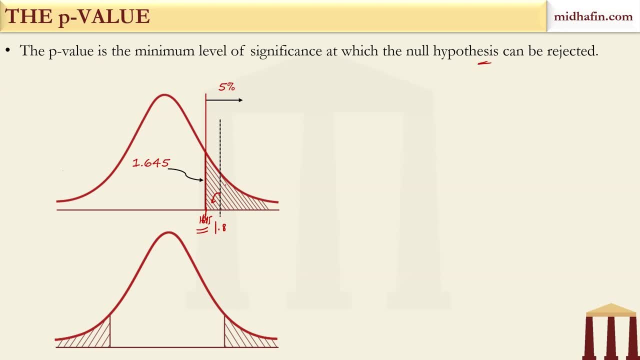 OK, the SSR or RSS And ordinary least square tries to minimize these error terms. OK. Next one thing I just want to highlight over here with respect to ordinary least square. before we proceed, Remember ordinary least square. We are talking about the error term, so we are not minimizing the perpendicular distance. 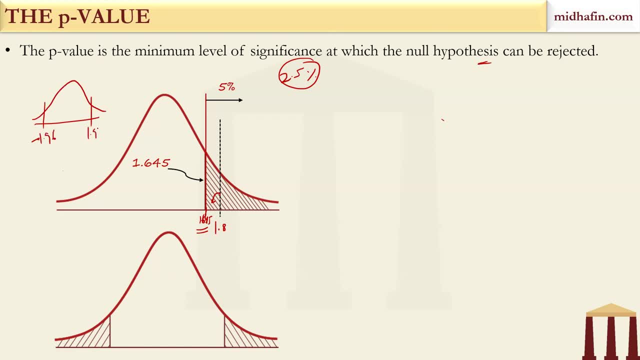 We are minimizing the vertical distance. What I mean to say is, Suppose these are your points, OK, OK, And you have to find out the best fit line. So there are many ways. Of course it is not only. OLS method is not there. 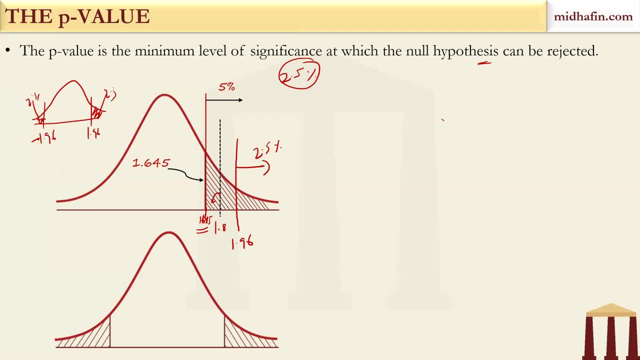 There are many multiple ways. OLS specifically minimizes the sum of the squared distances of the actual values from the predicted values, So one which you are predicting on the line, And these are the differences between the actual and the predicted. You can see that these are vertical distances. 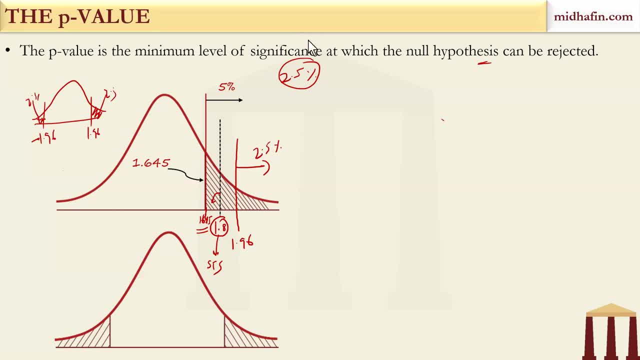 These are not perpendicular distance. OK, so there is a confusion sometimes. In fact, this concept itself is not clear, The visualization is not clear. what is happening to many candidates? So first make the visualization clear that what are we minimizing? We are minimizing the sum of these squared errors. 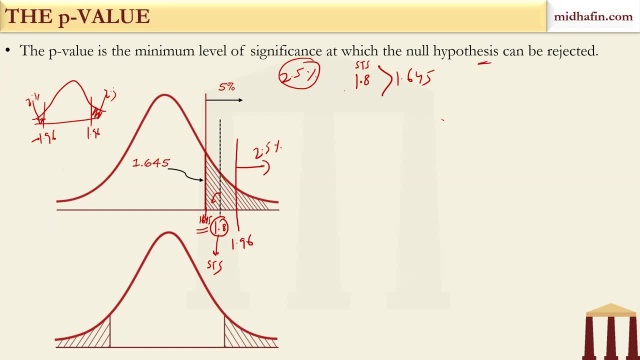 These are all the errors: Actual minus predicted: OK. and these are vertical distances. Remember, vertical distances, OK, not perpendicular distances. And once you minimize it, you get the value of beta. And once you have the value of beta, you get the value of alpha. 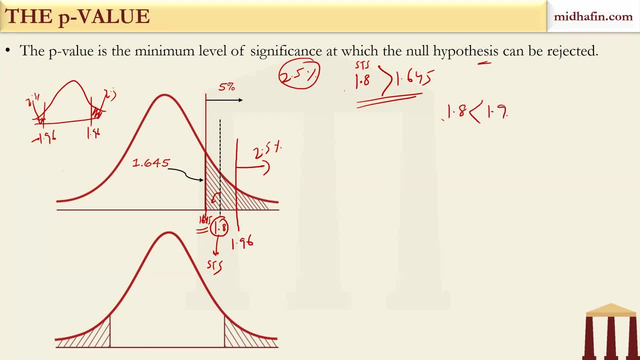 So this is the second parameter and this is the third parameter: total sum of squares. Total sum of square is basically the actual minus average, So this is the average value. What is the difference between the actual value and the average value? Now, it can be very easily shown, although we do not show it, that PSS is equal to ESS plus RSS. 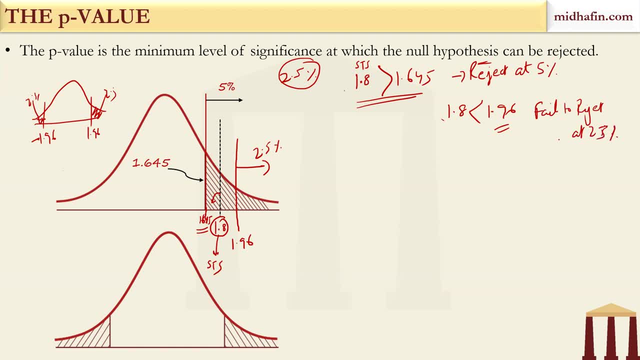 So this is a very important reason. OK, In the class we have used Excel sheets and some examples, also manual calculations, to illustrate these ideas and the calculation of related terms like R-squared numbers. So let's come to R-squared. 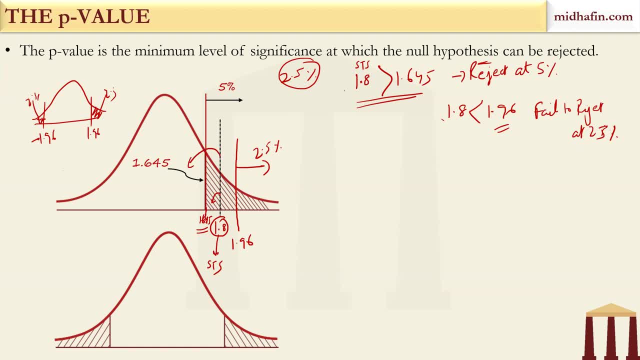 R-squared is the proportion of the variance in the dependent variable. that is explained by the variation in the independent variable. Again, this is the part which is very technical. I believe This is also a part where I mean, if you ask someone what is R-squared? 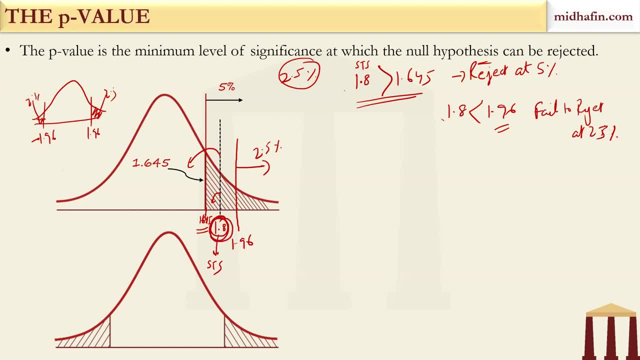 So R-squared they'll say percentage of dependent variable explained by the independent variable. Wrong, That's not correct. Percentage of the variation in the dependent variable explained by the variation in the independent, That is. this distinction is very important, OK. 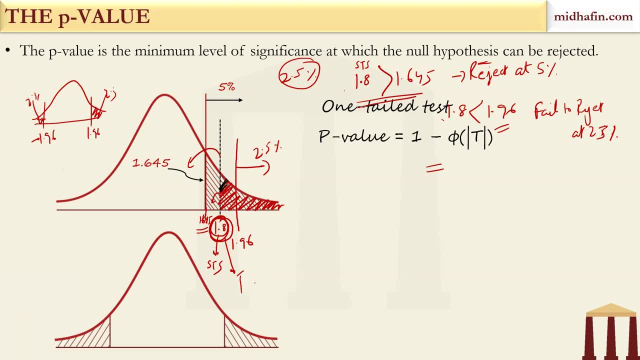 So R-squared is not. I mean, in layman terms, you can definitely say it, but this is technically incorrect. The technical definition, the technical definition of R-squared is: it is the proportion of the variation in the dependent variable that is explained by the variation in the independent variable. 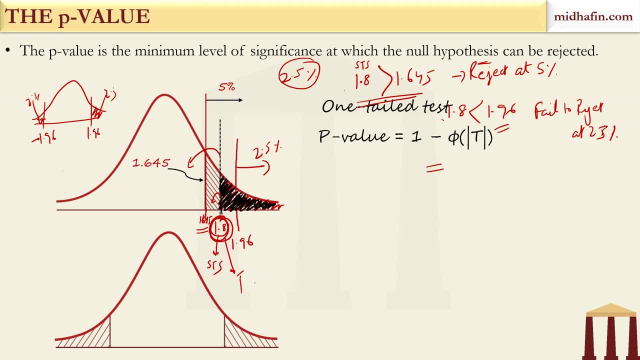 Now remember a very important point: Since we are dealing with linear regression with single regressor, in that case correlation is the square root of R-squared. This is only applicable for linear regression with a single regressor, because for multiple regressors there is a different story altogether. 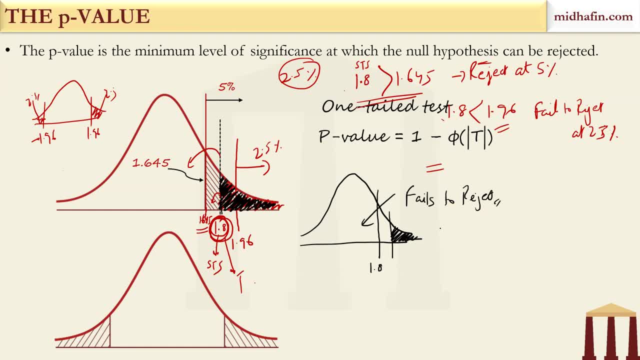 It is a different relationship. It's also a straightforward relationship, but not this one. OK, Now what are the assumptions? The expected values of error terms are zero. Data are realizations from independent and identically distributed random variable. Variance of X is greater than zero. 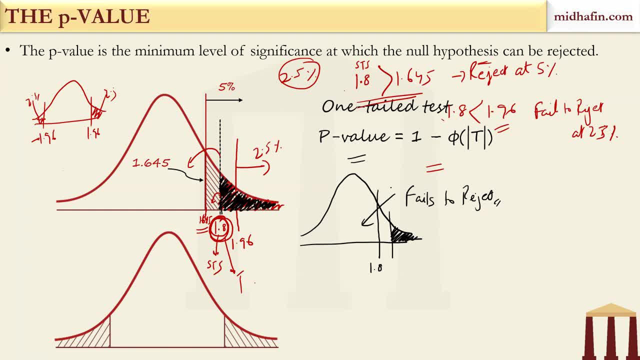 There is no correlation between error terms, So error terms for each data point, I mean if you take each data pair, if you calculate the error term, then the error term should be independent of each other. The variance of the error term should be constant. 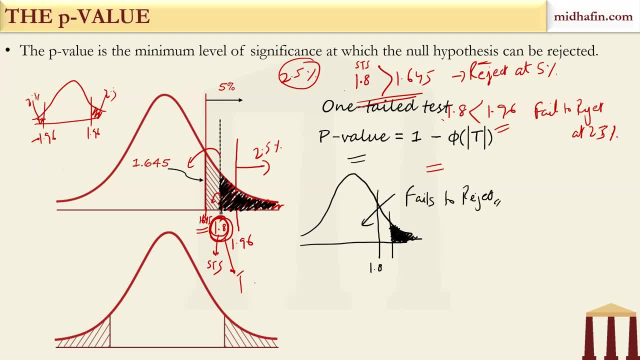 And this is a very this fifth assumption is a very important assumption. We'll see later on why. And the data contains no algorithms. As I said that this fifth assumption is very, very important, because this is the figure over here You can see that in this case, the variance of the error terms 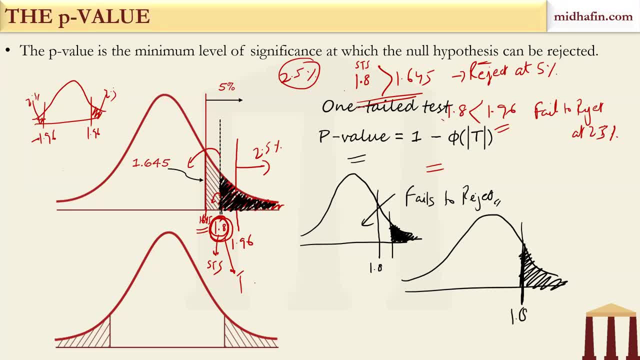 you see, the spread is not changing. as you are moving from left to right, The spread is almost. I mean to illustrate this, even dummy distributions have been drawn. These are dummy distributions, just to illustrate OK that. OK, this is the. 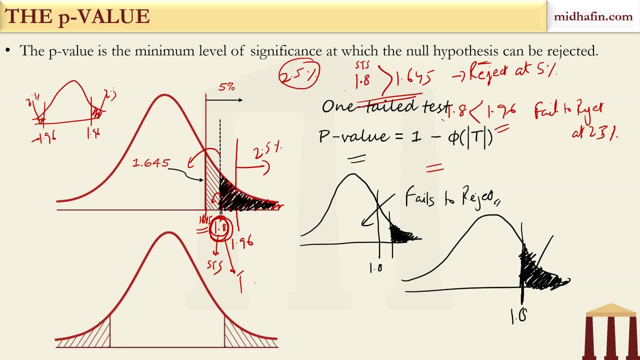 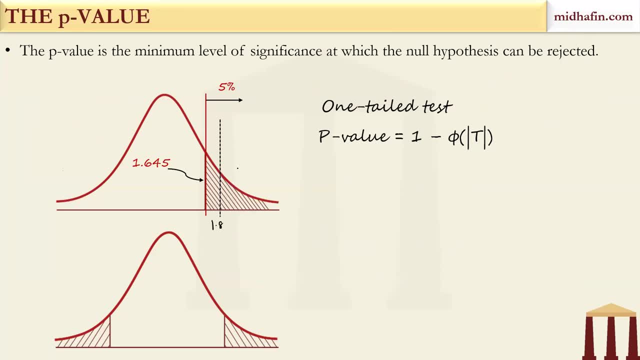 spread. I mean almost all the normal distributions you can see are having the same dispersion. OK, so the level of the error terms is not changing with the level of X And in fact it is constant. But in the second case the dispersion or the variance is. 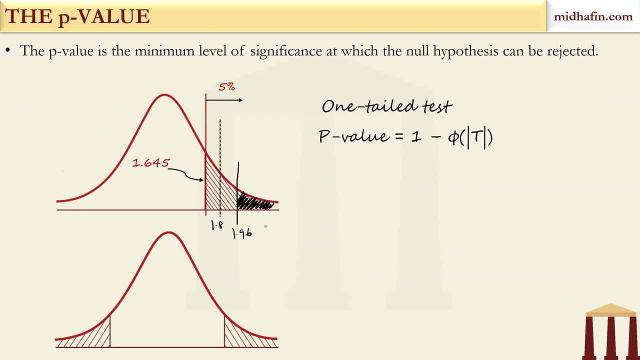 increasing with the level of X, and this is a problem. This is known as heteroscedasticity. In fact, there are two types of heteroscedasticity: conditional and unconditional. This is actually a specific case. This is actually conditional heteroscedasticity. 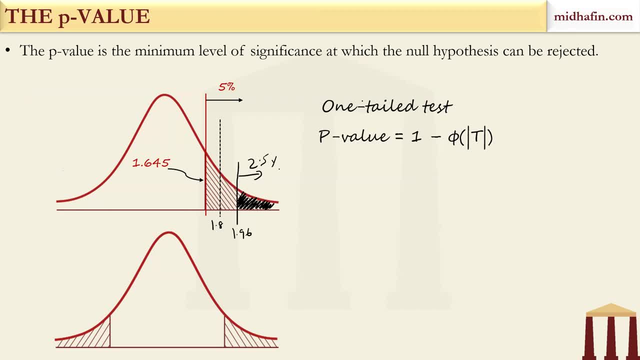 because the dispersion is increasing conditionally with X. I mean, there is, it is. if suppose it was sometimes increasing, sometimes it was decreasing, sometimes it was becoming random, even if it was not constant, even if it was changing, but it was not systematically changing with the level of X. 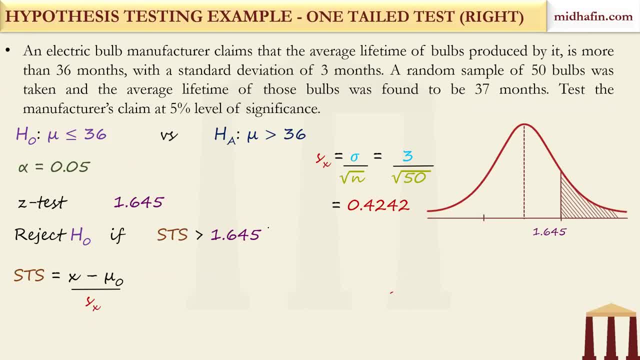 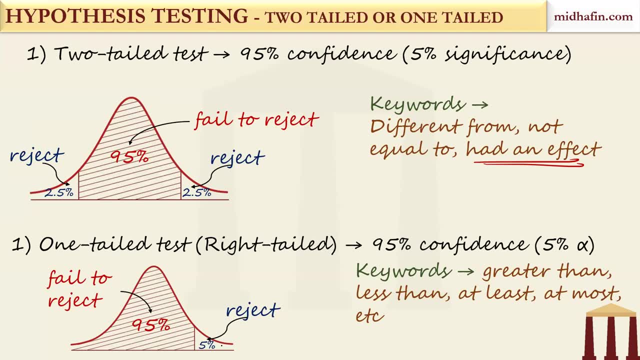 then it would be unconditional heteroscedasticity. Even that can be dealt with. Homoscedasticity is not a problem because this is the ideal condition. That is the assumption. But what about, OLS, Even if you have heteroscedasticity? 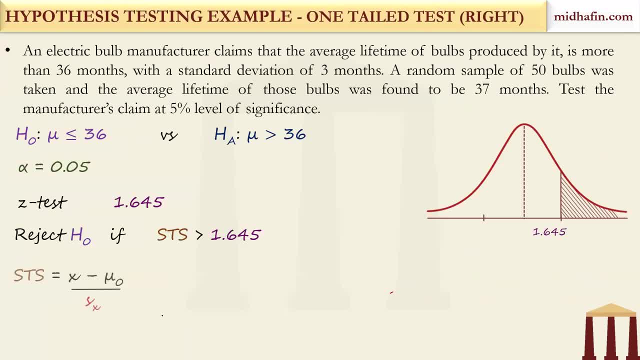 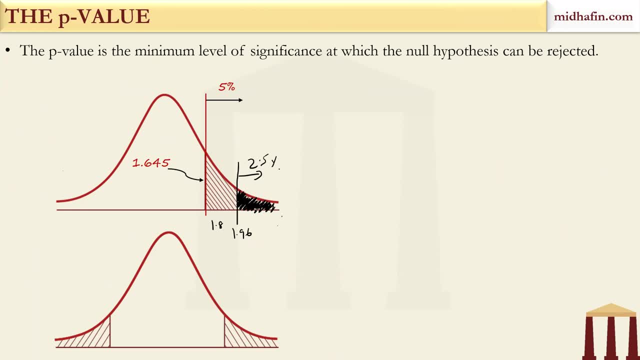 unconditional is still acceptable. still, you can manage Conditional. it is very difficult to work with conditional heteroscedasticity. OK. so there are some tests and there are some methods to remove it. Now, what are the properties of OLS system? 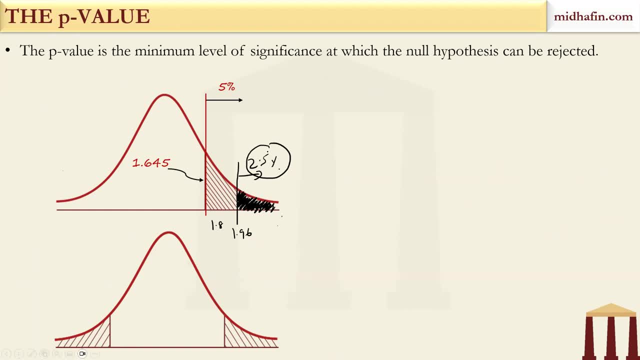 This is also one part which I think many candidates tend to ignore, because the hypothesis testing of beta will require- And this is something which has been given in such a complicated way in the book. We have tried to simplify it as much as possible, So you remember what we teach today only. 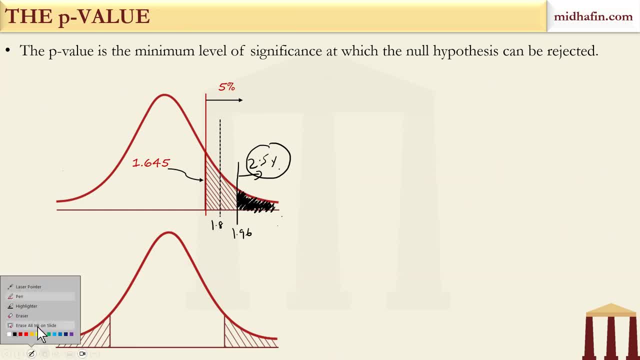 from the point of view of this learning objective. as far as regression coefficients, hypothesis testing, is concerned, OK, so this Properties of OLS slope estimator is being taught in the context of hypothesis testing of slope coefficients. OK, so in practice, what you do is the first. 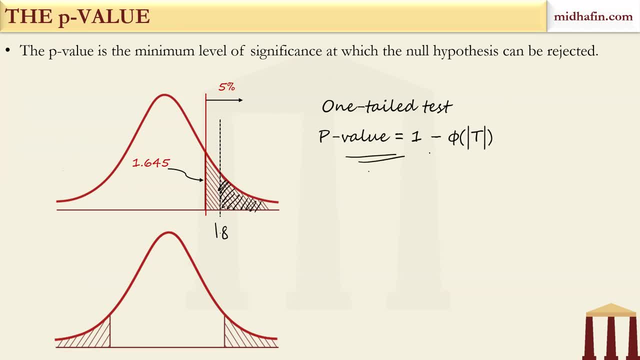 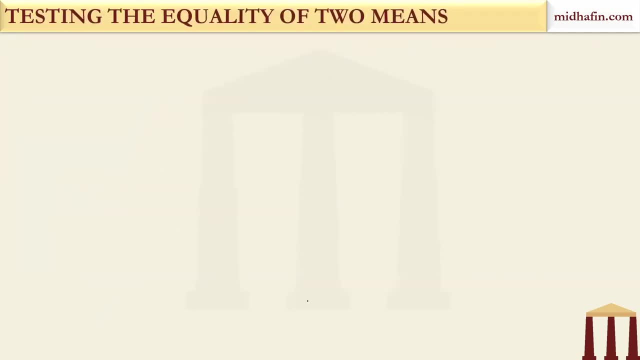 thing you do is you treat beta hat as a normal random variable which is centered around the true value. beta it means the mean you assume to be beta. See, when you have to test the hypothesis for beta, what do you need? Do you remember? how do we test the hypothesis? 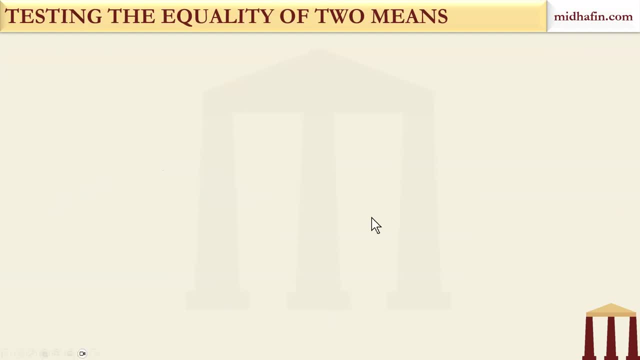 We need a hypothesized value. we need standard errors correct. We need estimated values of beta. So, estimated value of beta you have. You also have the mean now with the assumption of a normal variable. What else you need? The denominator is standard error. 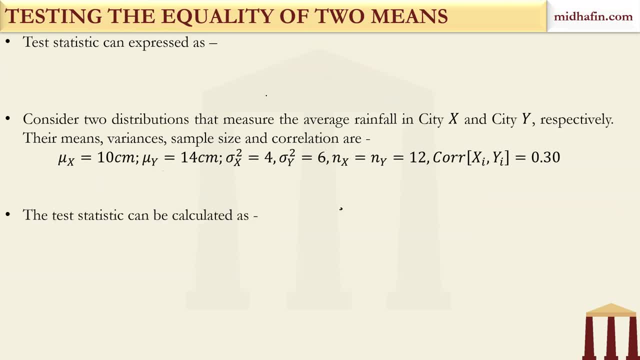 So estimated. standard error Is given by this form. Standard error of beta is s, divided by root, n, sigma x, hat and what is s. This is s. the square root of this is s. OK, so s is the square root of s square. 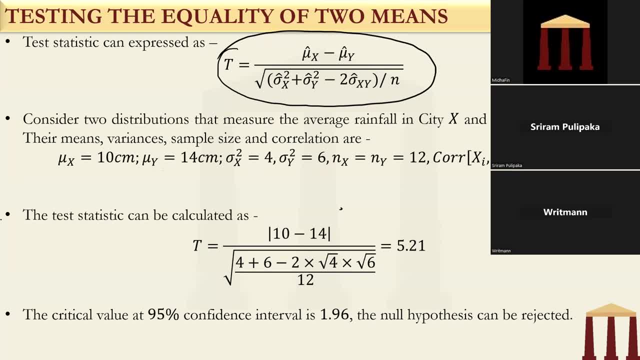 So these formulae, these two formulae, are important if you want to test the hypothesis for the statistical significance of beta. OK, so let's continue with the previous example. Let's continue with the previous example. These are the results we already got. 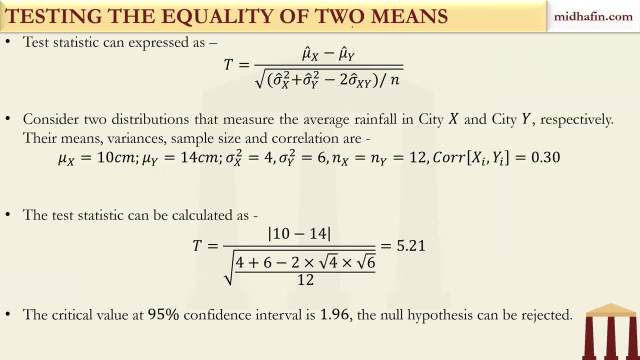 So alpha and beta were already estimated earlier for the same example. OK, Now, if you want to perform this test of statistical significance Now, before I proceed, I want to just ask any candidate who can reply on this: When we perform test of statistical significance, 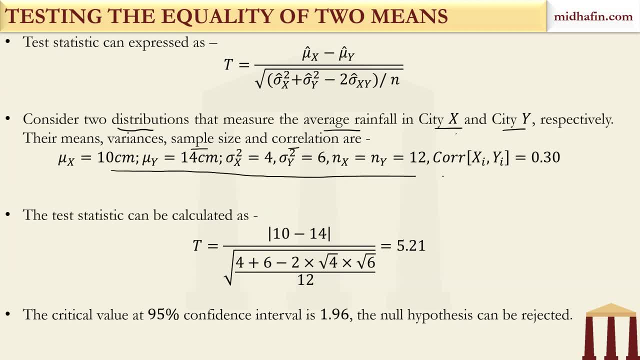 Against which value we are testing. it means what is the hypothesized value Over here? If we are testing statistical, it is Zero. Very good, It is zero Because you want a test of statistical significance. So statistical significance means whether it is statistically different from zero or not. 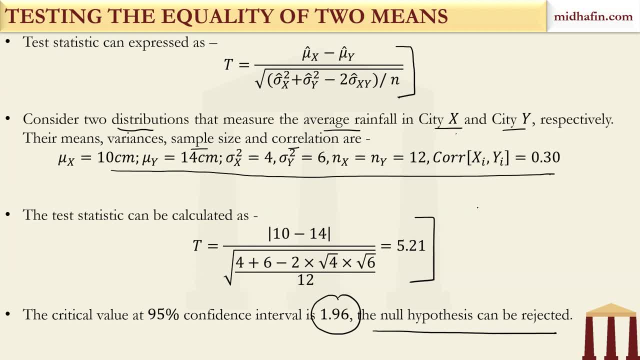 If it's not significant, it means it is zero. So test of statistical significance always imply a hypothesized value of zero. So this is how you will perform a test of statistical significance: Your null will be at beta equal to zero. Alternate will be beta not equal to zero. 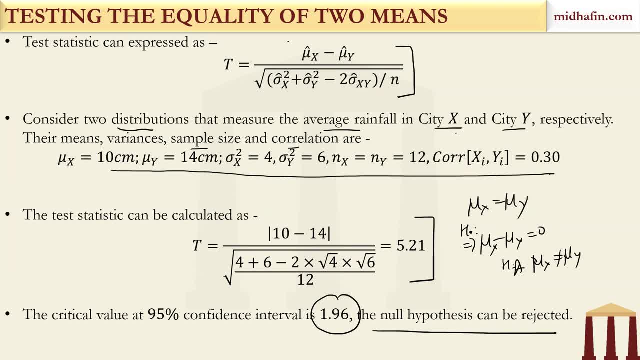 Got it. Then your sample test statistic: how you will calculate it. This is the formula for sample test statistic, The same formula that we've been using: Beta at minus beta naught divided by SE beta at Now, as I told you earlier that we were performing Z test in hypothesis testing, 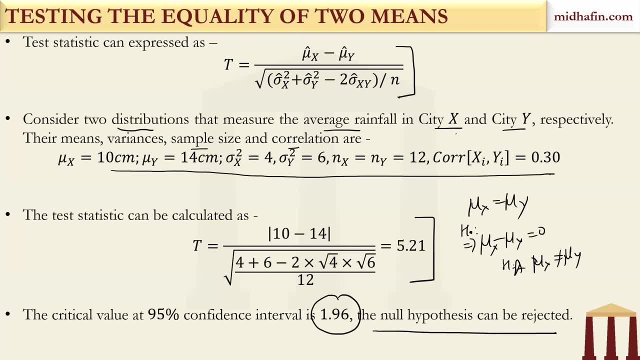 What did I mention about which test we'll do in hypothesis testing for linear regression? Which test? T test. So, over here in the exam, if T table is not provided, which I don't think they will, they will directly give you the two-tailed critical values or the T critical value. 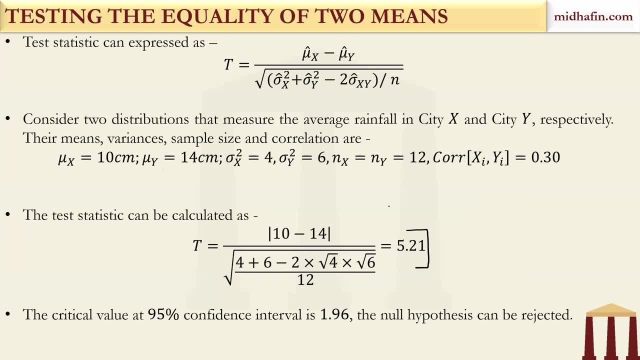 Most probably. If they don't give you, you should at least have an idea how to look at the T table. That is also very straightforward. So it is given to you that 95% two-tailed critical value is 2.09.. 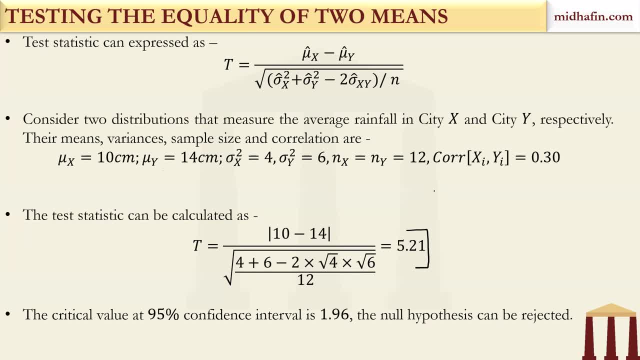 And why two-tailed guys? Can you tell me why we are using two-tailed, Why not one-tailed Again, anyone You can answer, Because here there are no keywords, Sorry. Equality: Very good, Because, see, we don't have a problem segment over here. 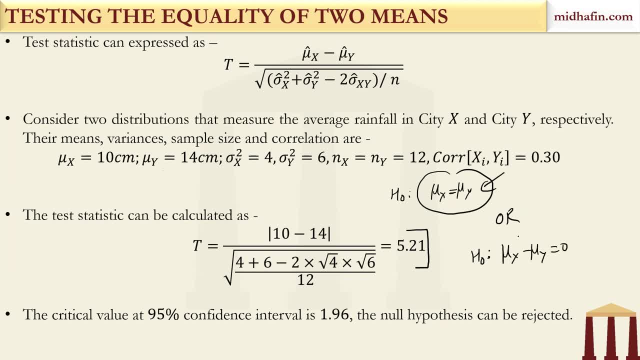 But the hypothesis itself, if you have equal to and not equal to, it means you are already testing two-tailed, because equal to not equal, not equal to can be on both sides, left-hand side also, right-hand side also. So it is very clear. 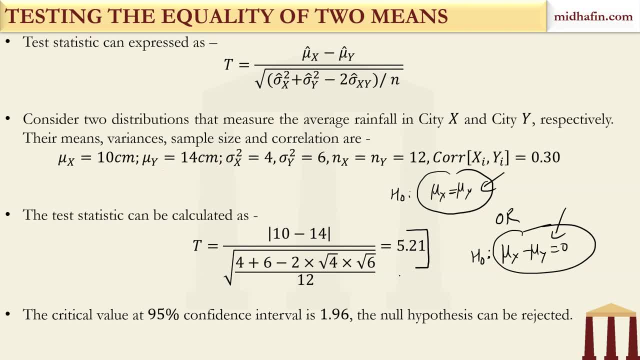 Is it clear to everyone? Is this clear to everyone? Okay, So make sure. Shreyas, are you asking this? Beta estimation is as close to mean. Can you just repeat, Shreyas, is it a question that you're asking? 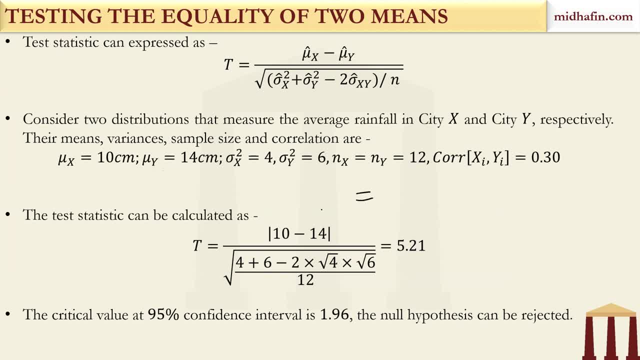 Or something that you want to convey. Okay, not a question. Okay, So you are mentioning that beta estimation is as close to mean of, may I know, mean of the true value? beta only right? That is what you're saying. 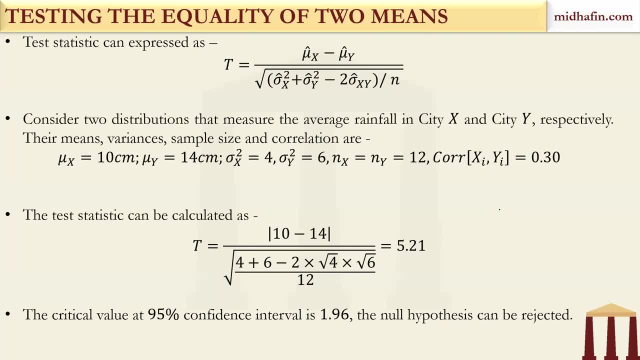 Okay, for two-tailed test. you're saying: For two-tailed test. you're saying: beta estimation is as close to mean. It's not very clear. Just try and reframe your sentence. okay, Beta estimation is as. yeah, please. 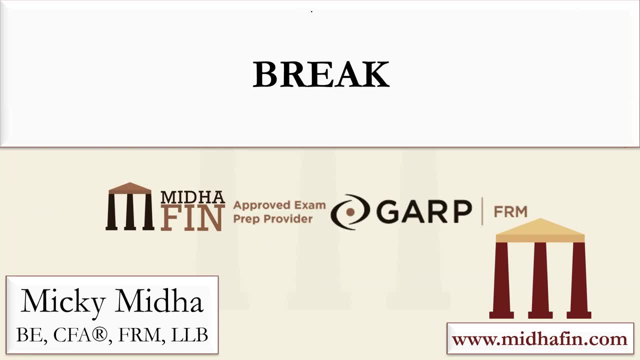 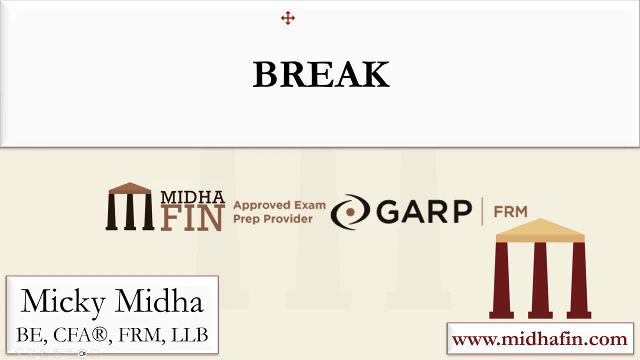 But in this case, actually see, in this case we don't have the idea about the mean. Okay, we are actually testing the statistical, So we are testing whether beta is close to zero or not, not the mean. So instead of the mean, you should say zero. 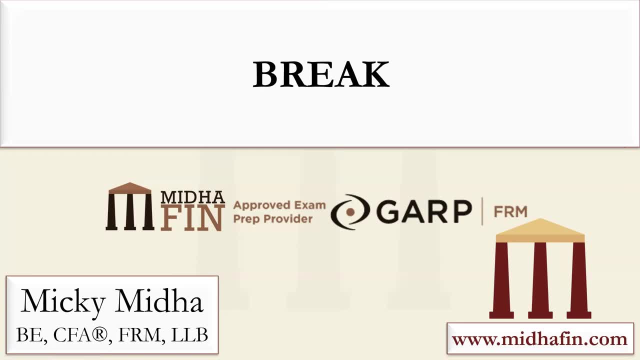 Got it. Okay, so that is the idea. fine, Okay, so what was the formula for standard error of beta? Okay, this, you know. what is the hypothesized value? This is very clear. This is zero. You're testing against zero. 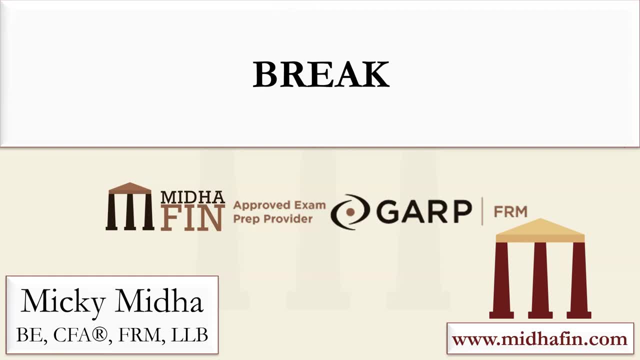 Okay, this is already estimated 1.5188.. What else you need? You only need the denominator standard error of beta. This is the formula for standard error of beta S by square root of n times sigma x cap. So again, let's reproduce the covariance matrix for reference. 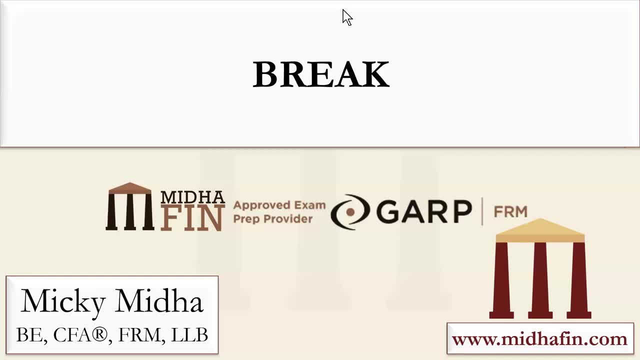 so that you don't miss out on the numbers. So one thing I can assure- I mean I'll not say assure you. I think I can say with a reasonable degree of confidence, I mean just like we've been using the hypothesis testing terms. 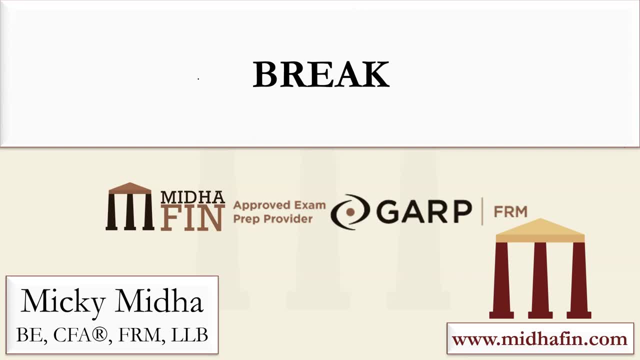 that they might not give you the full long calculation. It is possible that they'll directly give you the standard error of beta like this: They'll give you and they just. you just have to test, Okay, But what if you have to calculate? 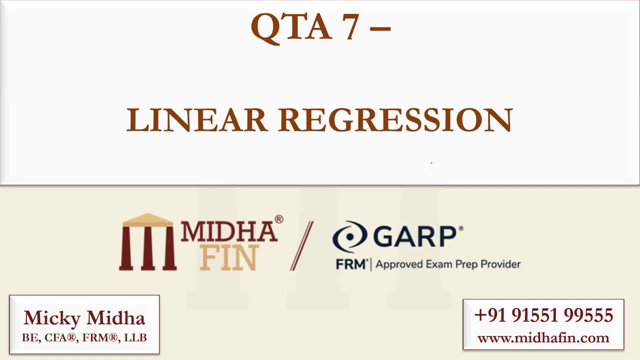 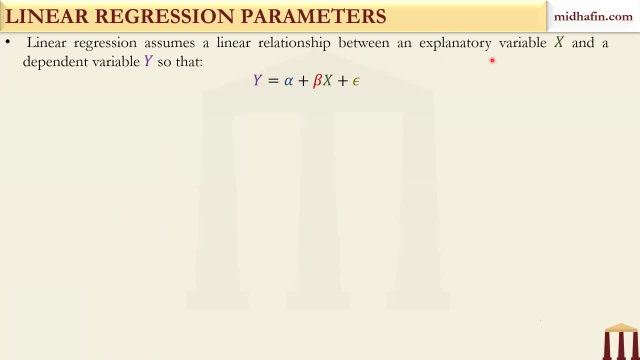 So, if you remember, This was the formula S divided by root, n, sigma, x, cap. But how do we get this S? So that is why I told, remember the formula of S square also. Okay, And S square was nothing but this much. 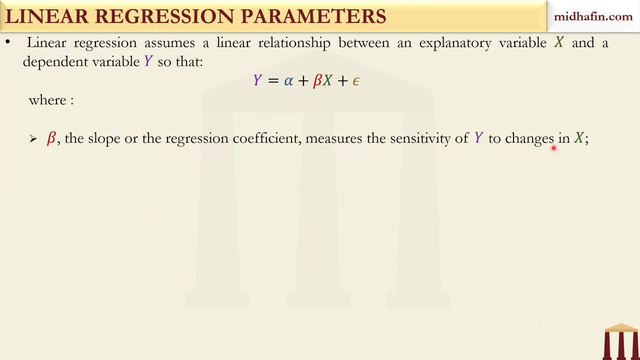 So this is how you will calculate S square: first, Then you will calculate standard error of beta. Is it clear? Okay, Also tell me. I mean we are going backwards actually. Also tell me: for calculating S square, we need one more parameter. rho. 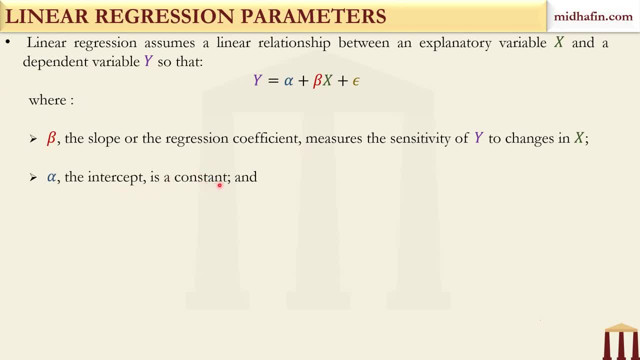 Do we have rho? Is it given? Okay? so why I'm going backwards? Because they will give you directly this, most probably. If not, maybe they will give you directly this So you can perform this. If not, then you have to do this. 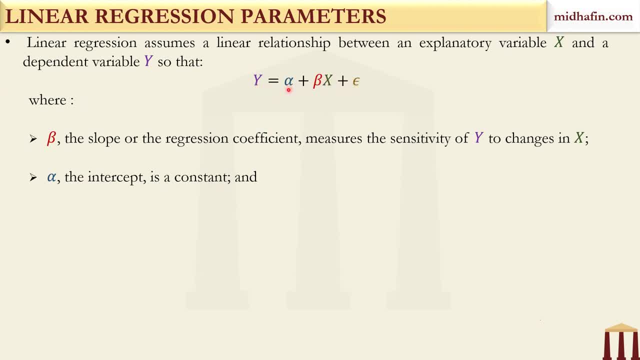 But for this also you need the correlation. How you calculate the correlation? Quite easy: from the covariance matrix Directly. you will calculate it as 0.6330.. Yeah, So just see all the calculations. Are the calculations clear? Check the calculations. 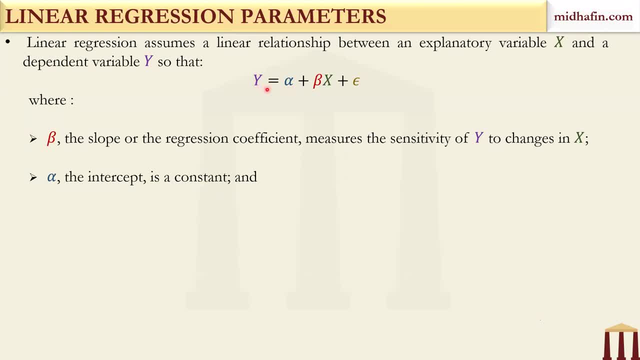 Just take the steps. You don't need to tally the numbers and all, Just check the steps. Are the steps clear or not? You can do the division later. Okay, Clear to everyone. Are the steps clear to everyone? Okay, And more. 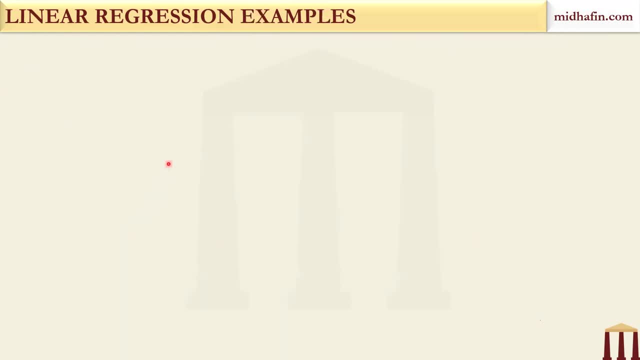 Okay, great, At least few of you should reply Now. standard of beta we have got as 0.4042.. Let's find out what is the sample test statistic: 3.76.. So we know that 95% total critical value was 2.093.. 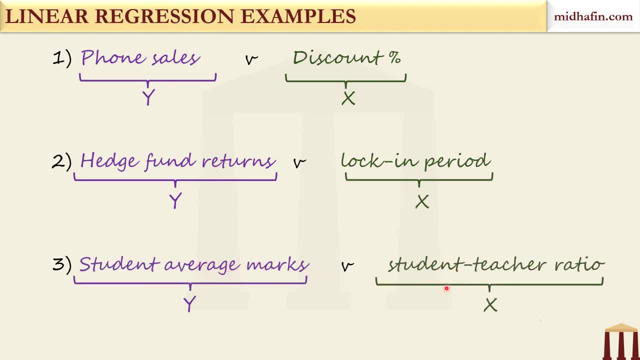 So this is: 3.76 is greater than 2.093.. It means we reject the null. So what is our conclusion? Do we have reasonable evidence to claim that beta is statistically significant? Because we are rejecting the null? it means that 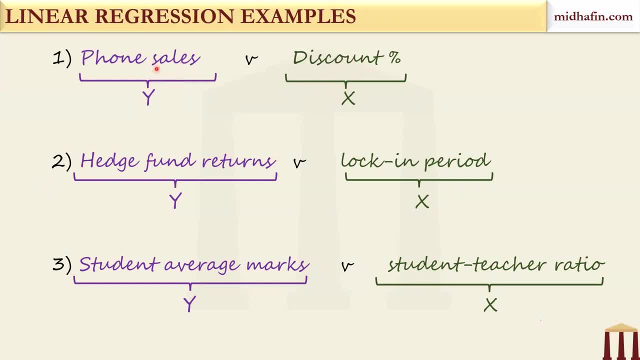 we are rejecting this. So do we have sufficient evidence? Now, In fact, this is correct. Okay, Yeah, So beta is yes, So we will conclude that beta is statistically significant at 95% level of confidence. Okay, So this is what hypothesis testing of slope coefficients will involve. 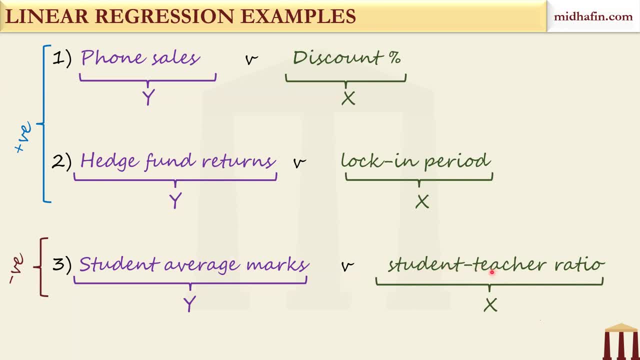 You may also be asked to construct 95% confidence interval for beta. So you know the same thing. I mean you will be given the critical value standard error. Either you will be given or you have to calculate. Process is same, Okay, So I will not go into this right now. 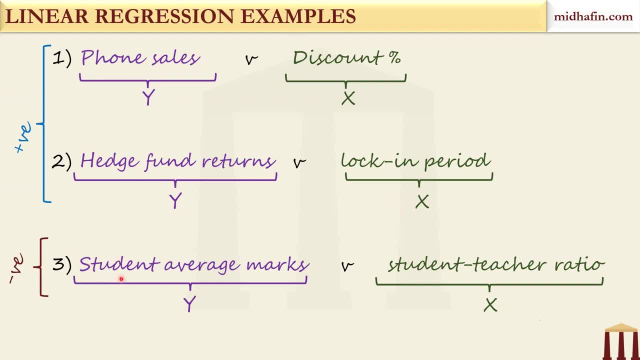 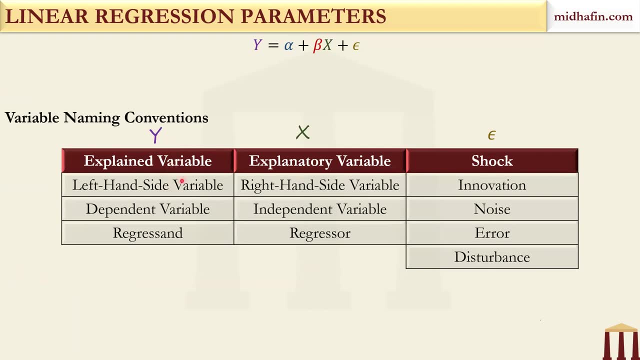 Then p-value again the same process as we have been doing in the hypothesis testing chapter. So there's no difference at all. Okay, fine, So that's it for this chapter. Are you guys okay if we don't take a five minute break now? 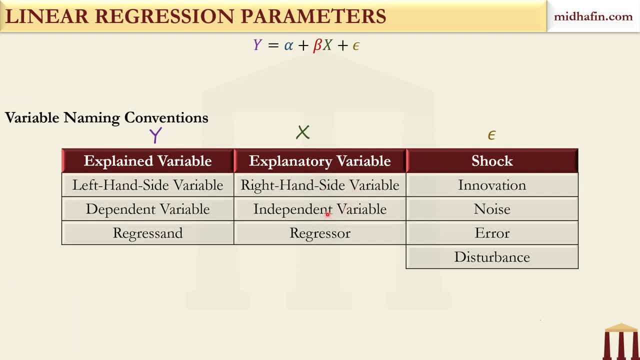 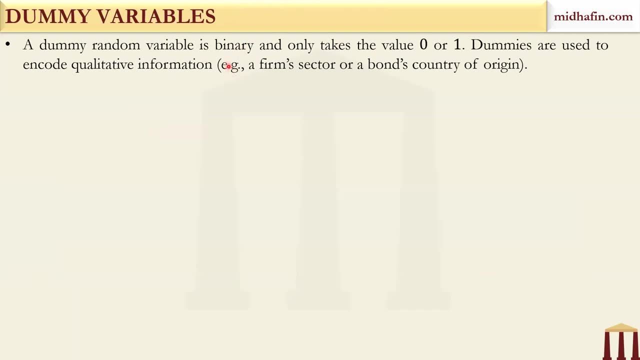 Can we continue? Okay, great, So let's continue with multiple explanatory variables as well. Okay, So regression with multiple explanatory variables. Now, multiple regression is a regression analysis with more than one independent variable, which is: yi is equal to alpha plus beta 1x1i plus beta 2x2i plus up to beta kxki plus a. 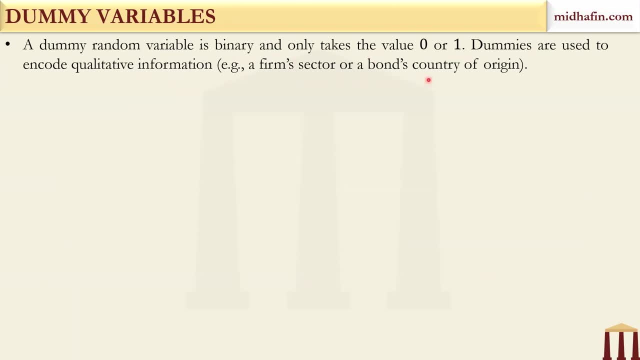 So there are more than one independent variables and these are the corresponding slopes. So assumptions are same. All assumptions of linear regression apply, with some minor modifications. Of course there are multiple regressors, So they will just be the assumptions will just be extensions of the previous assumptions. 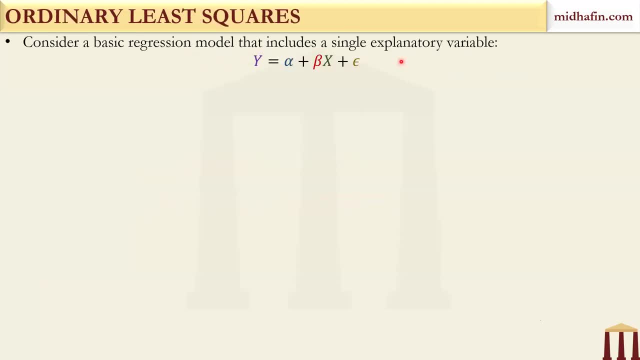 There is one additional assumption. This one: It assumes that explanatory variables are not perfectly linearly dependent, And this is very important. Again, there's a concept called multi-collinearity, in which this will be discussed once again. So what this tries to say is these variables- x2i, x1i, xki- these can be somewhat correlated. 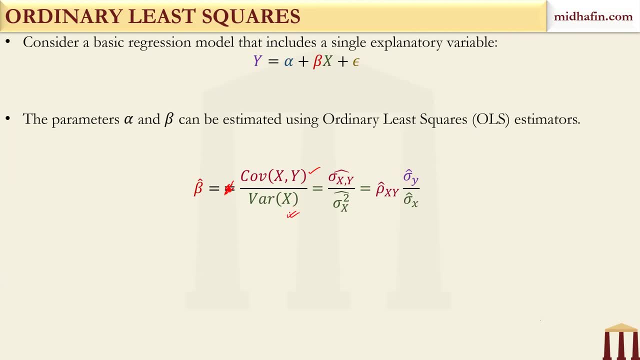 That is okay. See, the ideal scenario will be if they are independent, but that is not possible. Suppose: if you are carrying out a regression on the price of a stock, Okay, And you have explanatory independent variables like, say GDP, say inflation, say unemployment numbers. 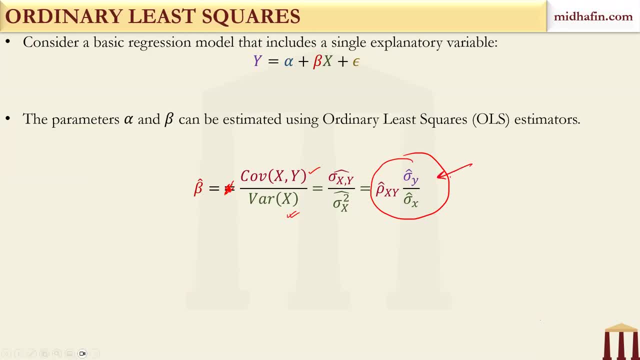 Can these be independent 100%? practically is it possible? Can these be independent? practically Not possible, right, So some correlation is okay, but they should not be perfectly correlated, Got it? So there is a possibility that maybe one of the parameters is perfectly correlated with, say, GDP. 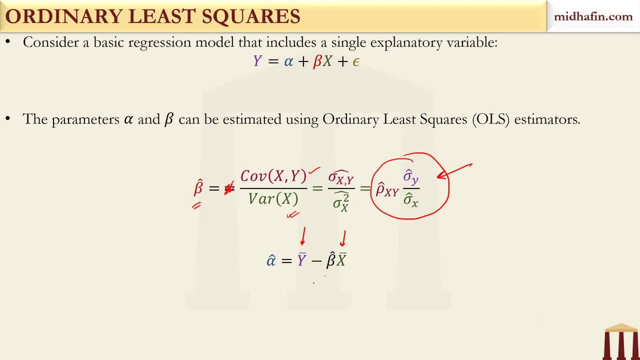 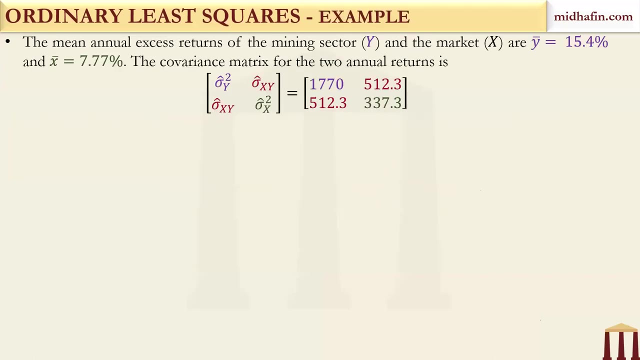 It's possible, Maybe one of the fact- GDP is an input in the calculation of some parameter, and even that parameter is being used. So then there is no point of including any extra variable. that is perfectly included, related with any other independent variable, because all the information is already captured. 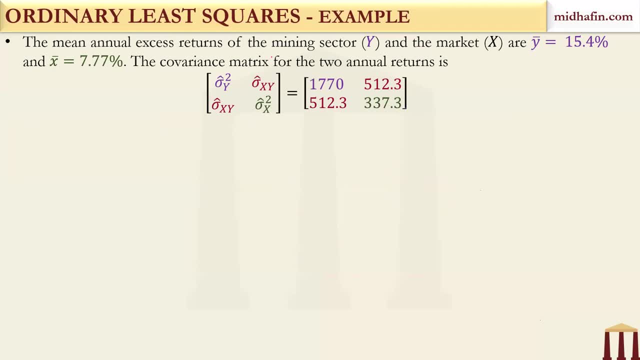 And this will lead to more problems. This will lead to problems of multi-collinearity. Okay, Now, what are the assumptions of multiple regression That we discussed? Now, what is the interpretation So earlier, in the last case, with single regressor? 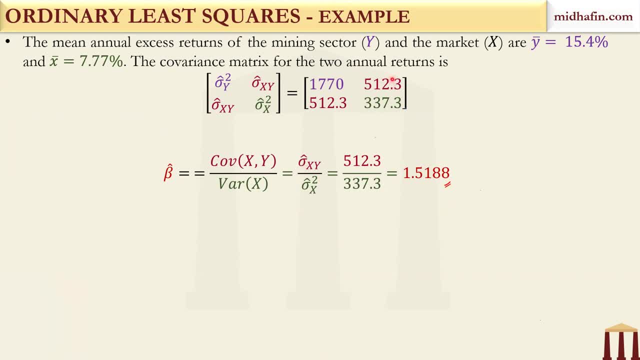 the interpretation of slope coefficient was that it was the change in dependent variable From a unit change in the corresponding independent variable, keeping all other independent variables constant. Okay, So basically you are controlling the effect of all other independent variables. Over there there was a single variable, single independent variable. 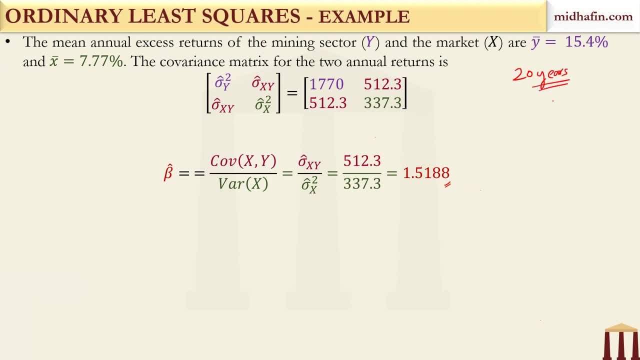 There was no need to control any other variable Over here. the interpretation is same. but you have to control the effects of other independent variables. You don't have to make them fluctuating, They have to be constant. So, for example, beta1 is the effect of a small increase in x1, holding all the other variables constant. 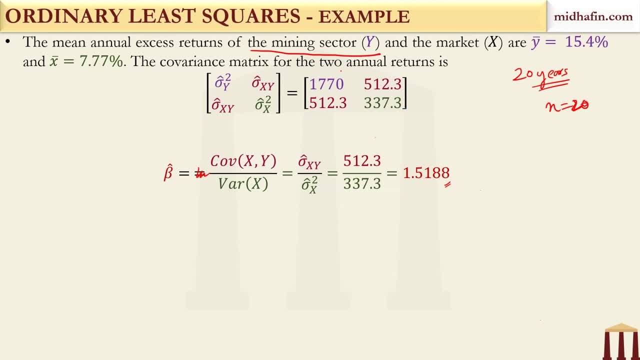 Okay. Now when the value of independent variable changes by one unit, the change in the dependent variable is not equal to the slope coefficient but also depends on correlation among the independent variables as well. Because see if, suppose, GDP changes by one unit. 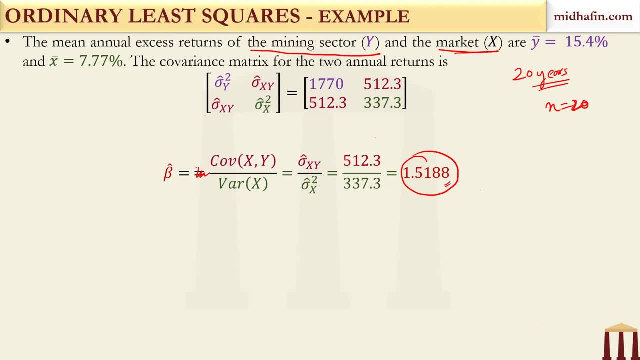 let's say in percentage terms by one percent, and you're carrying out a regression. and GDP affects unemployment also. So obviously the change in the dependent variable will not be the same as the slope coefficient corresponding to GDP, because at the same time 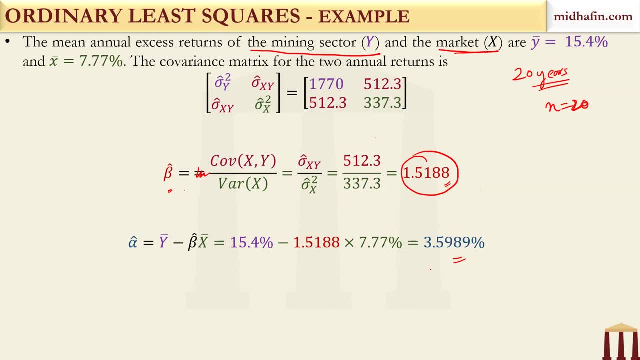 unemployment will also change. at the same time, inflation will also change. So that is why these slope coefficients, since we are controlling the effects of other variables to try, and you know, keep this definition alive over here. and it is actually the second point also. 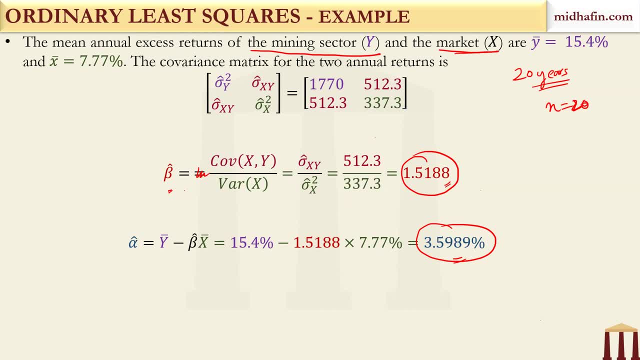 states that practically it is not possible, right? So that is why these are known as partial slope coefficients. They are not known as proper slope coefficients, they are known as partial slope coefficients. The interpretation of intercept is straightforward. It is simply the expected value of y when all xi's are equal to zero. 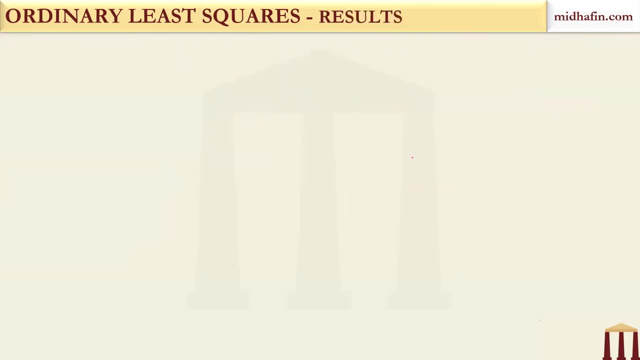 OK, now You all are very aware of the OLS regression for linear regression with a single regression. but most of the candidates they actually overlook the OLS estimators for multiple regression parameters. because it is actually difficult It is, the steps are very much detailed. 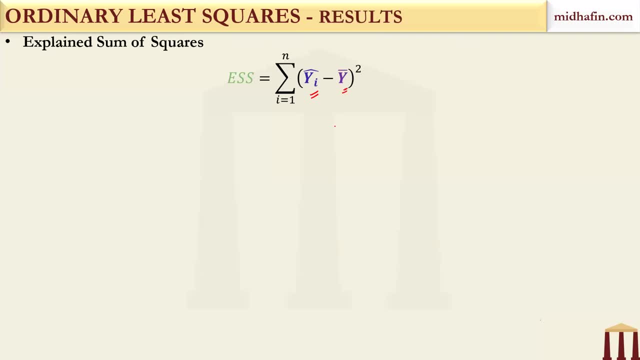 But again I'm saying: the good news is that they do not ask you to perform the entire regression, only the steps are important. That is what we have seen in the sample papers also and the feedback also. So let's say: this is a model with two independent variables. 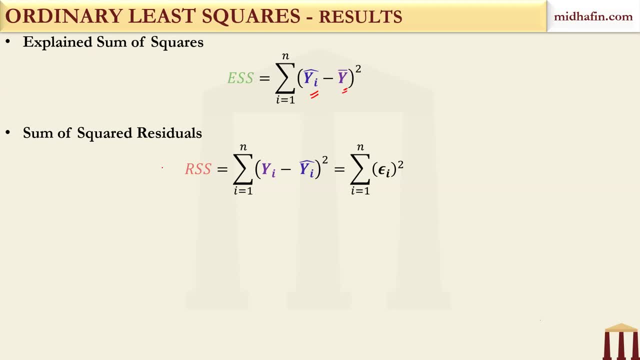 So what are the steps? if you want to calculate, See earlier it was very clear. the formula for beta was covariance between x and y divided by the variance of x. But over here you have two x's. So now for beta 1, you have 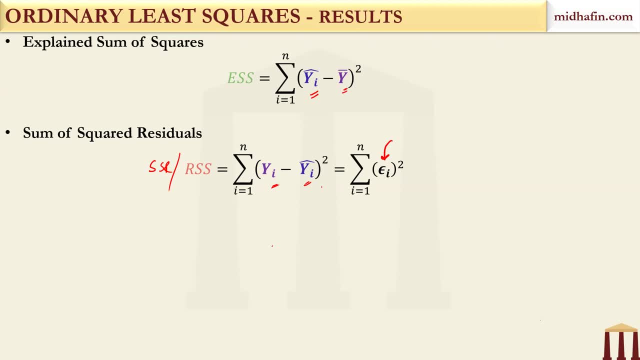 to first perform three single variable regressions. The first regression will be for x1 on x2.. So x1 will be regressed on x2 only And the residuals from this regression will be retained. Then the second regression will do the same thing on y. 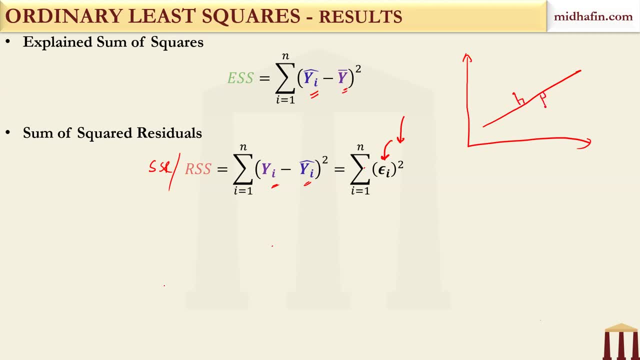 So basically, y is also regressed on x2 and the residuals are retained And finally, the residual of y is regressed on the residual of x. In fact, I think there was slight error in what I said. The first regression will regress x1 on x2 and it will retain the residuals. 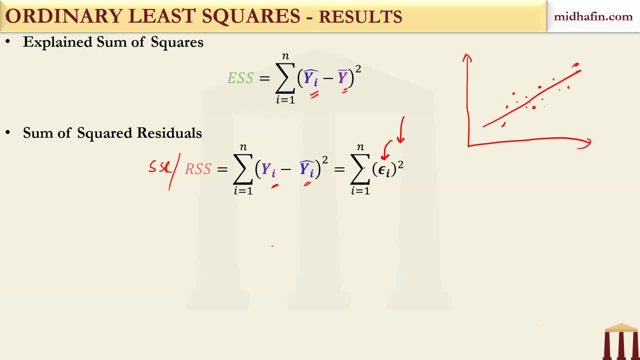 from this regression. The second regression will regress y on x2 and it will also retain the residuals of that regression. Then the residuals of the two regression will be regressed. OK, so these are the three regressions Which are carried out. 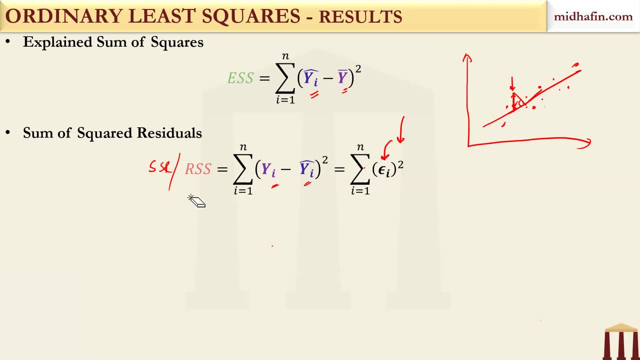 OK, and for beta 2, the same thing will be done. The only thing is that the rules of x1 and x2 will be interchanged. So the first regression will be done by doing regression x2 on x1.. So x2 will be your. 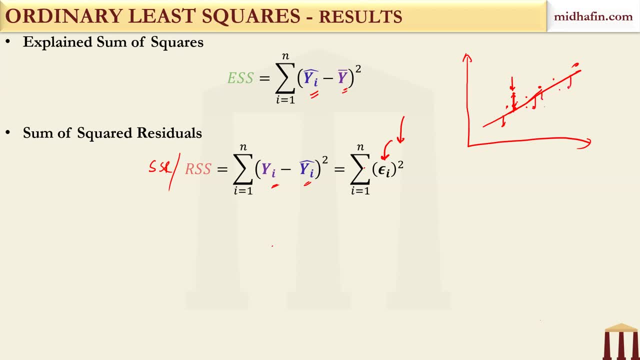 dependent variable. x1 will be independent, Then y will be dependent variable. OK, and x1 will be independent variable, and then residual of y on the residual of x2 will be done. OK, so the residual on the first two regressions will be done. 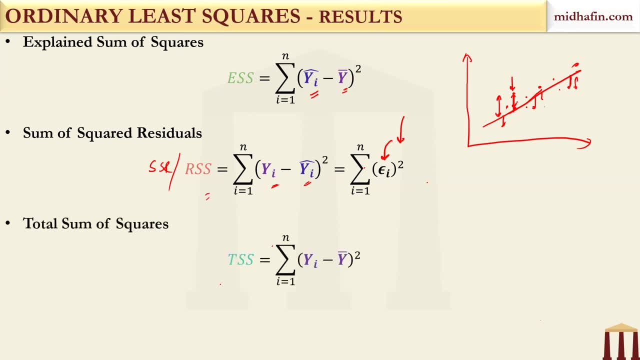 That's it. So these steps are important. guys, Don't worry about the detailed process. Of course you should. I mean, if you have gone through the curriculum earlier, then you might have gone through the steps and as well as the calculations. 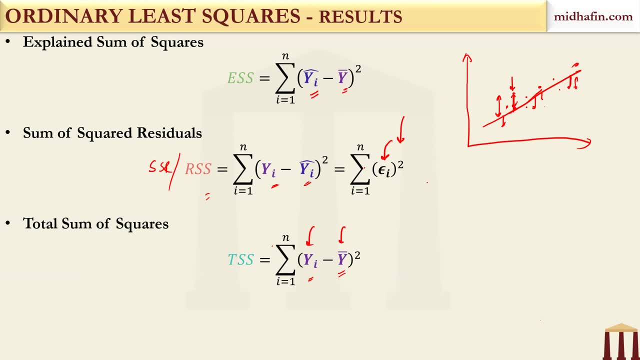 So keep that in mind also. But I think from the exam perspective, steps are more important. OK, So focus on the steps as well. properly Now, standard error of regression. This is the formula and it conveys the fit of the regression line. 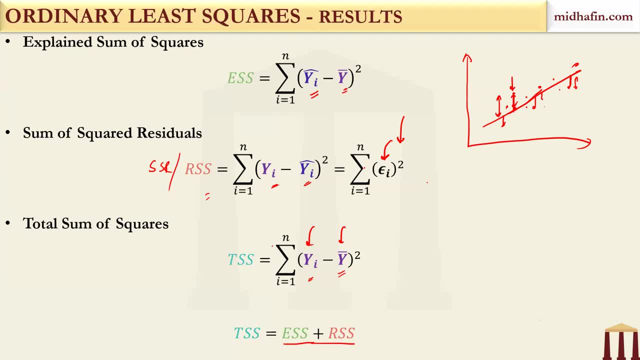 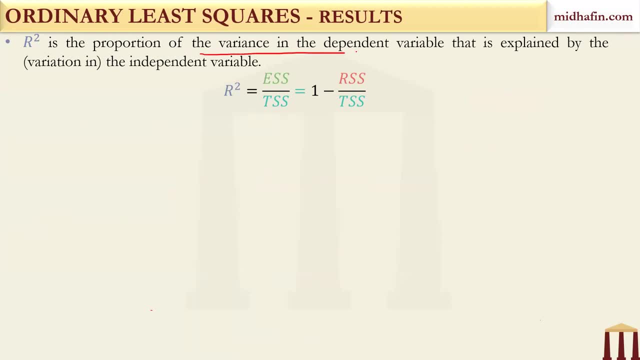 And the fit is better if standard error of regression is smaller. Now, if you remember, r-square was the proportion of variation in the dependent variable explained by the variation in independent variables, And I told you that earlier. the correlation was equal to square root of r-square. 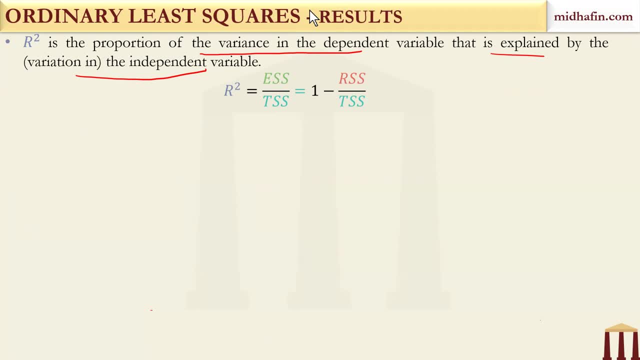 But I said for multiple regressors, that is non-regressive For multiple regressors. this is the case For multiple regressors. r-square is the correlation between, in fact, squared correlation. Squared is missing, So that correlation was between x and y. remember. 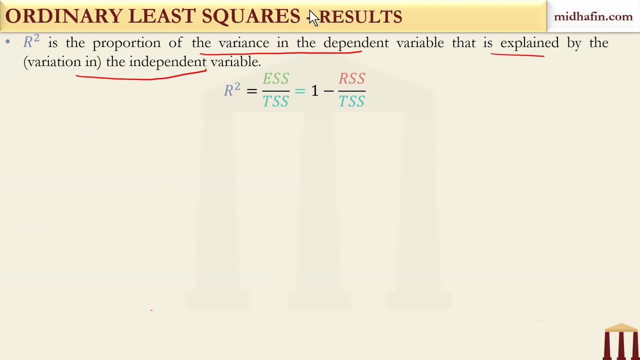 Earlier for single regressor. this has to be clarified. r-square was equal to rho-square between x and y, But this correlation is different. This is a correlation between yi and the fitted value of y, So between the actual and predicted values. 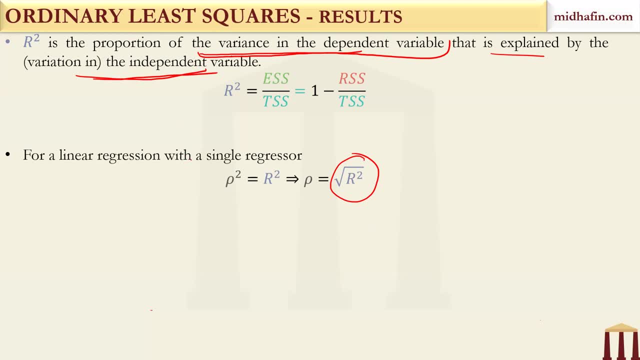 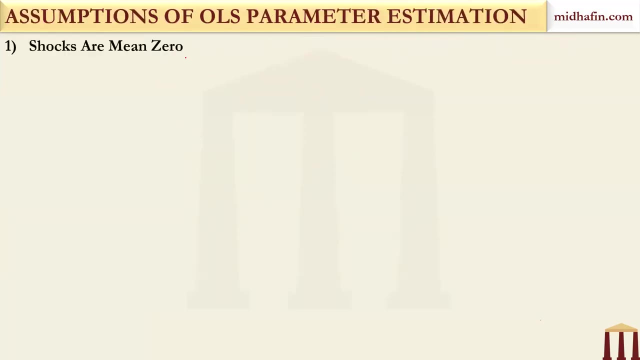 you take the correlation, you calculate the correlation, you square it. that will be your r-square. So this distinction is very important, asked multiple times in the exam. Now there are problems with r-square. Now, if you add a new variable, even if the new variable is insignificant, you will 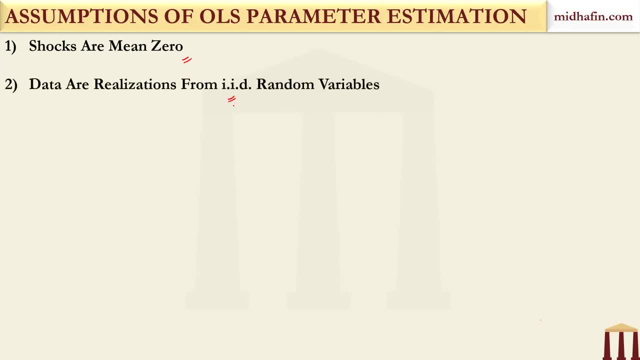 find that your r-square is always increasing, which means you will be under the impression that you are creating a better and better model. That will not be the case, OK, so that is one problem. Another problem is r-square is not comparable. 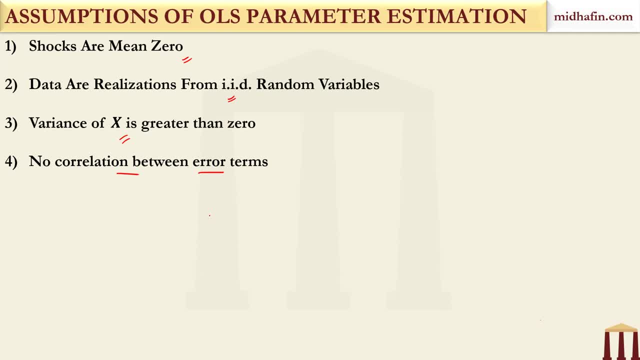 And there is no general value for which which can be considered as a good value for r-square. So, again, depending upon the problem being studied, maybe even r-square value of 85 might not be great, 85% or 90%. 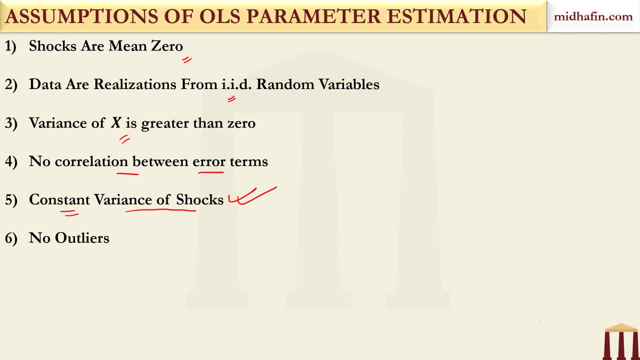 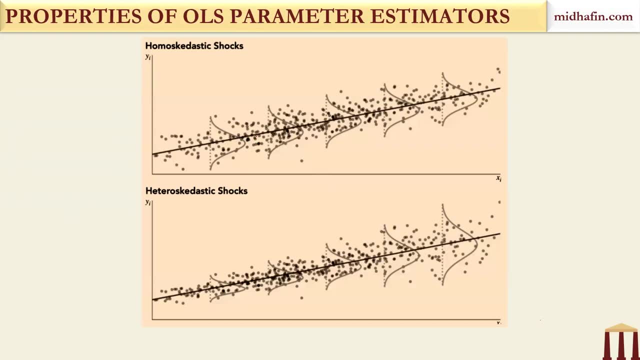 But for some other problem maybe 70% r-square will be very good. So it totally depends on your stream, the kind of success that other people have got based on that experiment. OK, depending upon the domain, as I said, OK, and it is not comparable also. 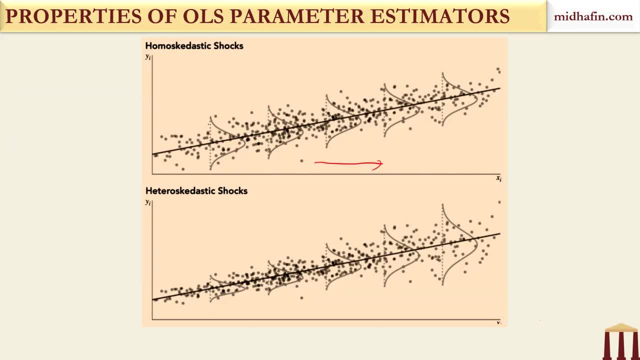 So what other measure you use to address some of these limitations, not all, but some of these limitations. the first limitation can be addressed How? By adjusting this r-square. So this is the formula for adjusted r-square. OK, It includes the number of independent variables also. 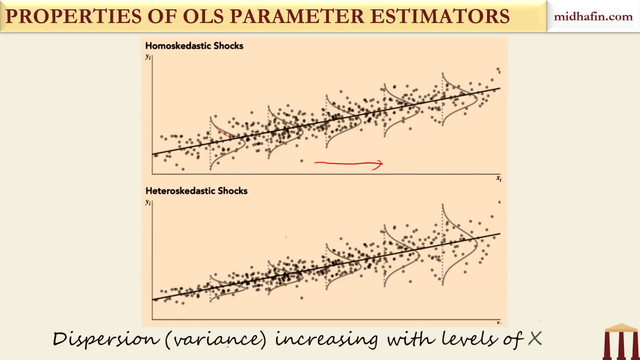 And the same formula can also be expressed in the terms of RSS and TSS, like this: 1 minus epsilon RSS by TSS, where this is epsilon n minus 1 by n minus k minus 1.. So one thing you have to remember: that this should be greater than 1, has to be greater than 1 because 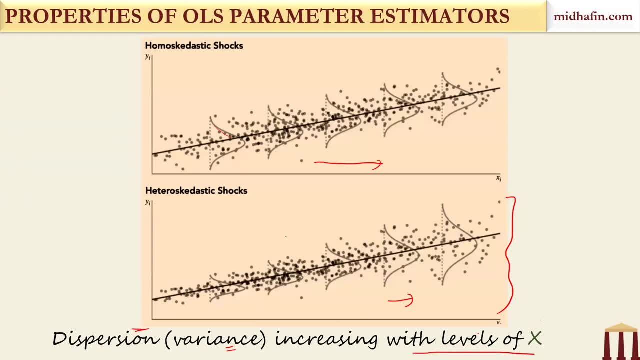 the denominator is less than the numerator. Now, if k increases, if the number of explanatory variables increases, then epsilon actually increases, but RSS decreases. OK, so the net effect adjusted r-square might increase or might decrease. So that is why adjusted r-square has this property that like r-square in fact. 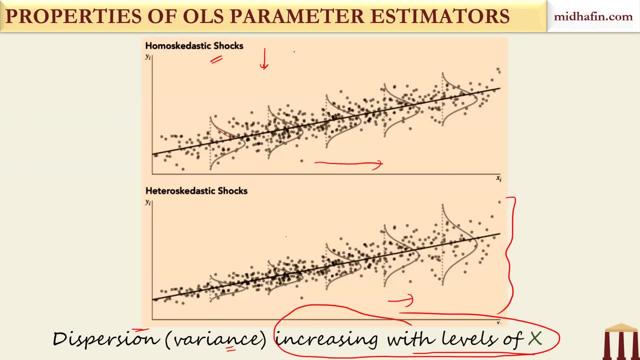 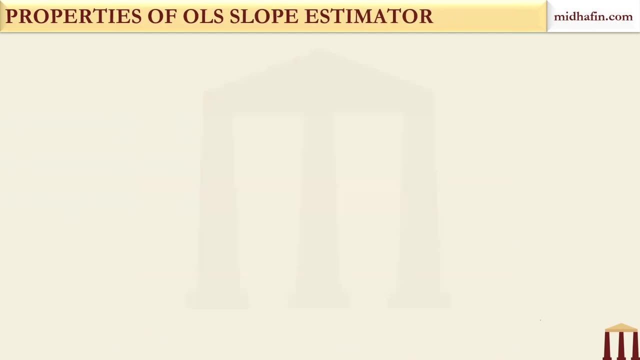 I should say it does not always increase. with the increase in independent it might also decrease. In fact, the example that we have given in our PDF: we have actually adjusted r-square, has actually decreased Right. So if k increases then there is no guarantee that adjusted r-square will increase. 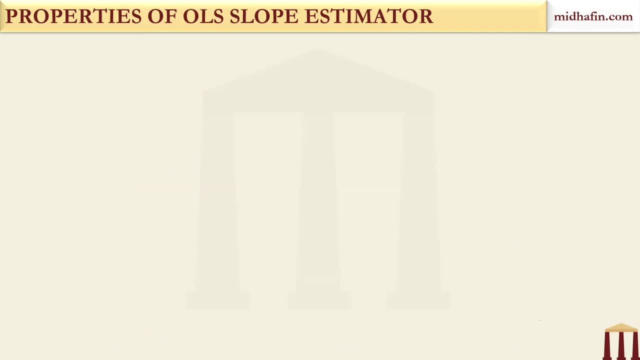 It may increase, it may decrease. That is why it is a better measure as compared to r-square, which always increases. Now, if you want to perform tests of null hypothesis for individual tests, you can do the same process which we have discussed earlier in the last lecture. 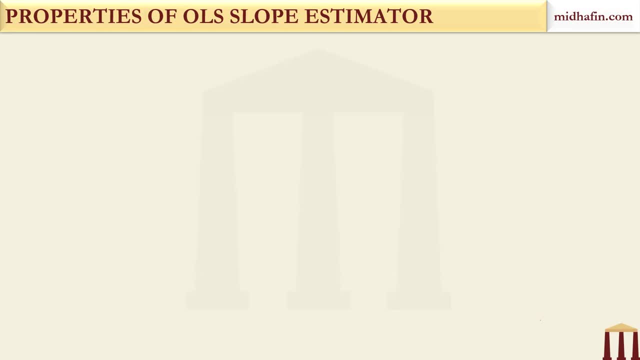 Linear regression with single regressors very straightforward. But if you want to do joint test, that is for single test. Now there are different kinds of joint test. One joint test is the joint test where restricted and unrestricted models are tested. Another joint test is there which was a part of the 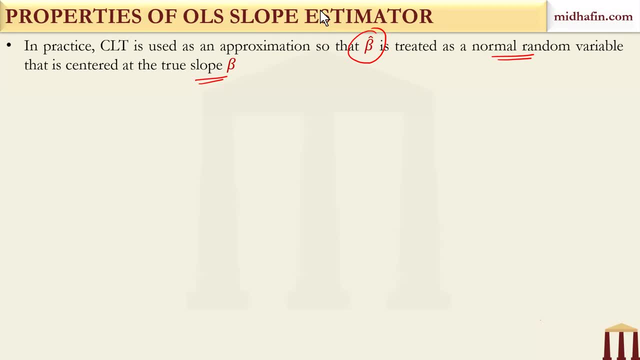 pre-2020 curriculum, which has been removed, which, again, I think was actually an important test. I don't know why they have removed it, So I will not discuss it today, but we have discussed it in our videos and the PDF. 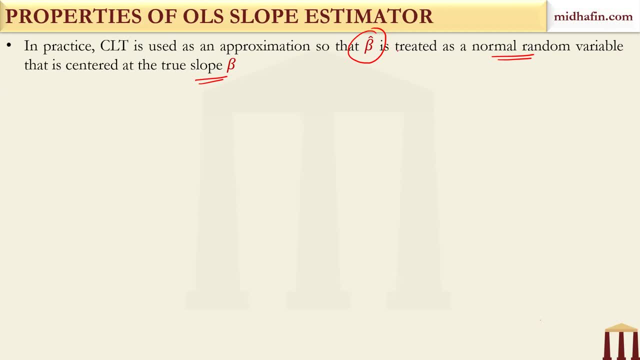 But from the exam point of view, since it's not there in the GARB book, so it might not be honest, But I'll tell you the crux of that test. So basically it was the joint test of all the coefficients together. 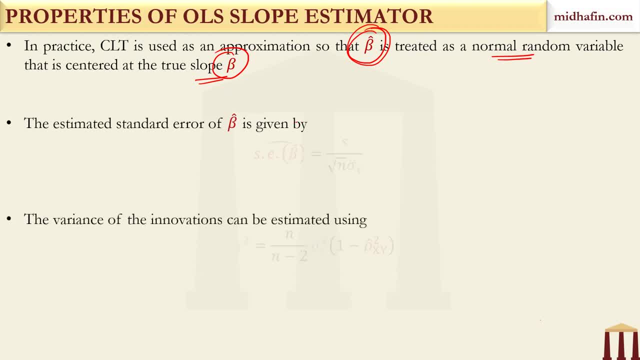 that all the slope coefficients will be equal to zero And the F-statistic. the interpretation of that test is there, But the test perform. how the test is performed, that is not there in the curriculum. So The joint test- I mean this question- can be asked in the exam. before I proceed, 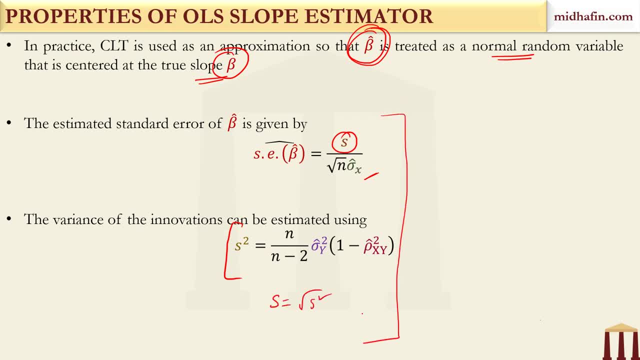 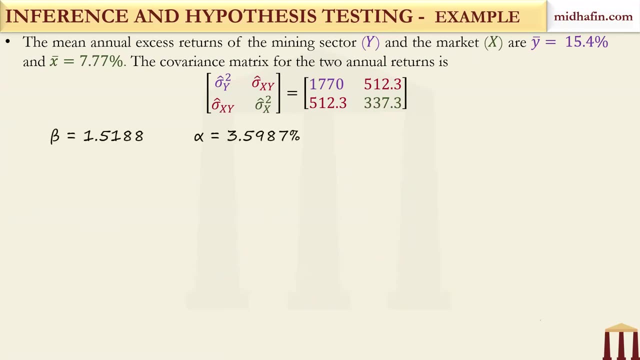 to the next joint test. that let's say, if you are given that you perform a joint test, So remember that joint test will always be performed using a F-test. So joint test means you are testing that beta 1 equal to beta 2.. 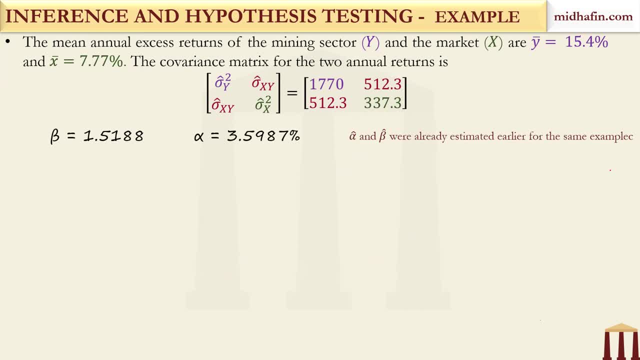 Let's say there are only two coefficients, one of them is not equal to zero. so both your coefficients are zero, versus at least one of them is not equal to zero. So HA is at least one of them is not equal to zero. So this is what you do. This is F-test. 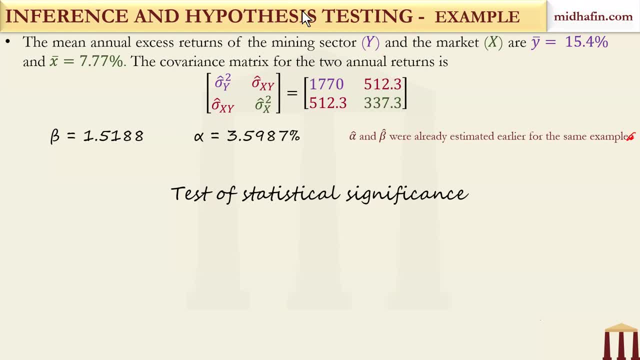 So a question can be asked in the exam that from the F-test you conclude that these are jointly statistically significant. let's say It means that you reject this null. It means you conclude that they are jointly statistically significant. Either they can ask this in the form of a direct F-stat value. 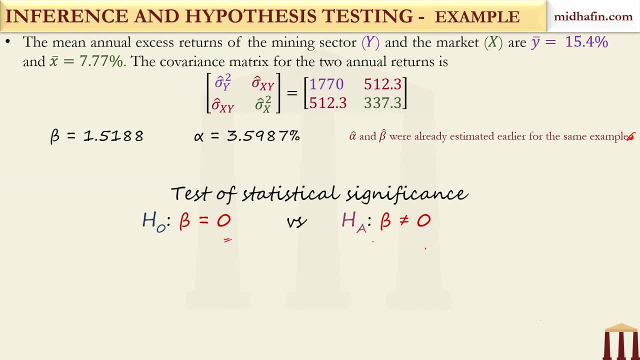 or they can give you the R-square value or they can give you the P-value. The most common question that we have seen is in the terms of P-values, So I discussed that. what is P-value? P-value is the minimum level of significance. 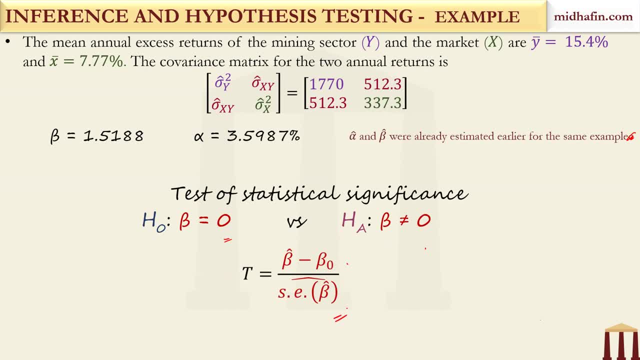 at which the null hypothesis can be rejected, Correct. So if I say that hypothetically, let's say the minimum level of significance at which the null can be rejected is 4%, Let's say hypothetically. So if you want to frame it in the opposite manner, 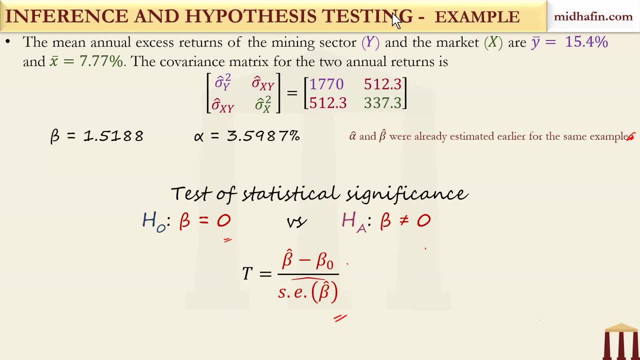 can I say I can be maximum 96% confident. Minimum 96%. Does this level of significance, does it translate to maximum level of confidence or not? Because significance level is 1 minus confidence level. Yes or no? Think about it. 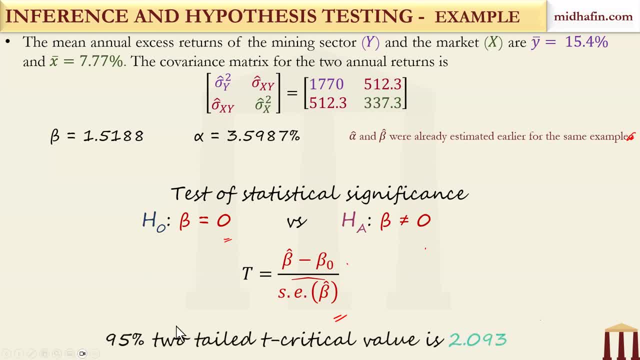 If this is minimum, this is maximum. Do you agree? Mathematically it makes sense, Everyone Right. So minimum level of significance corresponds to maximum level of confidence. Statistically, any P-value which is less than 0.05 is acceptable. 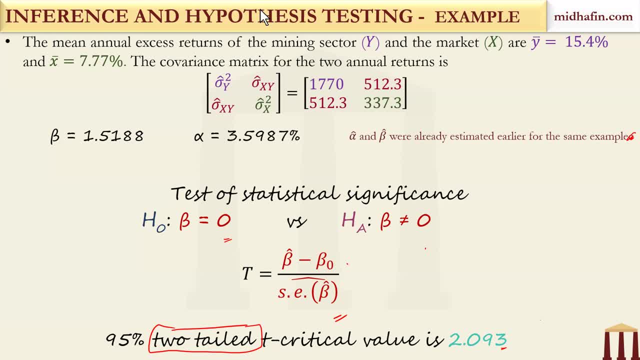 Any P-value which is greater than 0.05 is not acceptable. OK, again I'm repeating: statistically, any P-value which is less than 0.05 is acceptable, Greater than 0.05 is not acceptable. So it is possible that for individual t-tests, let's say for the individual, 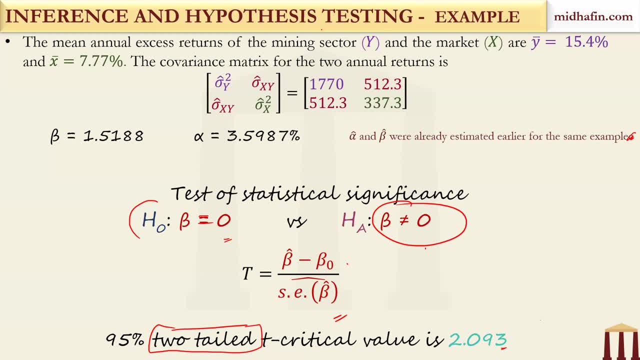 I'm giving an example. Let's say they give you a P-value of 0.12.. What will you conclude about the statistical significance of beta-1?? Tell me, What will you conclude about the statistical significance of beta-1? Statistically significant or not? 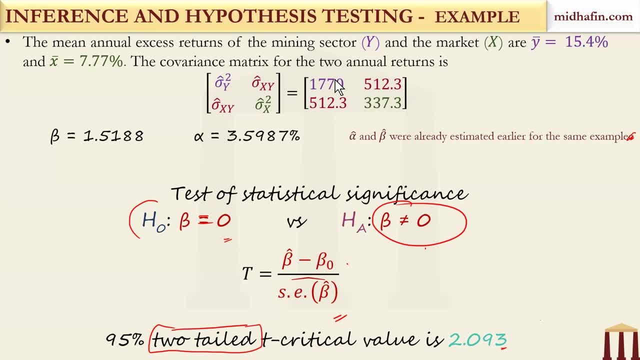 Because normally, yes, very good, If P is less than 0.05, then only you can conclude that it is significant. If P is greater than 0.05, it means you cannot be maximum 95% confident. You can only be maximum 88% confident, which is not statistically a good result. 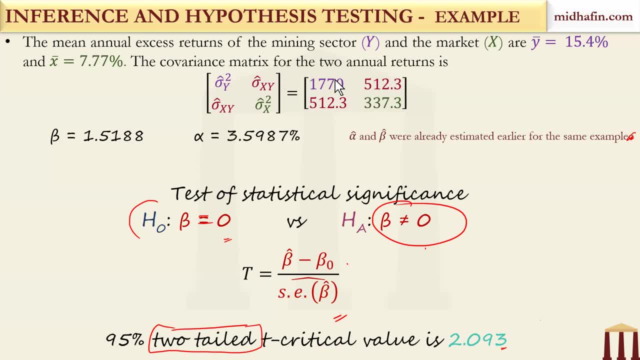 You should be at least 95% confident. OK. so for any test, if P-value is less than 0.05, it is OK, It means statistically significant. But if P-value is greater than 0.05, it is not statistically significant. 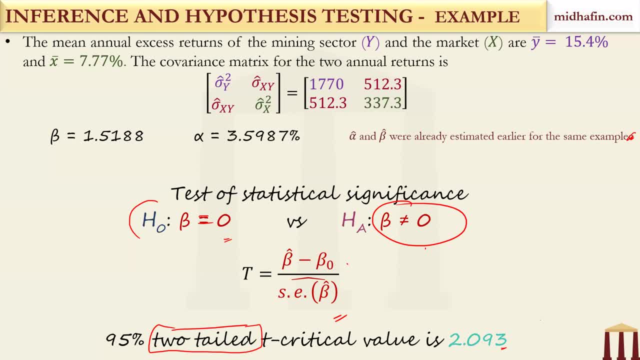 So it can happen. I mean, when we discuss multicollinearity- later we'll discuss this P-value part once again- and heteroscedasticity also, So let's continue. You understood P-value, let's continue Now. there are two models which they will give you. 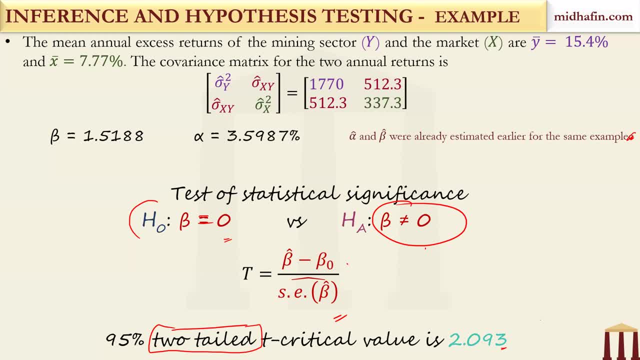 One is the restricted model, the other is the unrestricted model. So Again, since I'm assuming P-value should be less than 0.05, not greater than OK, P-value should be less than 0.05.. Got it. 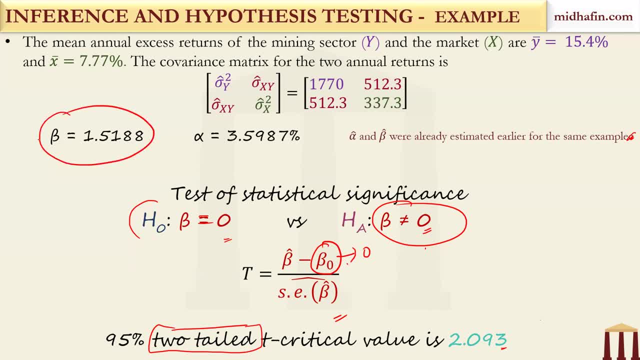 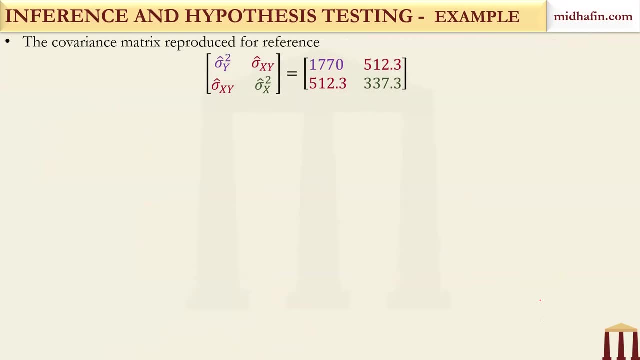 So I'm assuming that you are already aware of the capital asset pricing model, since you've done the course at least once, correct? So can I take that example of capital asset pricing model? Also, can I take the example of Fama-French model? 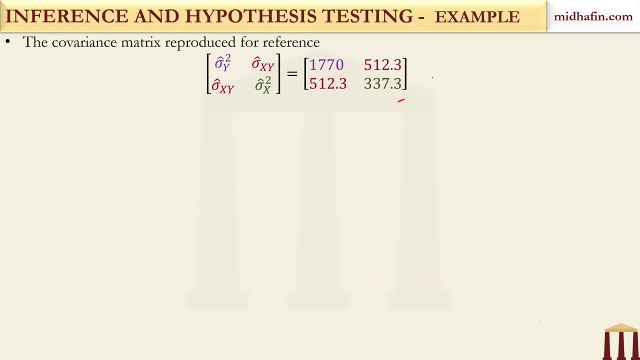 How many variables- independent variables- are there in the Fama-French model? Perfect Three: One is the market factor, one is the size factor, the other is the value factor. Correct, Three factors are there. And how many factors or variables are there in the CAPM? 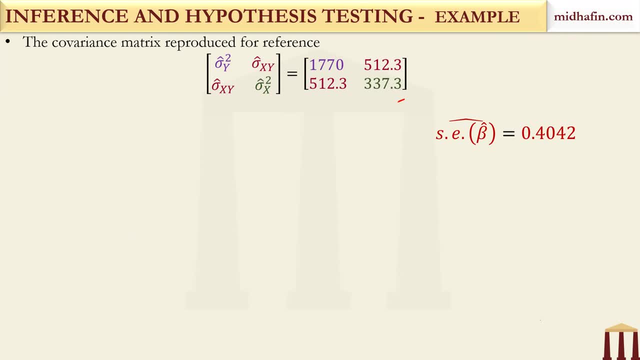 In the capital asset pricing Only one market factor, correct? So can I say that CAPM is a restricted version? Theoretically, CAPM is a restricted version of Fama-French, Correct? Yes, What is the number of restrictions we have to apply to Fama-French to give CAPM? 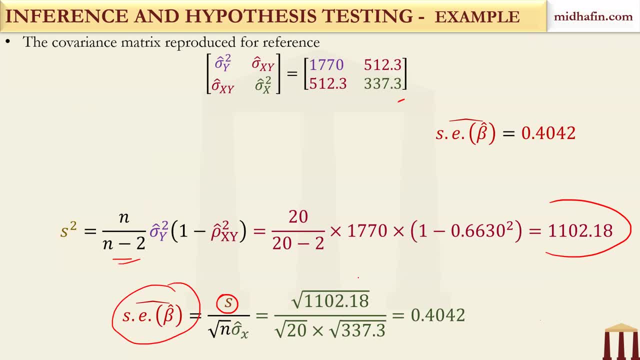 Two, Two, Perfect. This is what I was expecting. If you are already aware of this, then I can continue with this example. OK, So This part- this part was the earlier, the previous old curriculum F-statistic which I was talking about- 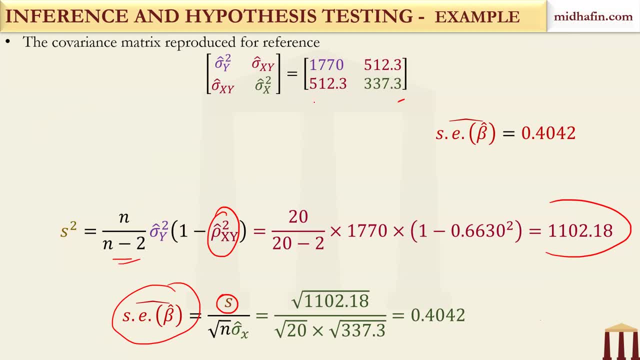 which will not be discussed right now. OK, this is the distribution anyways. So consider the Fama-French model. So, to imply restrictions, we will imply restrictions on which two factors Tell me: Size and value. Correct? So if we imply restrictions on size and value, 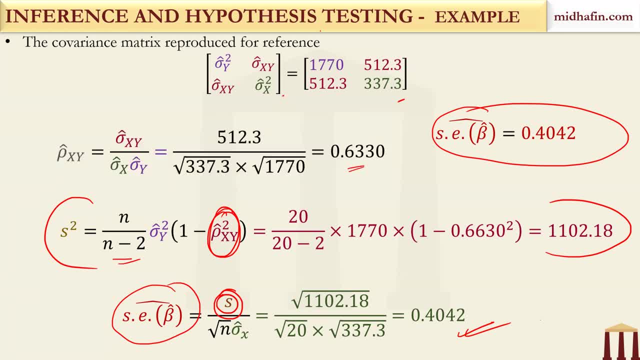 it means that Statistically we want that These two should be equal to how much, If I am applying this Zero? So if I make these two equal to zero, Can I say that Fama-French will convert to CAPM? 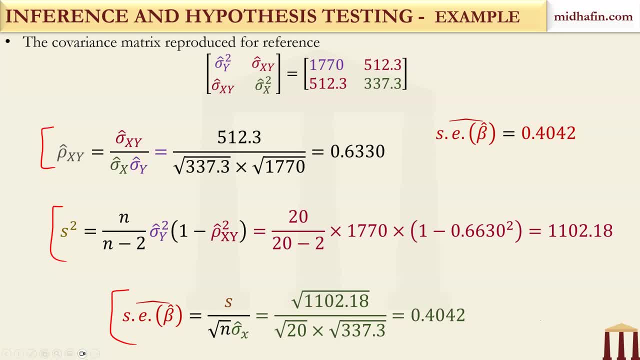 Correct. OK, So this is the null. this is the alternative hypothesis. So let's impose the null on the unrestricted model, which will give me CAPM. That is what I said. So CAPM gives you alpha plus, only the market factor plus is here. 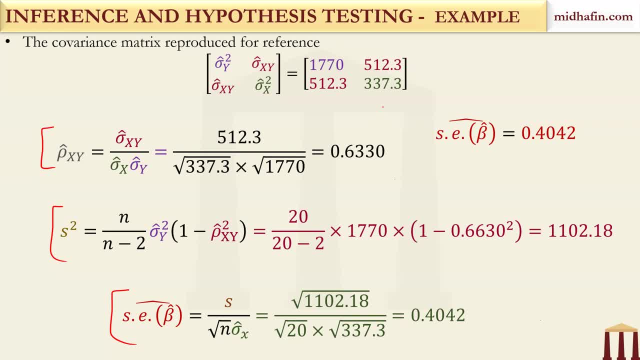 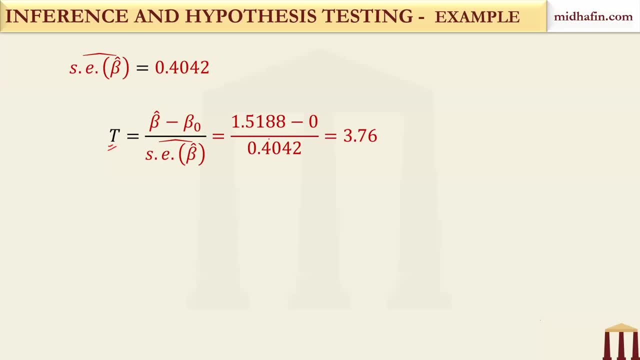 OK, let's continue Now. let's assume these are the parameters which are given to you: 40,, 200,, 50, Q equal to 2, KU equal to 3.. So remember, this is the formula that you have to remember. 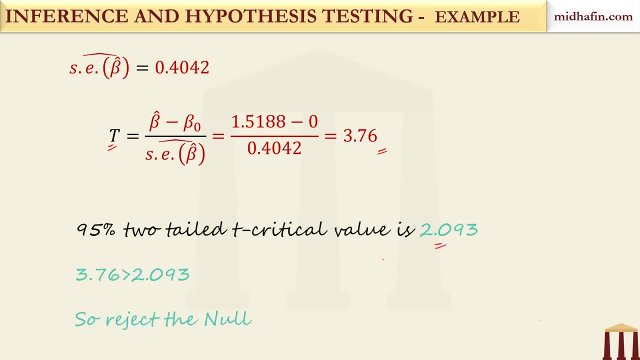 This is the formula you have to remember. OK, N, KU is important, then RSSR, RSSU, Q. what is Q? Q is the number of restrictions. OK, Q is the number of restrictions, KU is the number of variables in the unrestricted model.